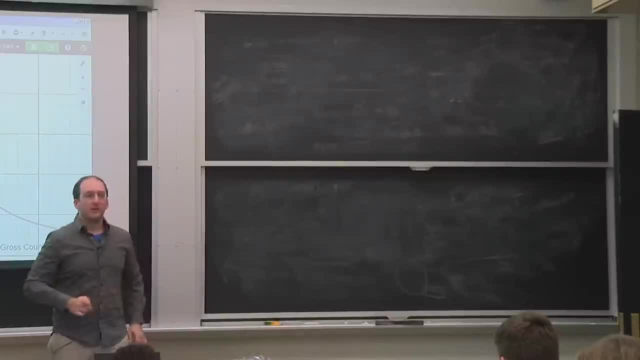 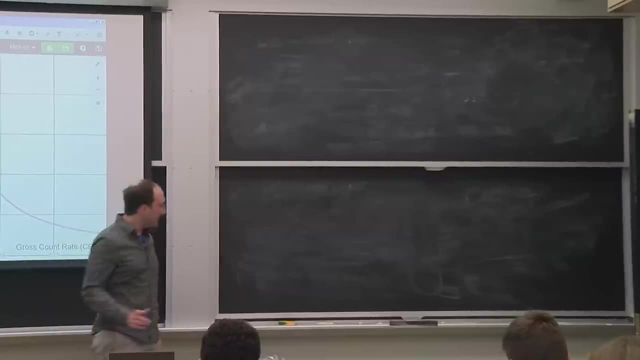 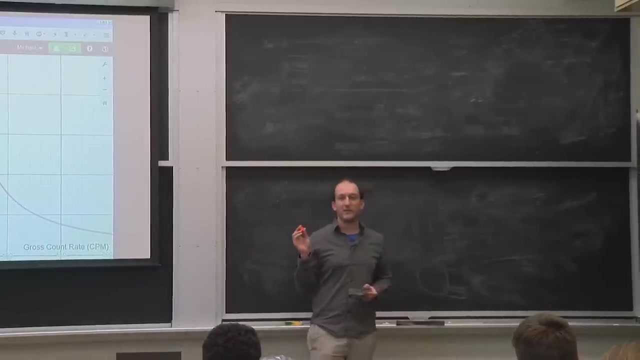 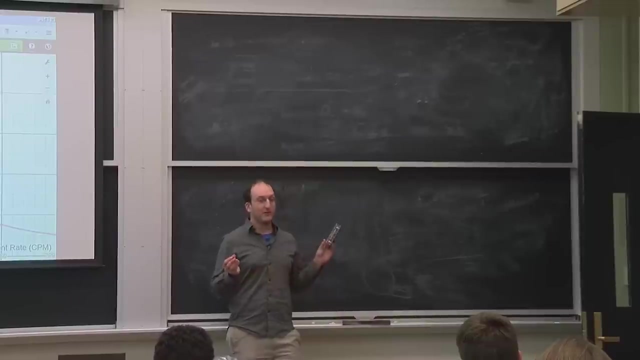 Okay, I think things have been getting pretty derive-y lately, so I wanted to shift gears to something a little bit more practical. So I started alluding to this hypothetical radiation source I might have right here, and things like: if you have a source of known activity, which we calculated yesterday, and you have a detector of unknown efficiency, how do you know what the efficiency is, How do you know what, let's say, your dose-distance relationship is, and how do you calculate all that? 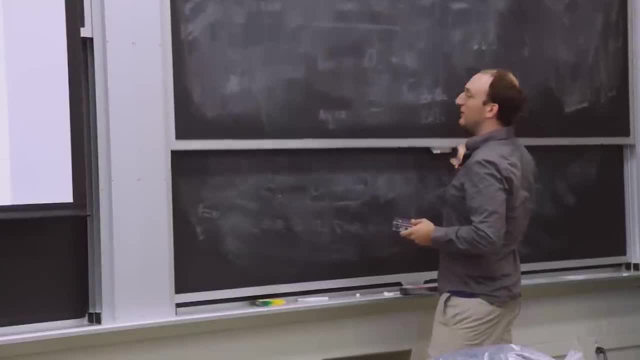 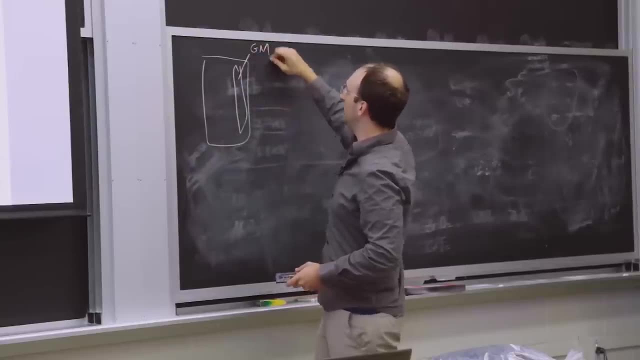 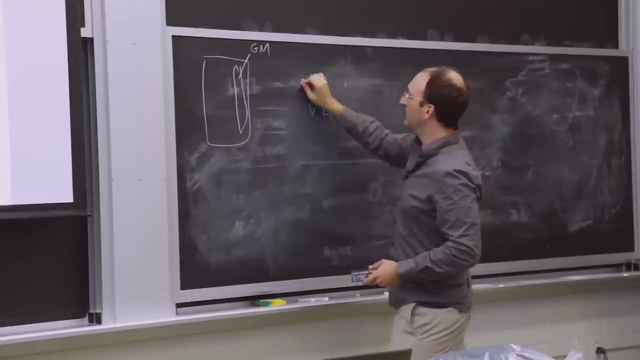 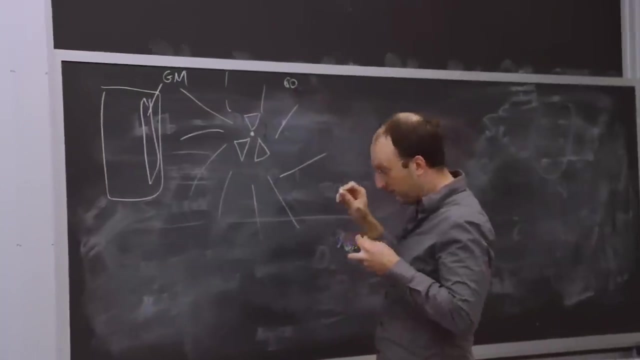 So let's take the general situation that we're starting to work out. Let's say we have a Geiger counter Right here, that's our GM tube, and we have a point source that's emitting things in all directions. Let's go with the stuff from yesterday. Let's say it's a cobalt-60 source- right, That was, it's now 0.5.. 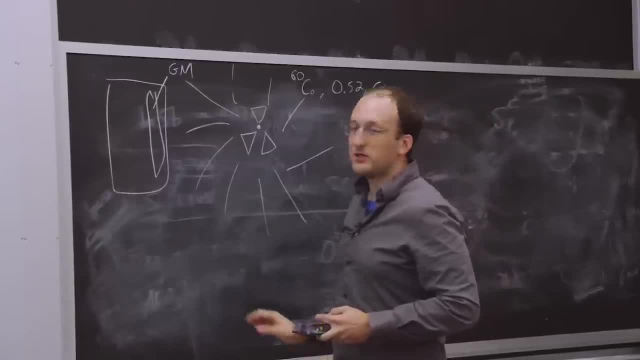 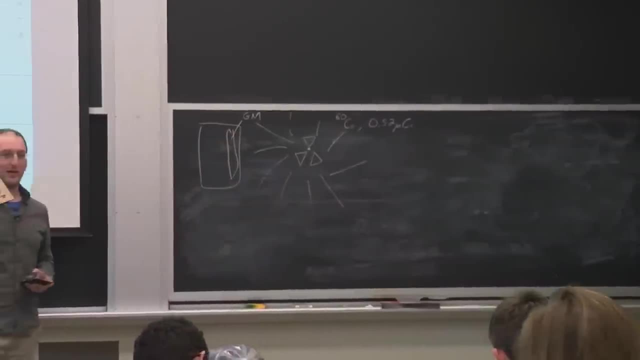 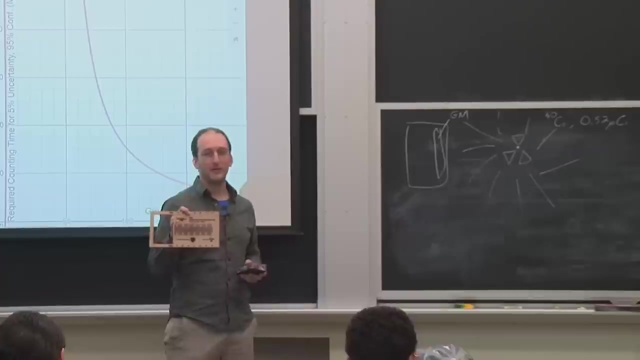 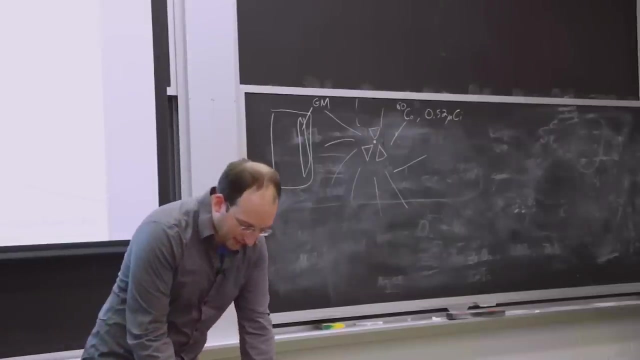 Let's go back to microcurie. The question is, how many counts do you expect in this detector when it's a certain distance away? So I've actually laser cut out a little Geiger counter jig from a previous class- and you guys can all do this too. Who here has been to the IDC before A couple, the International Design Center. So they've got a laser cutter that you can sign up to use, which is where I did this, and it's set to just take a Geiger counter and put your sources at some fixed distance away so you can discover the 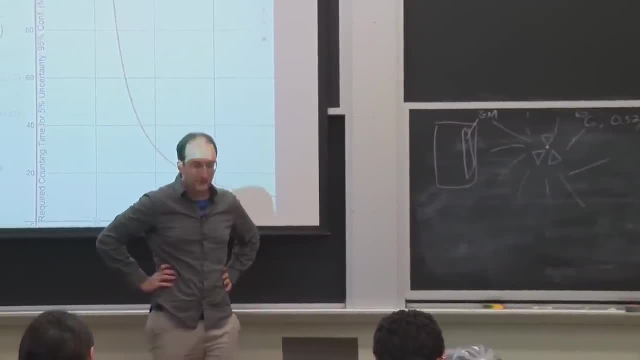 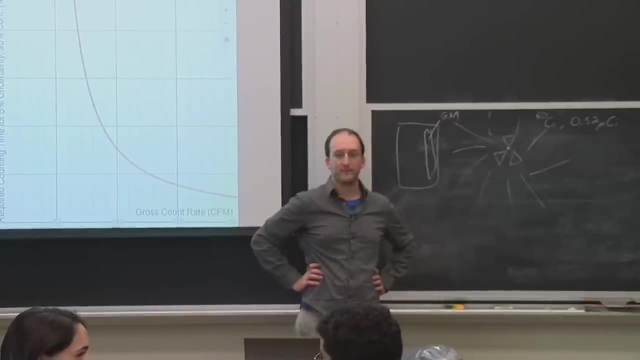 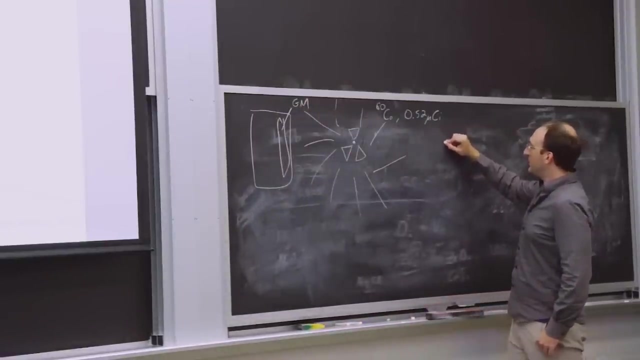 dose-distance relationship with things Speaking of, does anybody know what the relationship is between dose and distance, or measured activity and distance? Yeah, Luke, Whatever r is here, Close It's. let's say the measured activity would be proportional to 1 over r squared. Now, who knows where this comes from. 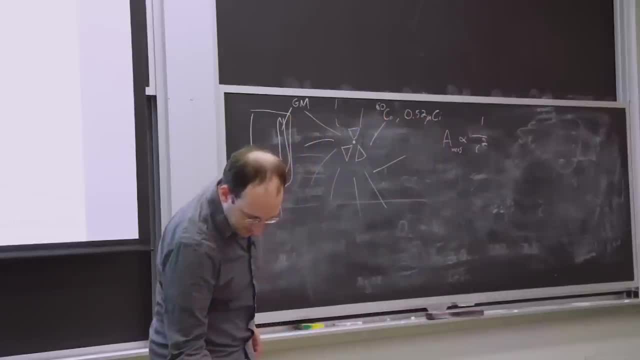 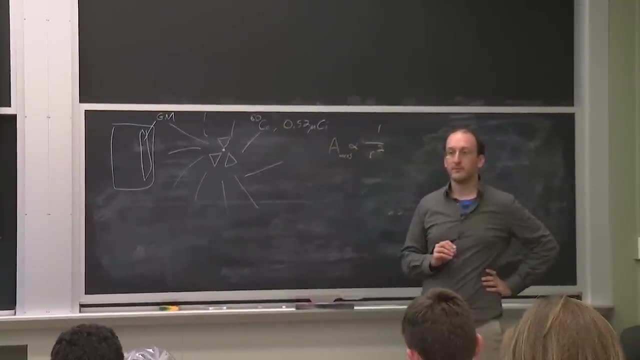 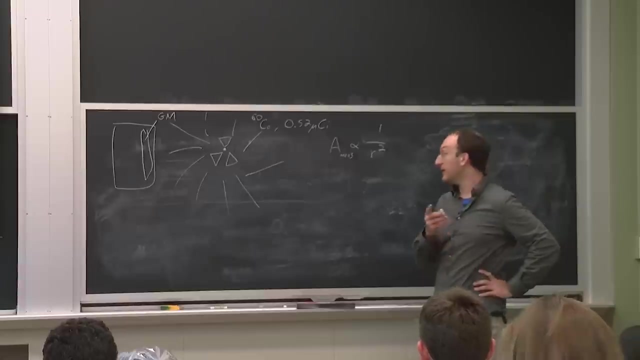 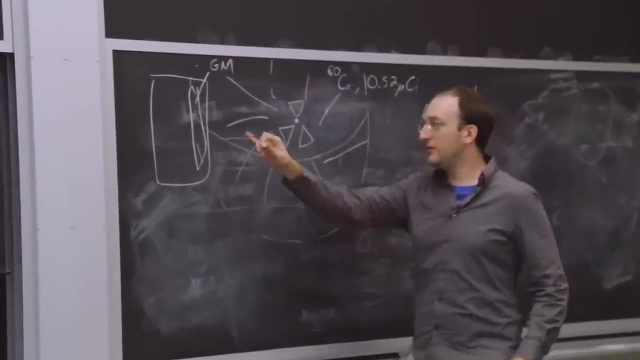 I'll move the source a bit away to lessen the, Lessen the beeping. Yeah Well, the flux of particles coming out is just the same over the surface area of the other way and the sphere is 1 times r. Yeah, exactly. If you were to draw a hypothetical sphere around the source right here, then you've got a, let's say you've got a detector that's roughly rectangular with a fixed area. 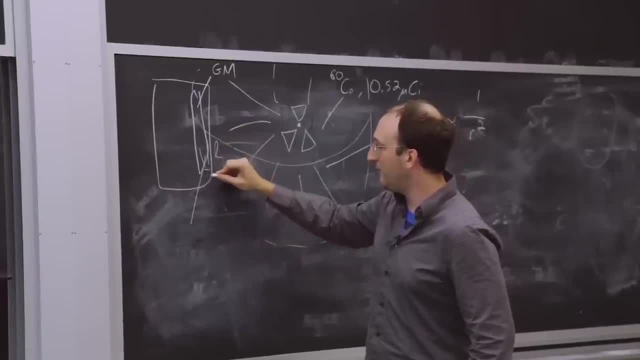 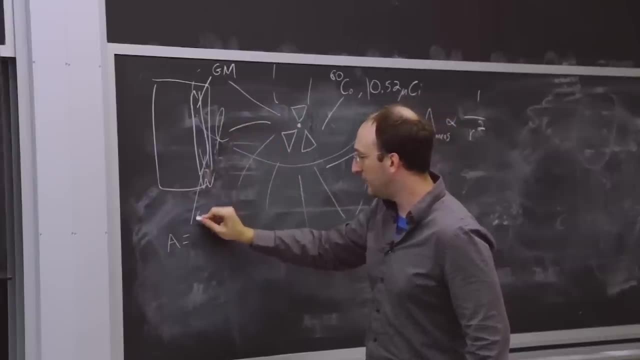 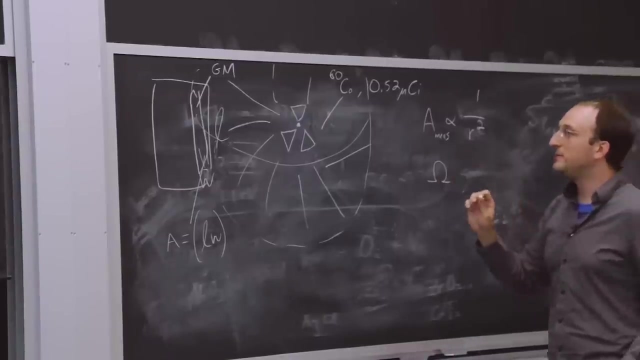 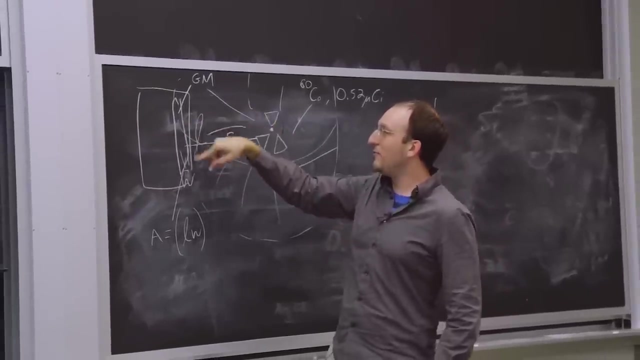 Let's say it's got a half length L, L and a half with W. Then the area- or I'm sorry, let's just say length L with W, the area would be just L times W And actually what Chris mentioned as the solid angle subtended by this detector right here, as, in other words, at a certain distance r away, how much of this sphere, how much of the area of this sphere does this detector take up? 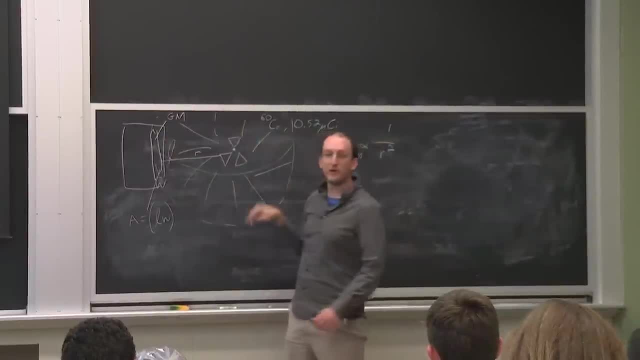 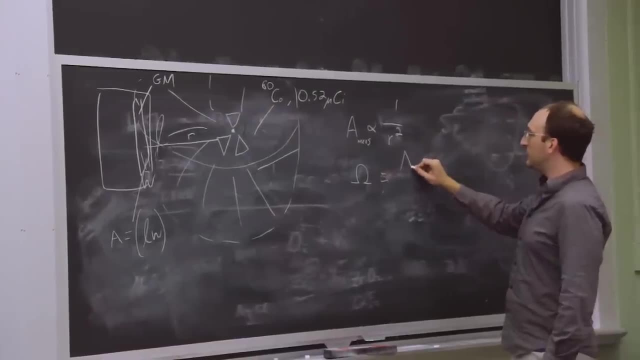 In other words, how many of these gamma rays are going to go in a different direction. In other words, how many of these gamma rays are going to go in a different direction than the detector versus how many will actually enter the detector. And a simple formula for the solid angle is just the surface area of whatever you've got over r squared. 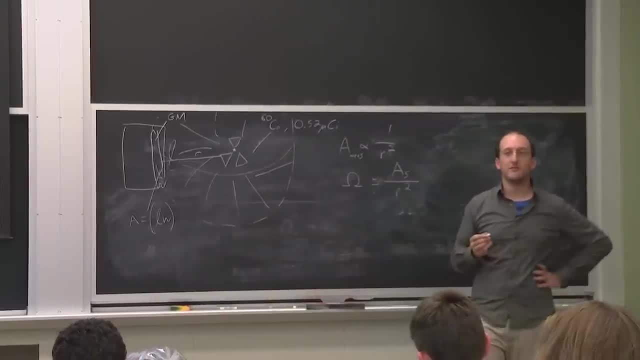 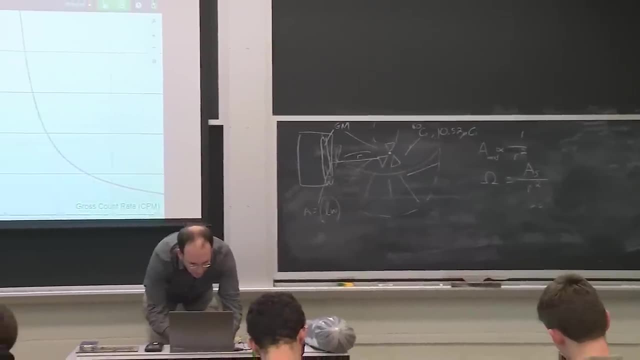 It's kind of a. it's a pretty good approximation to the solid angle of something for very long distances, And it's probably the one that you'll see in the reading, but I wanted to show you the actual formula, in this case for a rectangle. 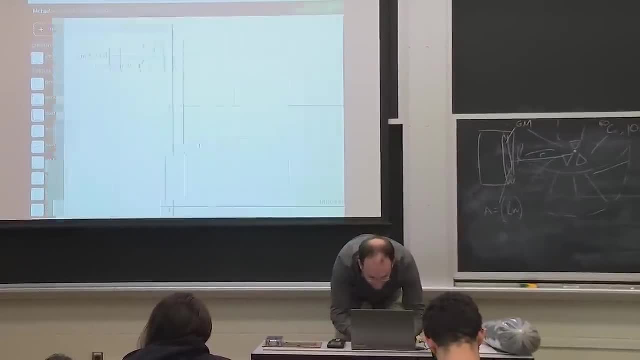 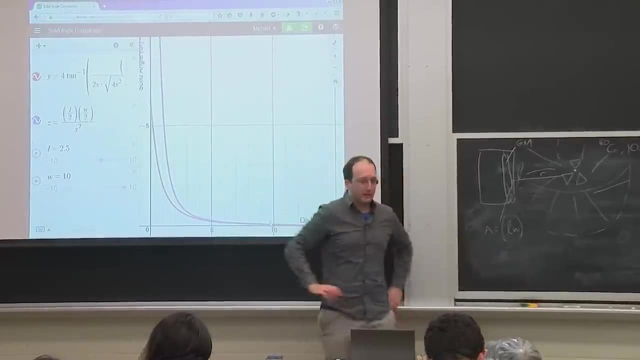 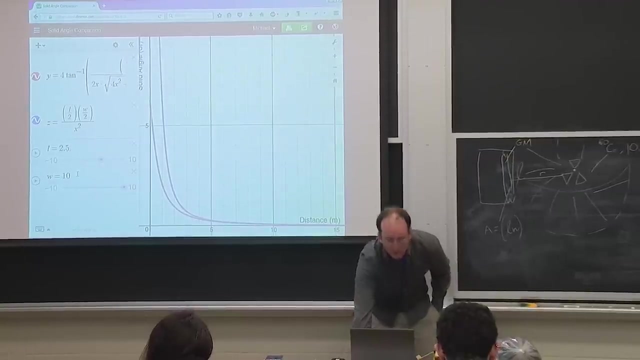 Solid angle comparison. Good, that's up there. So on the let's say, on the x-axis right here, this would be distance from the source to the detector in meters, And I've said that we've got some sort of a detector that is 2.5 by 10 meters in size. 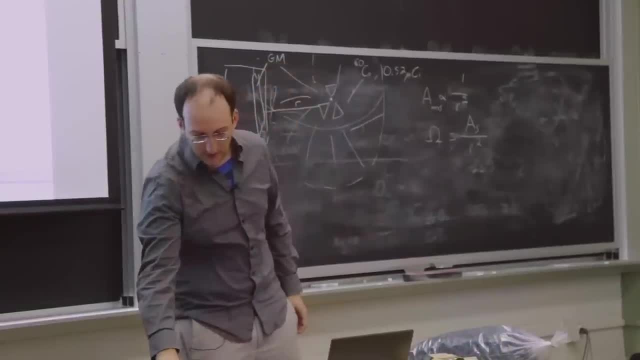 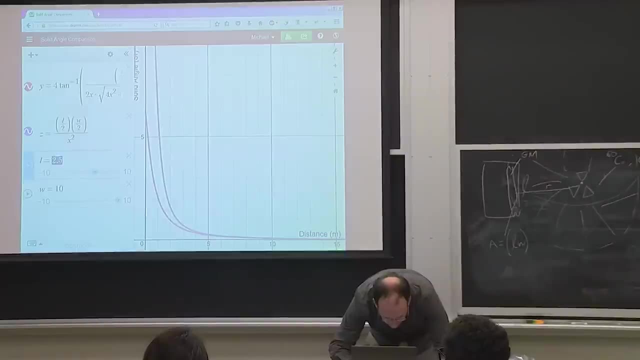 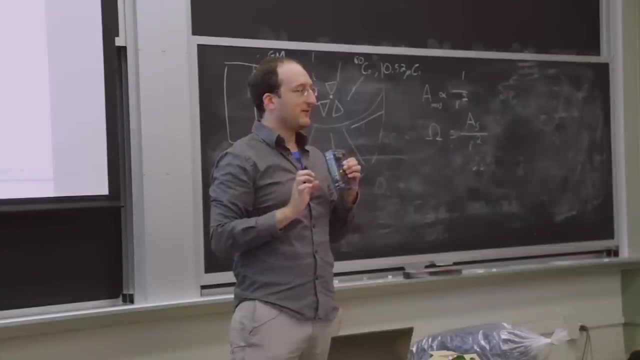 That's an enormous detector. Let's actually switch it to the units right here. So this is roughly 10 centimeters long. So let's change our length to 0.1.. 0.1.. And what's what? do you think the width of this Geiger counter is in meters? 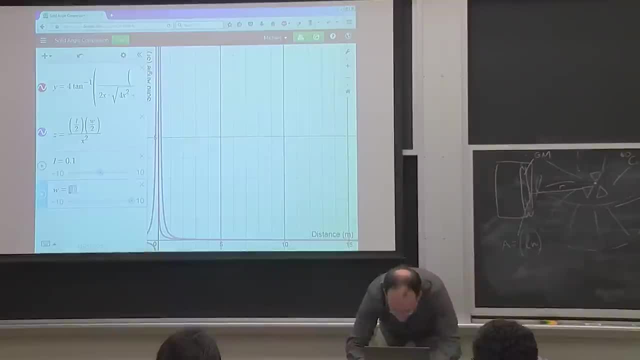 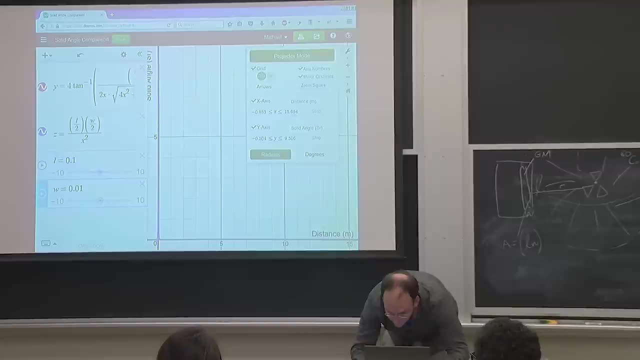 Let's see Centimeter 0.01.. We're going to have to change our axis so we can actually see the graph. So instead of looking all the way up to 15 meters away, let's look one meter away, maybe less. 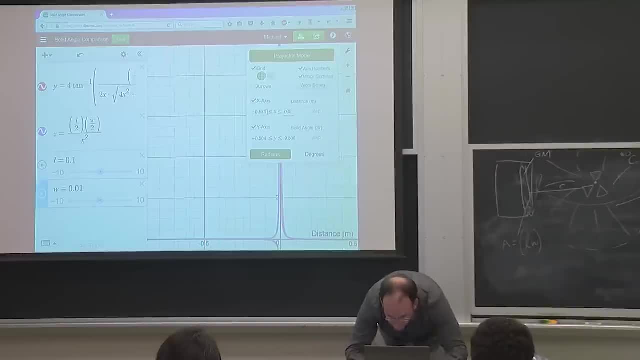 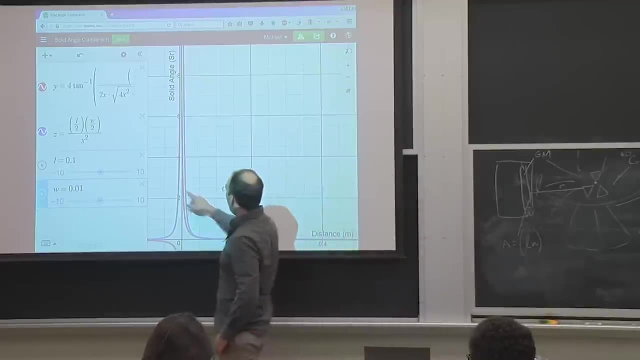 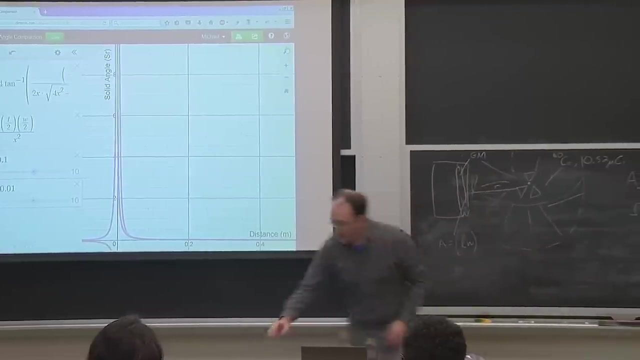 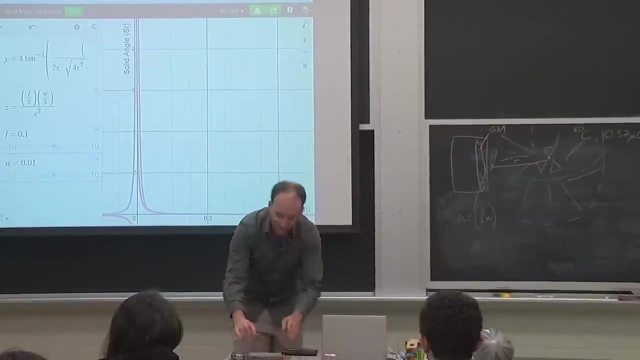 This whole thing is probably 50 centimeters, And we'll take a look there And what we notice is that, except for Extremely short distances, this approximate formula for the solid angle- or in other words, if I were to draw a sphere around this source, that's the radius of the distance between the source and the detector- how much of that sphere's area does the detector take up? 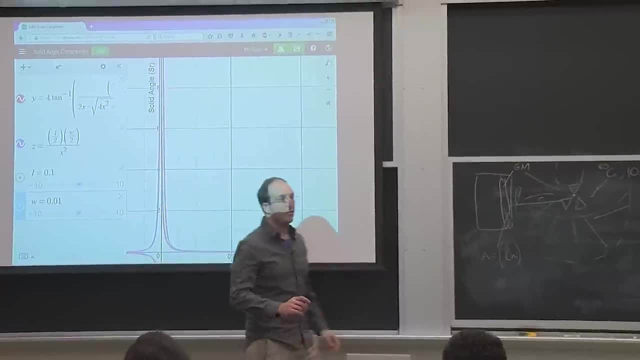 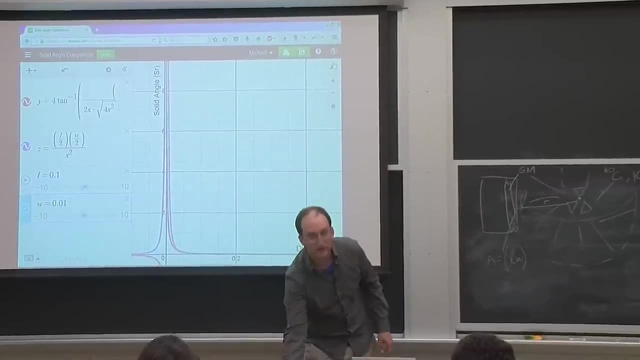 This actual formula, this approximate formula. the blue curve is a pretty good approximation of the red curve until you get really, really close to like 5 centimeters away, or about this distance right here. Does anyone know why this formula would break down? 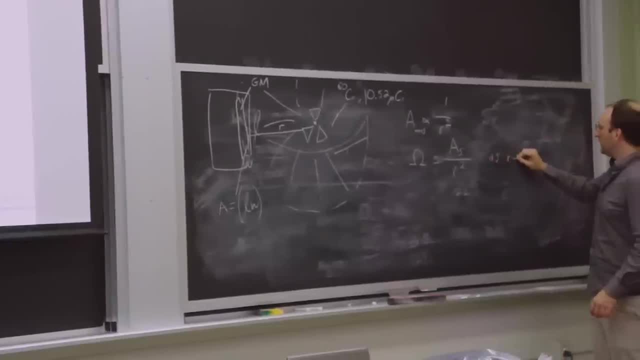 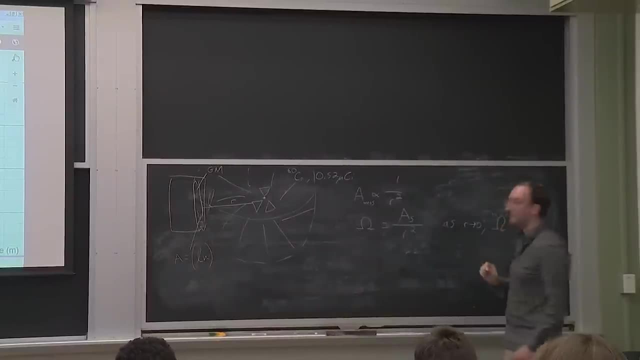 What happens as r goes to 0?? What happens to our solid angle or our approximation, for our solid angle Goes to infinity right? Can a detector actually take up infinity area on? well, anything, Never mind that unit sphere? Not quite. 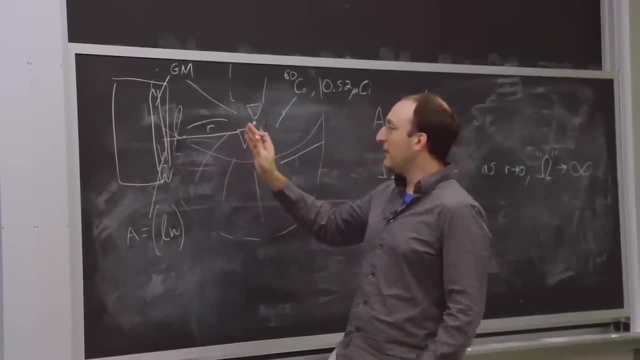 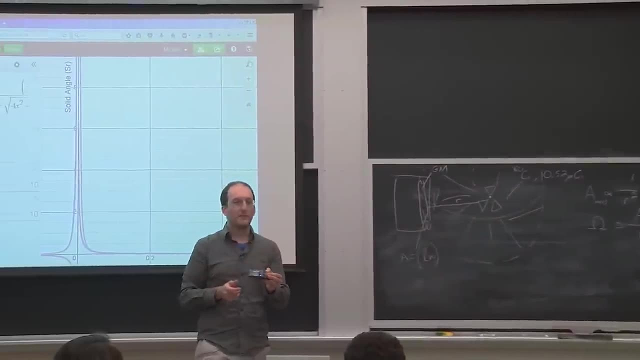 Not quite. So let's look at this detector and bring the radius down to 0, so that the source and the detector, if not counting for the thickness of the plastic, were right upside each other. If that solid angle went to well, infinity, then the count should go to infinity and does not compute. 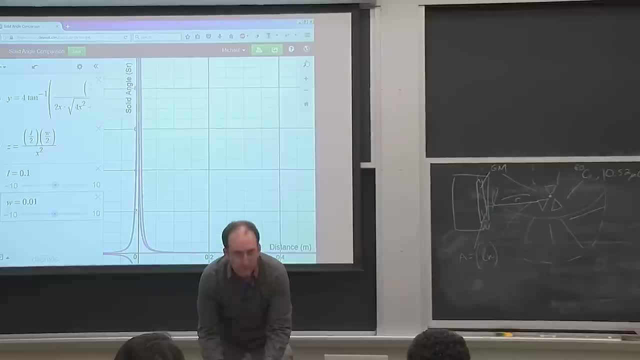 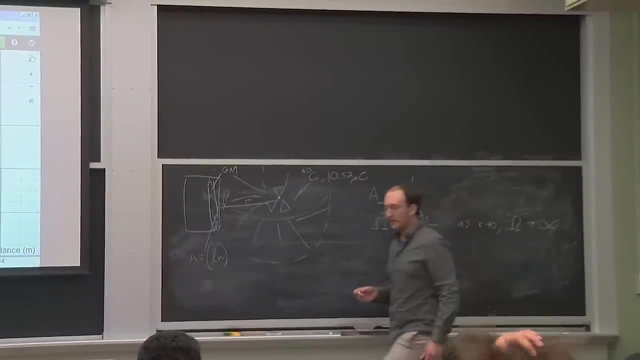 Does anyone know how many? first of all, who here has heard of solid angle before? So a little more than half of you. So solid angle's kind of the that's getting clicky. I'm going to turn that off. Solid angle's kind of the analog to regular old angle, except in 3D. 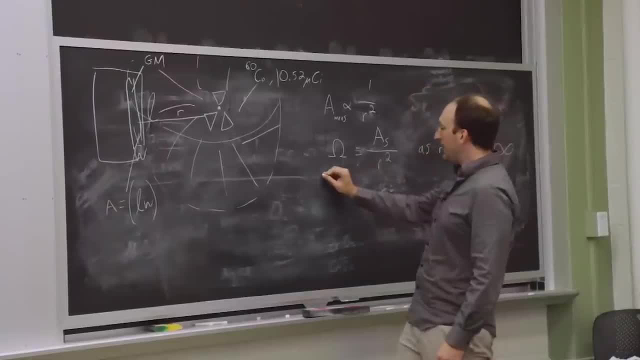 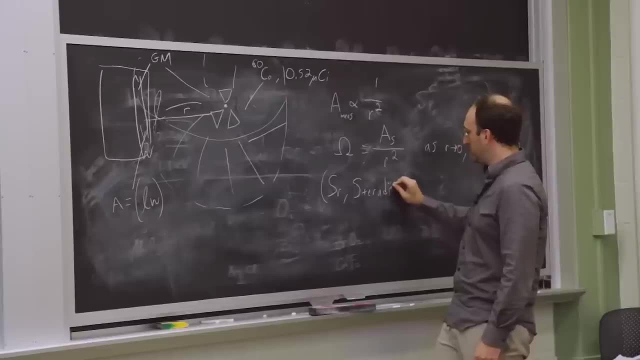 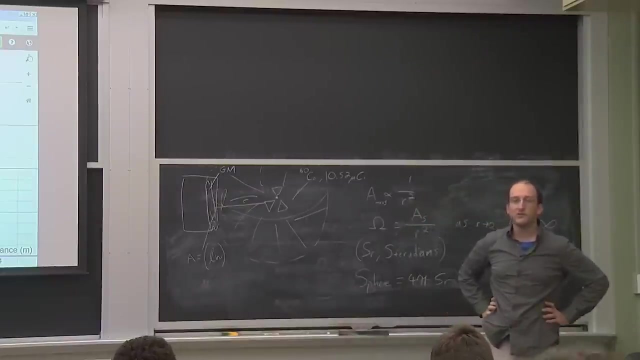 So, instead of looking at things in radians, this has the unit of what's called steradians- Steradians With a full sphere taking up 4 pi steradians. Interestingly enough, 4 pi is also the surface area of a unit sphere with radius of 1.. 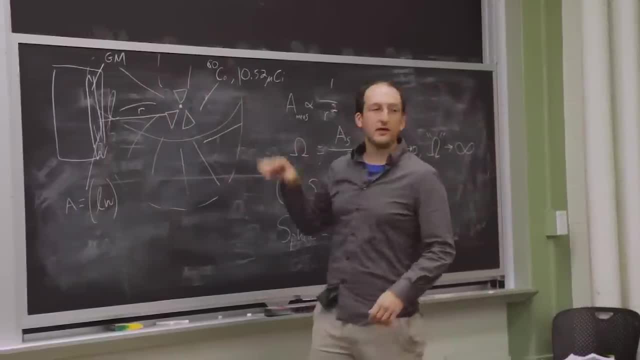 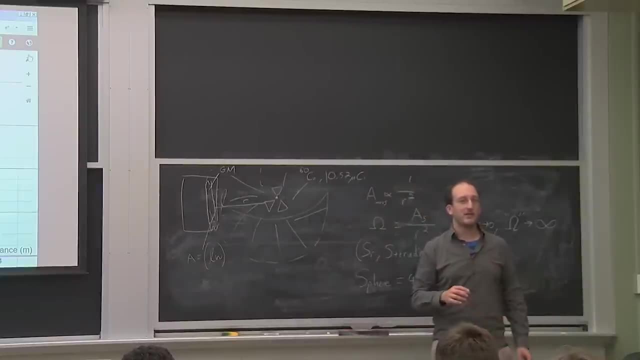 So that's where this comes from. If something were to completely cover a unit sphere, like if you were to, let's say, encase a light source in tinfoil completely and say how much of that solid angle does the tinfoil encase? it would be 4 pi steradians. regardless of the size of the sphere, how much tinfoil you had to use. 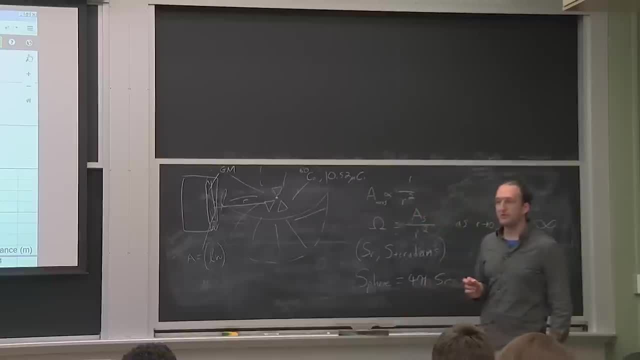 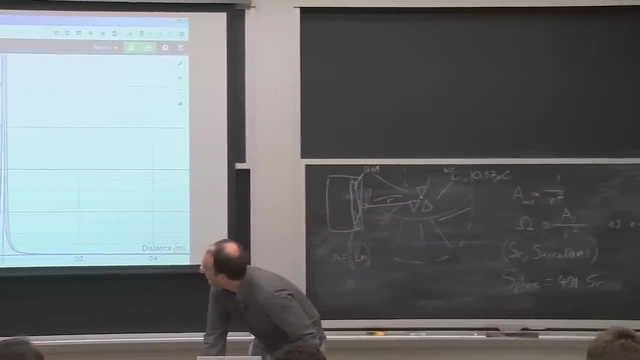 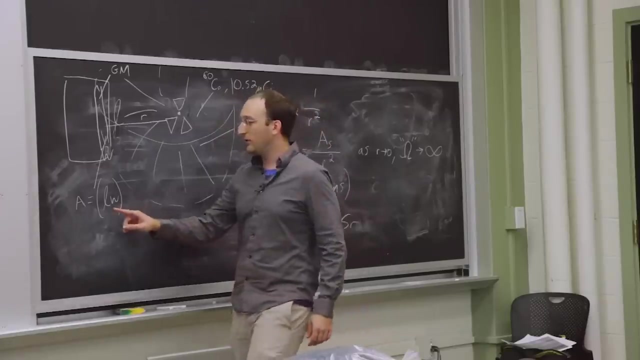 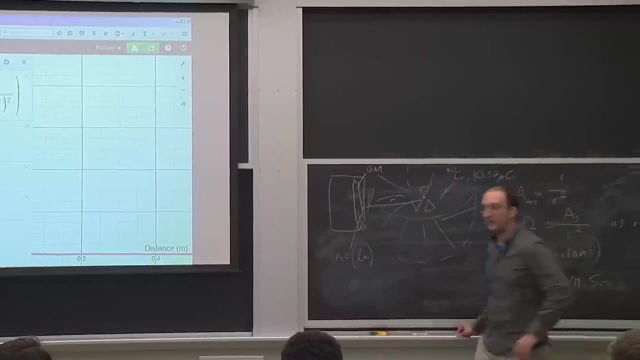 So this pretty simple formula isn't the best approximation for it And I'm not going to go through the derivation because, like I said today is going to be of a more practical nature. There is a more complex and rigorous formula for the solid angle of something, let's say, in this case, a rectangle of length l and width w, from a certain distance r or, in this case, on our graph, x, away from the sphere. 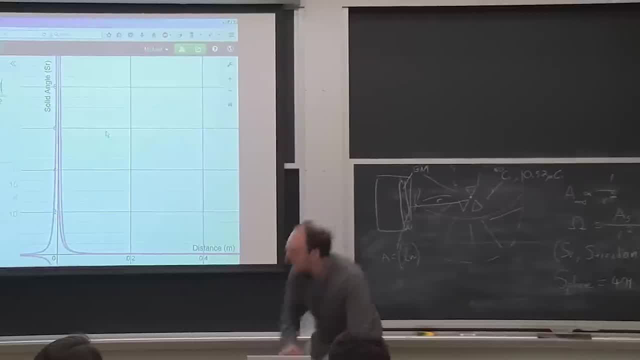 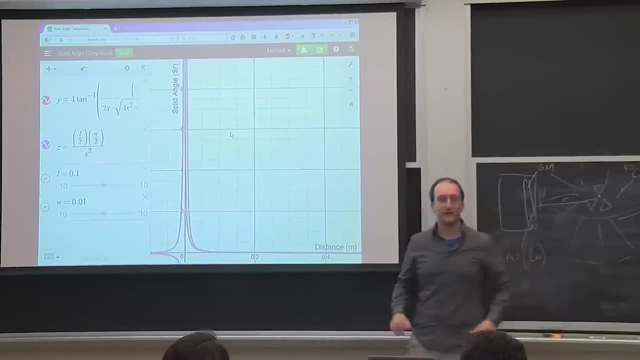 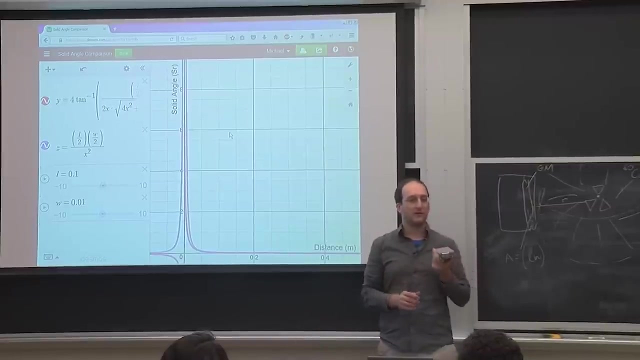 And you can actually see that red curve right there Once you get to a few centimeters away. it's pretty close. Anyone want to guess what the maximum value of the red curve is? If I take this source? If I take this source and slam it right up next to the detector, how much of the detector is? I'm sorry- how much of that sphere is the detector subtending? 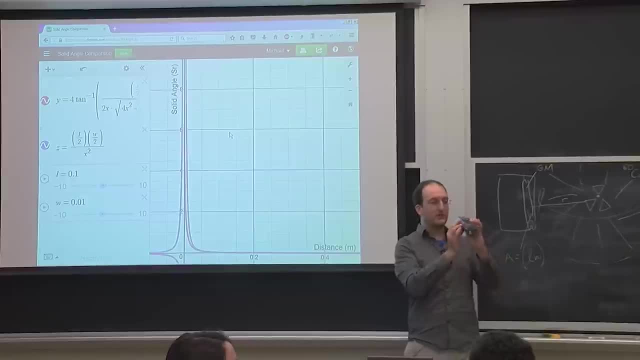 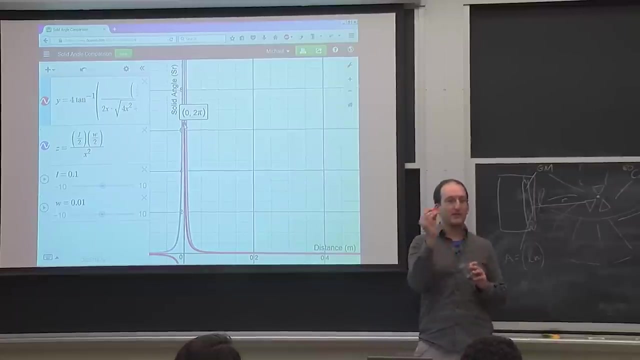 2 pi, half the sphere, Because it's, let's say, this whole side of the source is completely obscured by the detector and this whole side is free to move. And if you look really closely, yep at 0, the correct formula does give you 2 pi steradians, which is to say that half the gamma rays leaving this source would enter the detector, subtending 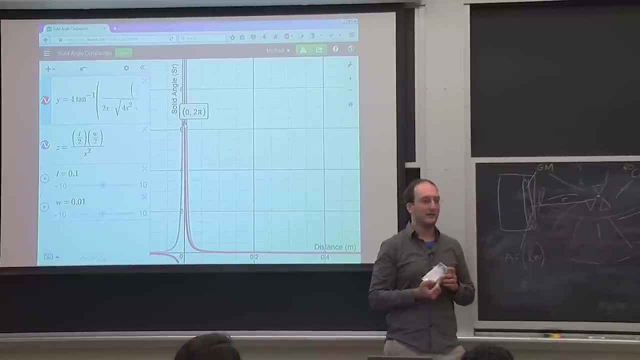 I didn't say anything about get counted yet. That's where the detector efficiency comes in And that's something we're going to be measuring today, which is why I have my big bag of burnt bananas. These are the ashes of roughly 50 pounds of bananas charred to a crisp at about 250 Fahrenheit for 12 hours in most of the dorms and a couple of the frat houses. 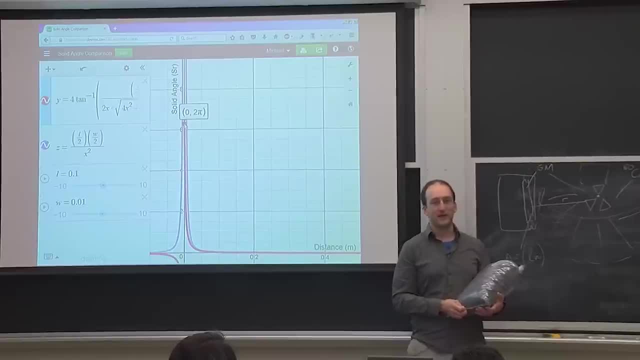 So last year I had the students- everyone- take home about 50 pounds of bananas, or 50 bananas, I forget which one. It was a lot And we did it. It was a lot and we did some distributed labor. So everybody peeled the bananas, put them in the oven. 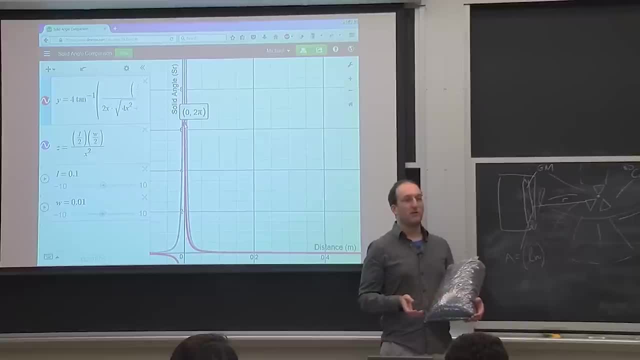 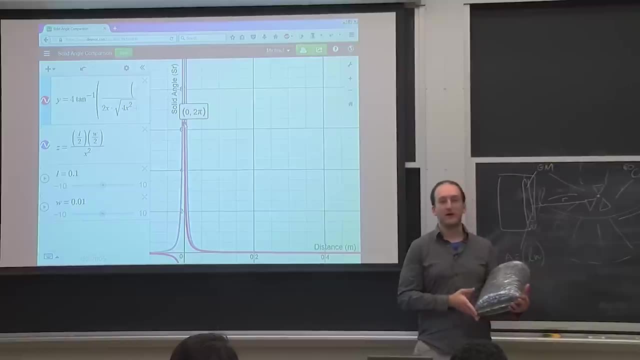 baked them, separated off the tin foil, baked off as much water and sugar as possible to concentrate the potassium-40 in the bananas. So there's a reason I've been using potassium-40 as a lot of examples in this class: because you're full of it. 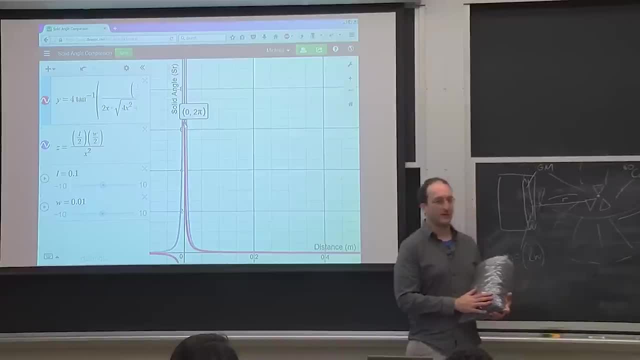 That's pretty much the short answer of it. If you eat bananas- which I think most of you guys do, you're intaking a fair bit of radioactive potassium, which is a positron emitter and also does electron capture and all that fun stuff. 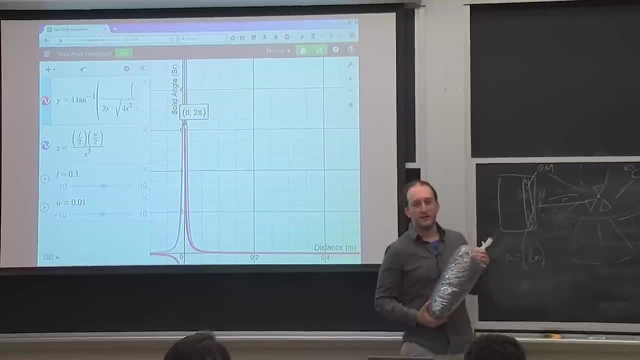 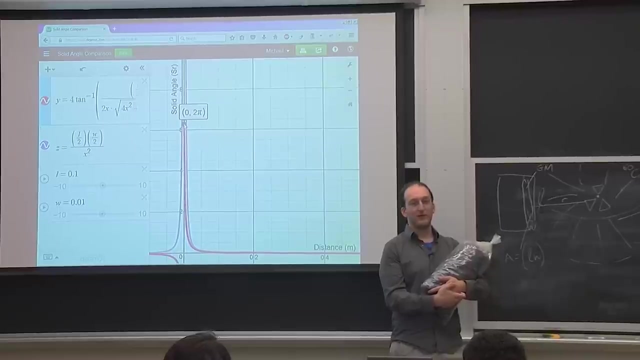 So today what we're gonna be doing is calculating the activity of one banana, But that's kind of a very difficult thing to do. So anyone know how radioactive one banana actually is in any units at all? Whatever it is, it's very, very, very, very little. 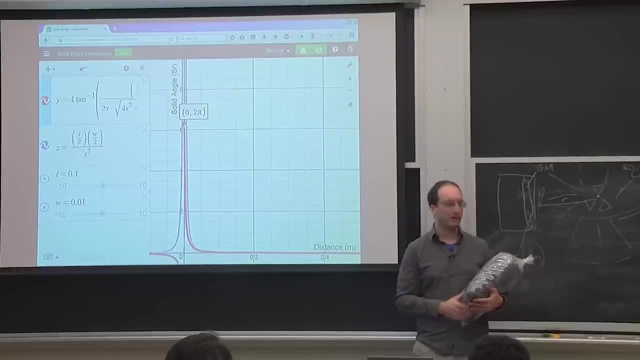 One banana contains a minuscule but measurable amount of radioactivity, And one of the ways to boost your confidence on any sort of radiation measurement is to boost your signal strength or to boost your counting time. And because I don't want to count for the next seven years, 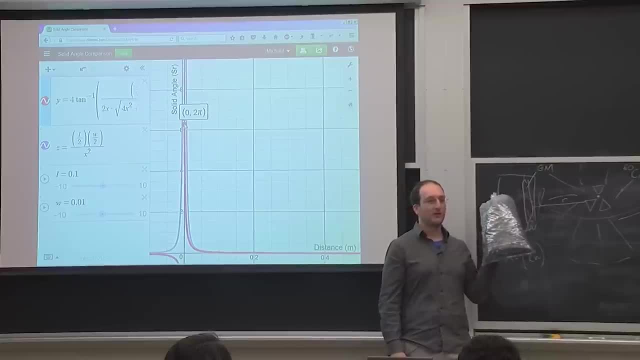 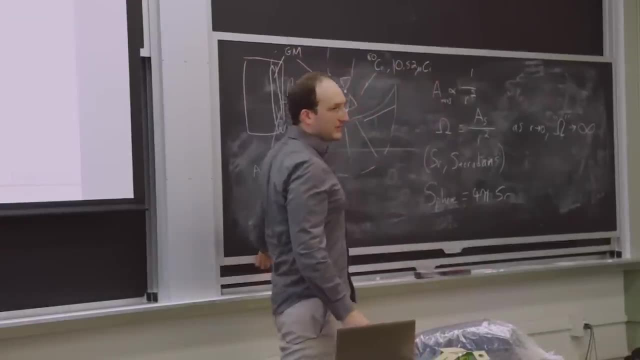 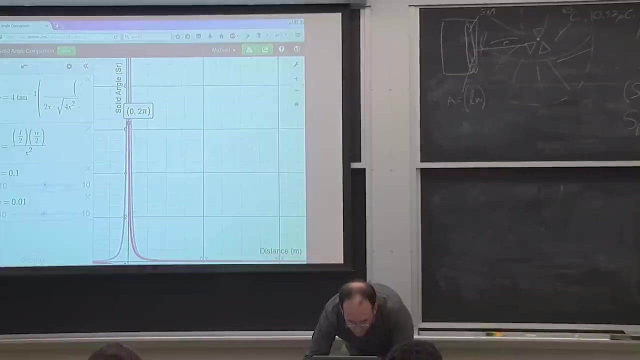 we've concentrated the ashes of 50 pounds of bananas in here to boost your signal strength, which is going to boost your count rate, which is the intro I want to give to statistics, certainty and counting. So let's take one of the homework problems. 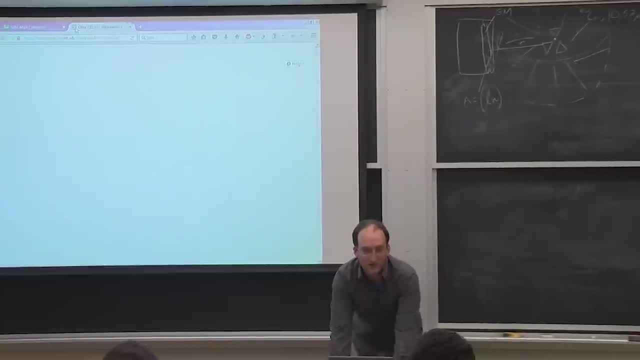 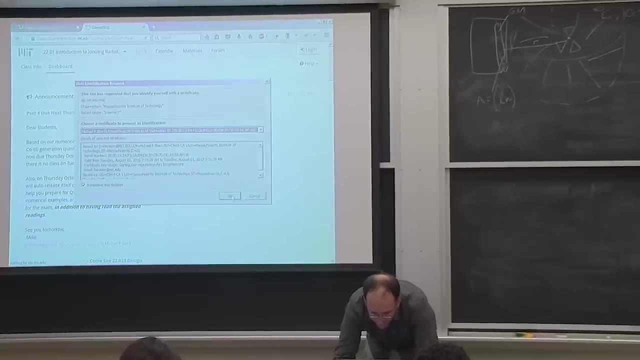 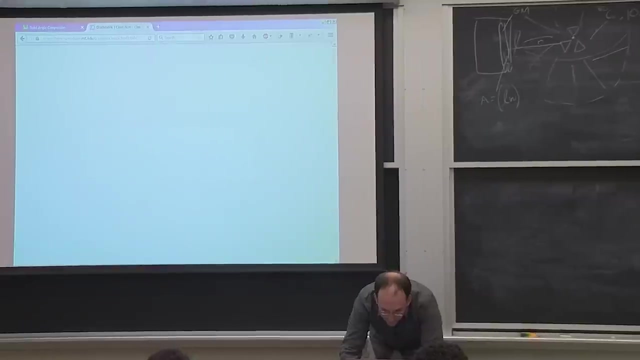 as a motivating example. You guys, did anyone notice the extra credit problem on the homework? Let's start talking about how we go about that. That should motivate the rest of the day, So I'll pull up that problem. set number four: 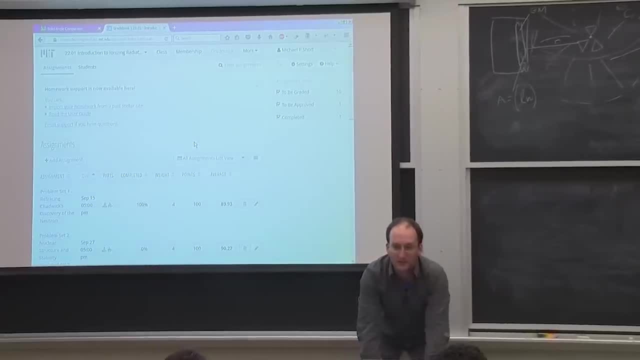 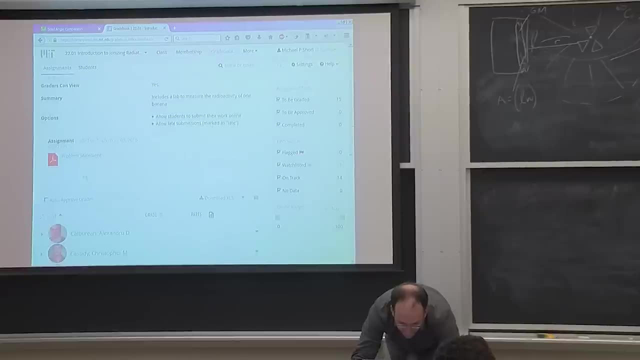 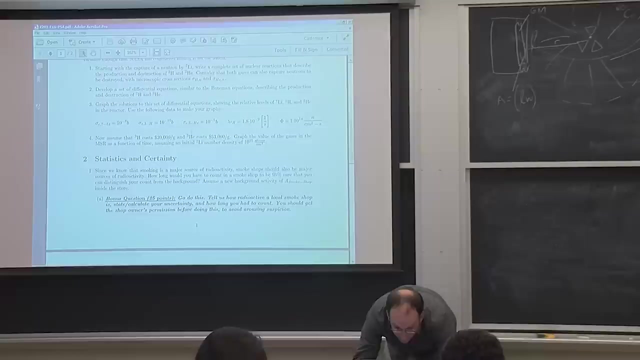 which, by the way, is due Thursday not Tuesday, because we have no class on Tuesday. That was a surprise to me, but whatever, I'll still be here. We don't get holidays, Just you guys. So bonus question. 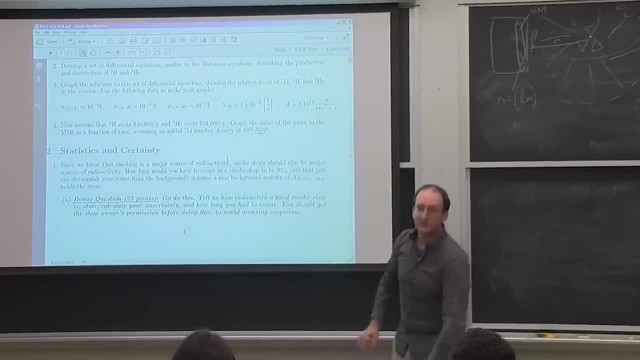 Go do this. So we all know that smoking is a major source of radioactivity And if you think about it, it's not just the smoke that contains those radiation particles, It's got to be the cigarettes, cigars and other smokables themselves. 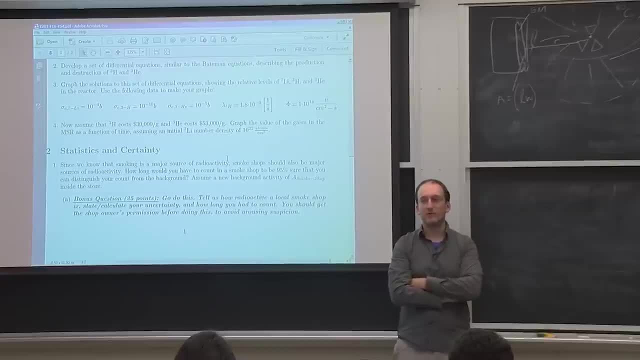 And so I was thinking there's no better concentrated source of smoking radioactivity than a smoke shop. There's one out at Alewife at the end of the T. There's probably some closer to campus, But I know there's a whole bunch. 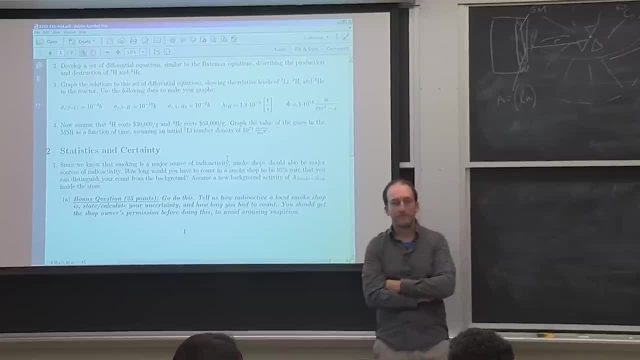 that are T-accessible, And so I was thinking it'd be neat for us to find out how radioactive is it to work in a smoke shop, Because there's all these radon decay. Oh yeah, You actually know. No, you have to be 21 to go into a smoke shop. 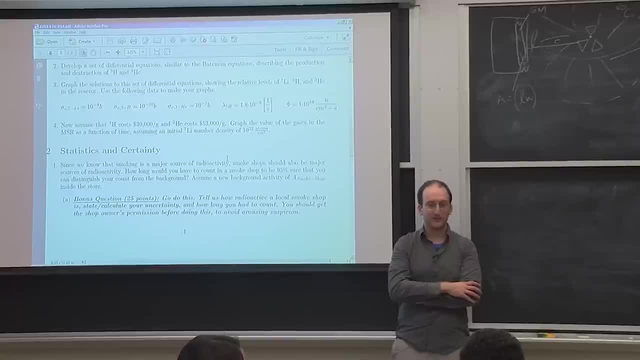 Are you serious? But you got to be 18 to smoke. Yeah, it's like a Cambridge Boston law Interesting. We may have to leave the city for this one. What about Somerville? Think It's still. you're not allowed to go in there either. 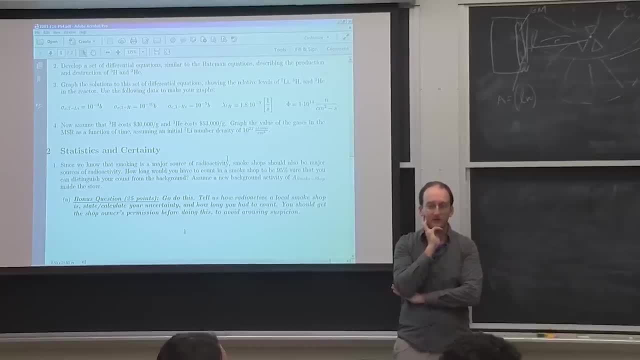 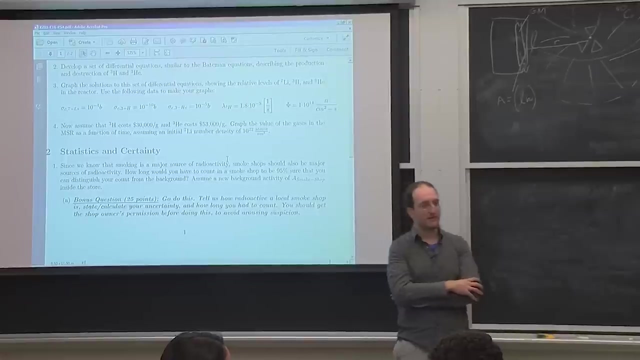 It's all Massachusetts now. Wow, Yeah, I hope you can find them. It's still like it's like town to town. Mostly the Boston area is 21,, but once you leave Boston It varies. Yeah, I don't think it is where I'm from, from Swampscott. 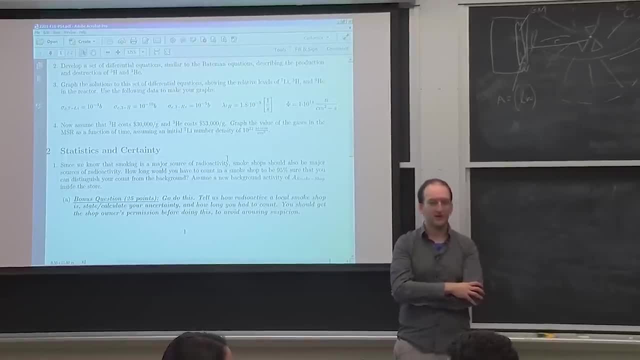 I don't think it's 21. But that's kind of up on the commuter rails. You don't want to go to Swampscott. At any rate, I would think that. OK, it's probably a fairly radioactive place to work. 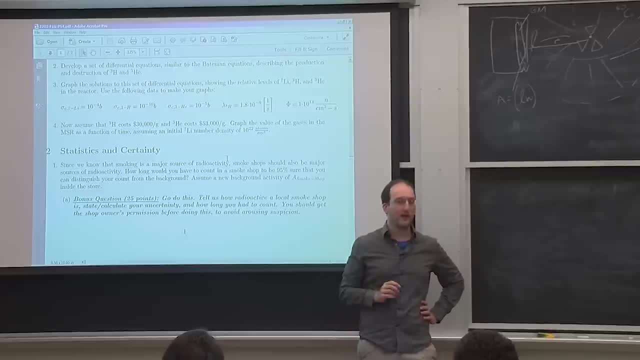 But the question is: how long would you actually have to bring a detector in and count in order to be sure that there's any sort of measurable difference? And so, without deriving all of the stuff about binomial Poisson and normal statistics, I'll 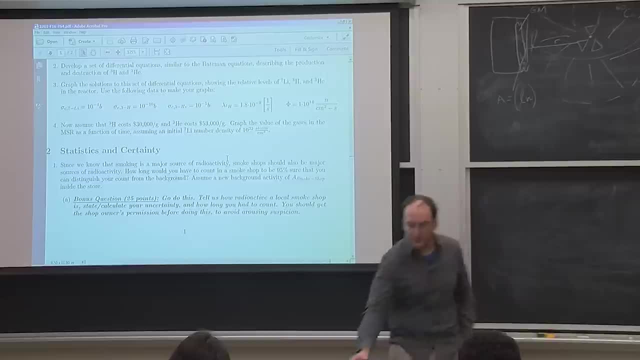 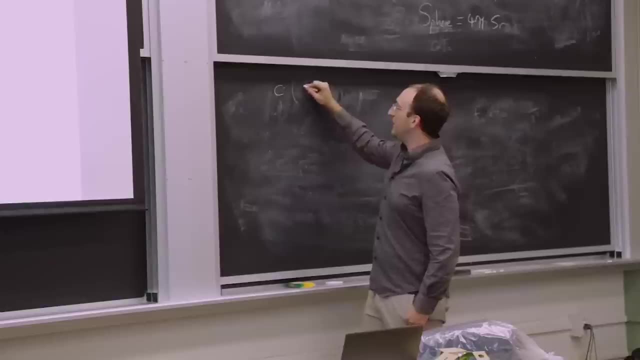 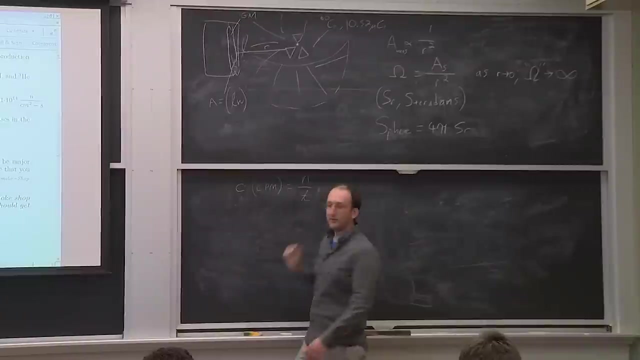 say that's in the reading for today. I want to show you some practical uses and applications of this stuff. Let's say you were to measure some count rate in some experiment And we'll put this in units of counts per minute, which would be the number of counts divided by the counting time. 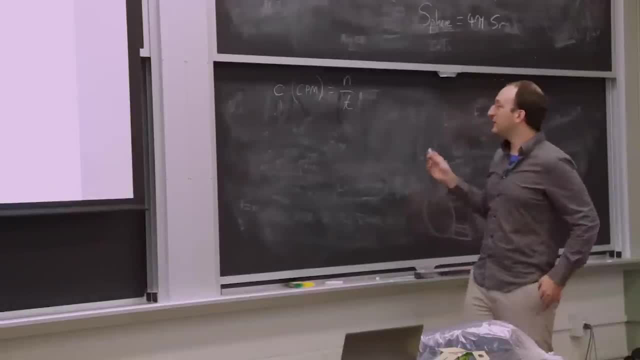 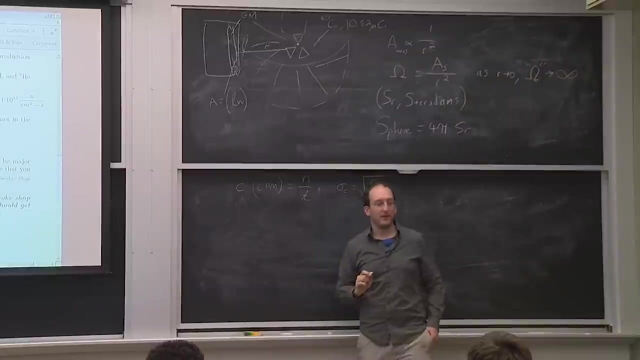 That's about as simple as it gets. But from Poisson statistics you can say that the standard deviation of that count rate is actually just the square root of the count rate divided by time. And that's kind of the simple thing right here. 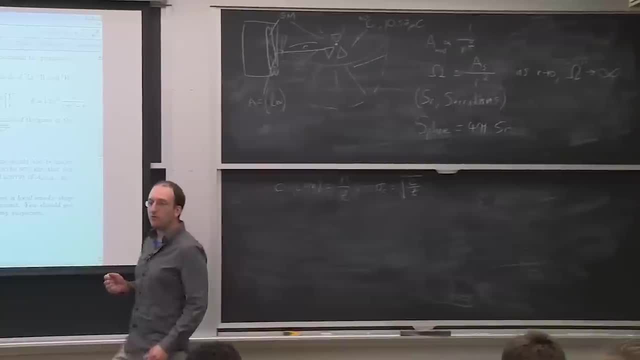 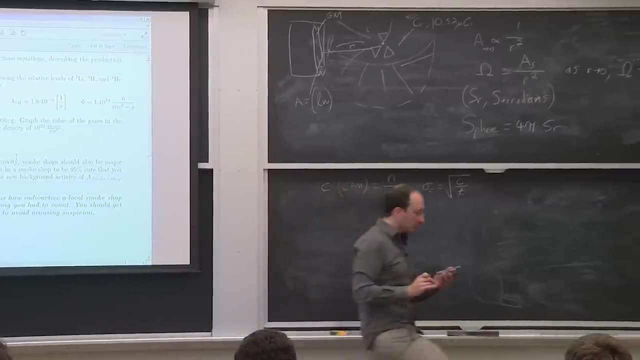 But usually in these sorts of experiments if you want to know how much more radioactive is one place than another, you have to take a background count. So if I wanted to know how much activity that source was giving off? there is lots of background radiation. 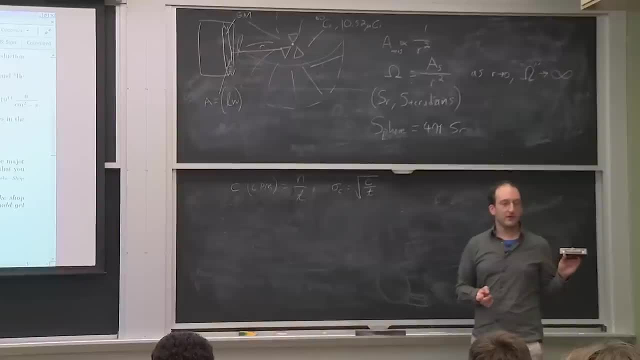 that will be going over in about a month. I would have to sit here for quite a while and wait for the slow clicks of whatever background radiations in the room to get enough of a count rate going on. You can imagine the slower the count rate. 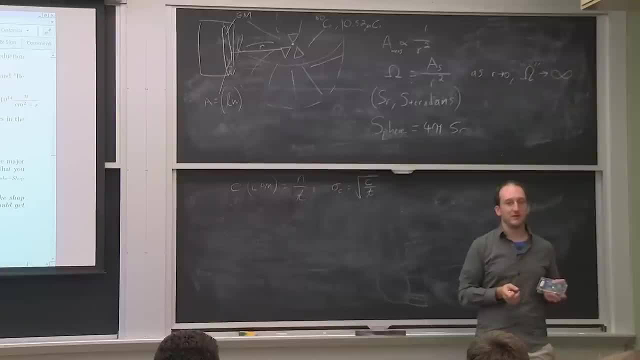 the less certain you can be that the number that you're measuring is actually accurate. So the idea here is that this standard deviation is a measure of confidence that your value is actually right. So the two things that you can do to decrease this standard deviation: you could increase your counting. 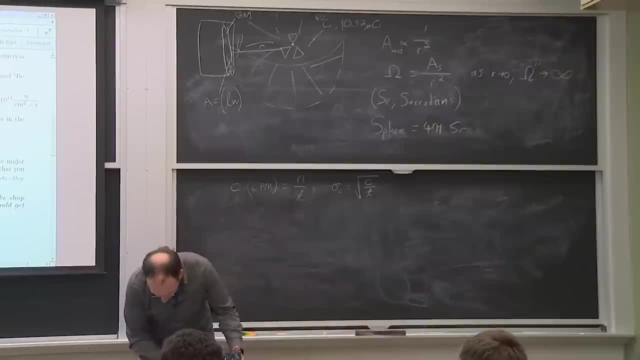 time right. Why is there a C on top? That didn't look right. It actually is OK. Yeah, Yeah, there we go. So by counting for longer you can decrease your standard deviation. This is going to take forever. 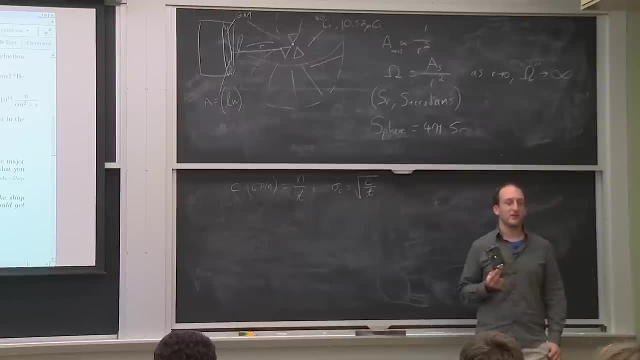 It actually takes about 67 minutes- because we've already done this calculation- to get a 95% confidence on 5% uncertainty for this sort of background count. I mean, how many counts have we had so far, like 12,, 14?? 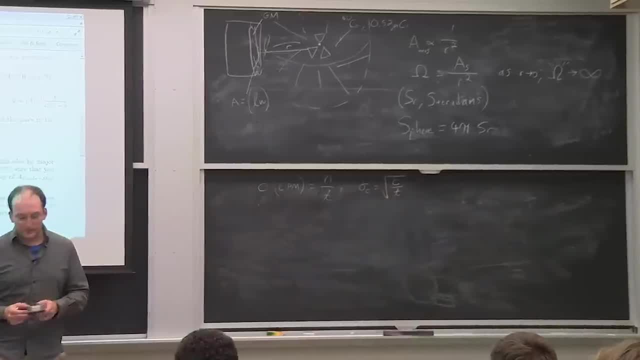 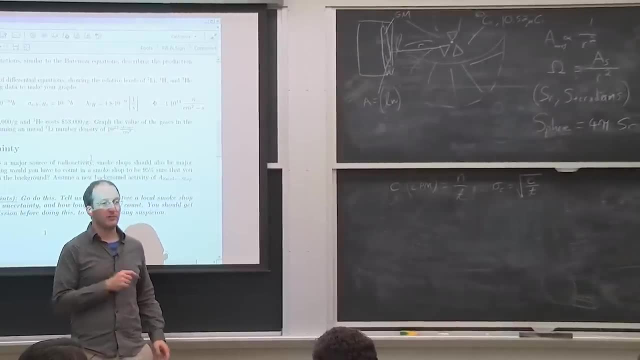 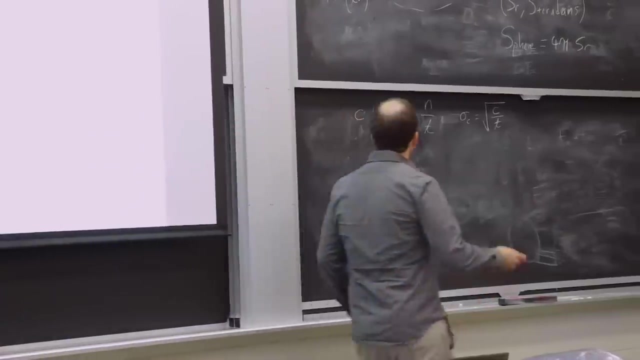 Yeah, not very many. Then you've got to be able to subtract that count rate from whatever your source actually is, And the way that you actually measure this is pretty straightforward. The way that you do error subtraction is not as straightforward. So let's say we're going to separate these two experiments. 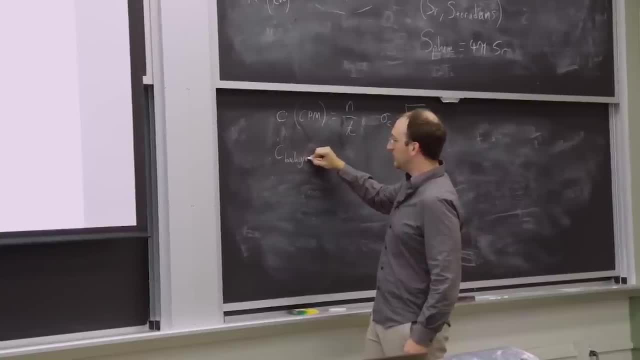 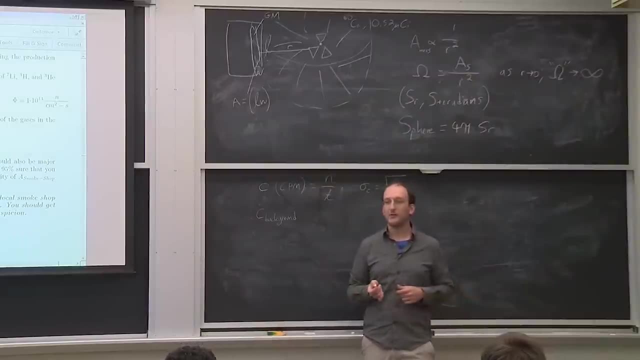 into a background. We're going to do a background experiment which we're actually going to do in an hour, When we want to count these banana ashes, we're going to have to count radiation coming from the detector itself, which will account for cosmic rays. 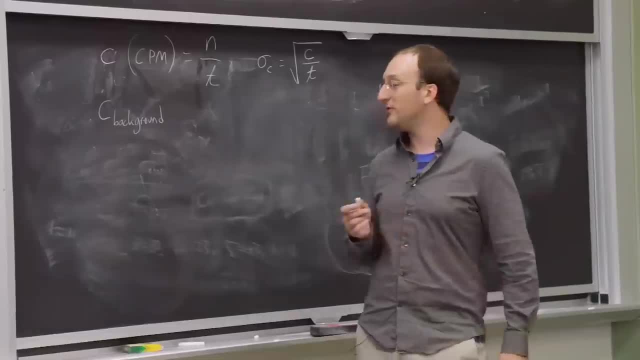 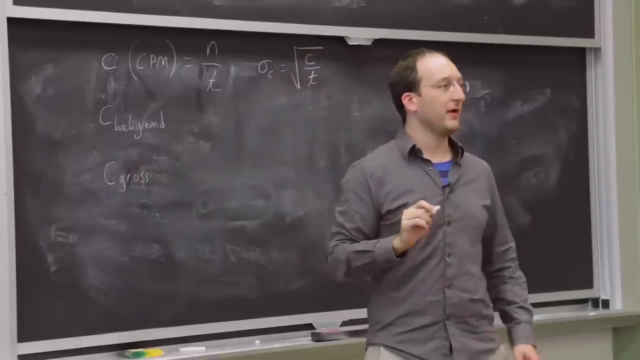 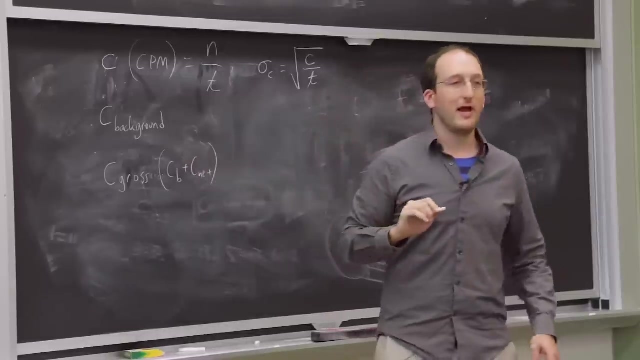 contamination in the detector, whatever else might have been spilled in there from previous samples, And we're also going to take some sort of gross count rate which will be our background, plus the net count rate of our actual source, And that's what we're going for. 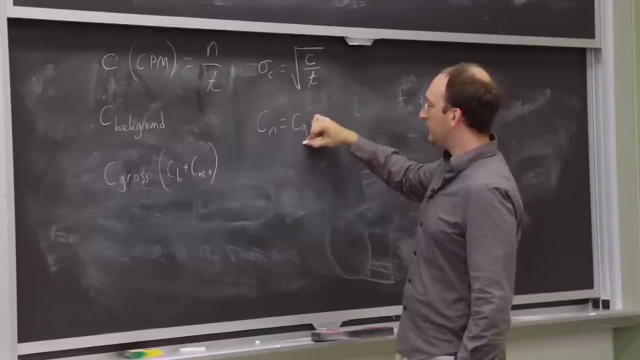 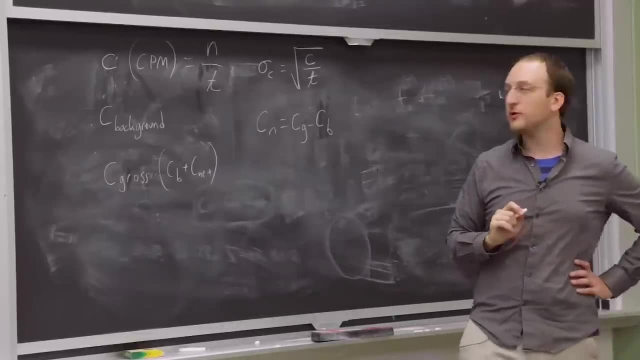 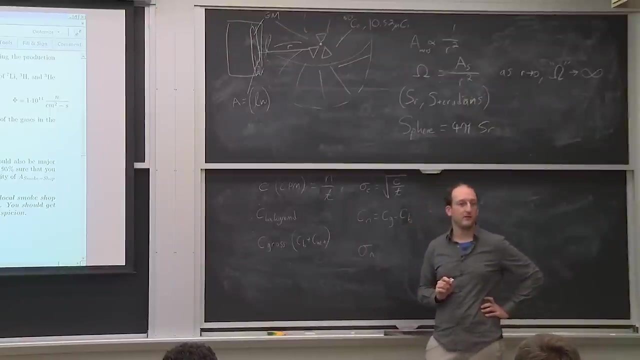 So the net count rate is pretty easy, just the gross count rate minus the background. Let's keep the symbols the same Minus the background count rate. Does anyone know how to quantify the uncertainty of this net count rate? You just add the two. 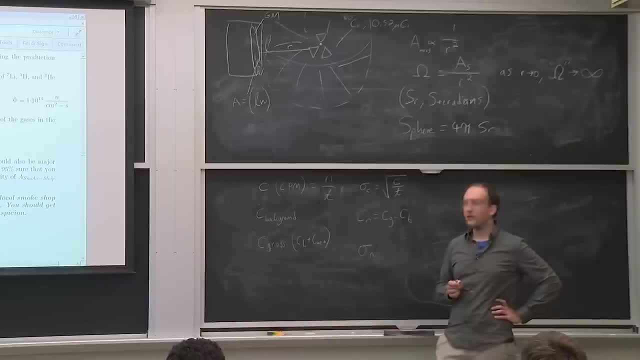 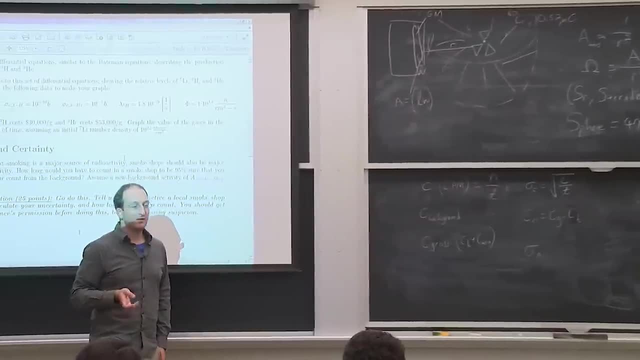 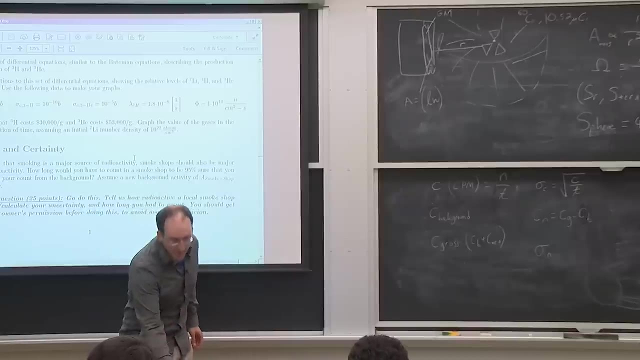 Anyone. Well, in this case, we have to account for the fact that radiation emission from anything is a truly random process, So it's actually random. There is no correlation between when one particle leaves and the next particle is going to leave. And because it's a truly random process, 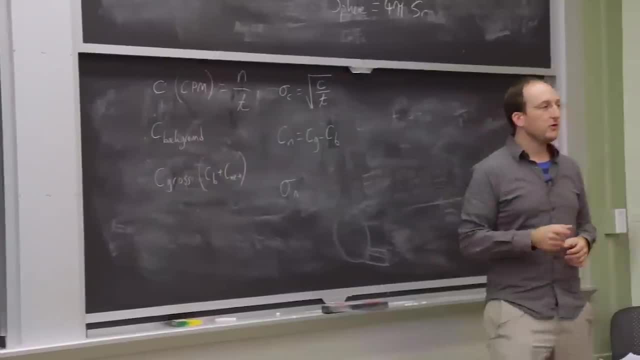 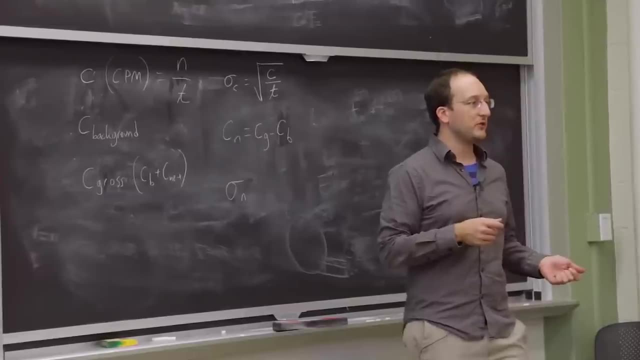 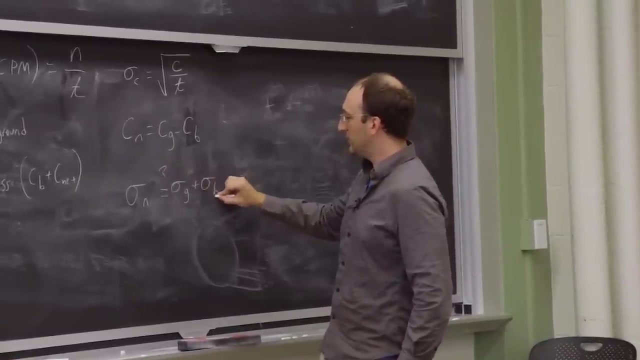 these errors in the background rate and the gross rate could add together or could subtract from each other. In other words, one might be a little higher than it should be, One might be a little lower. It's lower than it should be If you just add together the two standard deviations. 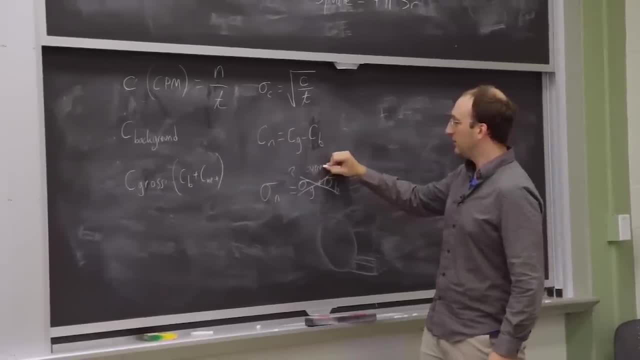 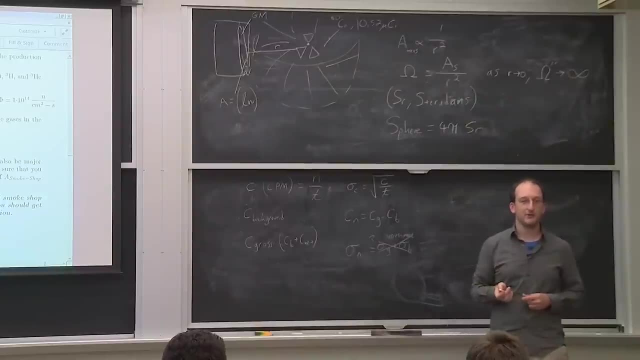 you actually always get an overestimate of the true error because you're not accounting for the fact that these two experiments may have partially canceling errors. So in this case that would be your worst case scenario, which is not your most likely scenario. 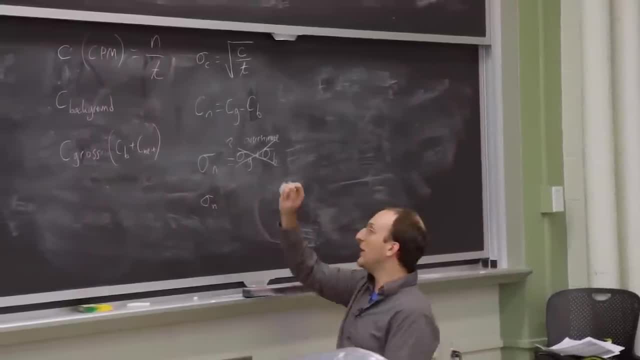 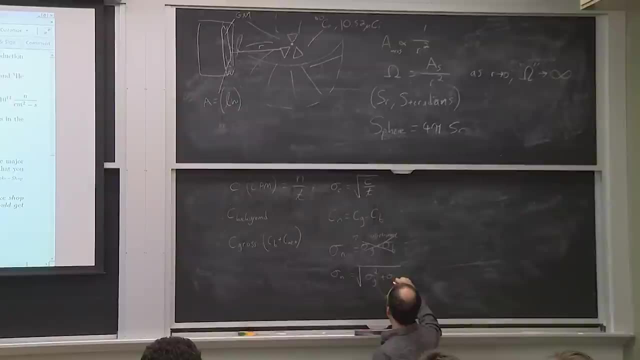 What you actually want is to do what's called uncertainty in quadrature, Where you actually add up the sum of the square roots of those errors Kind of looks like the magnitude of a vector, doesn't it? Kind of looks exactly like the magnitude of a vector. 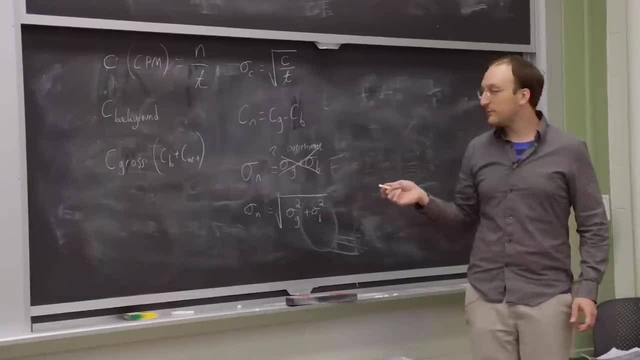 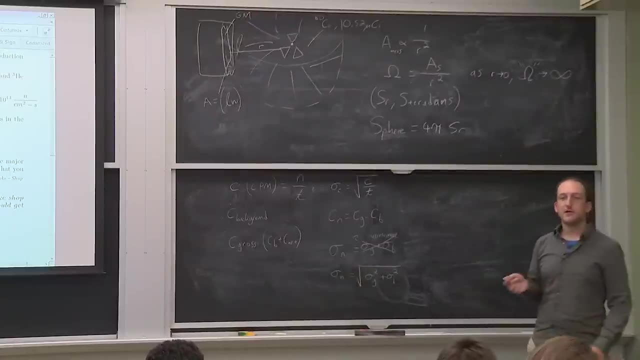 So in this way you're accounting for the fact that more error in each experiment does increase the error on whatever net experiment you're doing, but not linearly, Because sometimes you have partially canceling errors And with enough statistics if you count for long enough. 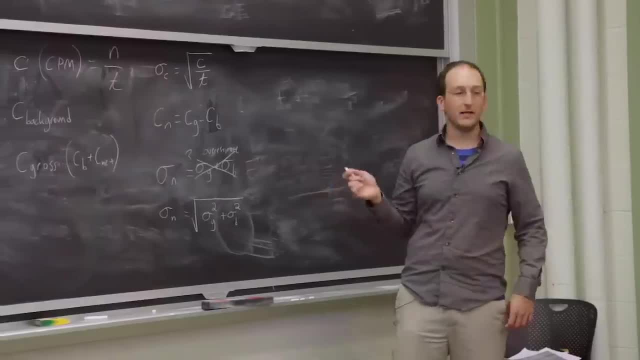 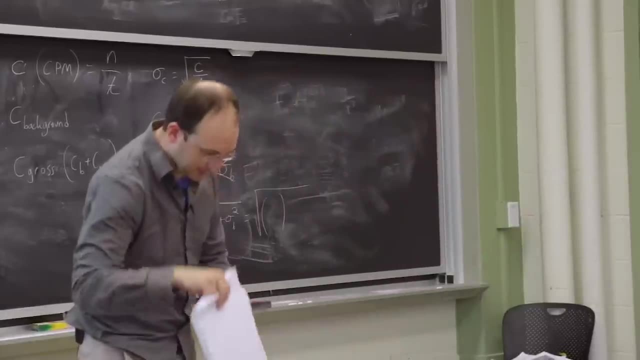 or you count, enough counts, then these things on average are going to add in quadrature, which we'll come out to, And I want to make sure I don't have any typos, So I'll just keep the notes with me. 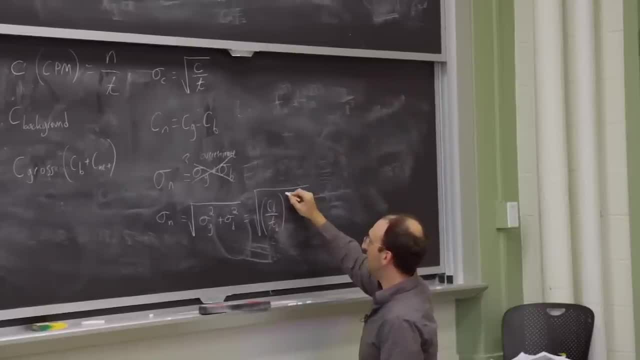 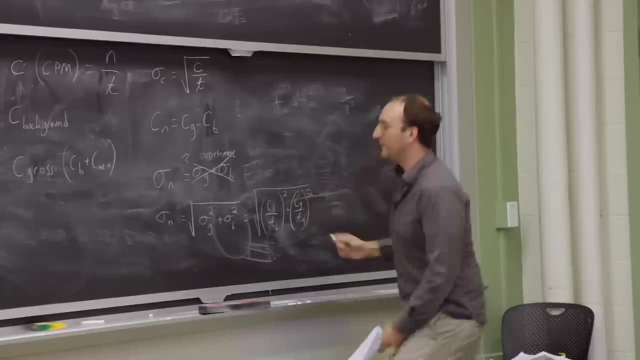 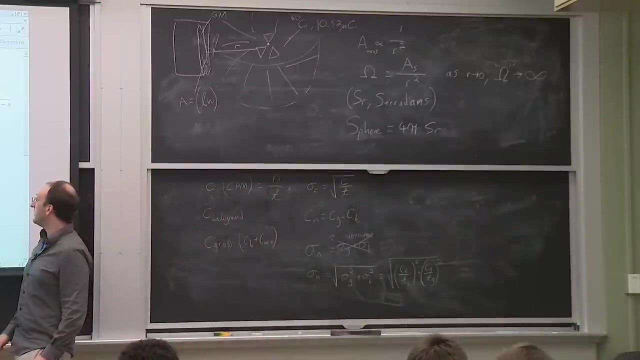 So you'd need the background count over the background time squared plus those. There we go, And so now I'd like to pose a question to you, The same one that's here in the problem set: How long do you have to count in the smoke shop? 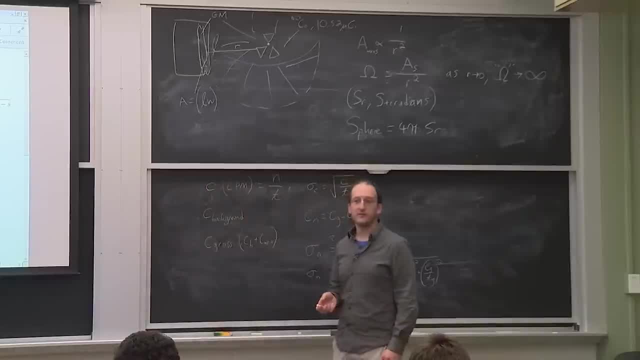 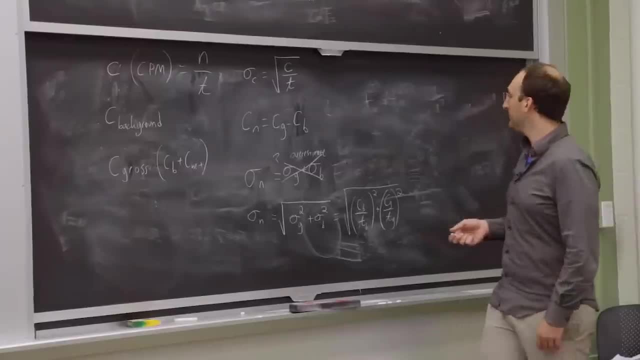 to be 95% sure that, let's say, your count rate's 5% uncertain, And we're going to spend the rest of today's class taking apart that statement and getting at what it should be. So, again, what we want to say is: 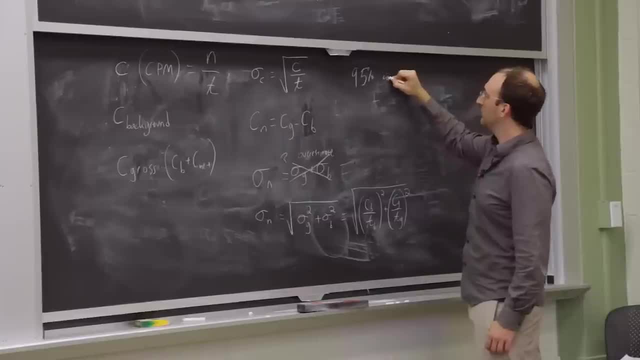 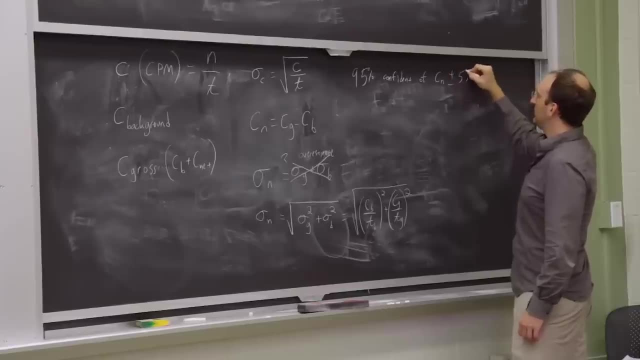 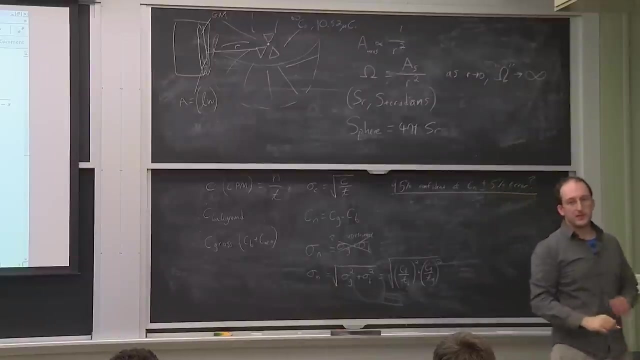 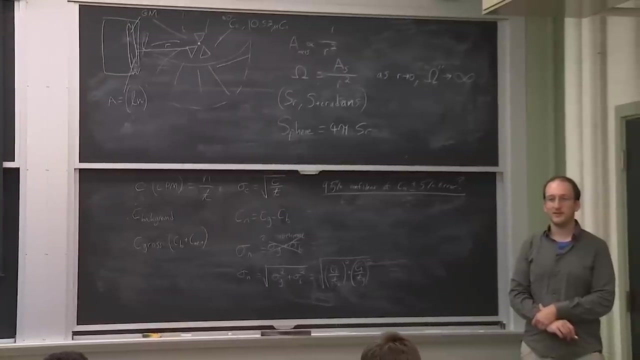 how do you know that we're 95% confident of our count rate plus or minus 5% error? That's the main question for today. Does anyone know how we'd start Anyone get to the reading today? I see some smiles. 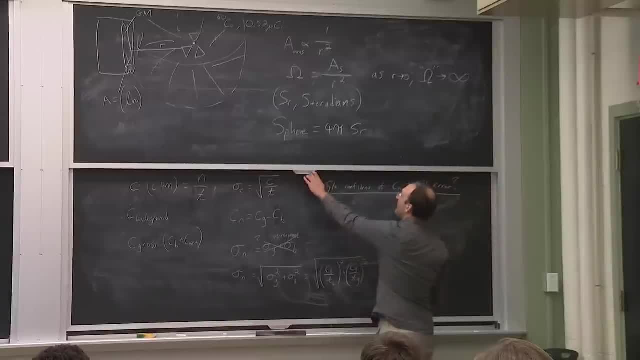 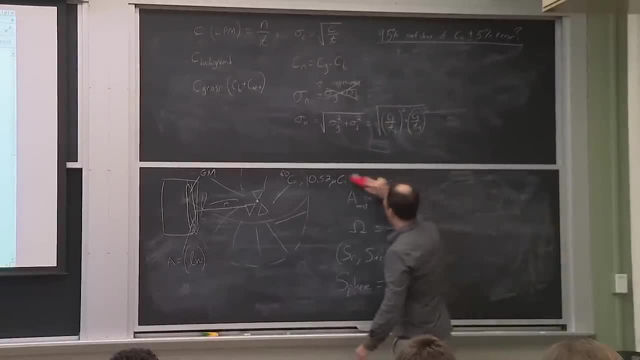 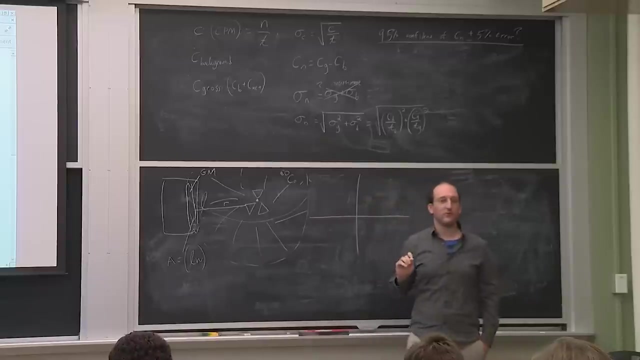 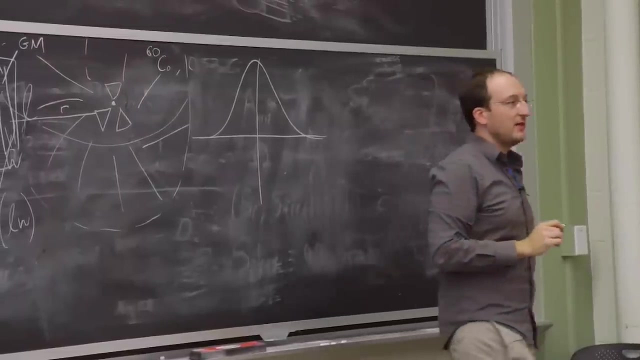 OK, We'll start from scratch then, All right. So who's here Is her. I've heard of a normal distribution before. A lot of you guys, great. The idea here is that, with enough counting statistics, this very rare event: binomial distribution. 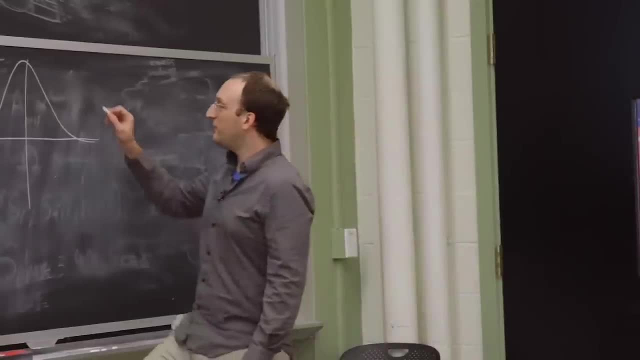 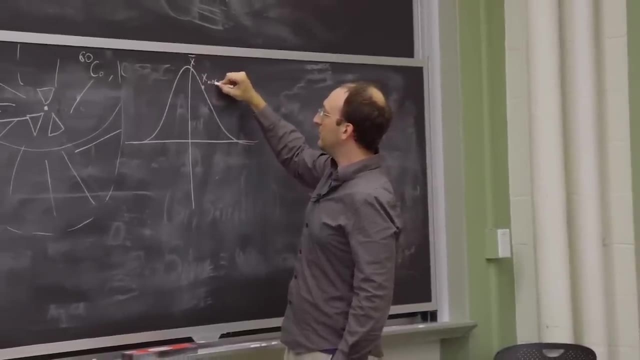 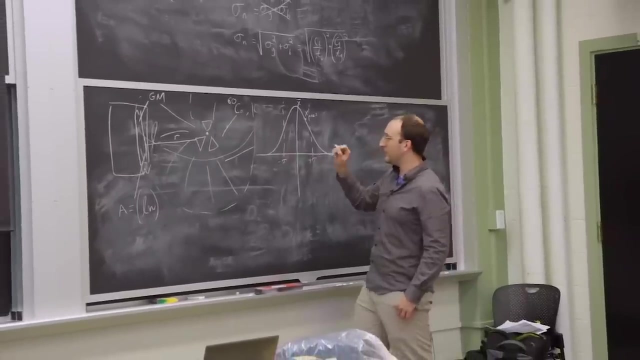 approaches a normal distribution where you can say: if you measure a certain count rate, let's say this would be your mean count rate, and if you measure some other count rate to limits of plus or minus 1 sigma or 1 sigma, And if you can characterize this. 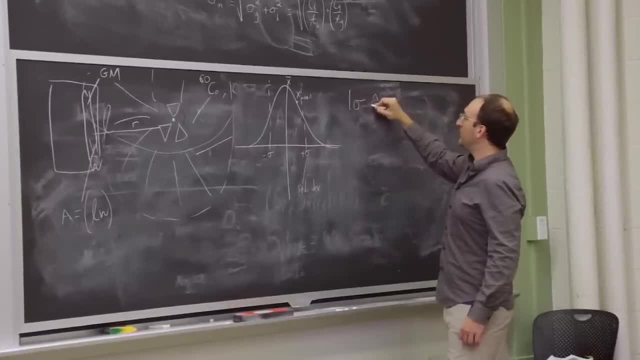 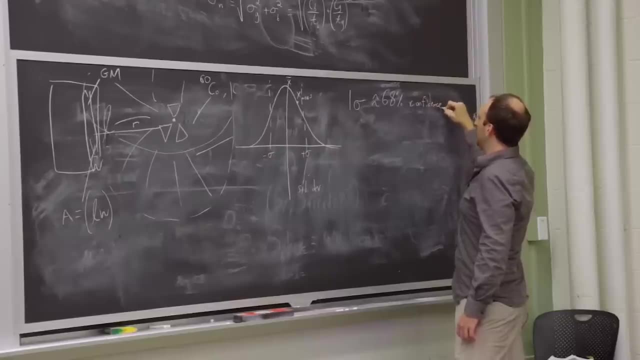 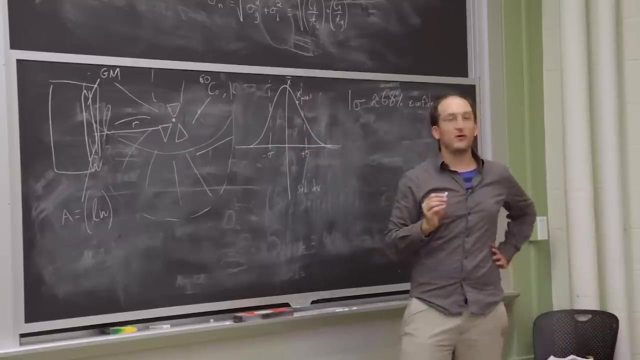 and the result is that it's a standard deviation. then, with this standard deviation, 1 sigma gives you about 68% confidence in your result. Confident- yeah, Spelled it right. The reason for that is that if you go plus or minus 1 sigma, 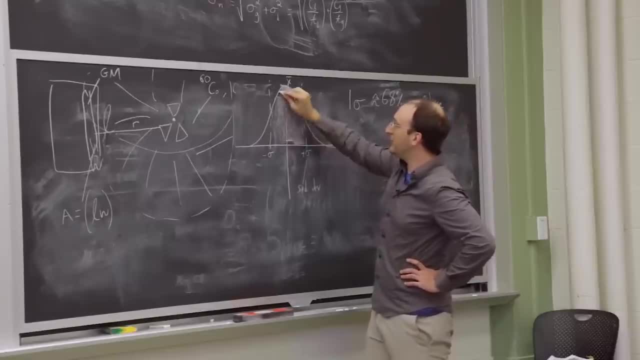 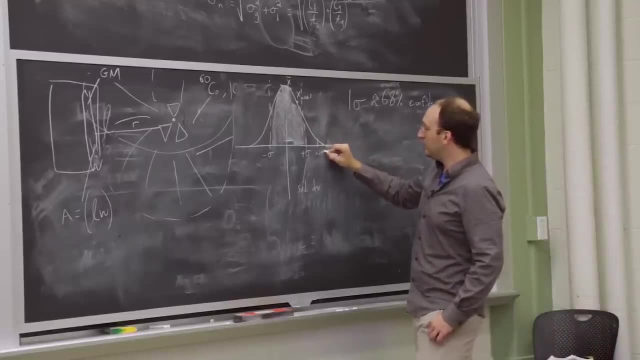 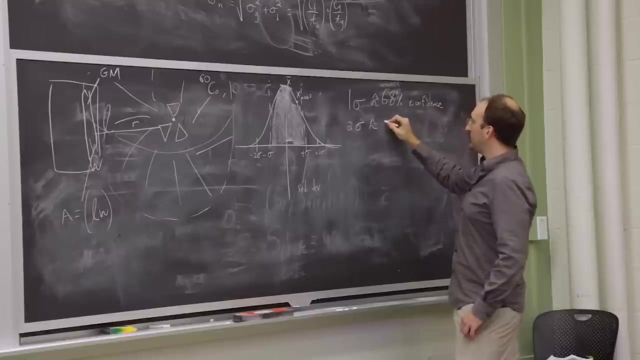 away from your true average. right here you filled in 68% of the area under this normal distribution. go plus 2 sigma or minus 2 sigma, it's around 95%. confident 3 sigma is getting towards 99 point. what was the number? 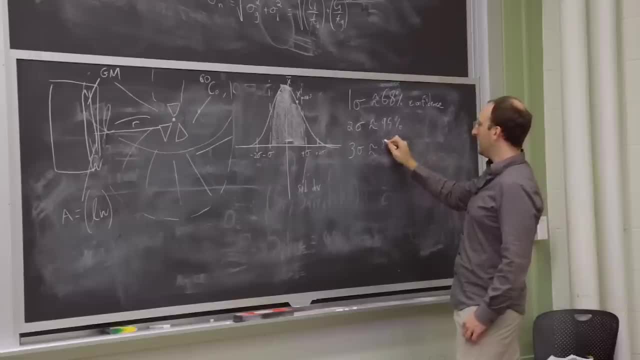 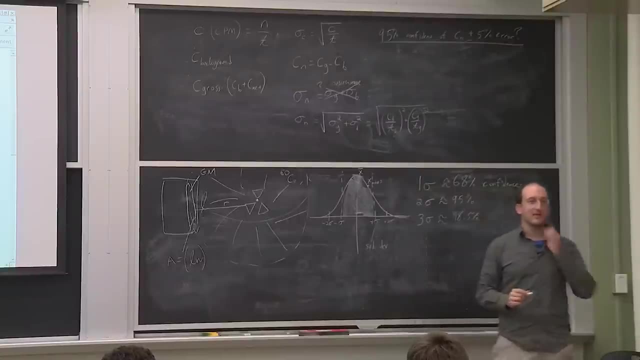 again, I think it's 6.. Maybe it's more like 98.5%, And then so on, and so on, and so on. There's actually societies called 6 sigma societies, And the way that they get their name is: we're so confident of things, we can predict them to 6 sigma. 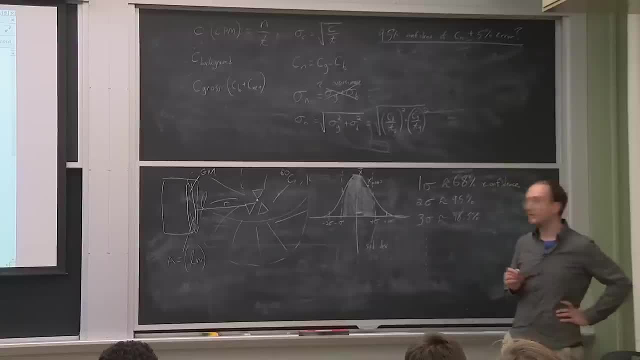 which is some 99 point, a large number of nines percentage of the area under a normal distribution. So if I ask you how long do you have to count to be 95% confident in your result? you have to give an answer that will relate two times. 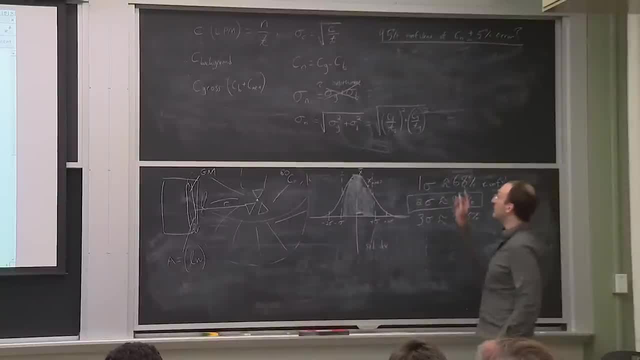 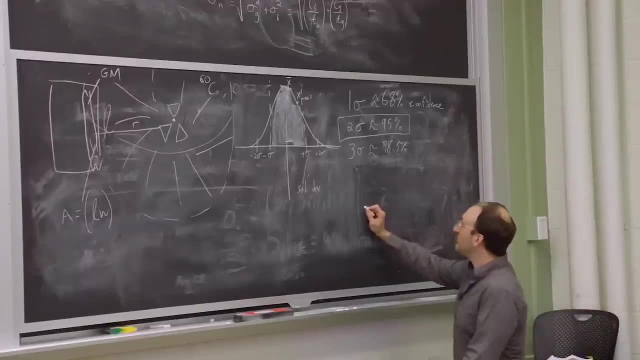 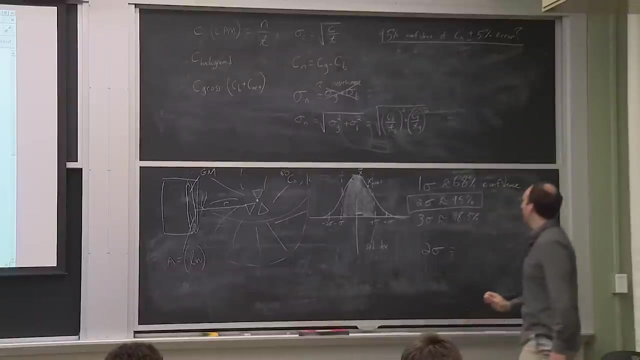 this standard deviation. And now we know the formula for standard deviation of this net counting experiment. So we can formulate our equation Thusly: let's say, in order to be 95% confident- in other words, 2 sigma- that our counting rate is within 5%. 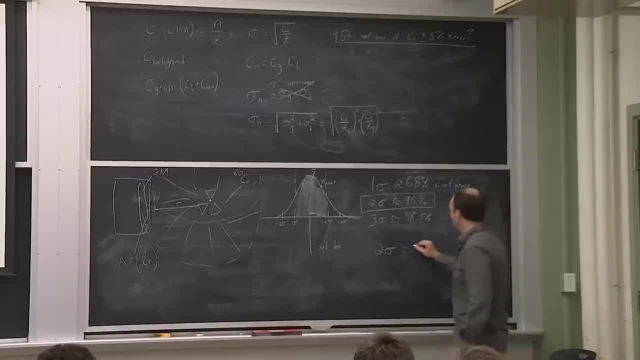 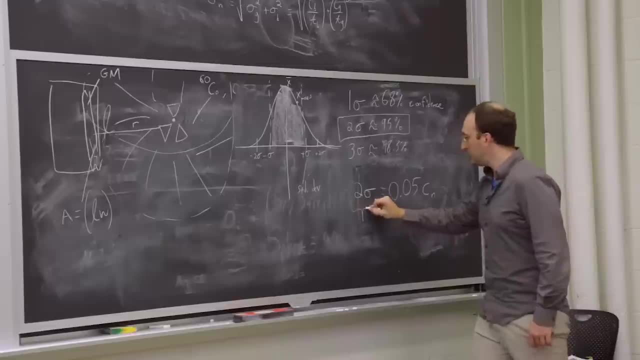 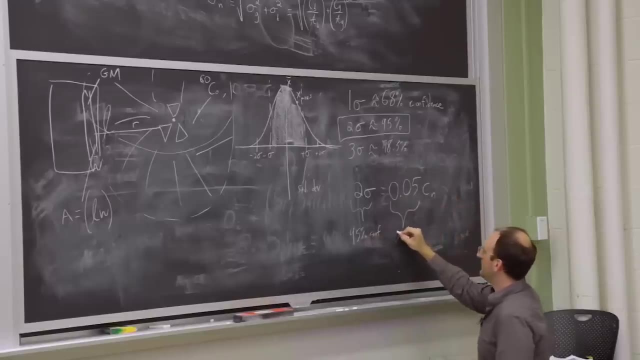 of the actual value, in other words plus or minus 5% error. We put our error percentage here and our true net count rate there. So this part right here tells us the 95% confidence. This part right here is our 5%. 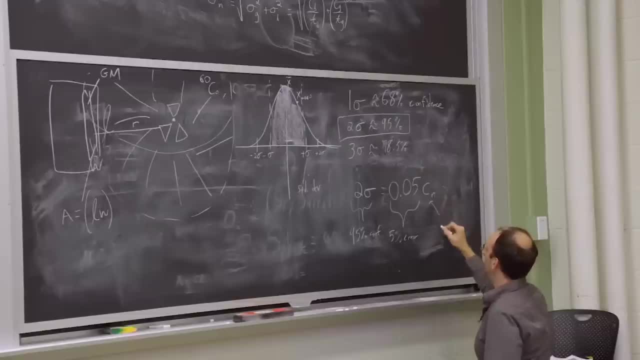 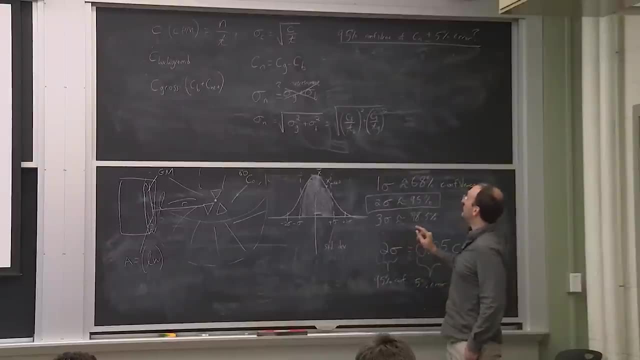 And this part right here is our 5% error, And that part right there is our count rate. So then we can substitute in our expression for sigma. our uncertainty in quadrature and find out things like well depends on what the information we're given is. 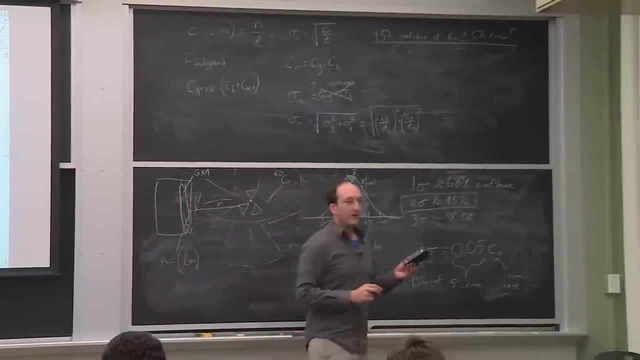 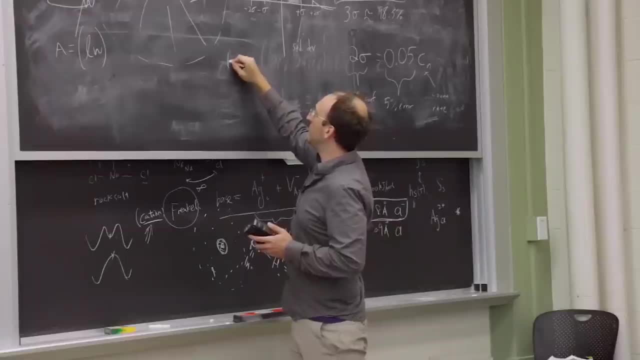 Let's say, before you go to the smoke shop you take your Geiger counter and for an extremely long time you count the background counts somewhere. So let's say, in this problem, the known quantities, we know, our background count rate. 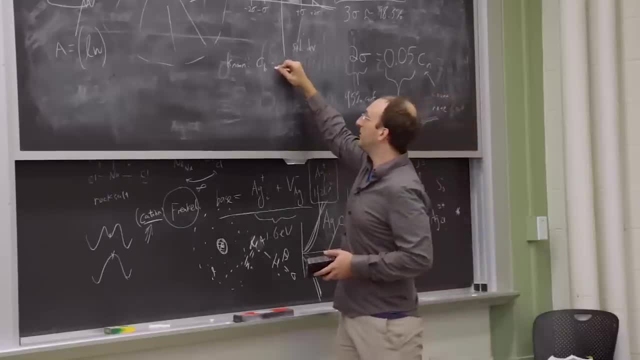 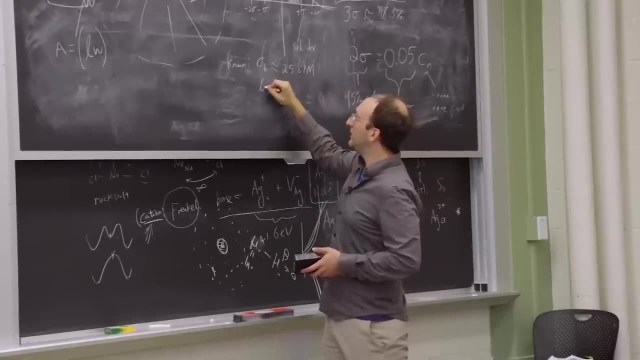 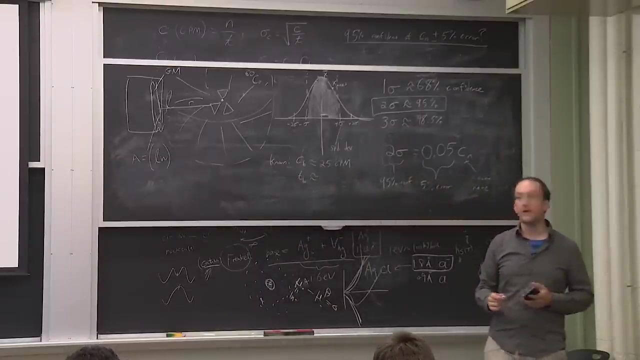 because you can do that at your leisure at home. And when I did this it came out to about 25 counts per minute And known is the background counting time. And when I did this to get within 95% confidence of 5%. 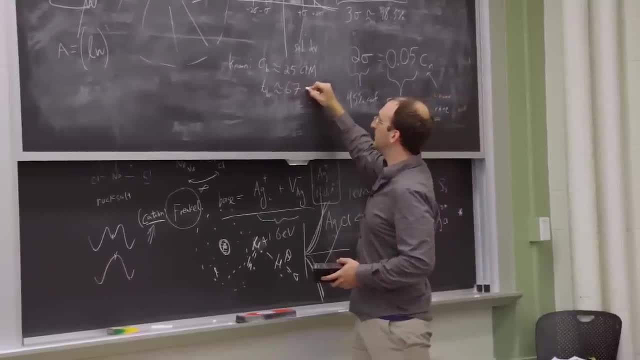 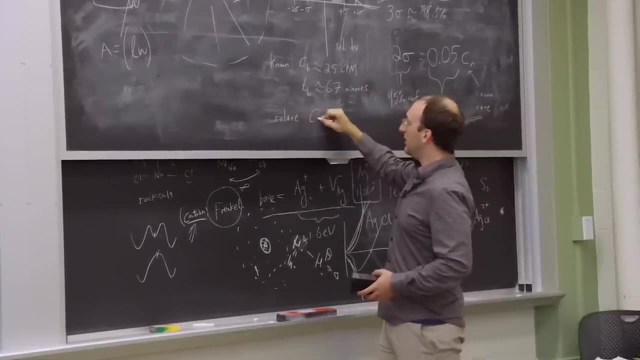 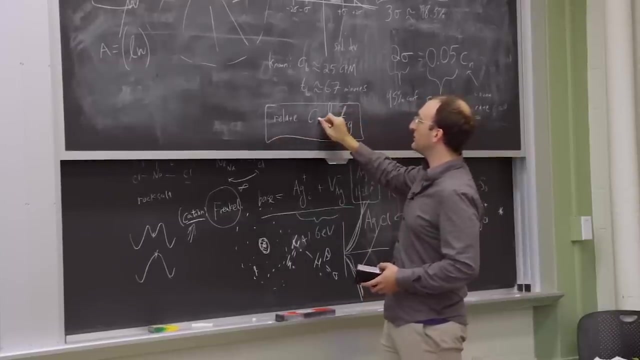 error. I had to do this for 67 minutes, And now all that's left is: we want to relate our net count rate and our gross counting time, or our gross count rate and our gross counting time, because it's like the same thing. 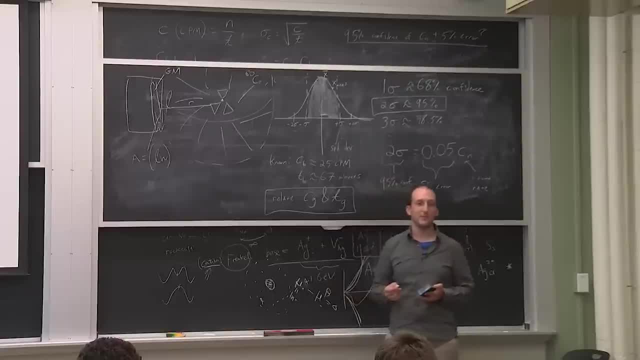 So this is actually how you decide how long you have to sit in the smoke shop to count in order to satisfy what we asked for: 95% confidence that your count rate is 5% error. So let's start substituting this out. 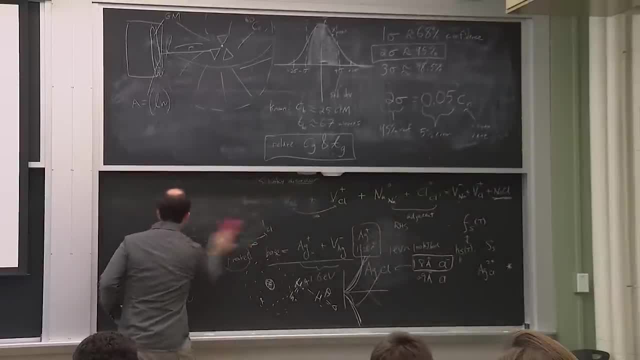 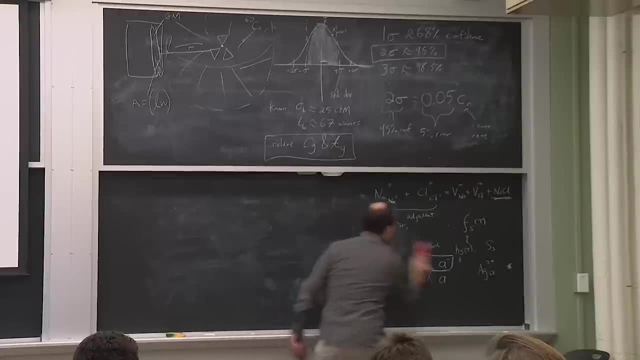 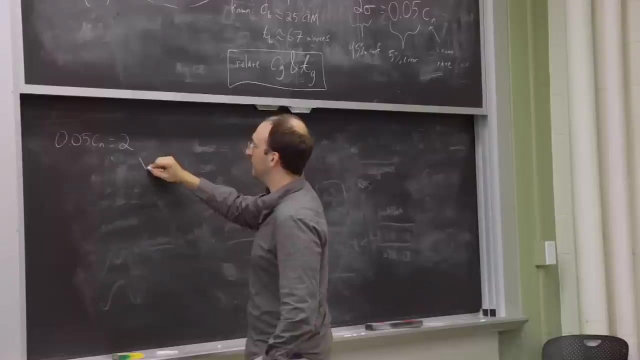 That's not mine, so we can get rid of that. So we'll take that expression and substitute in everything we can. So 0.05CN. 0.05CN equals 2 sigma, And there's our sigma expression, which I'll rewrite right here. 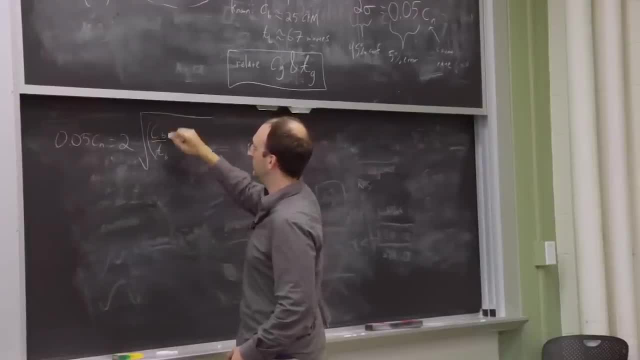 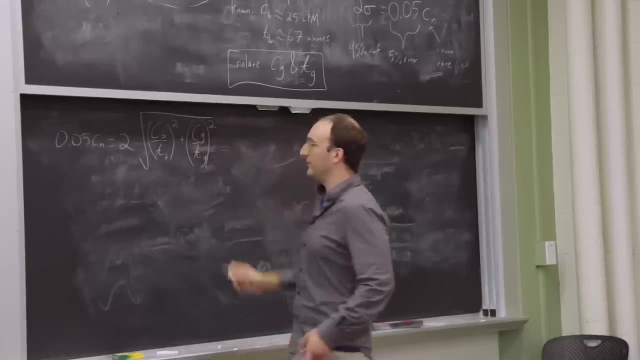 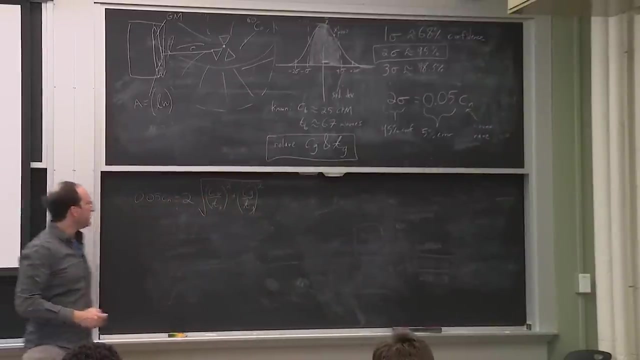 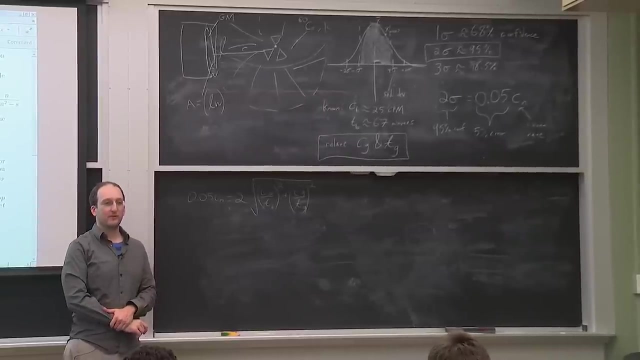 So we have CB over TB squared, plus CG over TG squared. OK, What's next? How do we relate TG and CG? Well, let's start with the easy stuff, right? What can we cancel or square or whatever? Just somebody yell it out. 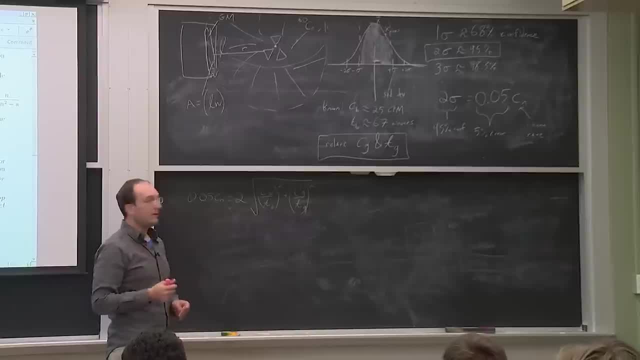 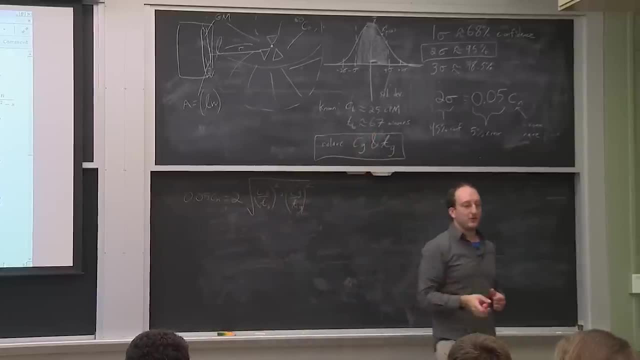 Do we have numbers for these counts? Yep, so we have numbers for CB and TB, but not CG and TG. We have not yet answered the question. when you go into the smoke shop and talk to the owner and he says fine. 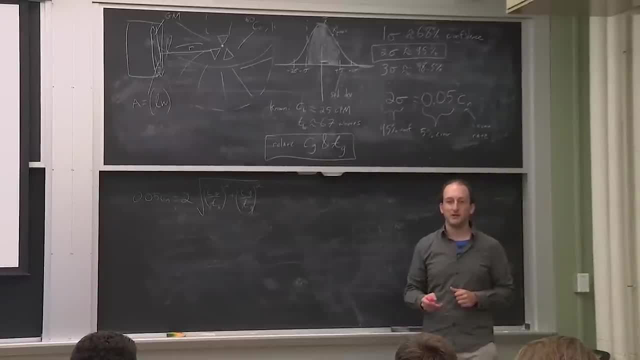 You're going to sit here with a radiation detector. How long do you have to be here looking all weird? You want to have an answer, And so if you get some initial estimate of CG, you can tell him. this is my approximate TG. at which point? 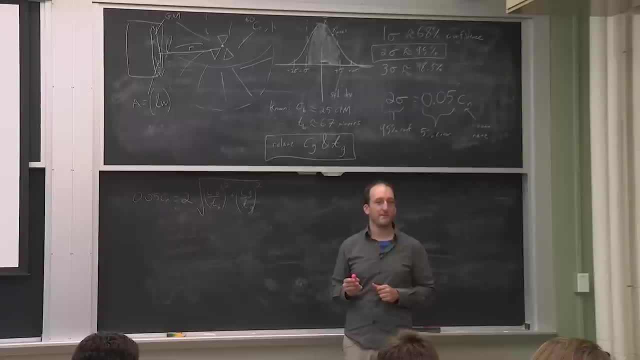 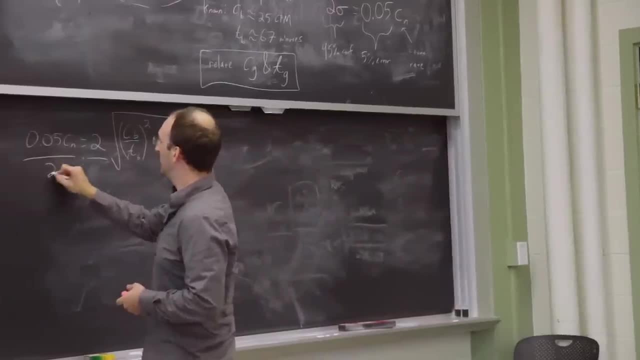 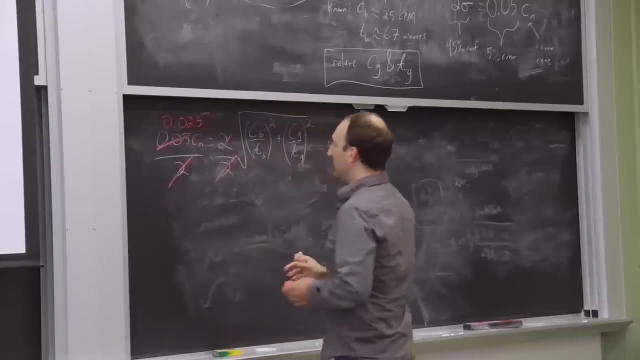 he or she will say yes or no, depending on how they're feeling. So why don't we just start? Divide by 2, right Divide by 2.. 0.02CN- 0.025.. We can square both sides. 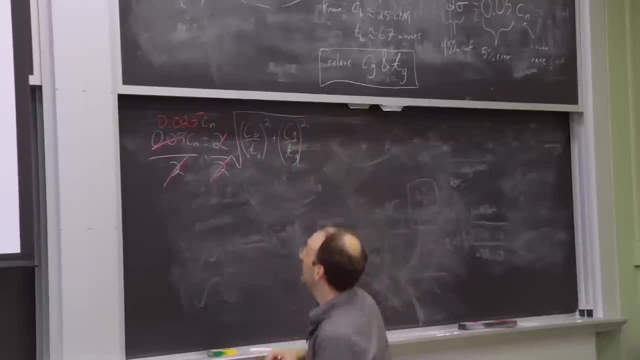 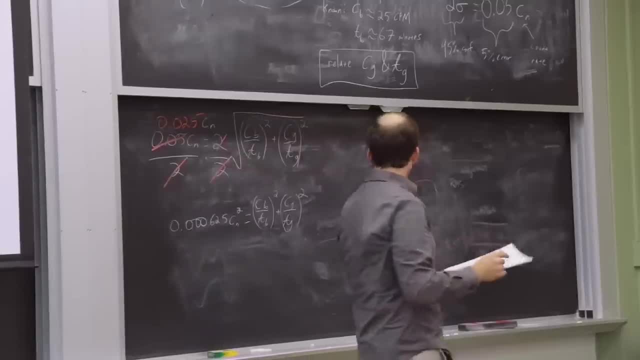 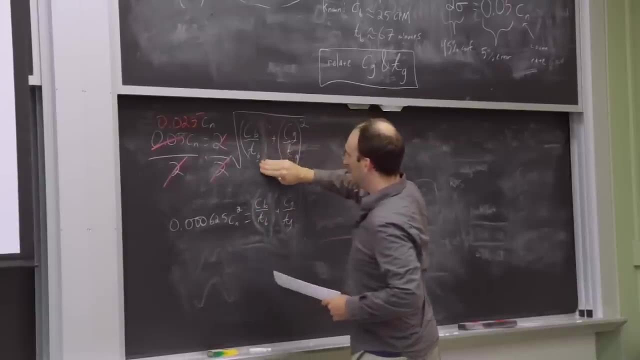 Squared. What's the way to go about it? I want to make sure I do the efficient one. Oh, I'm sorry Those aren't squared, Because those are already our standard deviations had the square root in them. There we go. 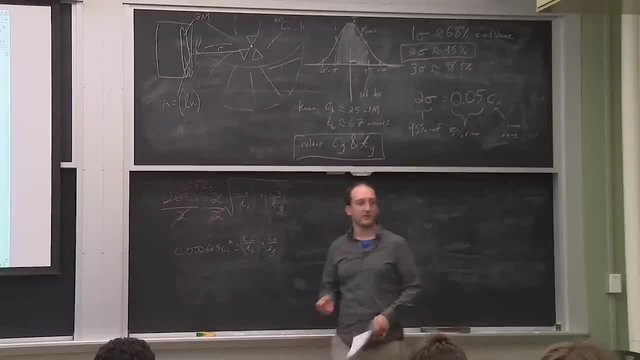 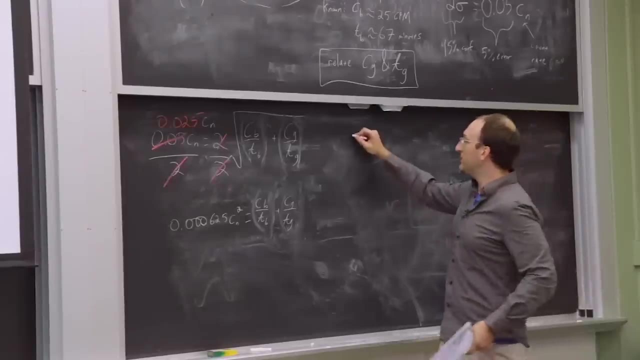 That's more like it. OK, what's next? We got too many variables, Yeah, Isn't there still a square value formulation? Is there still a what See right? The value's still under the Because, in this case, the standard deviation. 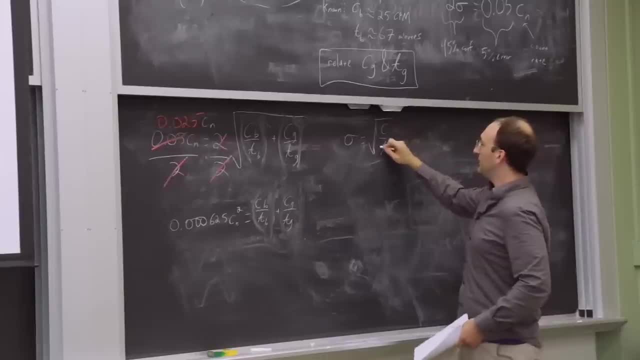 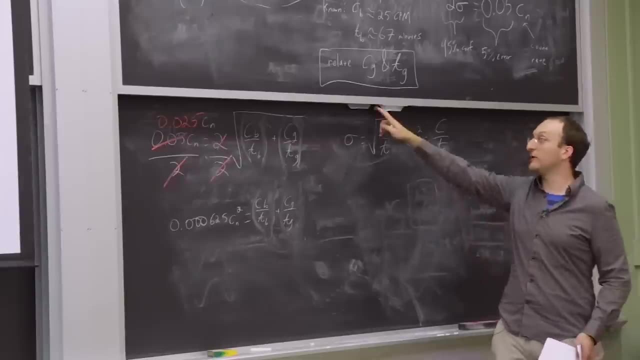 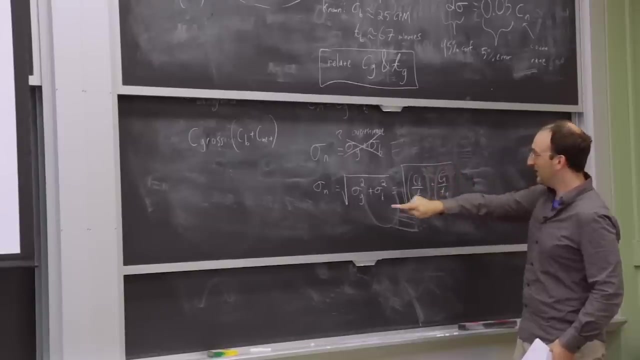 is the square root of the count rate over the time. So the standard deviation squared is just count rate over time. Was there an earlier expression we have to correct? Yup, That's where it came from, That's right. That's not because. 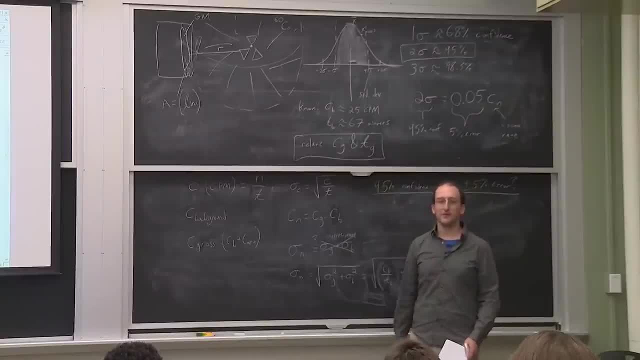 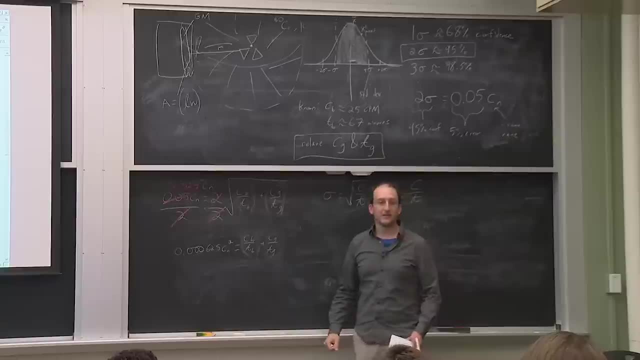 That's right, There we go. Good tracing out that. OK, now that everything is corrected here, what's next? We've got too many variables. yeah, So the standard deviation you have units of MICHAEL SHORTLANDER- Not quite. 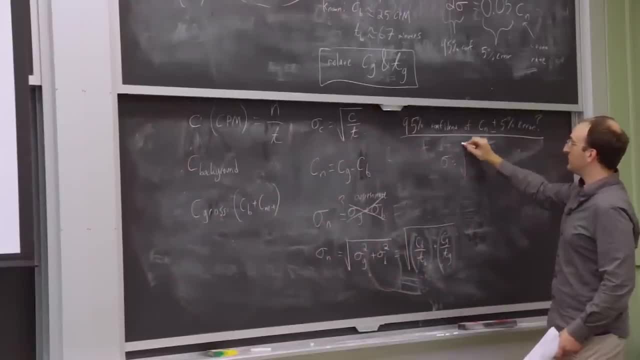 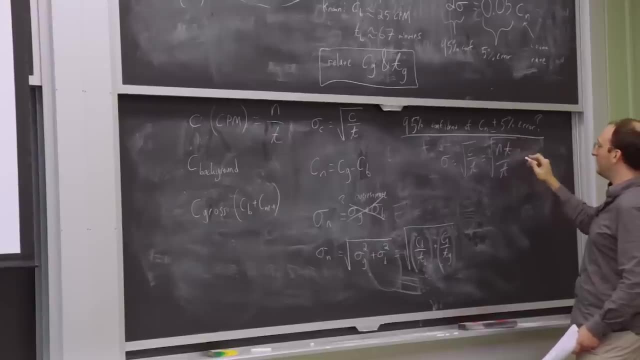 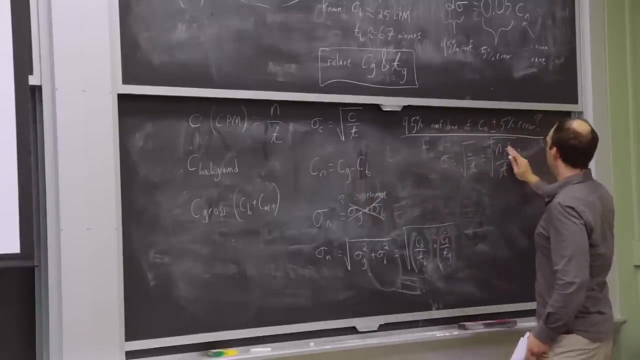 Because there's a count rate in here, So the units of standard deviation. if this is square root of count rate over time, which is the same as number of counts times times time over time, right Yeah, Because again a count rate is a number over time squared. 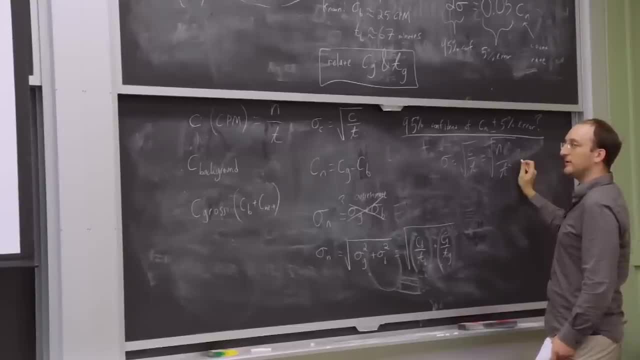 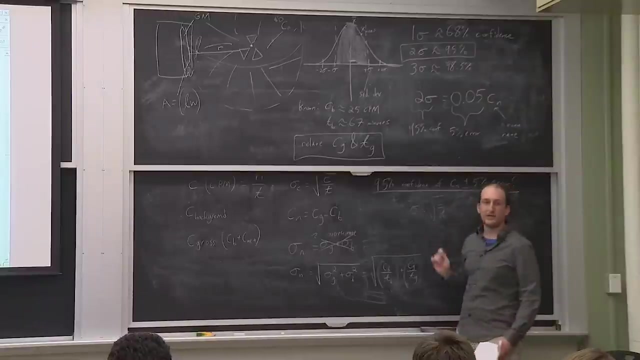 That doesn't sound right, though, Let's see- Hold on a sec, MICHAEL SHORTLANDER- Although the standard deviation's got to have the same units as the count rate itself, because they're additive right, Because you usually express some count rate plus or minus. 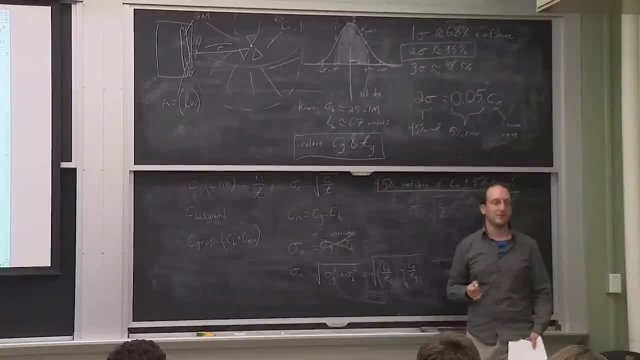 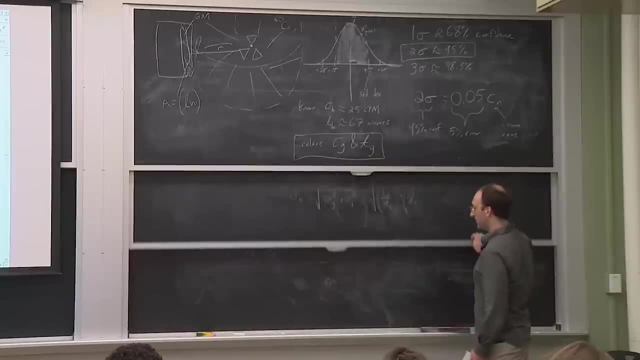 either sigma or 2 sigma, so they've got to have the same count rate. So standard deviations are expressed in counts per minute. if your counts are expressed in counts per minute, OK cool. So we've got too many variables, but it's. 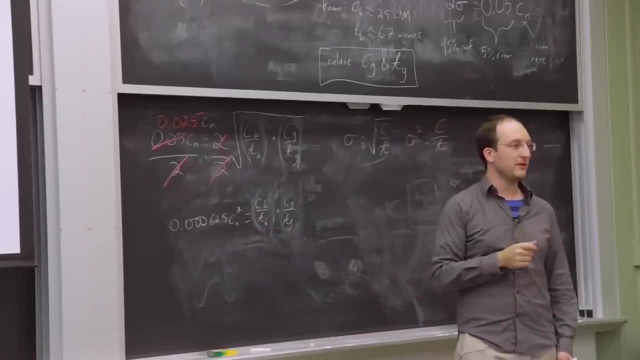 easy to get rid of one of them: either Cn or Cg. Do you have a question? No, I'm just going to say this in a position. MICHAEL SHORTLANDER, Great, OK, so you're going to say the same thing that I was saying. 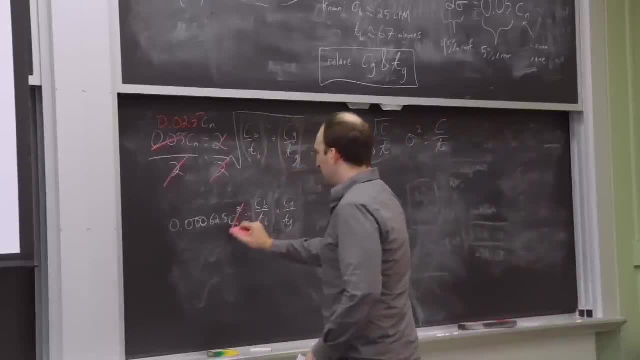 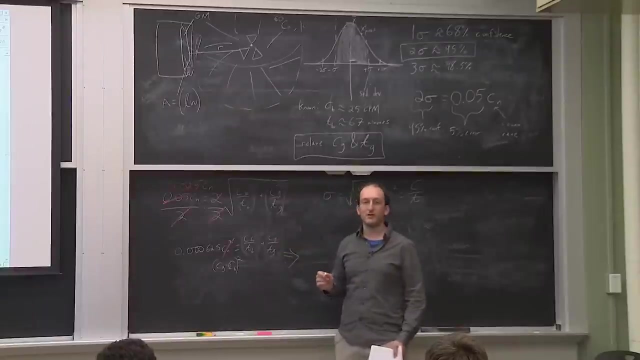 Yeah, sorry, MICHAEL SHORTLANDER, I was going to do Cool. So we'll take out our Cn and we'll stick in a Cg minus Cb, And we're trying to isolate Tg as a function of Cg. 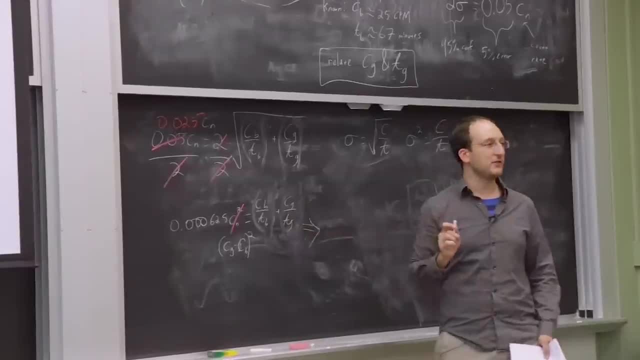 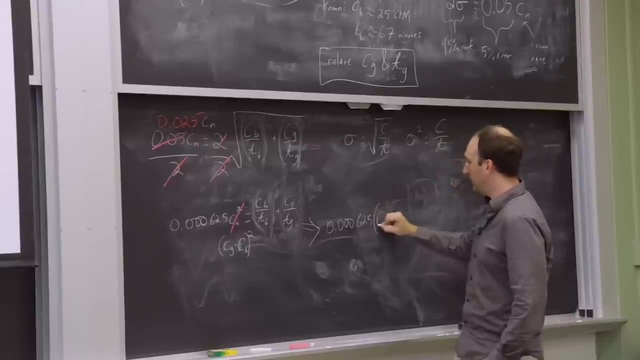 or vice versa. There's a lot of Cgs and not a lot of Tgs, so let's just keep the Tg on its own. So we'll have 0.000625 Cg minus Cb, So we'll have 0.000625 Cb squared. 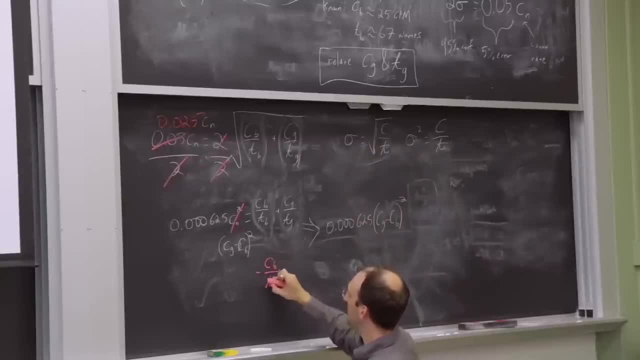 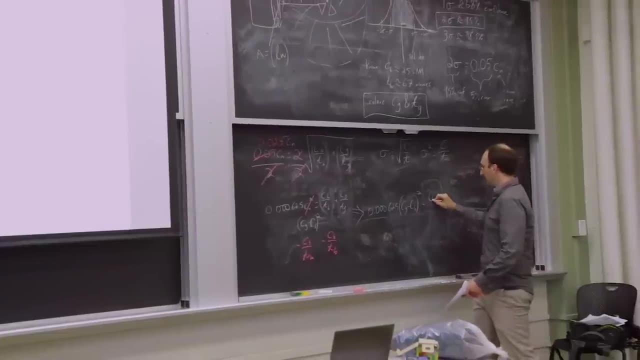 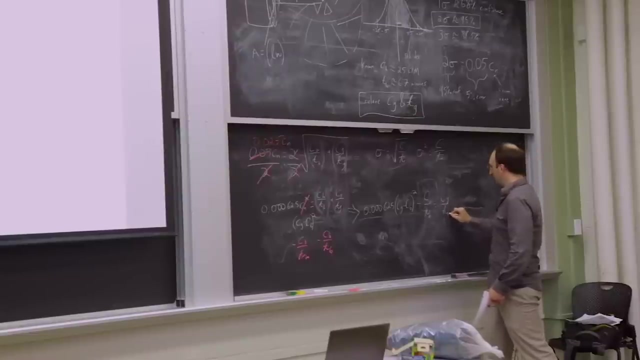 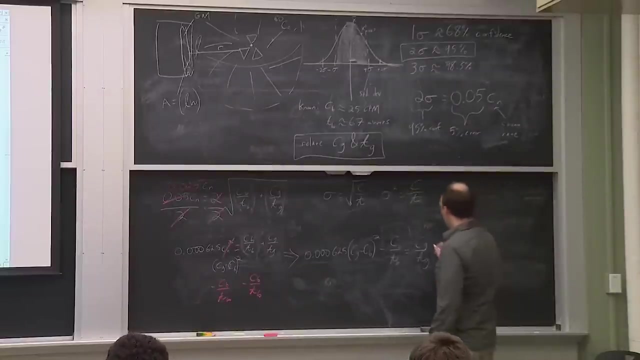 And I'm going to subtract Cb over Tb from both sides minus Cb over Tb equals Cg over Tg. And do I have to go through the rest of the math with you guys? I think at this point we've got it pretty much solved. 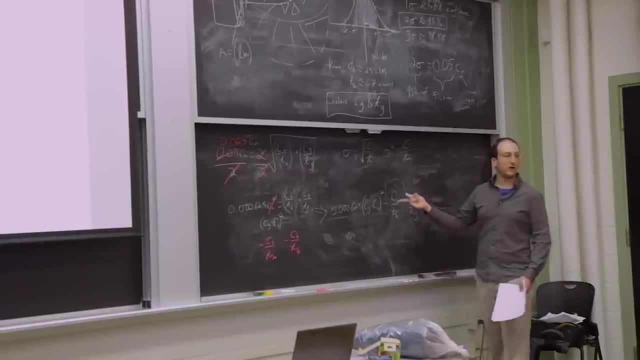 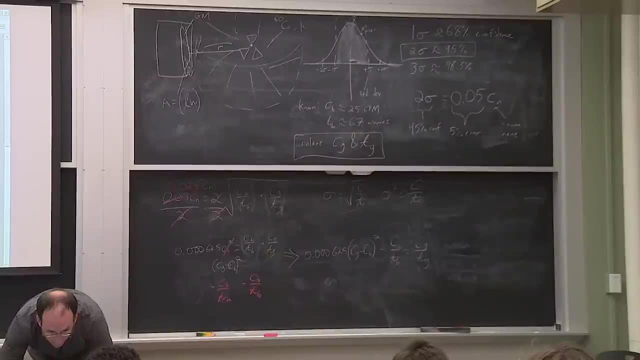 We divide everything by Cg. OK, OK, Flip it over and you end up with- actually I've already written out the expression which I want to show you guys here- Back to smoke shop counting time. So I want to show you some of the implications. 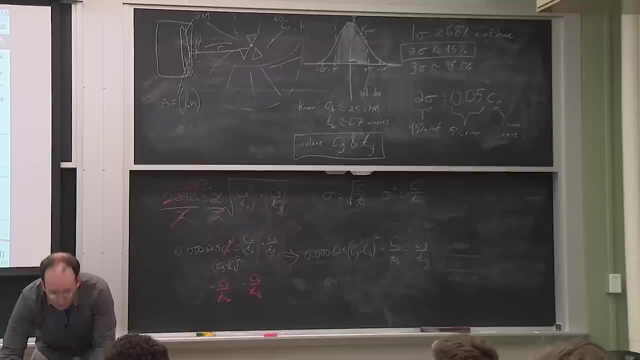 of this expression, That number right. there is just a more exact part, a bit of 2 sigma Instead of 0.05,. let's see, Yeah, instead of 0.05, we had something much, much closer So. 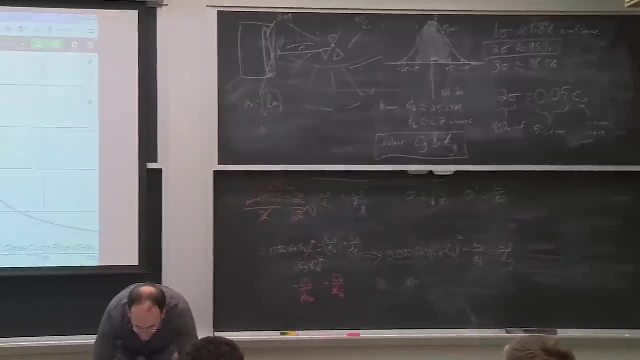 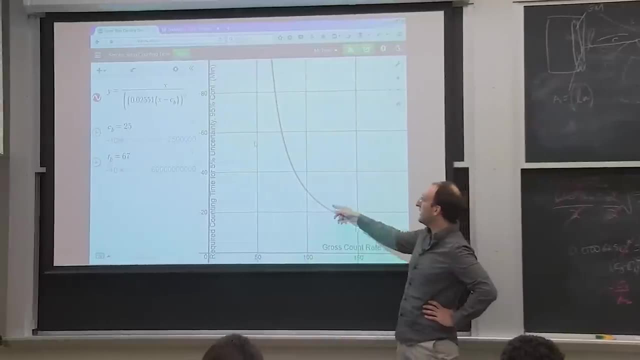 So what I want us to look at is this graph: right here We've got a nice relation now between the count rate and counts per minute and the gross count rate and the required counting time to get to that 5% uncertainty. Well, there's a couple of interesting bits. 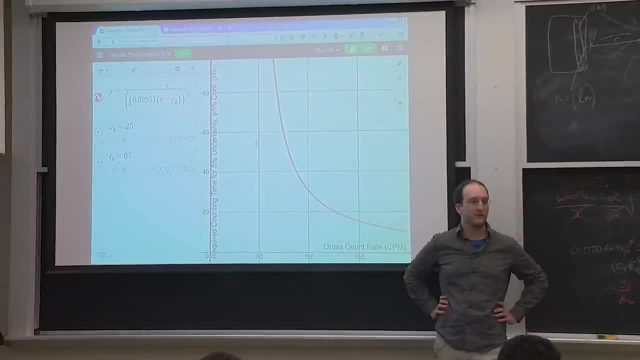 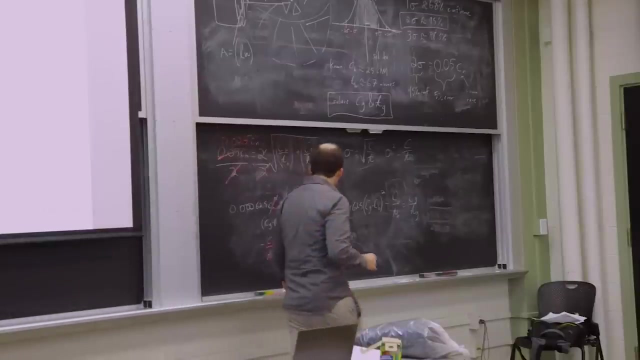 about this equation? What are some of the features you notice? Yeah, The count rate is extremely low, so it's going to take a little more time. Yes, Yes, The count rate is extremely low. It's going to take an infinite amount of time. 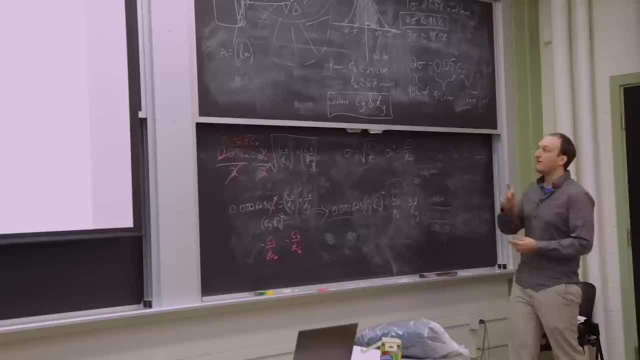 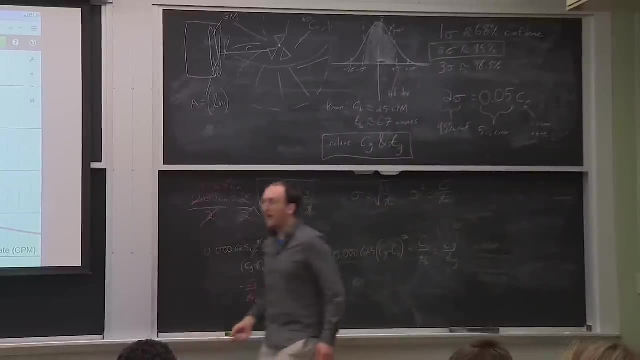 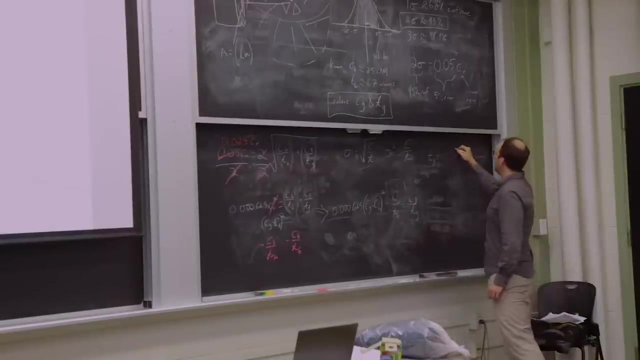 You're actually right on some levels. So if we have that expression right there, so let me just actually get it all the way out so we can see, because I want to show you some of the math-related implications for this. So if we had our counting time is what do we have? 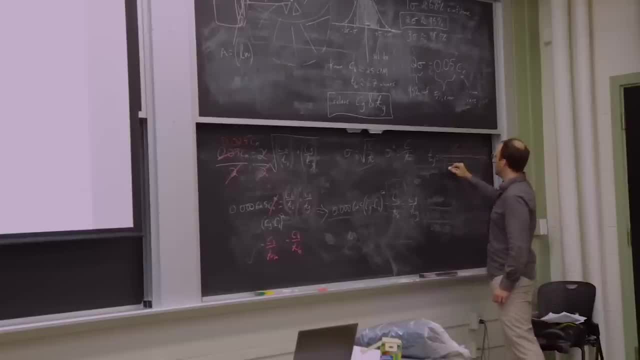 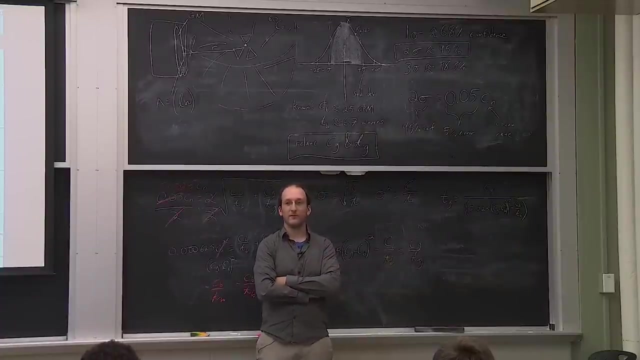 CG over 0.0, let's say 2.5.. CG, CG minus CB, squared minus CB over TB. At what point is this equation undefined? Yes, the second one, That's right For the condition. so, like Sean said, for the condition where 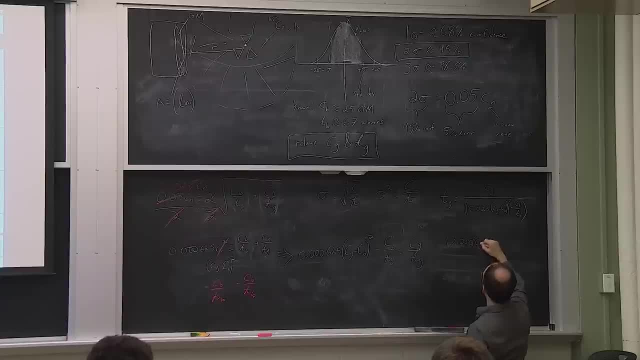 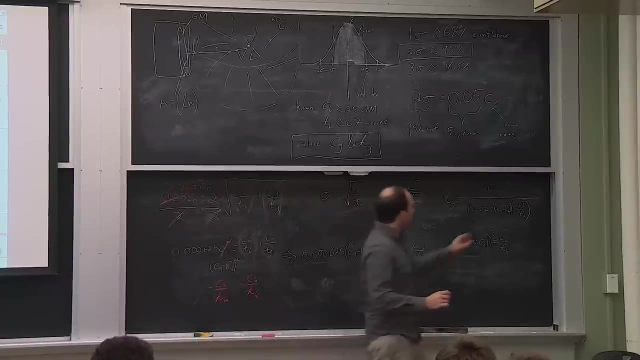 0.025 CG minus CB, let's just call it CNET: squared minus equals CB over TB. this equation is actually undefined, which means that if your CB and TB, let's say if the uncertainty whoops stepped on the cord, 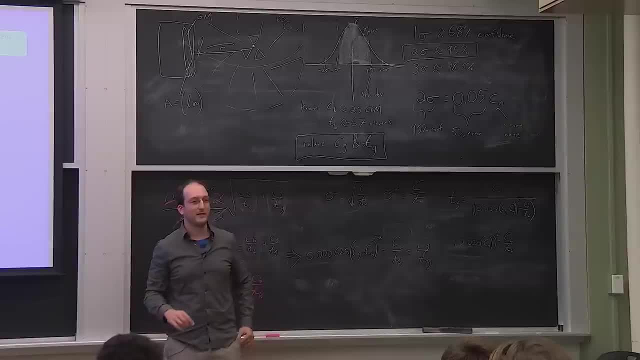 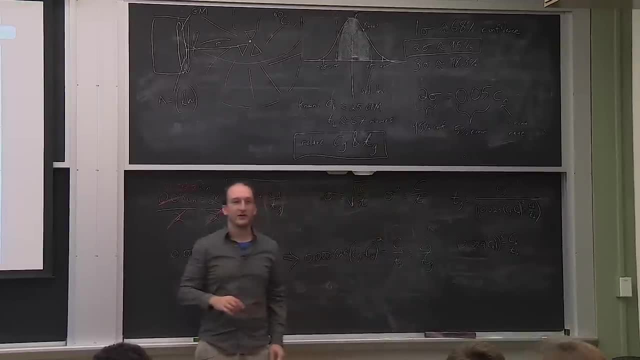 if your uncertainty from your background counting rate experiment is such that you can never get the total uncertainty down to, let's say, 0.025.. Yes, to, let's say, 5% error. with 95% confidence you can't actually run that experiment. 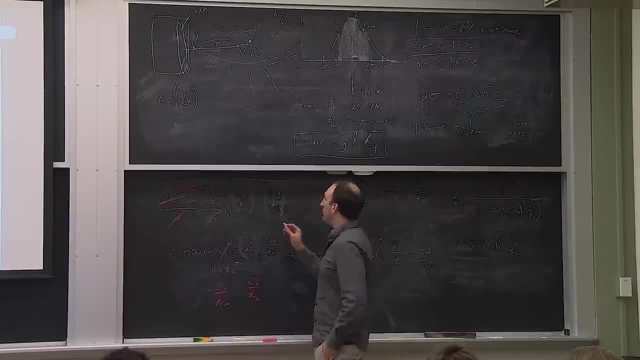 Because these uncertainties are added in quadrature. if you're trying to reduce sigma down to a value below that already, how can you do that? You can't have a negative standard deviation, right? So what this actually means is that when you're designing this experiment, 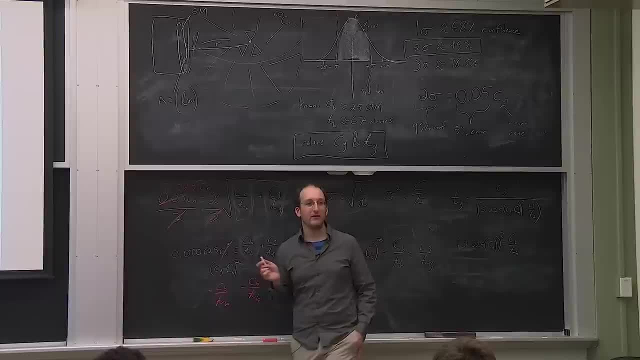 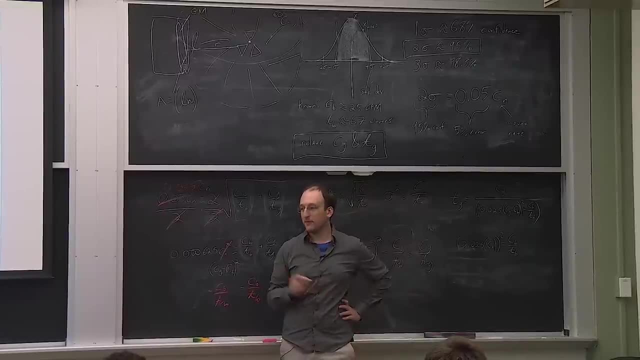 even if you count for 67 minutes at 25 counts per minute, like we can now- And you can do that in the air- That might not be enough to discern the activity of the smoke shop or the source or whatever you happen to be looking at. 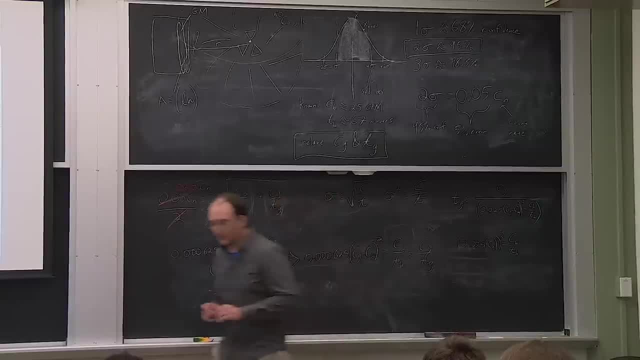 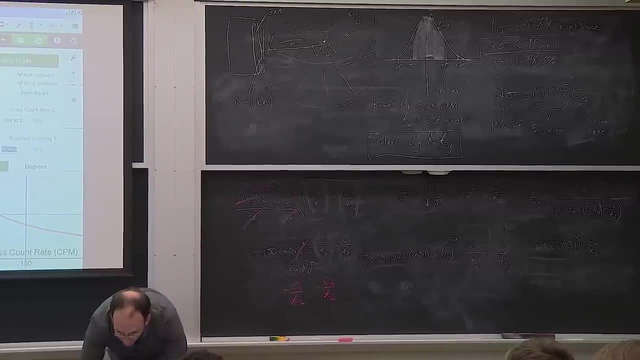 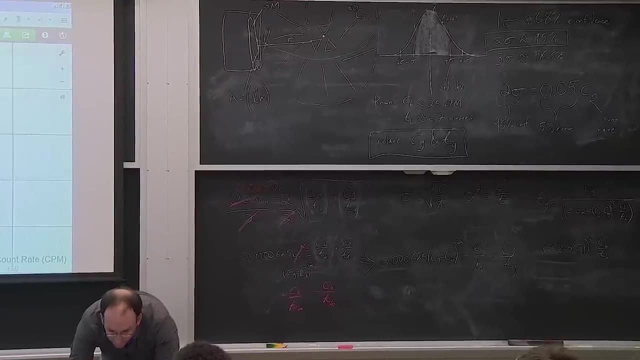 to 95% confidence within 5% error, And so let's actually look at that on the graph. If we keep on scrolling up, just by adding stuff to the y-axis, eventually we see that it gets all straight And right here at about 49 counts a minute, suspiciously close to the bottom. 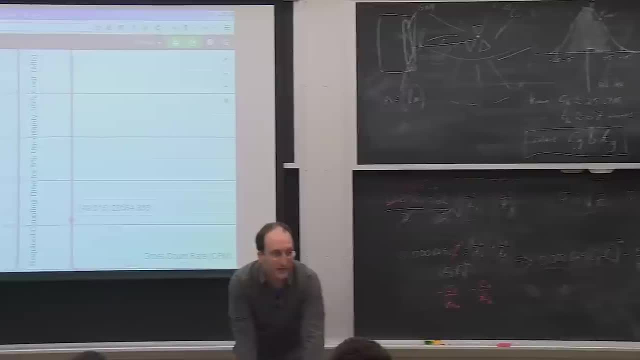 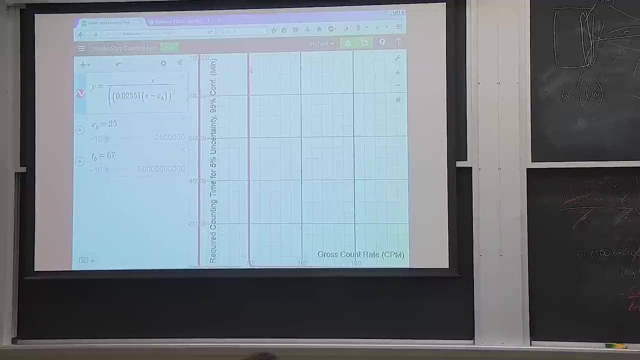 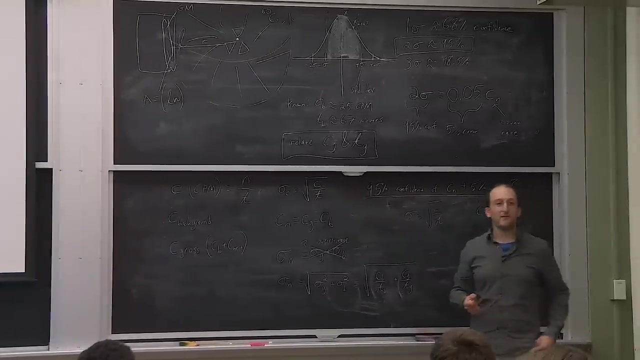 you'll never actually be able to get within this confidence and error interval. So there's always some trade-offs you can make in your experiment. Let's see, There it is. So sometimes do you necessarily have to be 95% confident of your results? 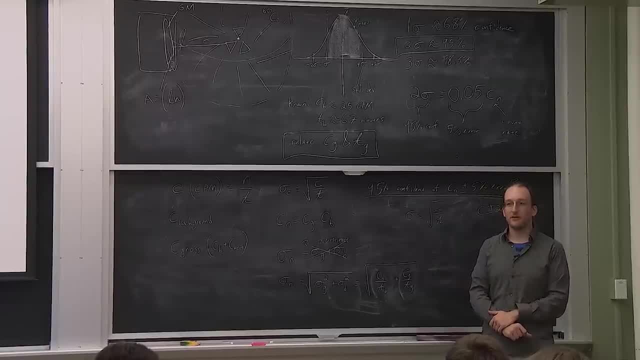 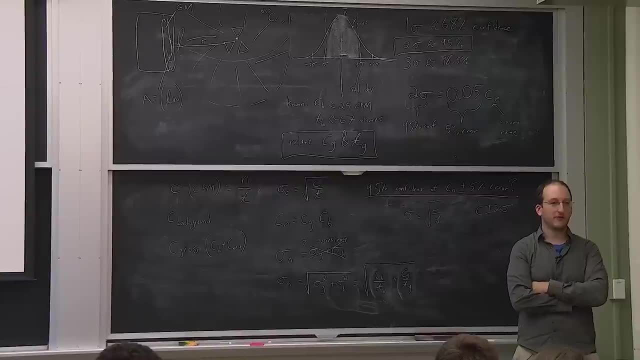 Depends on what you're doing, Or do you necessarily have to get within 5% error? That's probably the one you can start to sacrifice. But it's not. You can start to sacrifice first. So usually you want to be confident of whatever result. 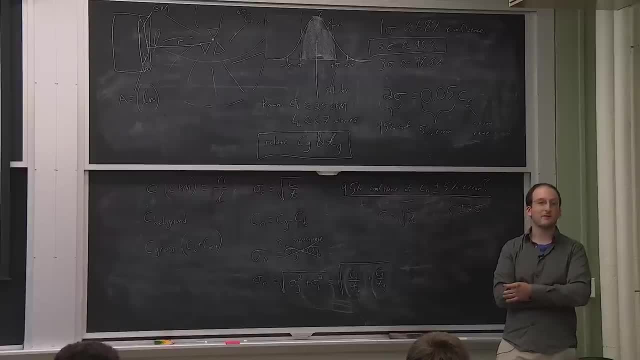 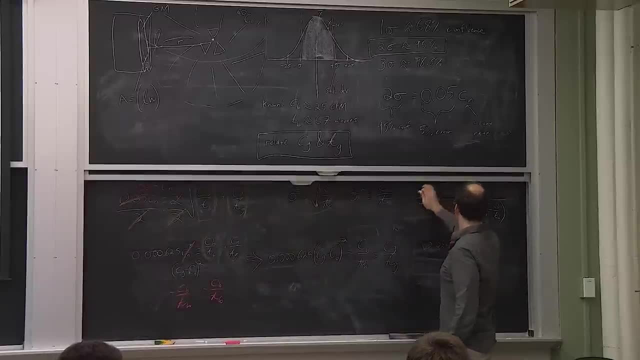 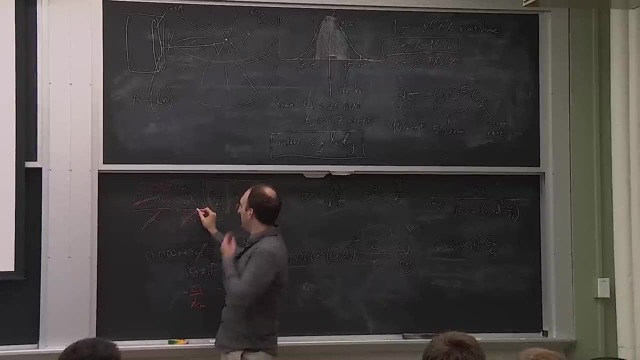 you're saying and be confident that you're giving acceptable bounds. So you can remain at 95% confidence, which means: where did that part go? Yeah, over here. which means: keep your 2 sigma, But you can then increase your allowable percent error. 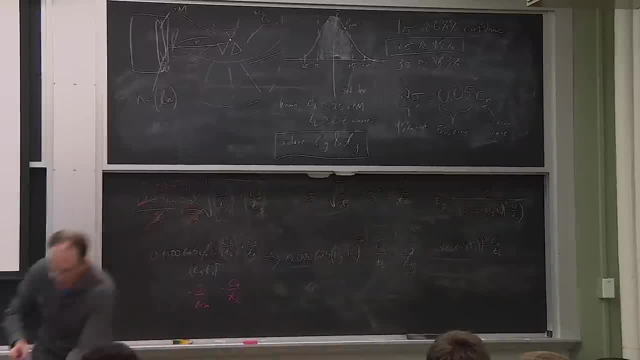 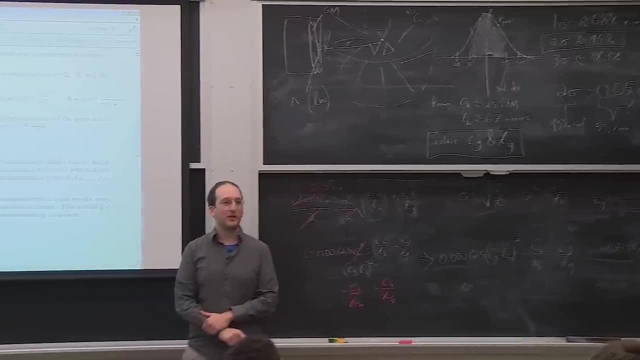 So if you can't get within 5% error- and I believe the homework doesn't actually say that for a reason- yeah, we don't tell you what error to choose, But we do say try to get to 95% confidence. 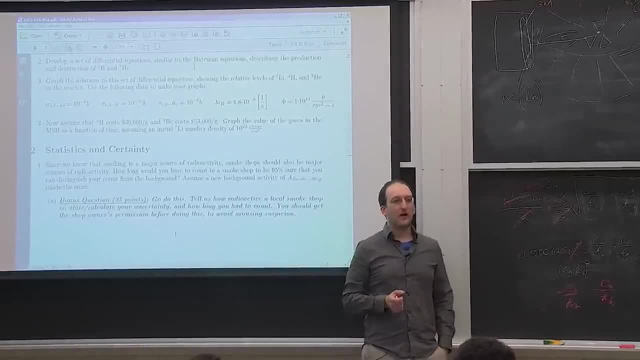 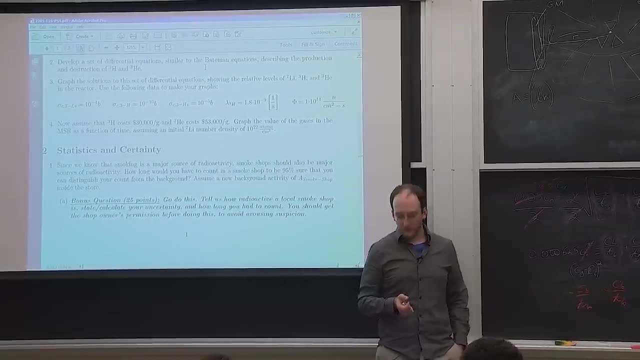 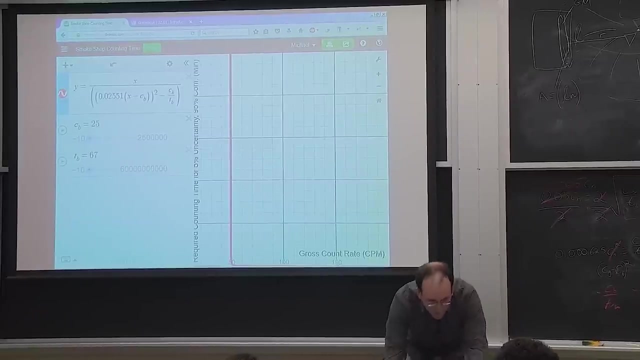 So then the question is: for a reasonable counting time, to what error can you get within 95% confidence? The more error you allow, the shorter time you have to count for, And I want to show you graphically how some of that stuff interplays with each other. 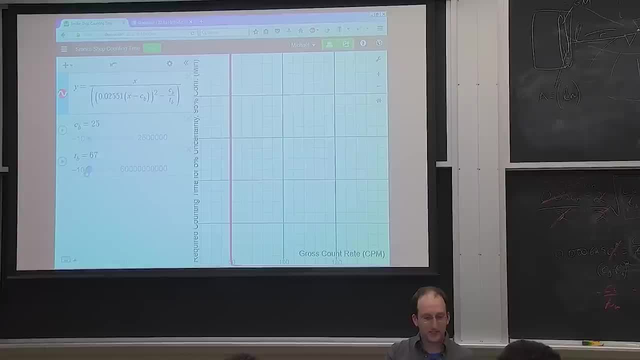 Let's say you were to increase your counting time, Which we can do here with this slider. So for the same background counting rate, if you increase the counting time, what happens to the uncertainty on your background experiment? Does it go up, down or nothing? 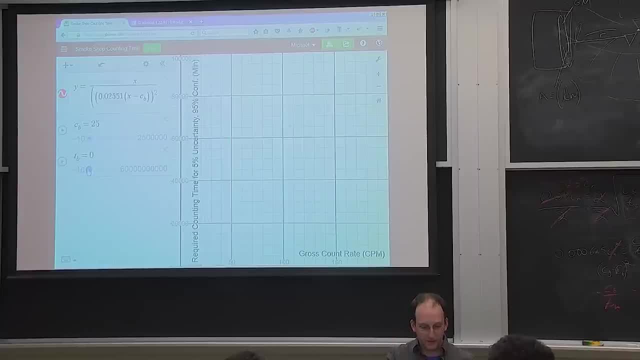 It's going to go down. Yeah, count for longer The uncertainty goes down. I'm going to have to change the bounds here to something more reasonable. So we were at 67 minutes And now notice As you increase your counting time. 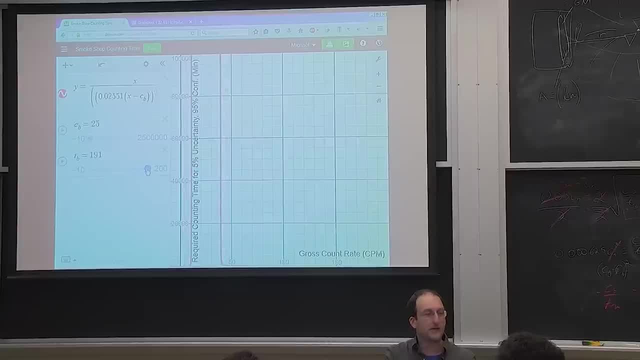 even though you haven't changed the counting rate. it then takes less time to distinguish, whatever your source is. So let's say, count for less time in the background. You have to count for more time in the experiment until it just kind of explodes. 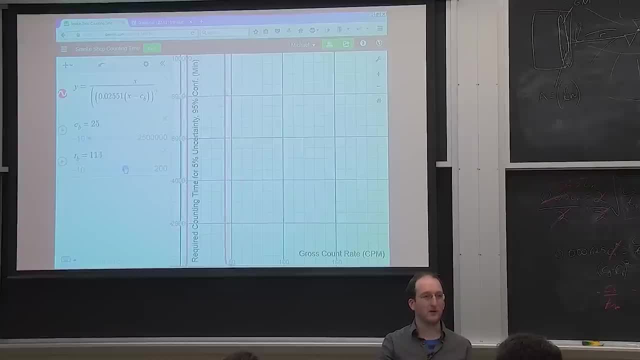 Count for more time in the background. You have to count for less time in the experiment in order to get to the uncertainty and confidence you want to get to. So if you doubled your background count time from 67, minutes to 134,, then you can measure count rates. 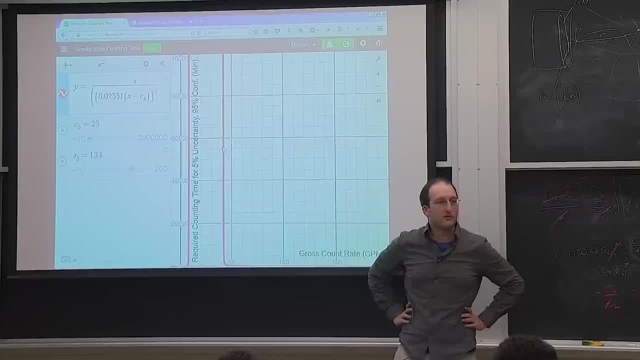 as low as 42 counts per minute gross. So when you start going into the smoke shop you can, let's say, count for a few minutes, get some very crude estimate of the counting rate and then decide how long you have to let your background accumulate. so you 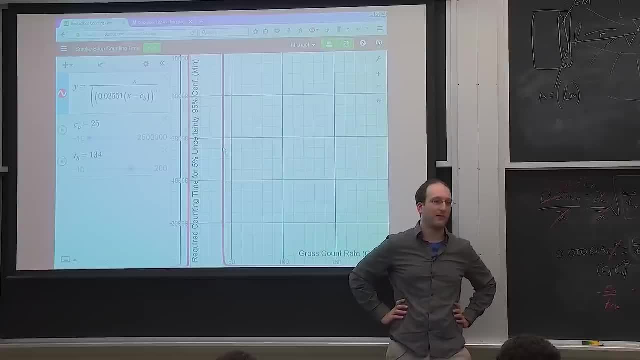 can distinguish the activity in the smoke shop to within some confidence and some error. Yes, So there's a background and then a smoke shop. So if you're sitting here, your idea is how do you do it? Sitting and setting? It's definitely location dependent. 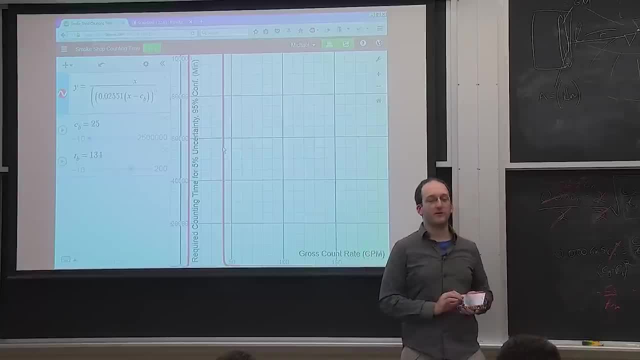 So we will get into background counts and sources of background radiation in about a month. But to give you a quick flash forward depends on your elevation. to say how much of the atmosphere is protecting you from cosmic rays Definitely depends on location. So in New Hampshire the background 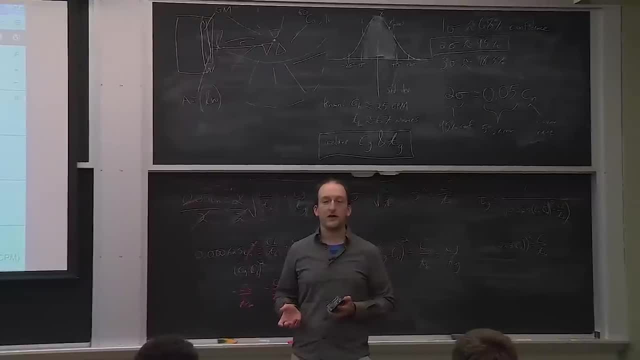 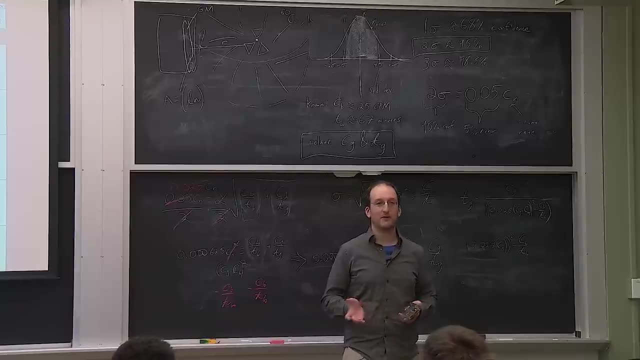 counts quite a bit higher because there's a lot of granite deposits And granite can be upwards of 52 parts per million uranium radium. Conway granite in particular, named after Conway, New Hampshire, is pretty rich in radium ore. 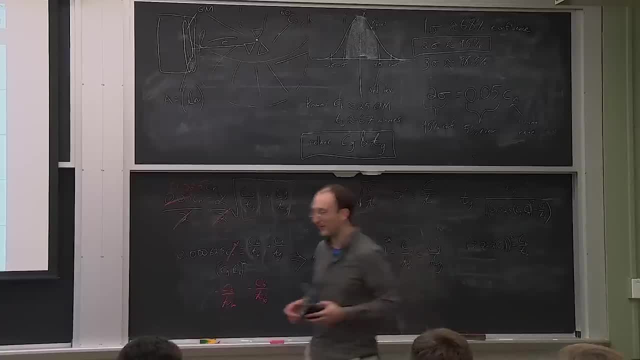 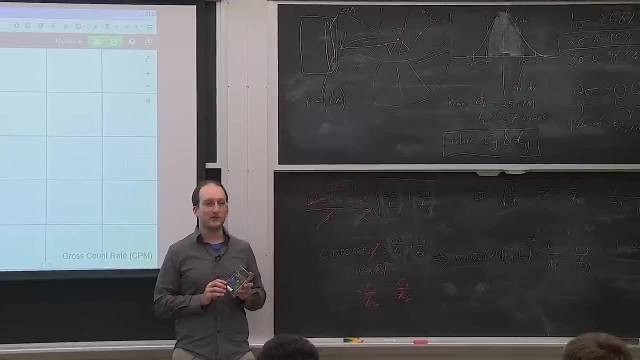 Is that where you're from? No, the last place I went. Oh, there you go. OK, Yeah, It's also neat You can use background counts as a radiation altimeter. One of my graduate students actually built a Geiger counter. 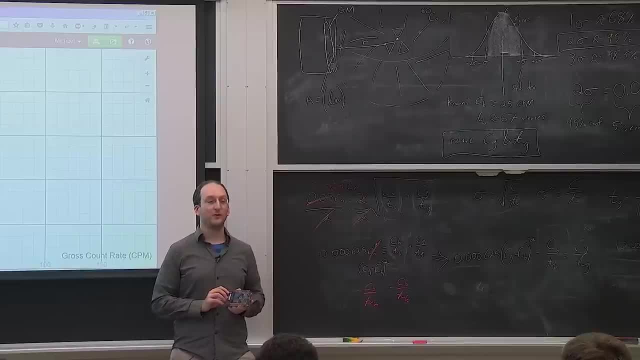 interface to an Arduino where you could actually tell what the height you were flying at is by the amount of background radiation increase. So certainly it's going to depend where you are right, But you want to make sure that you're in an area to answer Sean's question. representative of where. 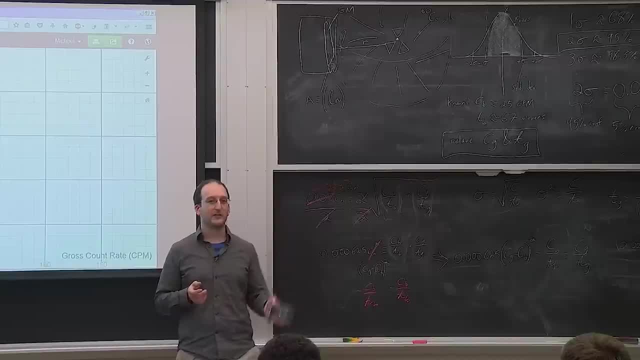 the smoke shop is. So you can't go into the reactor and drop this in the core and say I'm doing a background count, That's not a valid experiment. So yeah, you'd want to be, I don't know. same block right. 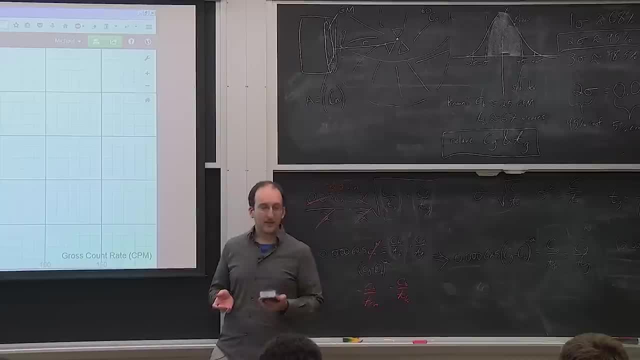 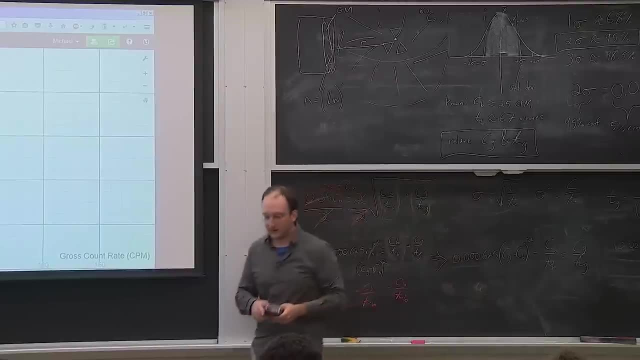 That would be pretty good. And then go in there and see: can you measure any sort of increase? Get a crude estimate of your CG, your gross count rate. Use this formula right here to estimate how much time you've got to wait. 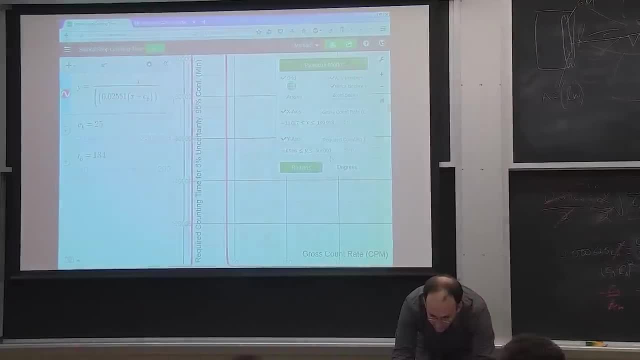 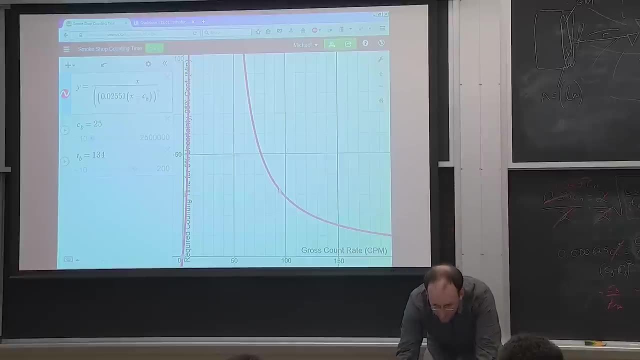 So, for example, let's shrink our y-axis down a little and be more optimistic than we probably should. Let's say you go in there and you get a count rate of 100 counts per minute. That would surprise me. You'd only have to count for an extra 28 minutes. 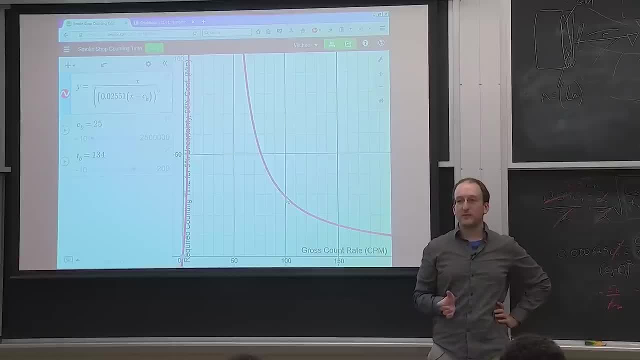 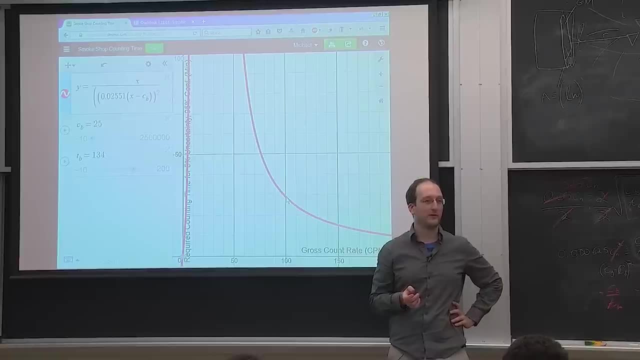 to nail that net count rate with 95% confidence to 5% error. Let's see now what happens if we increase the allowable percent error. So let's say 10% error would be acceptable. We just take that number double it. then all of a sudden, 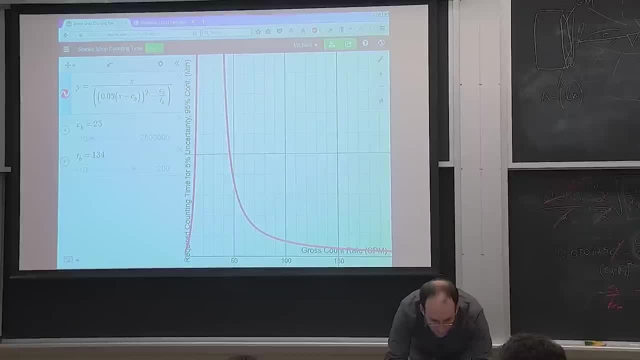 you don't have to count for nearly as long. So again, at 5% error, which means a 0.25 here. at 100 counts per minute, you'd have to count for well, about 30 minutes If you're willing to accept 10% error. 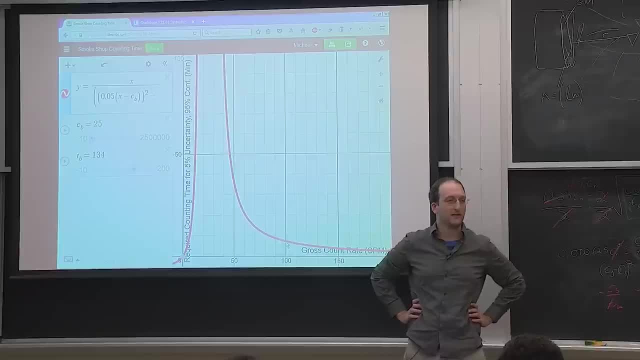 that goes down to 7 minutes And 18 seconds. So do you guys see the general interplay between confidence, percent error, counting time and counting rate? Who here has built an NSE Geiger counter before? Awesome, So this is definitely a try it at home, kids kind of thing. 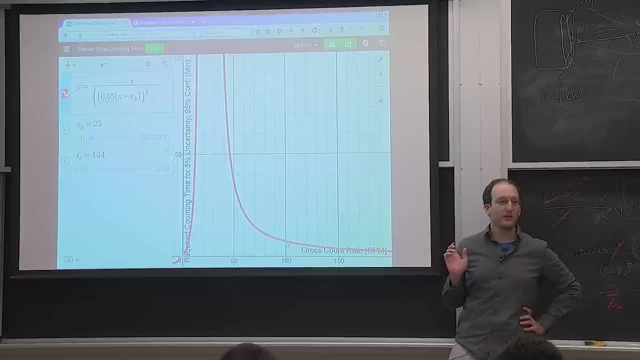 If you want to find out, is something radioactive? this is what you can actually use to find out. answer the question: is it discernibly radioactive to within some limit of error or limit of confidence? That's what we're going to be doing here. 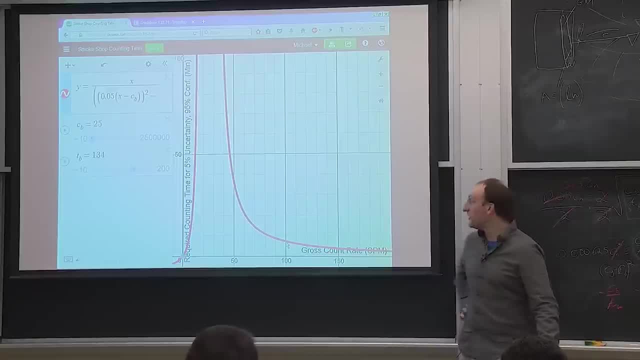 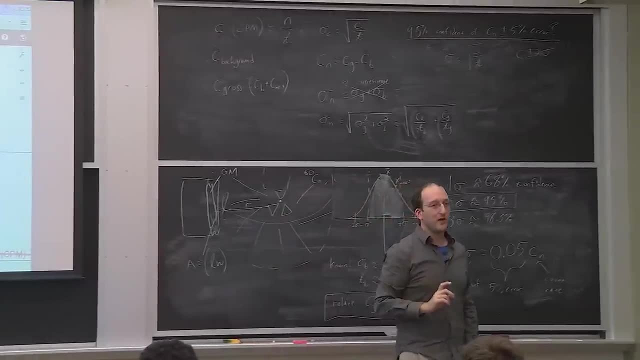 with a much, much, much more sensitive detector. So the only thing missing from our complete picture of going from the activity of a source, which we've shown you how to count, to dealing with the solid angle, which is just a simple formula. 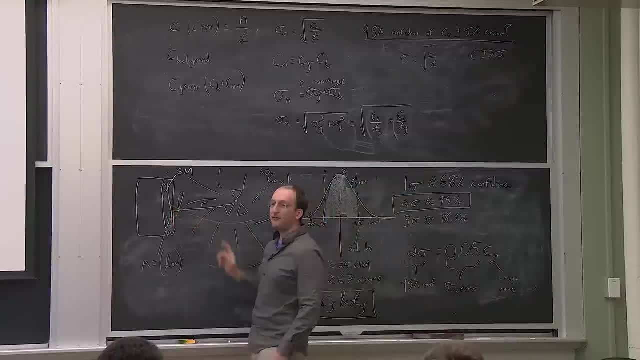 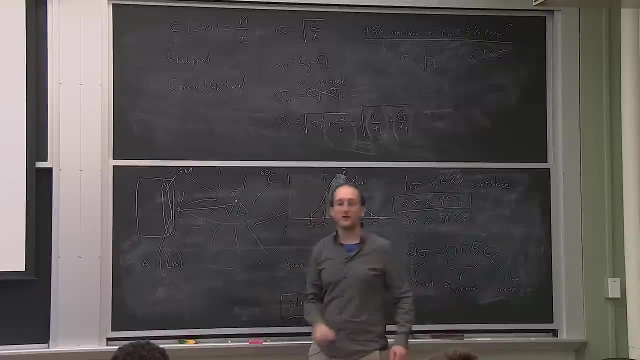 to dealing with statistics and uncertainty is now the efficiency of this detector. Out of the number of radiation quanta or whatever that enter the detector, how many interact and how many leave out the other side. That's what we're going to be spending most of the next month. 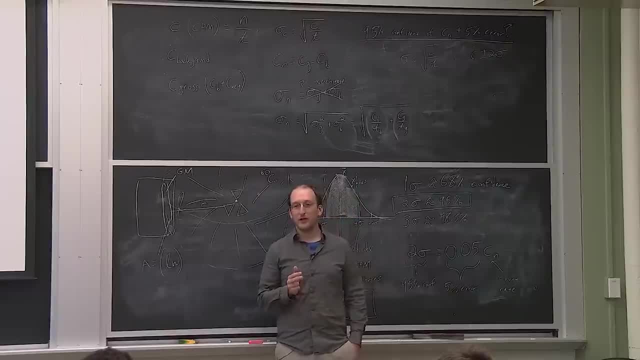 on when we do ion, photon, electron and neutron interactions with matter. So we'll find out what's the probability, per unit length, that each one undergoes an interaction, what kind of interactions do they undergo, and then we'll complete this actual picture. 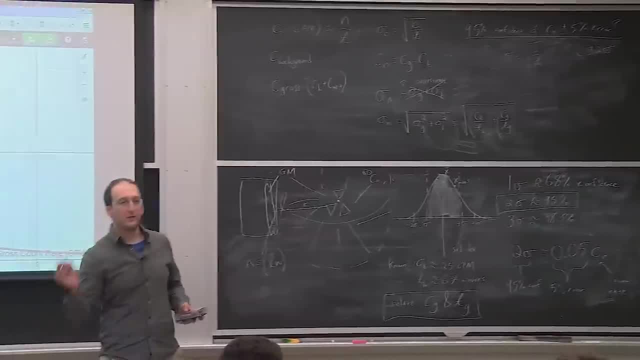 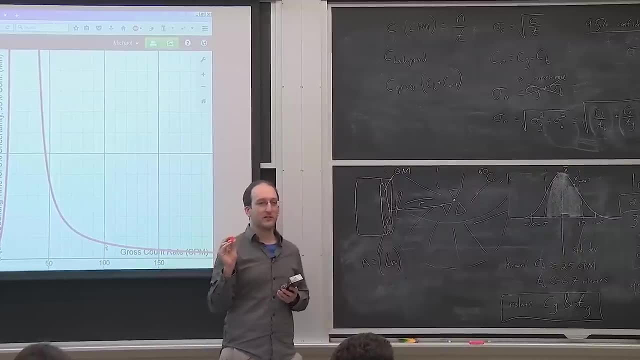 So you can take a source of, let's say, unknown activity, put it a known distance away from a known detector with a known efficiency, and back out what the activity of that source is with accuracy. That's what you're going to start doing on this homework. 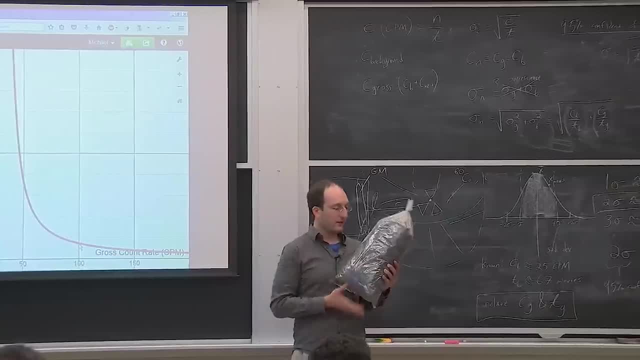 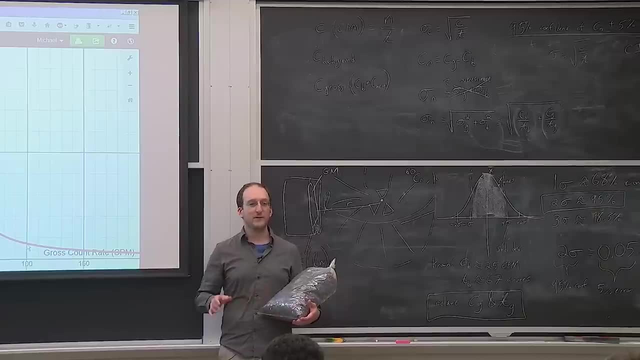 as well for the banana lab. The only thing you don't know is the activity of this bag of bananas, But we're going to give you all the information, like the efficiency of the detector and the geometry of the detector, and you're going to be able to measure the number of potassium. 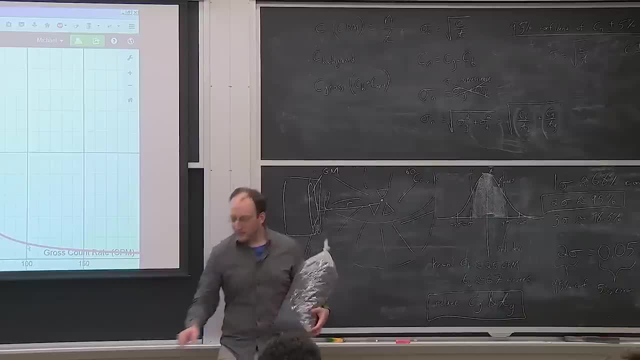 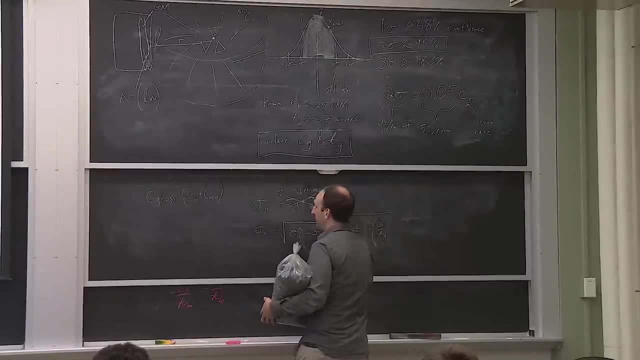 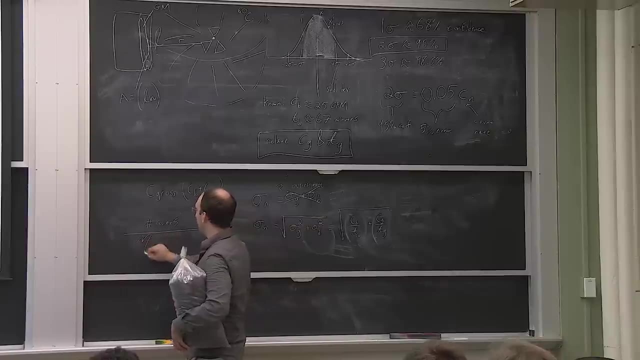 40 counts that the detector picks up. So by taking, let's see if we have some space left. We had a little bit here. So by taking that number of counts and dividing by, let's say, the efficiency of the detector. 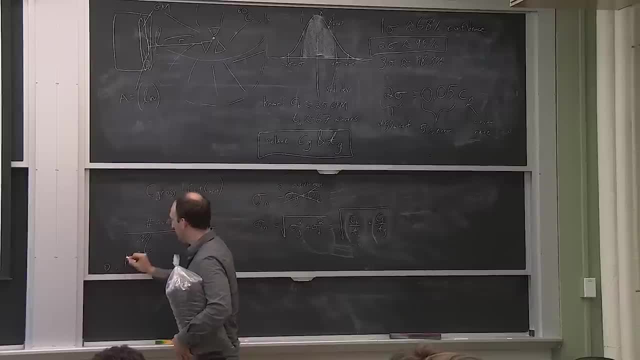 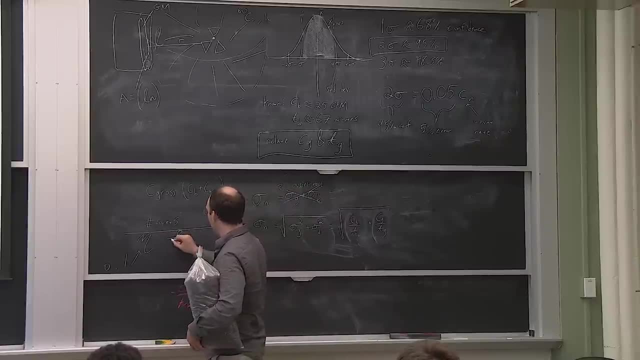 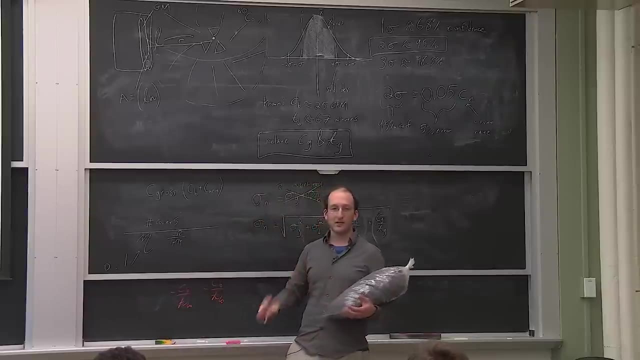 where that efficiency is going to range from 0 to 1,- probably much closer to 0, and also dividing by, let's say, your solid angle over 4 pi to account for how many of the emitted potassium 40 gamma rays actually get into the detector. 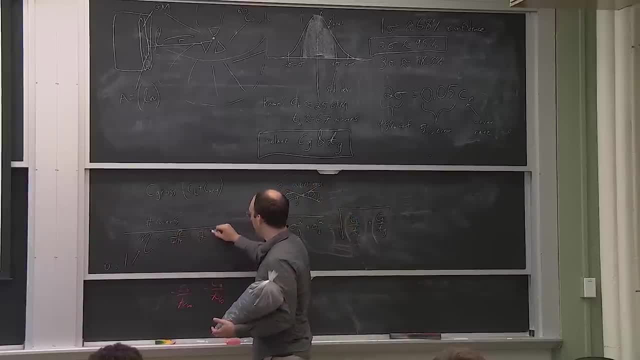 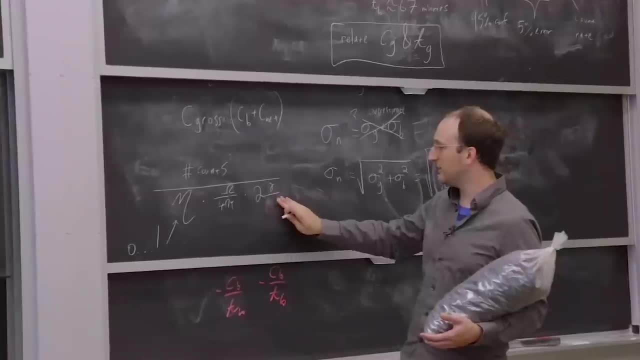 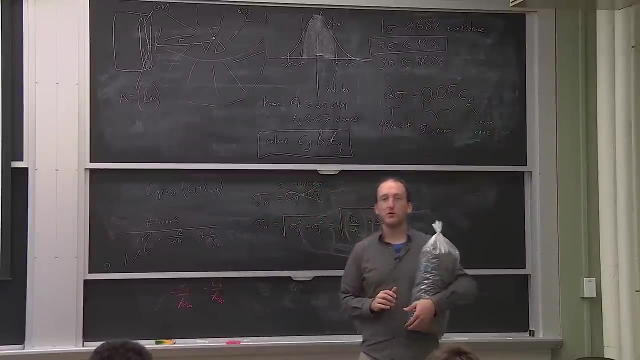 And Dividing by 2 gamma rays per disintegration. I think that's what we had last time, Or was that cobalt-60?? Yeah, We've been using cobalt-60 as an example, So remember we had 2 gamma rays emitted per cobalt-60. 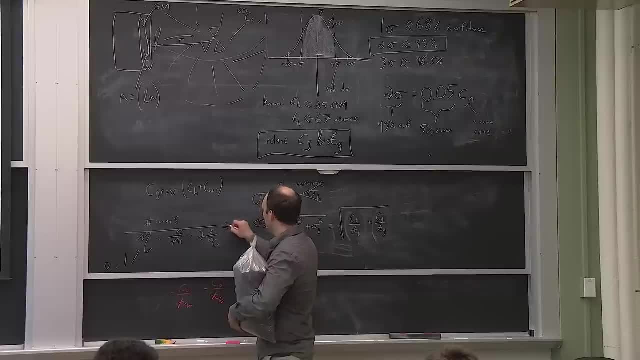 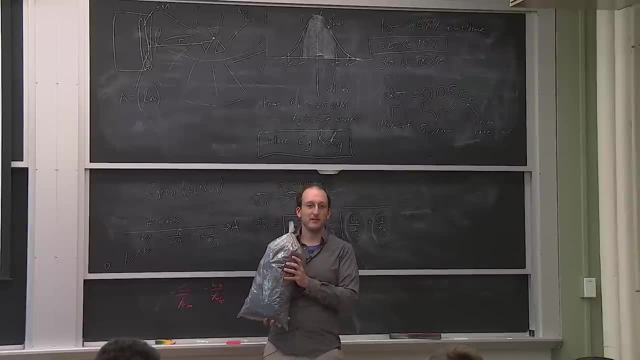 disintegration on average, Then you can get to the actual activity of the source. Once you know the activity of this bag of bananas, you can then divide by either the mass, or the mass of one banana, or the number of bananas, or whatever, to get the final answer. 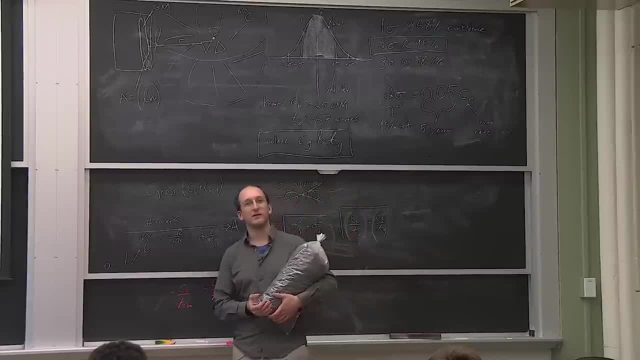 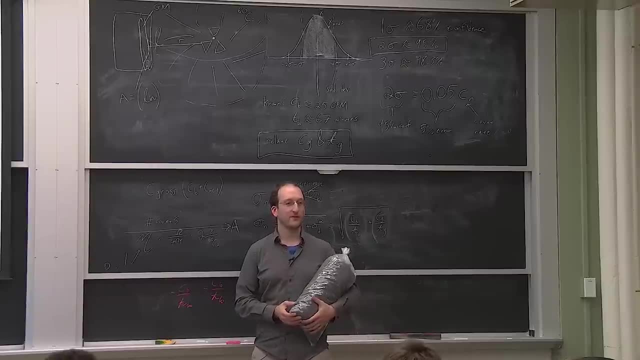 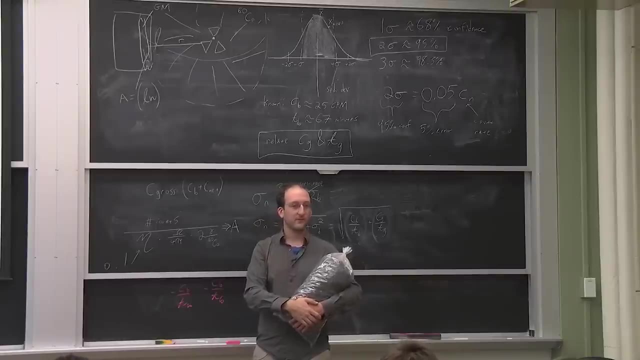 That's what we're going to spend the rest of today doing. So, since it's getting on 5 of 5 of, do you guys have any questions about what we covered today or what we're about to go do? You said that for solid angle. you want to do it. 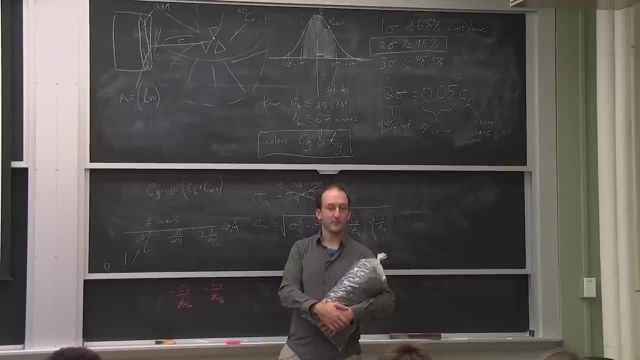 Yep, So for a solid angle, you just call it angle 2.3.. Yep, So for a solid angle, you just call it angle 2.3.. Yep, So for a solid angle, you just call it angle 2.3.. 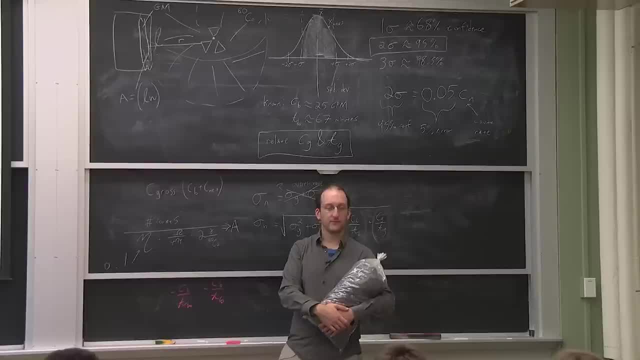 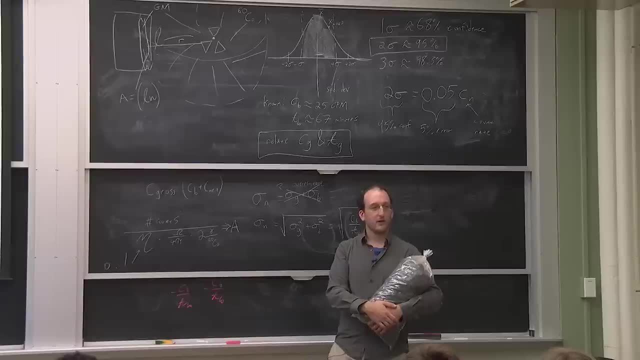 So for a solid angle, you just call it angle 2.3 over r squared. In this situation you're doing the solid angle over 4 pi because you only have maximum half the sphere, Not necessarily. Let's say you were to encase your detector. 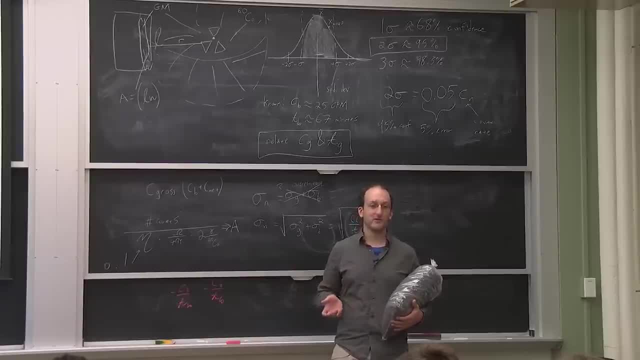 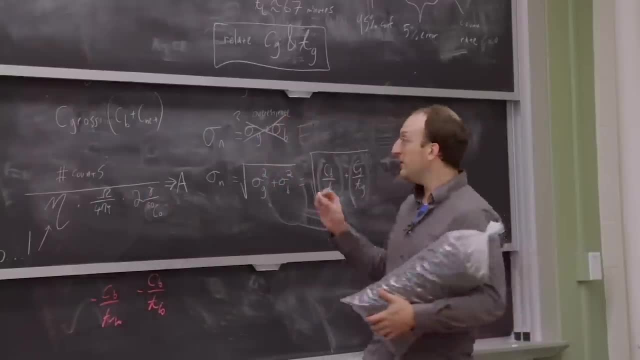 in an infinite medium of radiation material. right, Then you could subtend 4 pi. So the idea here is that if you captured every single gamma ray, your solid angle would be 4 pi. So if your solid angle is 4 pi, then that would equal-ish. 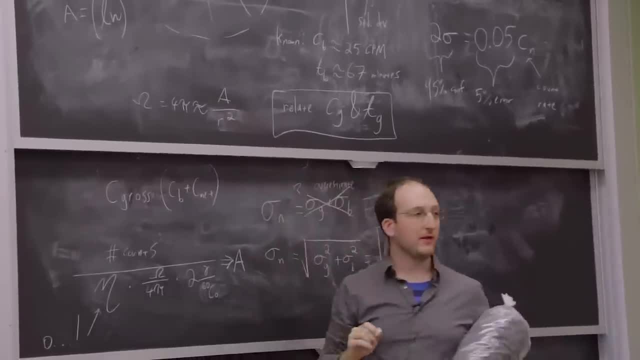 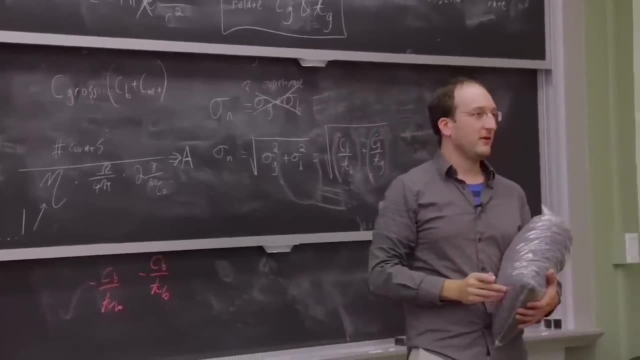 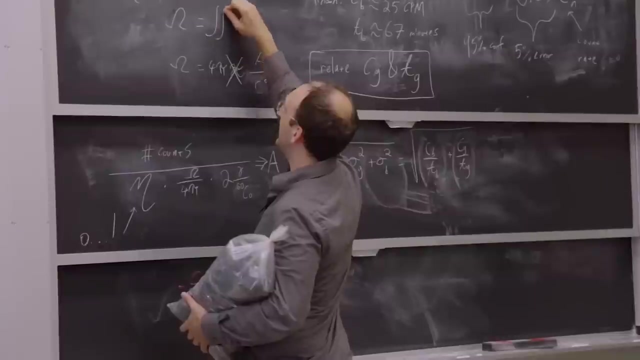 the area over r squared of your thing. But this is actually not that good of an approximation when you put a source very, very up close to a detector. So there are actual formulas for solid angle where the real formula for solid angle you actually end up having to do a surface integral of the sine. 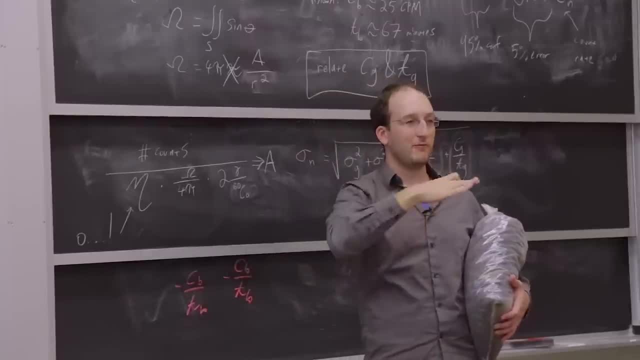 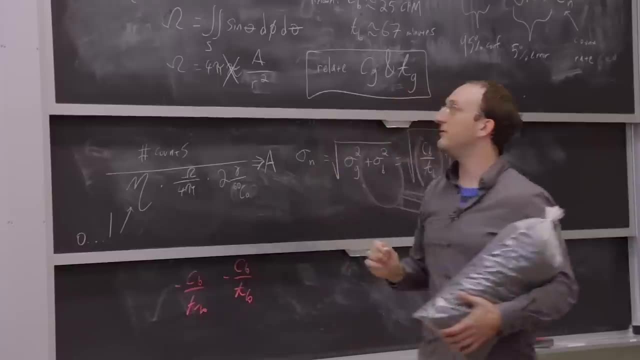 let's say, which accounts for the fact that the object that you have might be, let's say, tilted towards or away from the detector. So you're going to have to do a surface integral of this unit, sphere times, some differential d theta. what is it? d phi? 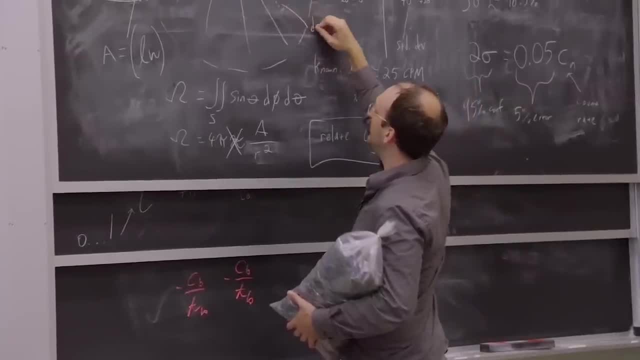 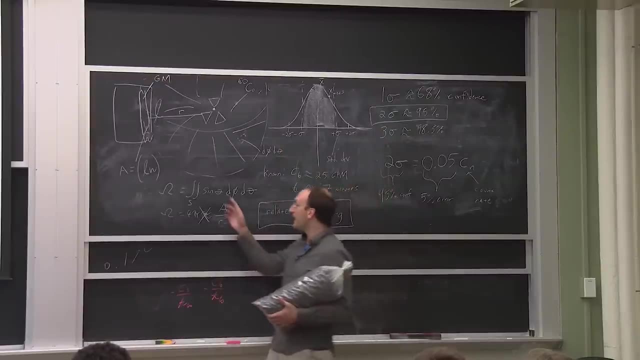 d theta of this unit sphere. So you'll have to integrate to say how many of these little d phi d thetas are actually subtended by your detector And the value of that actual surface integral gives you the real solid angle. That's the super simple one. if you just 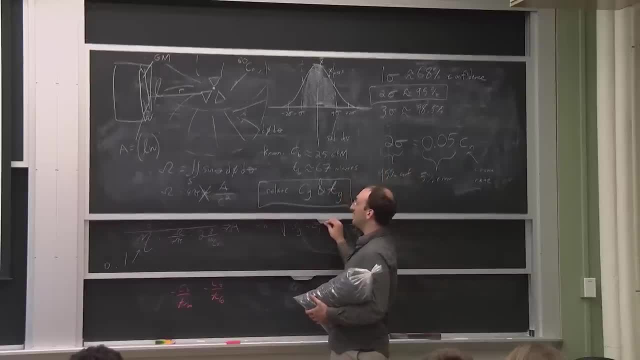 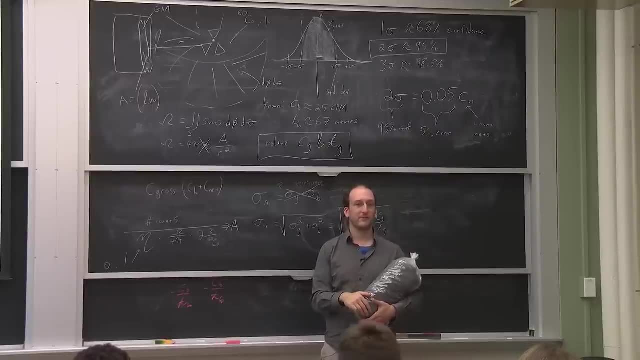 know the area of something and you know that you're kind of far away. So whenever possible, use the exact formula. So any other questions? Yeah, Sean, You said that that expression that you'd given for cobalt-60 is just the simulations per second right. The two gammas per cobalt-60, this one, Yeah, That accounts for the fact that, if you remember the decay diagram for cobalt-60, how does that decay? By beta emission. It goes to one energy level and it tends. 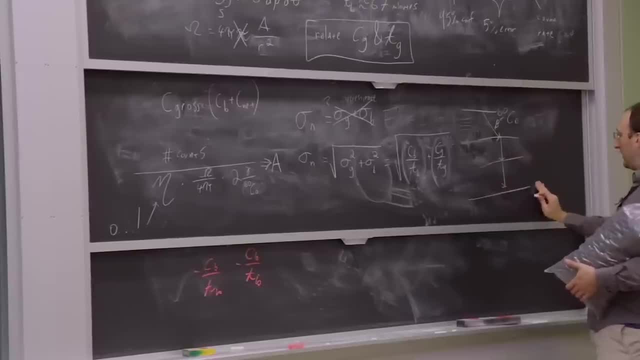 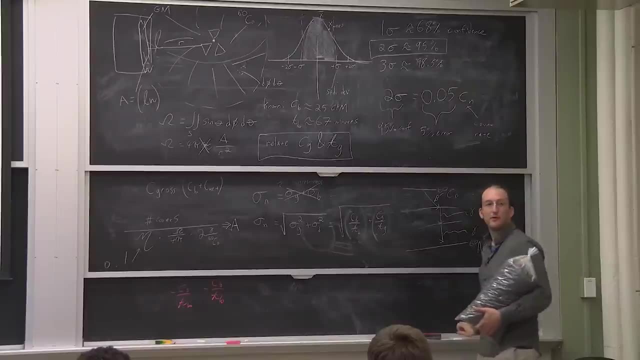 to go down by two gamma decays to nickel-60.. So each time it gives off a gamma ray to one level and a gamma ray to another level. So in this case, one becquerel of cobalt-60 would give off two gamma rays per second. 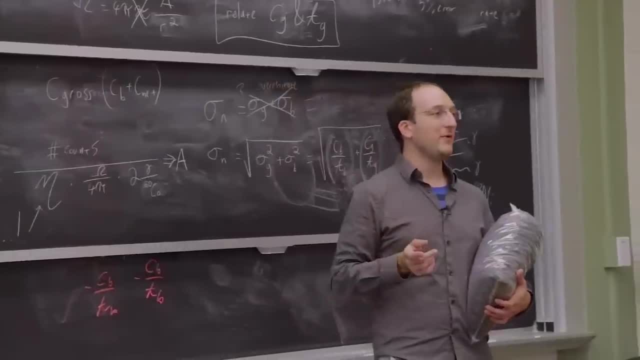 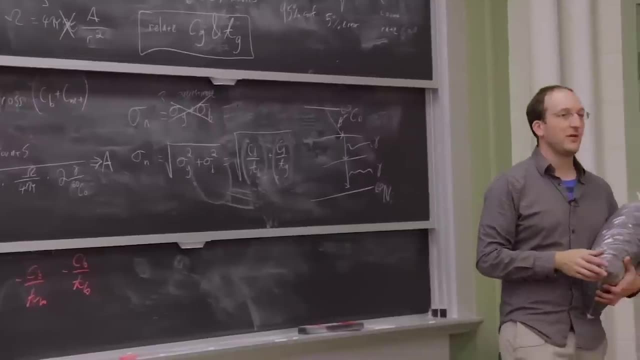 So if you are measuring a number of counts, at each count one gamma ray was responsible- You have to then divide by the number of gamma rays per disintegration on average in order to get the actual activity of that source. So remember, activity is measured in disintegrations. 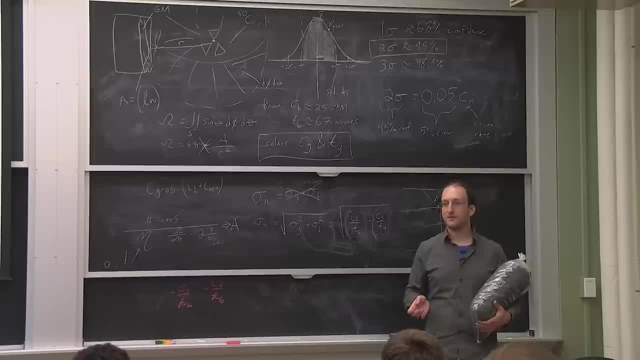 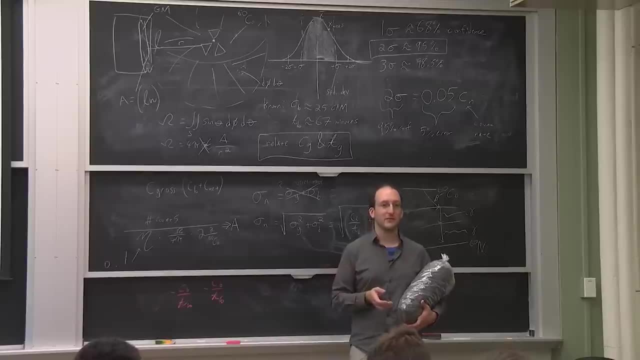 not in number of gamma rays emitted. That's the difference here. Dose, you'd actually care about how many gamma rays you absorb, But activity is how many atoms are disintegrating per second. Yeah, The units of cobalt-60, is that just? 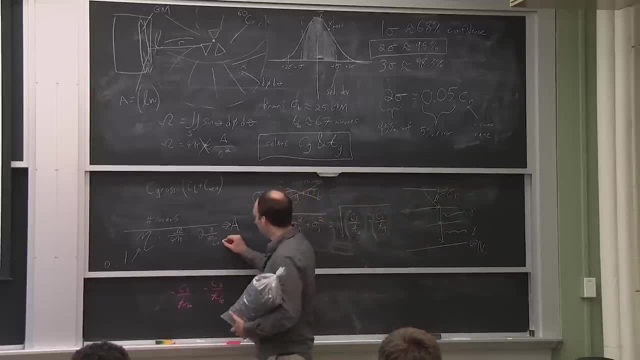 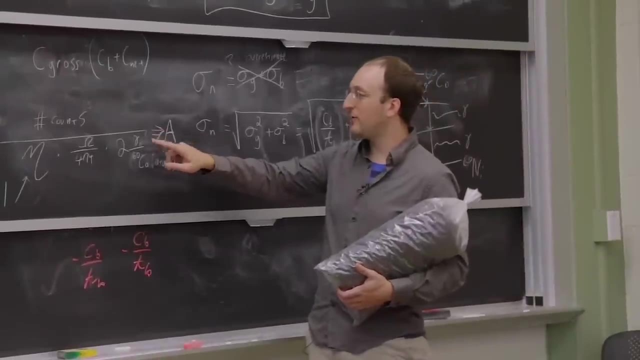 The units of cobalt-60?? It's just two gamma rays. Oh, this would be like atoms of cobalt-60.. And those gamma rays would be gammas per atom. So in this case it's like two gamma rays per atom of cobalt-60. 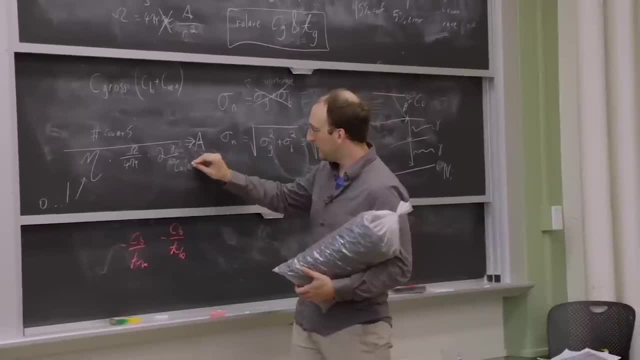 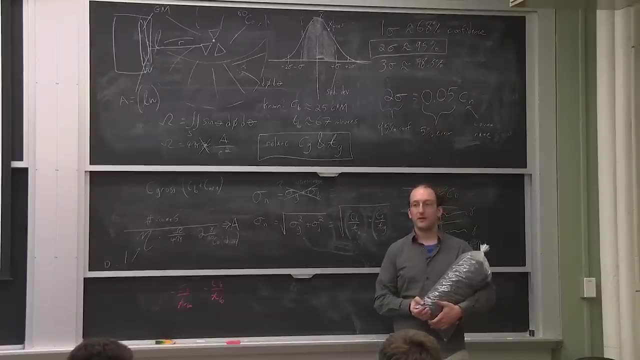 disintegrating or, better yet, per disintegration. So you've got to know what material you're looking at in order to know how many gammas or how many betas or more that you're going to get per disintegration. Yeah, 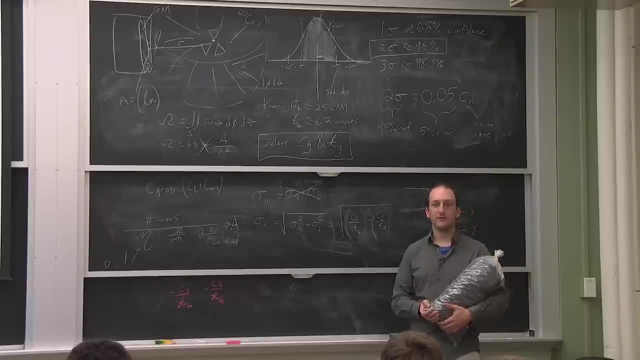 Who here has heard of this uncertainty in quadrature before? Just a couple of folks, OK Yeah, the idea here is that again, if you just add the errors up, you're probably overestimating the error and selling yourself short. 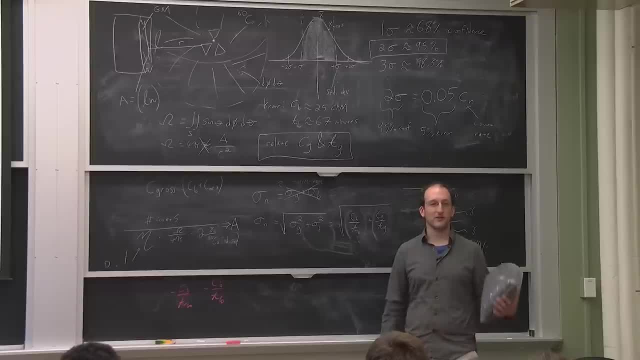 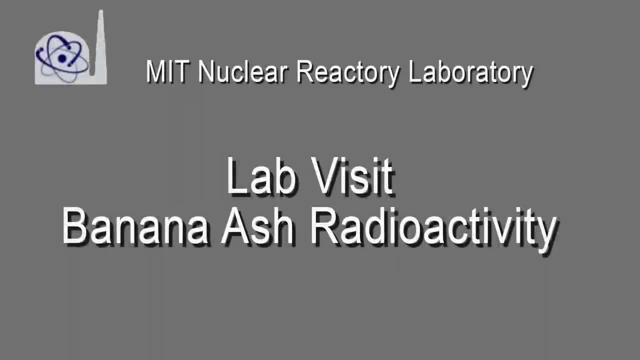 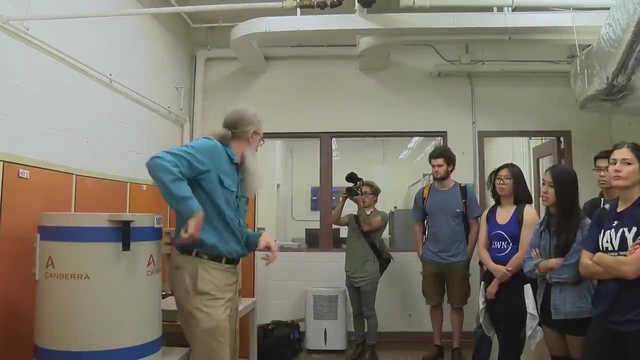 Cool, In that case, if there's no questions, let's go do this. So follow me to the counting lab. OK, so this is my counting lab. These are three high-purity germanium detectors. Have you explained high-purity germanium detectors? 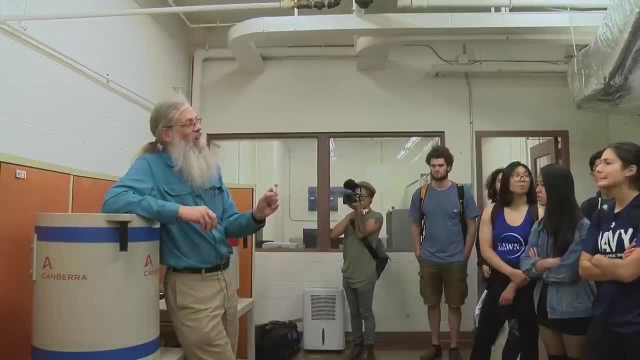 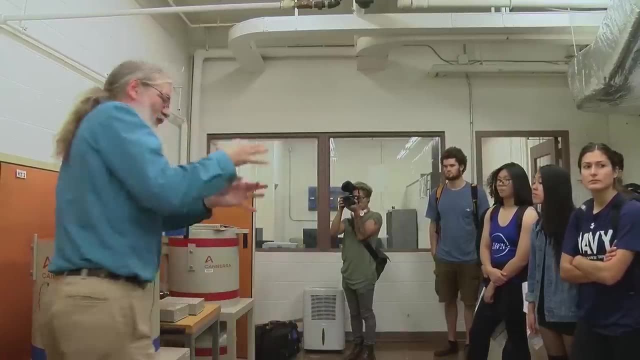 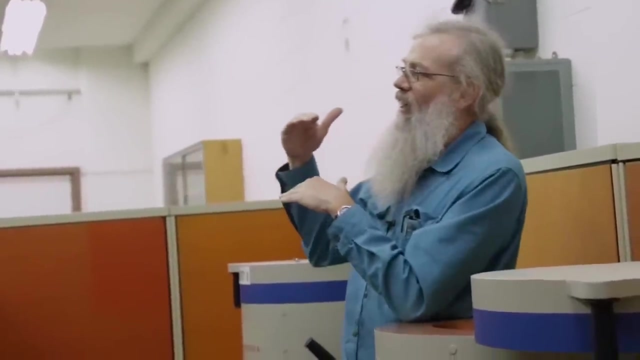 OK, have you explained any detectors? Just the Geiger counter we were playing around with today. OK, well, here Down in here there's a little high-purity germanium crystal with a couple thousand volts across it. When a gamma ray goes into it makes some electron-hole pairs. 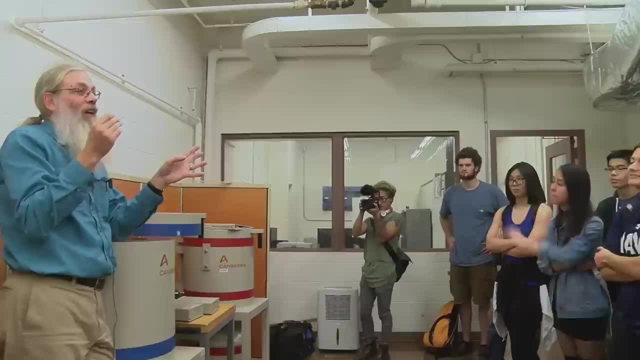 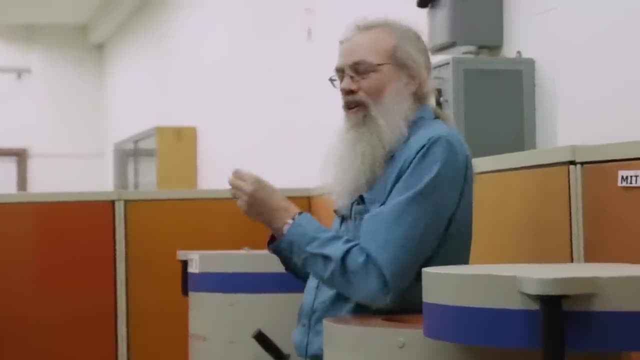 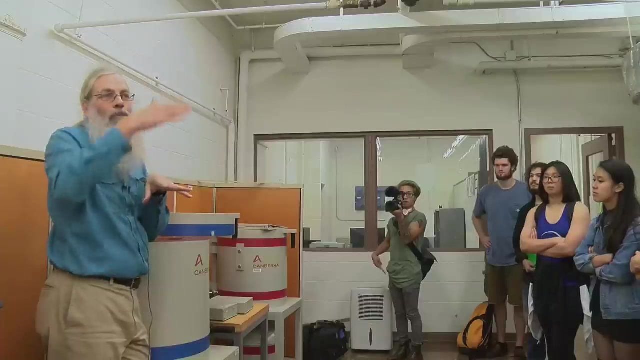 Nod when I say electron-hole pairs, OK, good. And basically you get more electron-hole pairs the more energy of the gamma you have. So you collect the current from that And you get a little pulse of current And the height of the pulse tells you. 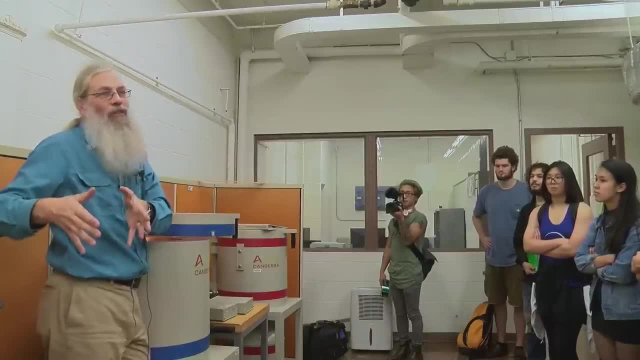 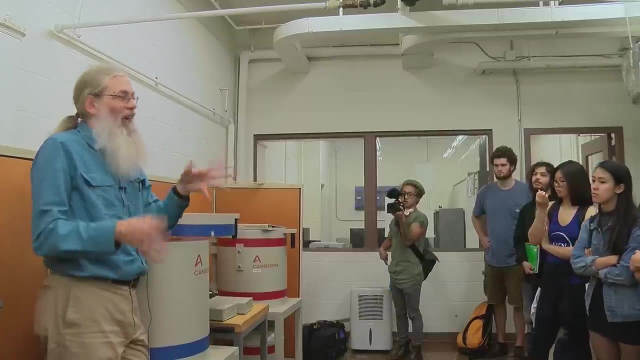 how many whole pairs you had And then back it up to what the energy of your gamma was. That works fine if you collect all of the gamma energy. You don't always quite do that, But anyway. so that's how the. I mean I don't know 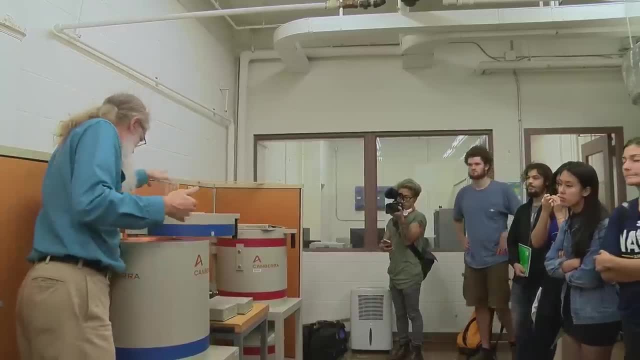 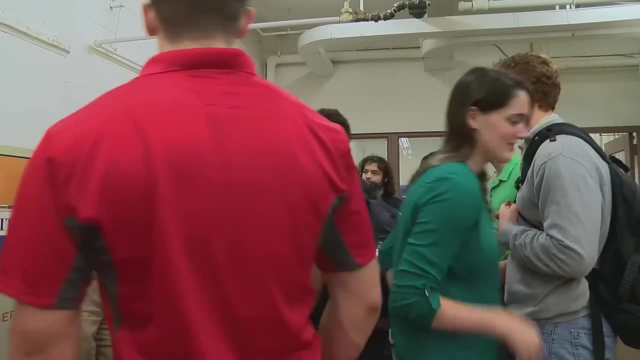 You all can scooch up. I mean there's not a whole lot to see in there, But it's worth a look. I mean, you can't really see the crystal. There's just an aluminum cylinder in there. The black part is just a carbon fiber window. 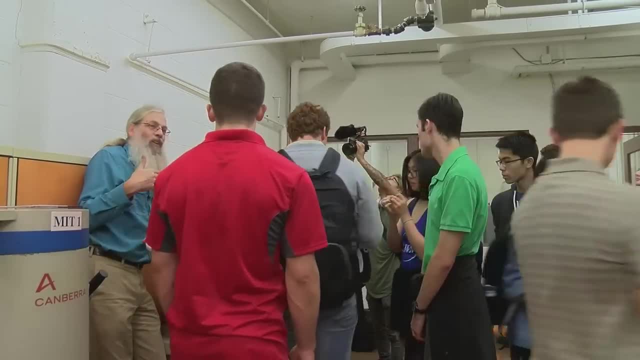 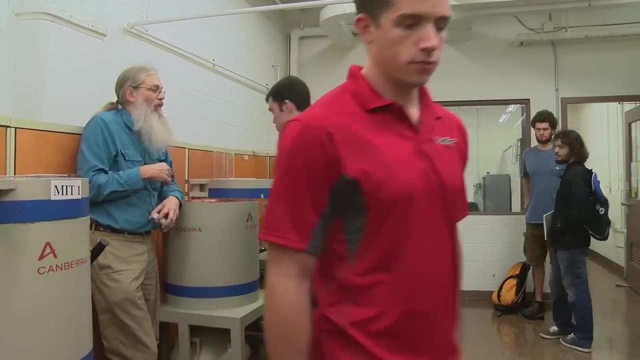 Because you don't want to cut off the low-energy gammas. So it's got a really thin- OK, It's got a really thin- carbon fiber window on it. What's with the hundreds of pounds of copper on the side? What's with the hundreds of pounds of copper on the side? 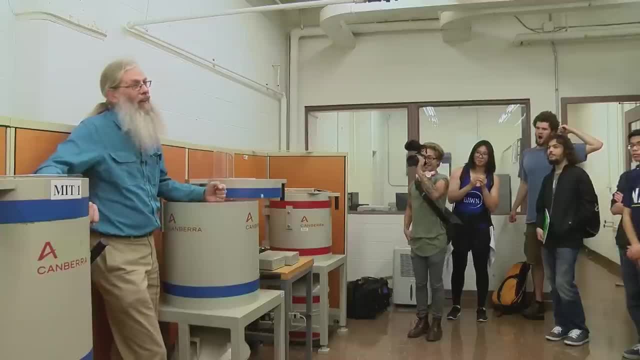 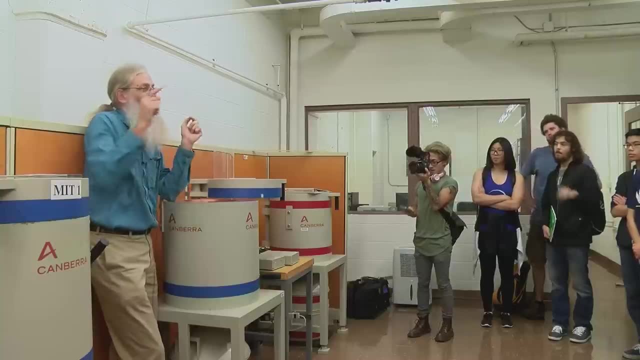 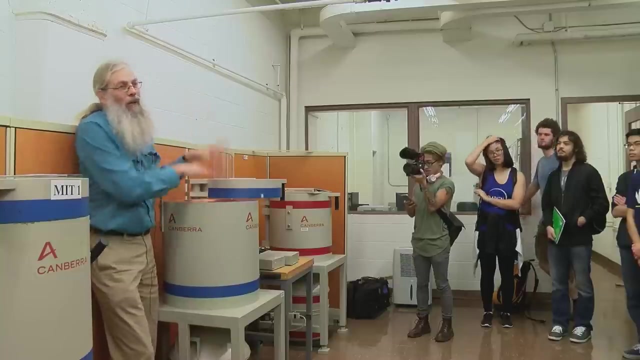 There's not a hundreds of pounds of copper on the side. These guys are lead, which does two things: It shields the detectors from the activity out here, from you guys from the activities coming out of here, Because sometimes I'm counting very low activity samples. 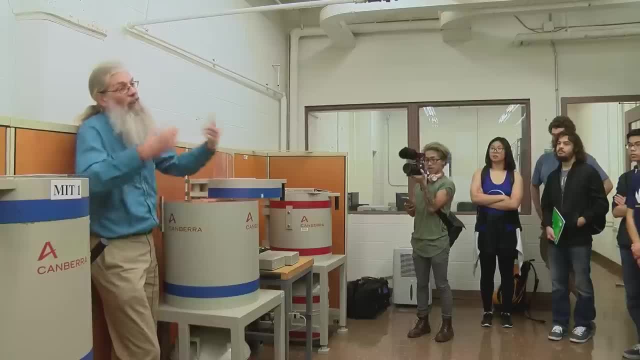 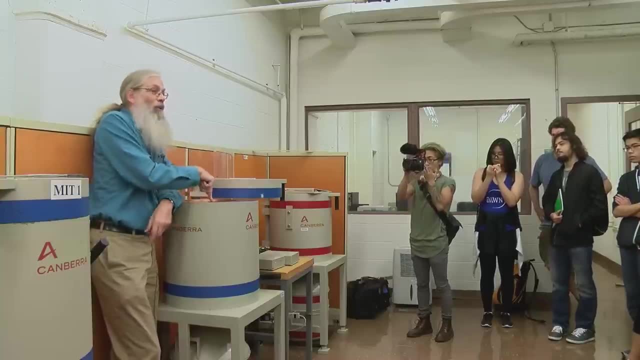 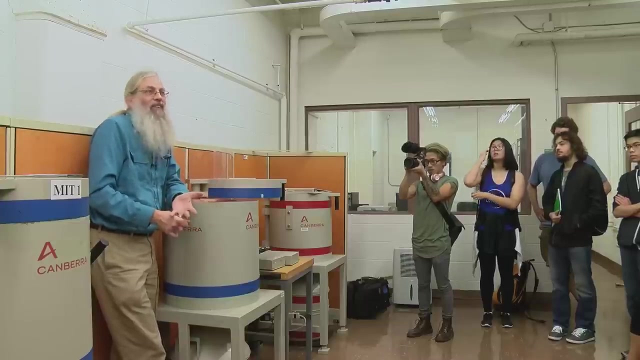 And it also, if I'm counting something that has a lot of activity, it shields us from that activity, So it kind of goes both ways. The reason there's copper is if you get a high-energy gamma ray into some lead it makes x-rays. 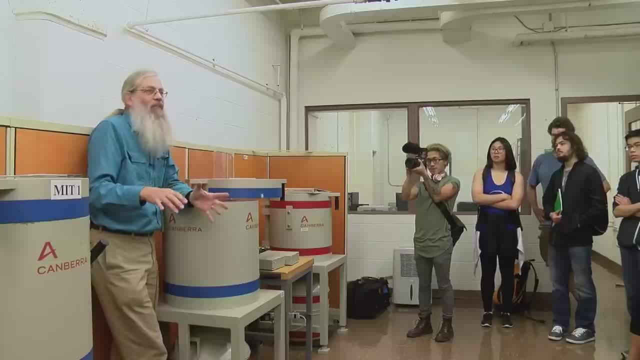 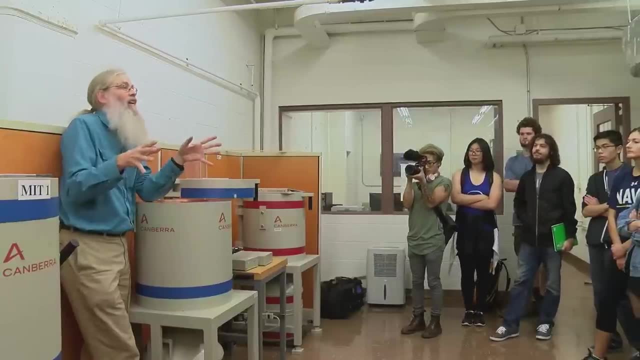 And it makes a very nice 75 keV. You guys know keV Good, We've done x-rays Awesome. It's a really nice 75 keV gamma x-ray. that interferes with trying to count things around 75 keV. 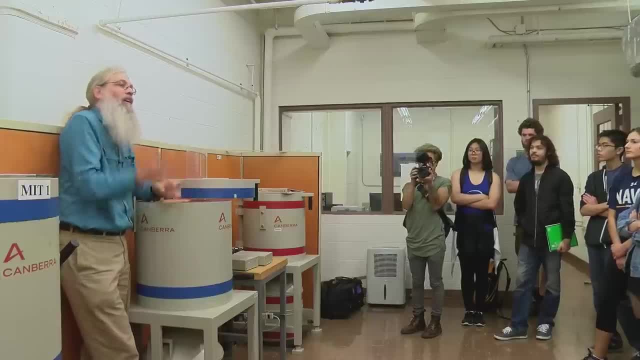 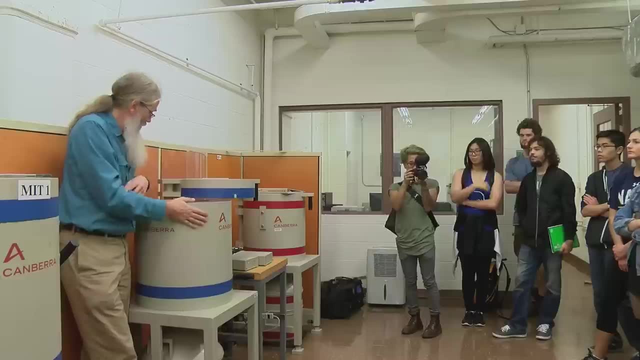 Because you're getting all the energy, You're getting all these x-rays coming out of lead, So you line it with copper, which makes a lower-energy x-ray and filters out the lead x-rays. So anyway, yeah, so this is just these. 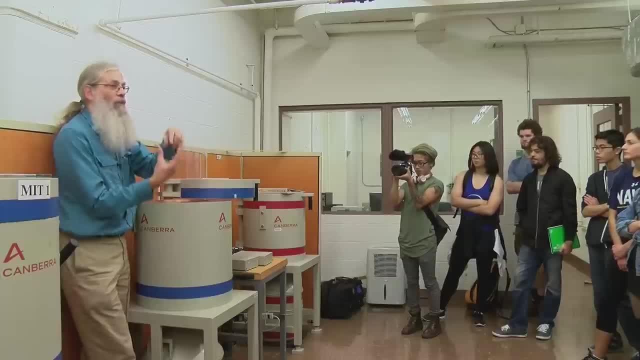 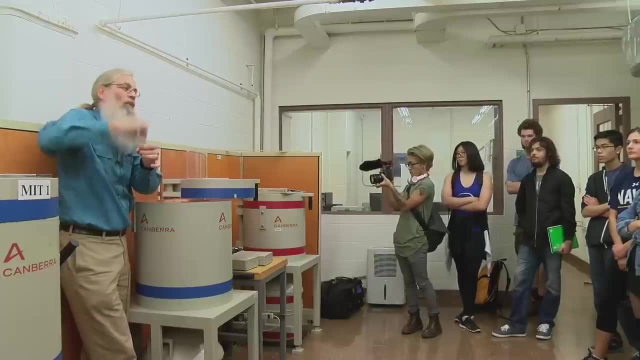 I've got two germanium detectors. That one's also germanium, It's a well detector, So it's got a little 1 centimeter hole in it So you can stick a sample right in the germanium. They're hooked up through a little electronic box. 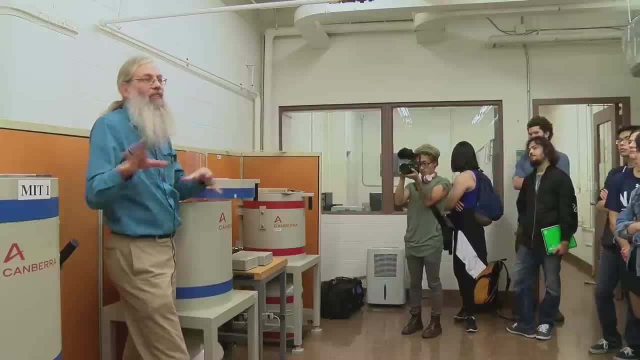 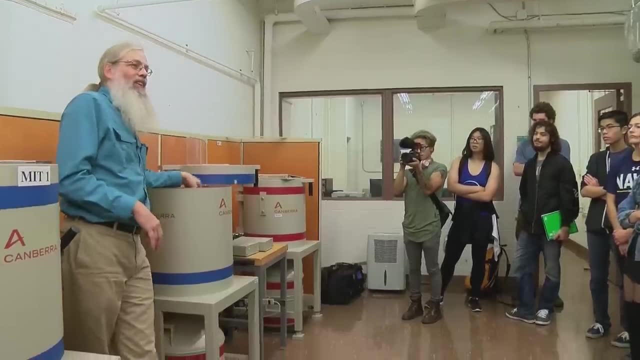 and go into the computer And you can see the good stuff over there. that does all the peak height analysis. Oh yeah, liquid nitrogen doer, Thanks for pointing. Yeah, you cool the electronics and everything down so it cuts out the thermal noise. 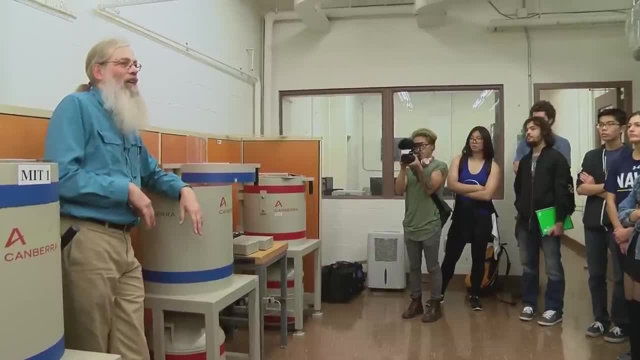 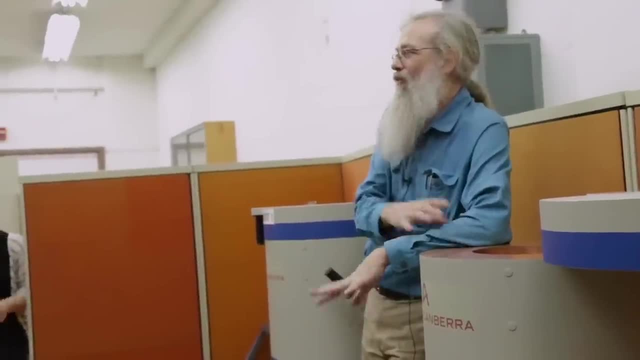 Because you're looking for really tiny little signals here. so you cool everything down And that way it's not too noisy. These guys are OK. warming up, It doesn't destroy the detector- The old detectors you had to keep cold all the time. 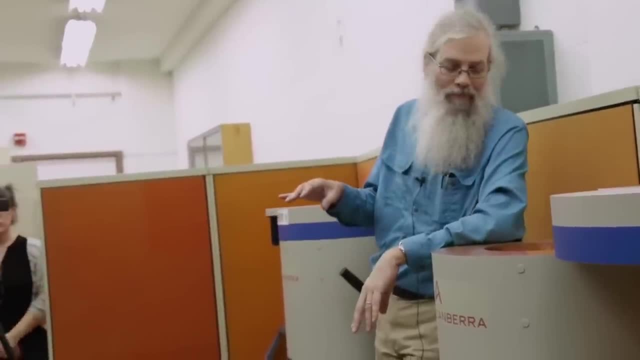 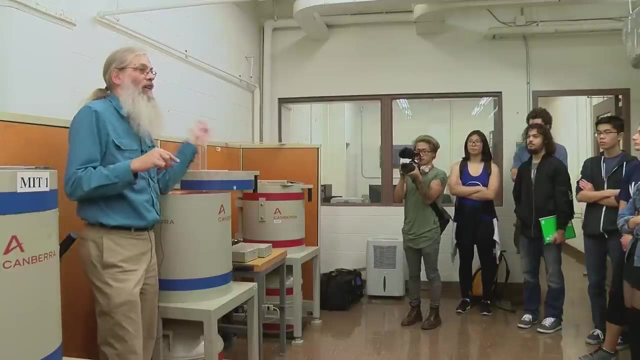 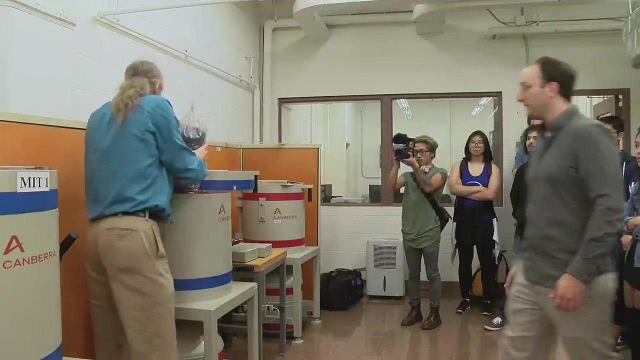 than they were just paperweights, um. but so this is just the counting lab. uh, i've got an actual sample counting in here right now. we'll take a look at the spectrum. in a minute your bananas are gonna go here, um, and let's see if we can smash it down. yeah, because it'd be nice if i. 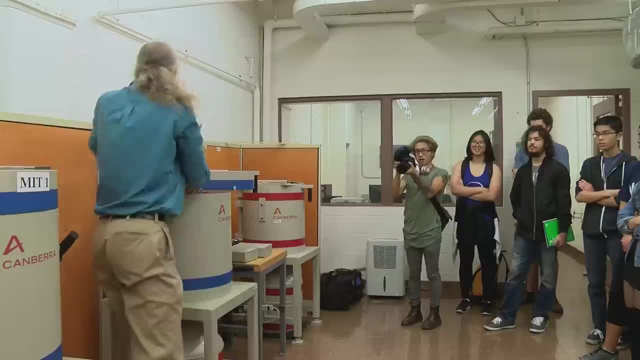 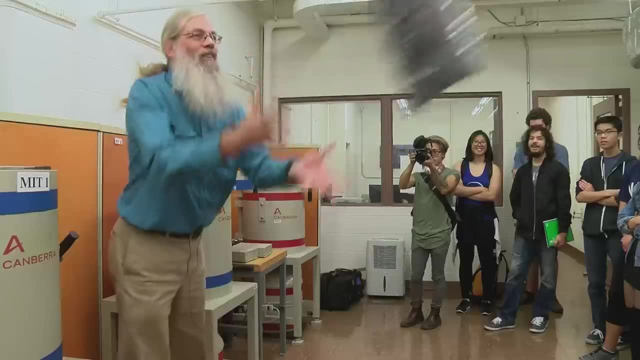 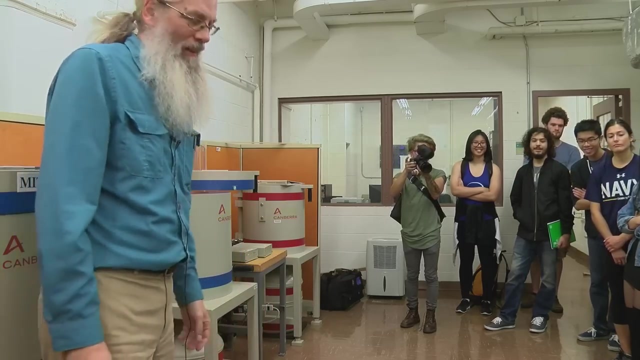 could close the lid. oops, almost well, we'll smash this down here. one of you guys do this, you. you smash that down until it fits in there, although don't break the bag. oh okay, we'll get another bag. no, it's okay, it's just banana ash. um, we'll find another bag, that's okay. 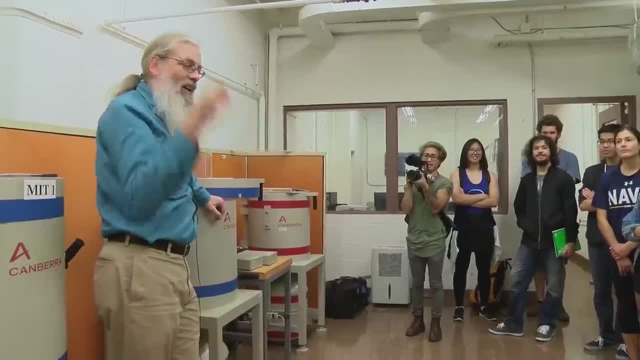 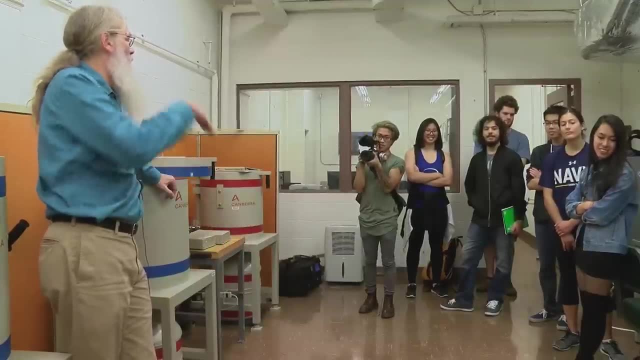 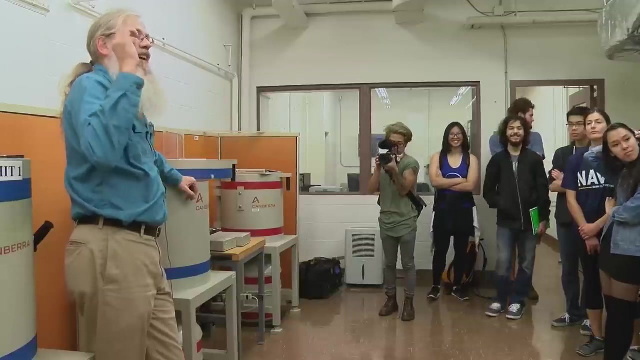 you know, i'm all about. i'm all about making mistakes. um, yeah, yeah, yeah, just be a little more gentle. we'll throw some duct tape on it and it'll be fine. um, so you're looking for potassium 40 in your bananas, correct? where else do you think we got? 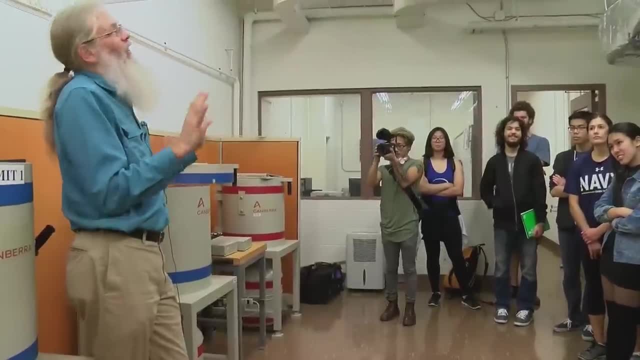 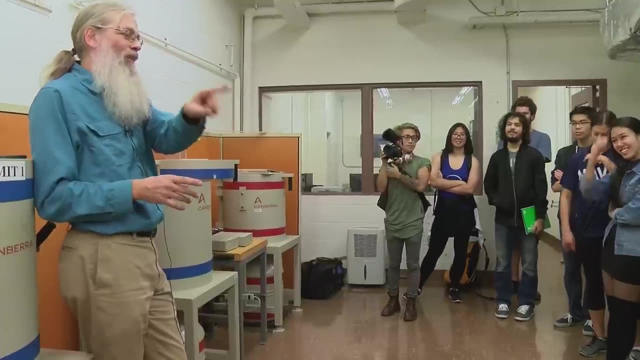 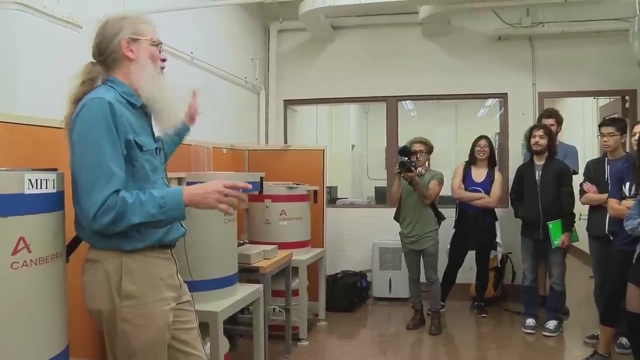 potassium 40, or do you think there's any other potassium 40 in the room? yeah, right, so that's right. when you do the banana count, we we frequently take a spectrum on this with the lead closed and we always see potassium 40.. there's potassium 40 everywhere. so after we get the count of the 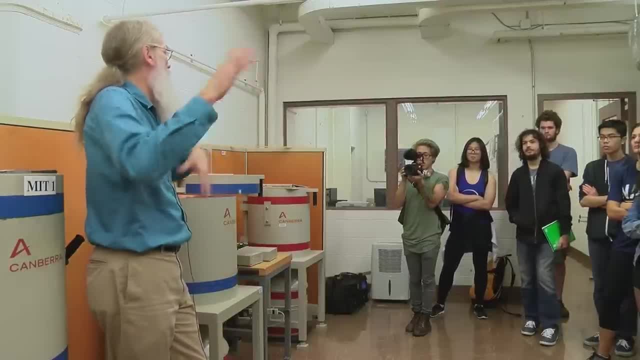 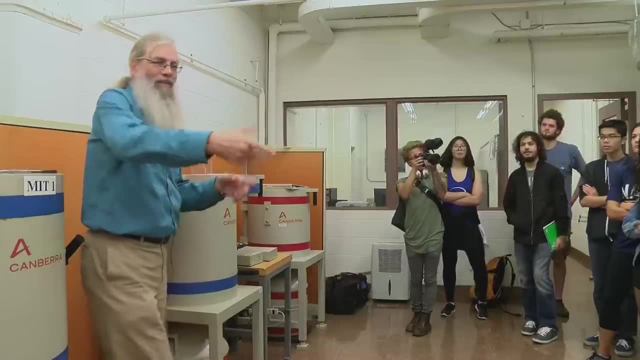 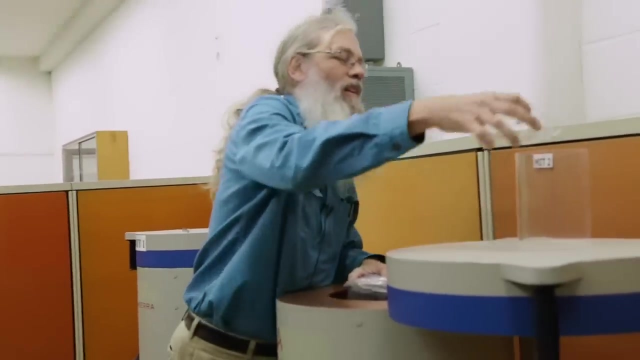 bananas. we'll take a background count. you'll want to subtract the two signals. just did that 15 minutes ago, you're so ahead of me, okay? um, i think that's all. is this going to fit now? okay, close enough? um, i've got this thing. i've got a whole bunch of little spacers, if i'm counting. 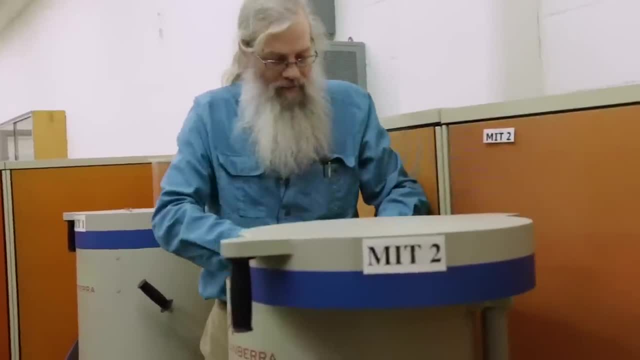 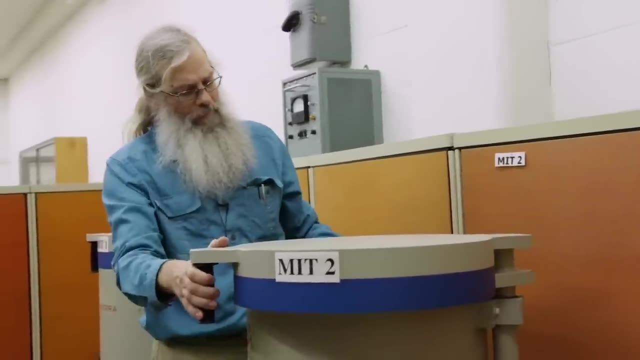 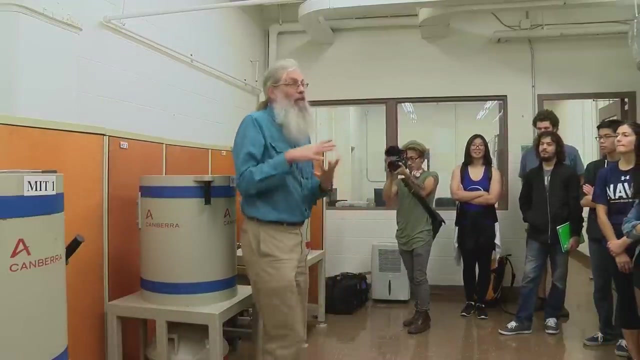 hot, and by hot i mean radioactive hot. um, i, like you know, i'll space it out a little further. no, that's fine, we just got to close the lid. okay and okay. um, if i've got something that's very radioactive, i'll just space it out away from the detector. um, if you've got something, 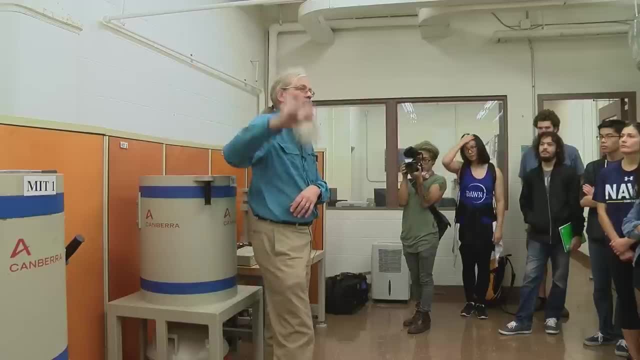 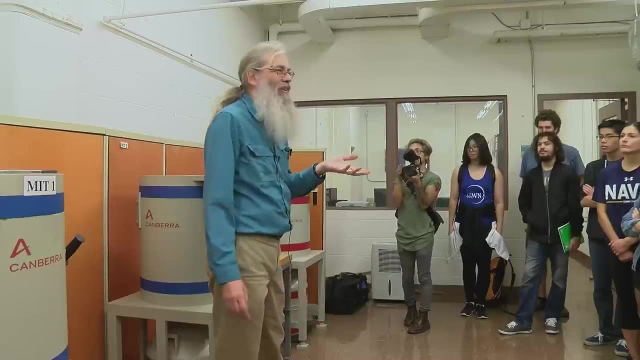 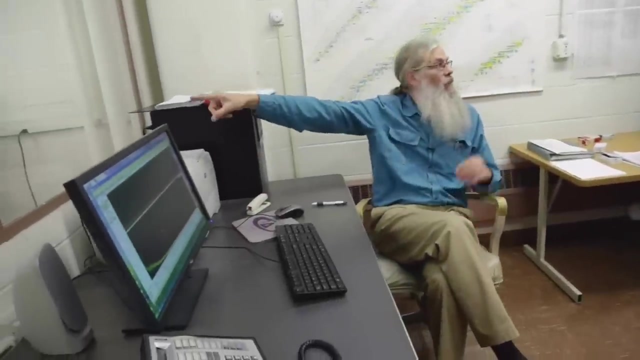 that's really hot, um, it just kind of swamps out the electronics. we do just go over solid angle too today. there you go, um. is there anything else i want to say in here? no, let's move this way. this is the spectrum i'm collecting on mit one. uh, right now, i don't know how long has that been? 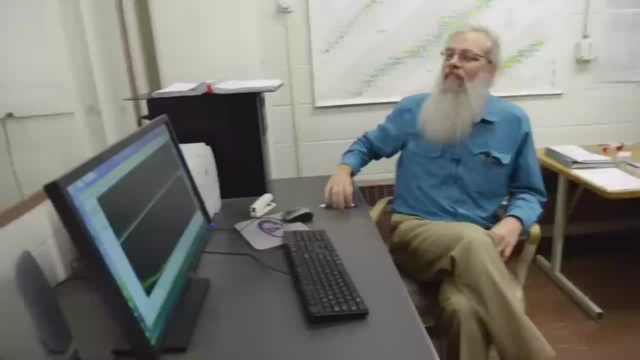 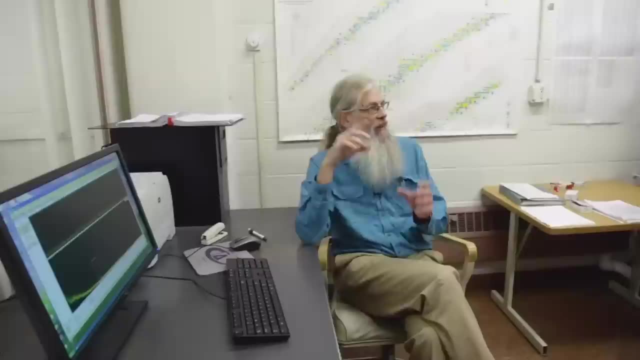 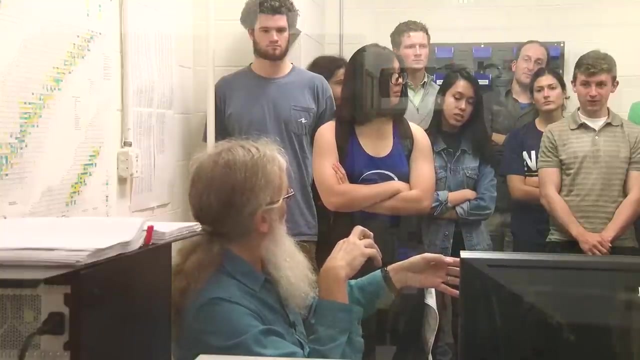 going, uh, half a day and less than that um anyway. so this is a sample of quartz that was irradiated um next to the reactor. you guys are going to do shorts in like a month. did you bring your samples? we're getting them, okay, good, anyway, this is a sample of 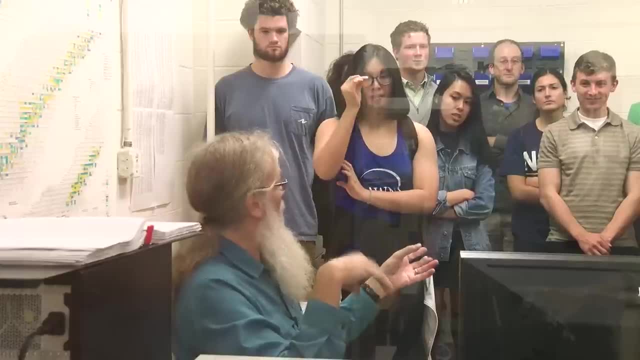 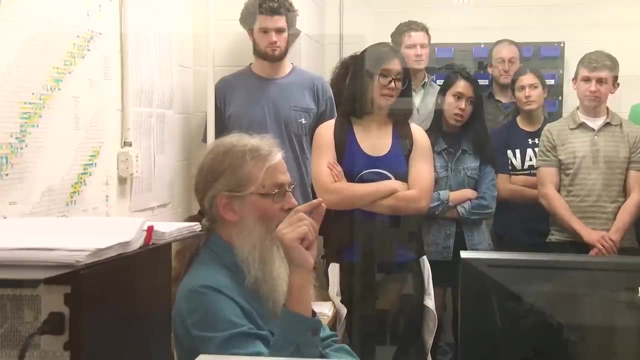 quartz that was irradiated in the same spot. you guys are going to do your radiation um sort of in the graphite region of the reactor. the reason we're running it is the people who are looking at this quartz want to run it for 80 hours and we'd like to know if there are. 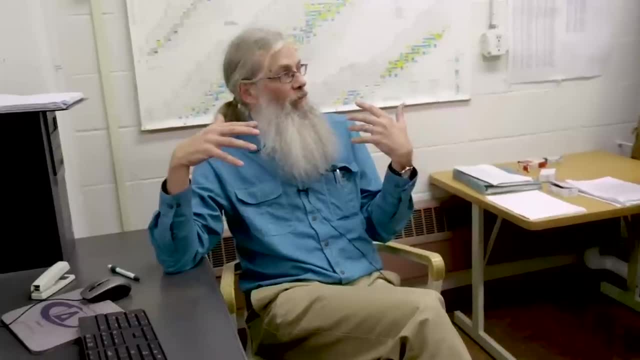 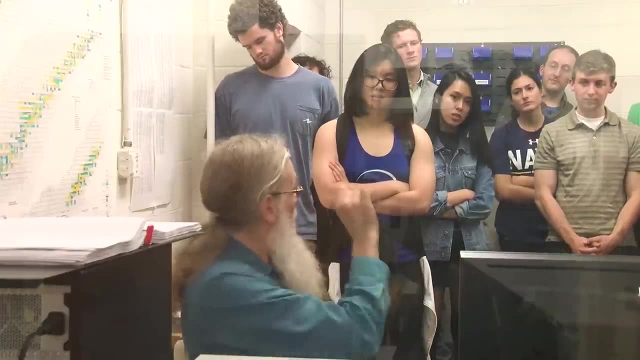 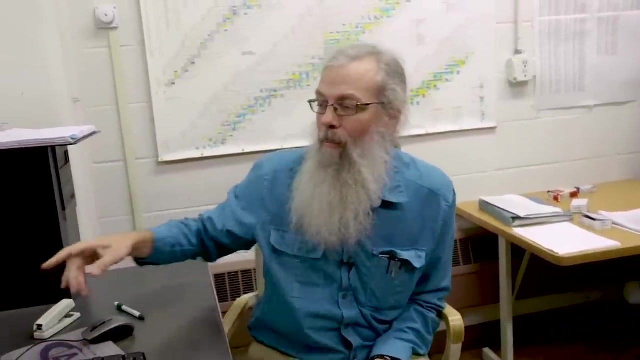 any impurities in it. that'll cause grief, meaning a lot of activity when it comes out. so we run it for a short period. i think this ran six hours, um, and it's just a little tiny piece, um, and so i can look at the gamma spectrum coming out of this so you can see there's a whole mess of peaks in here. 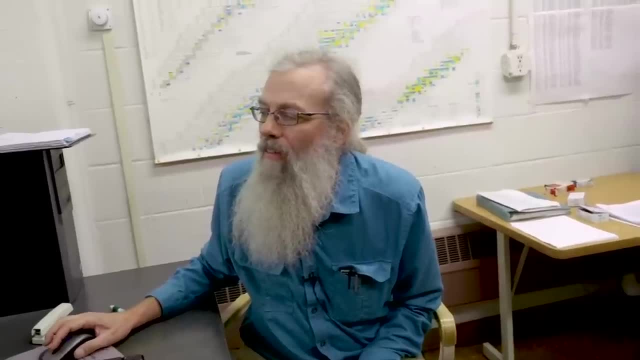 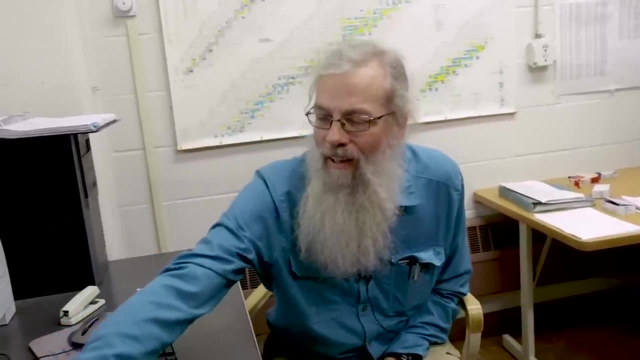 um, this one, yeah, see that, you see that lovely little peak right there. can you all see that you're not? yeah, okay, so that's the full spectrum, that's the peak, that's a tungsten 187 peak. so i did put up one little thing right behind. you see, that's the 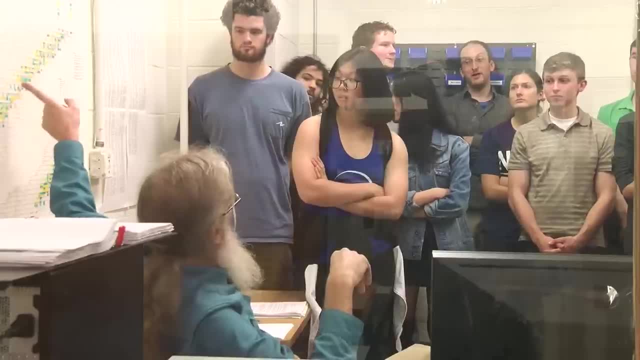 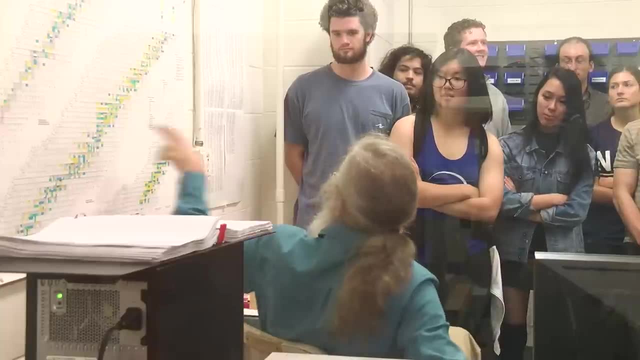 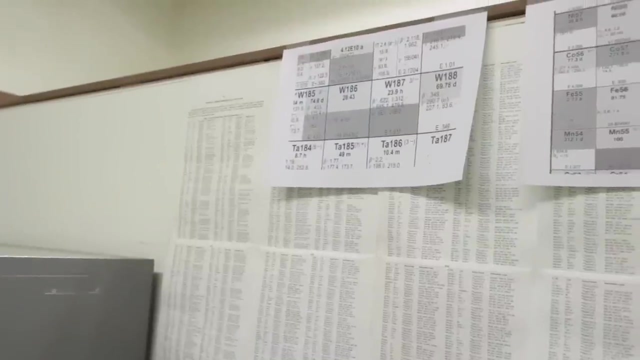 okay, have you all seen the chart of the nuclides? this thing every day, every day. good, i've got one of these on every wall in every lab and office and a little handbook. um yeah, so the tungsten, uh 186 activates into tungsten 187.. so i mean, if you've looked at the chart of the 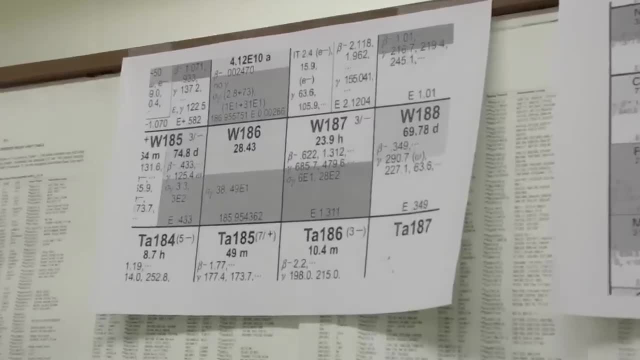 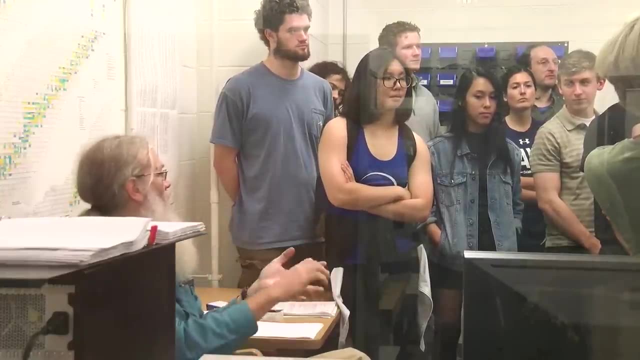 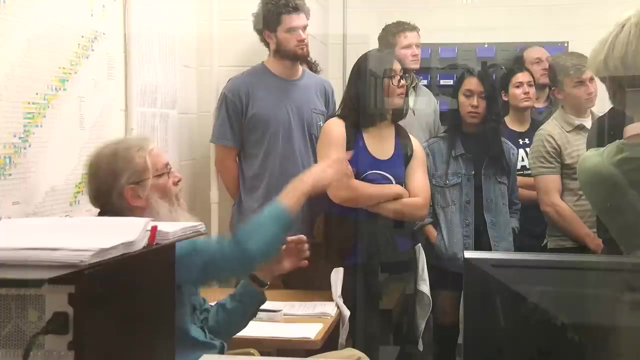 nuclides. you can tell that there's all the sort of parameters you would need to calculate. you know how much activation you'd get, based on neutron flux and time. and across the 28.43- that's the abundance of that isotope- you can see the sigma gamma 38, that's the 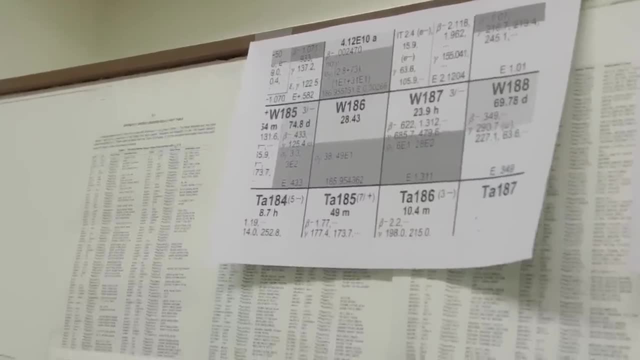 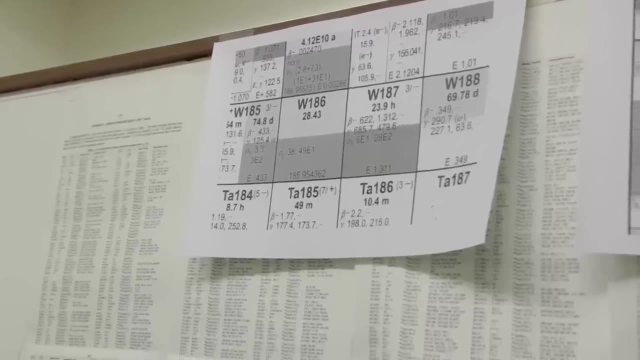 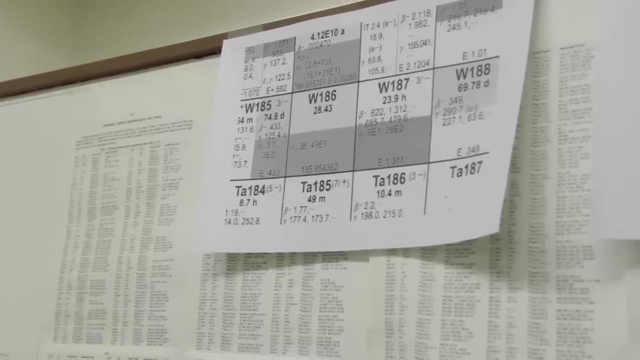 cross section for thermal neutrons. um, and so that's how likely you'll get, from 186 to 187. 187, that's the half-life, 23.9 hours. so with all of that, oh, and underneath the uh 23.9, you've got uh. 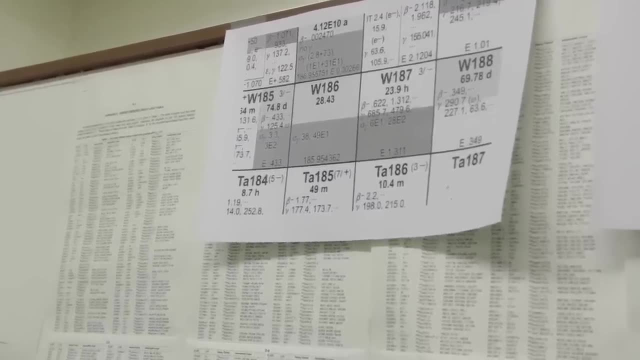 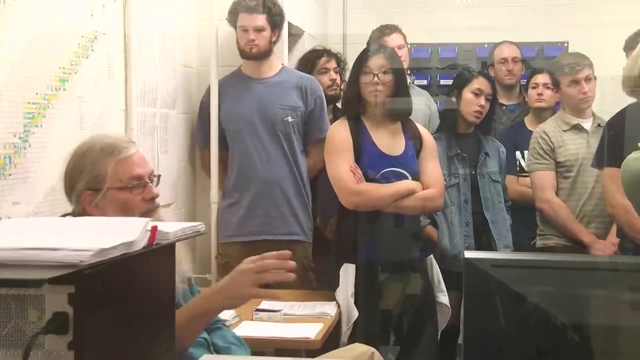 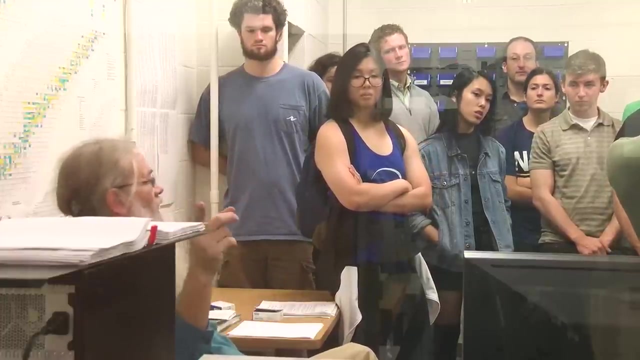 what the gammas are: 685, 479, it's got a whole mess of gamma. so that's a bunch of the gammas in here from that so you could knowing how big that peak is, what the efficiency of the detector is for collecting that peak in that geometry, the half-life, the cross set, you know that whole mess of parameters. 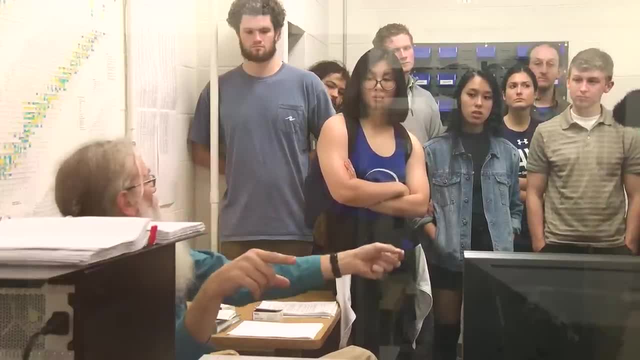 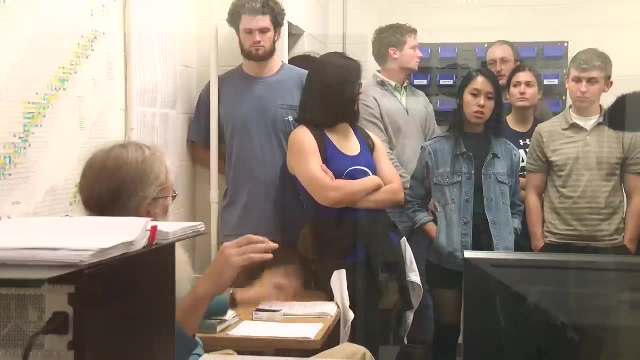 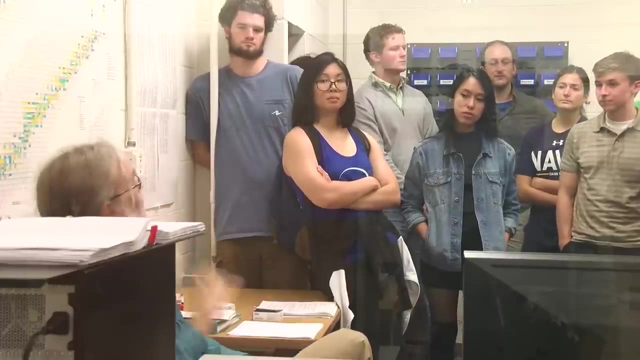 you could back calculate how much tungsten is in the sample. so that's kind of how naa works, which i assume you've explained we have. okay. actually, the whole idea behind doing those short naa activations is these guys are going to calculate what's in their samples. there you go. once we get the data, um, but that's not how. 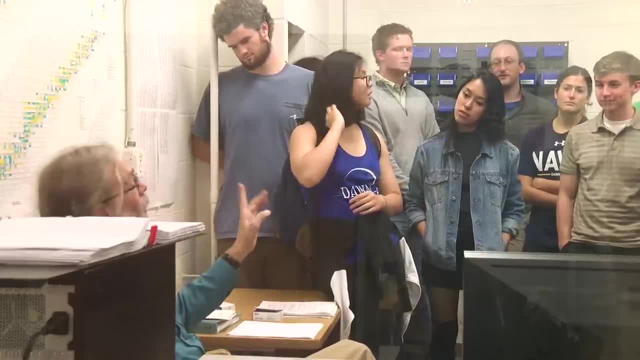 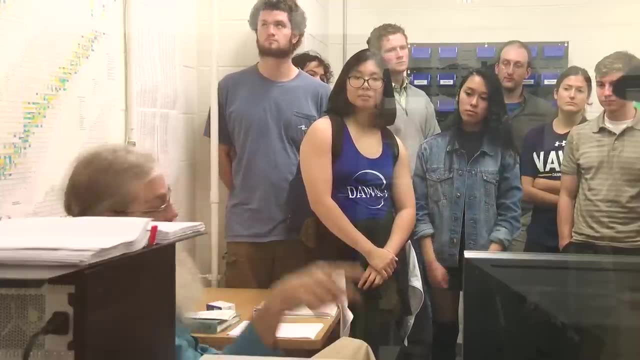 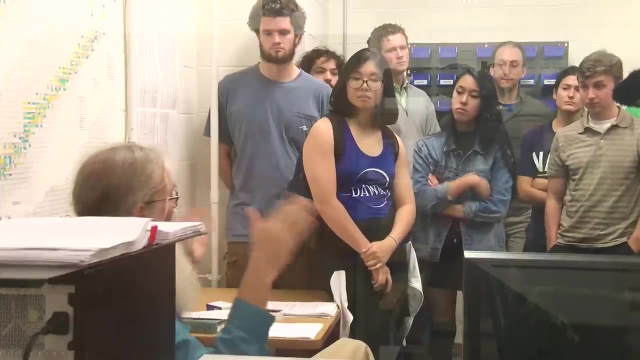 i do naa, so we're doing a simplified right, right, no, no, so there's. there's two things you could do. one of the things you could do is you take all those nuclear parameters and you calculate it just from the peak height. the other way, that everybody who does naa, or almost everybody who does naa is. 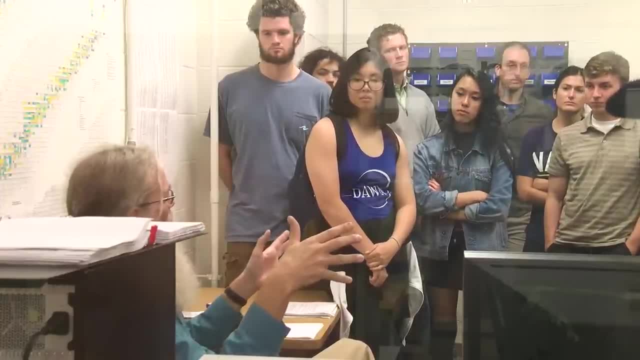 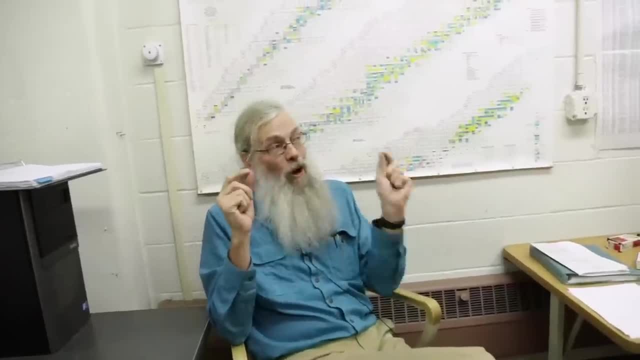 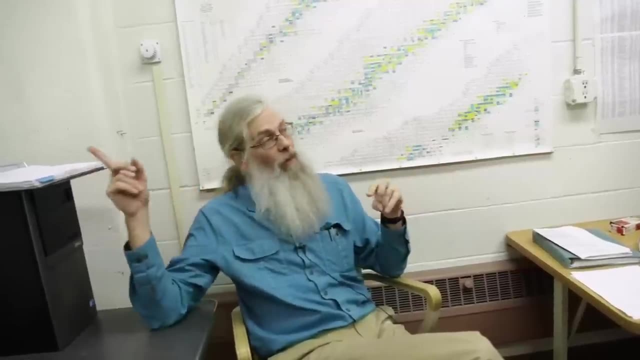 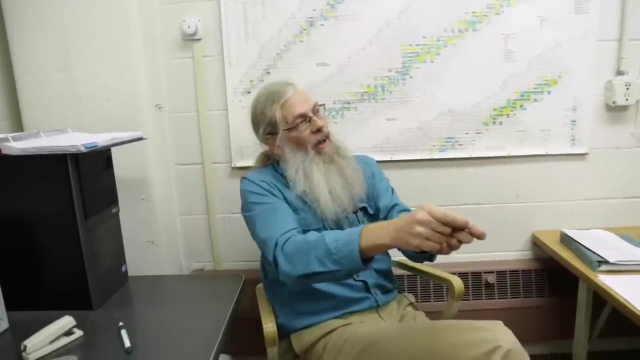 standard, which means um a material that you know how much tungsten is in it or how much a whole mess of other things are. so i run a bunch of different standards. so along with this pizza piece of quartz, i ran a standard um irradiated it. at the same time i'll count the quartz and 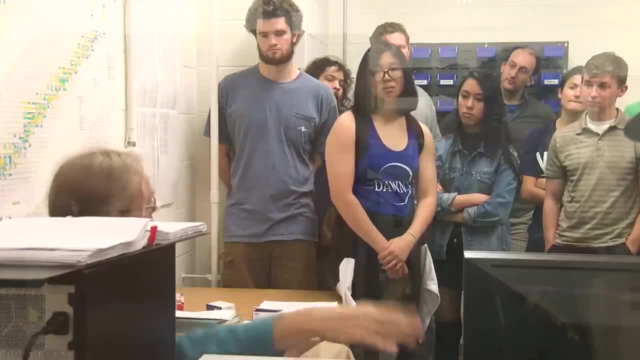 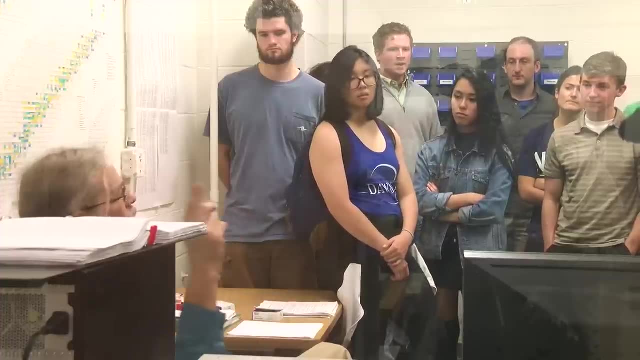 then i'll count the standard and by comparing the peak heights and doing all that stuff- the decay corrections and the weight corrections- then i calculate how much tungsten is in my sample. so i don't actually use the cross sections or the flux or any of that other stuff, all of those. 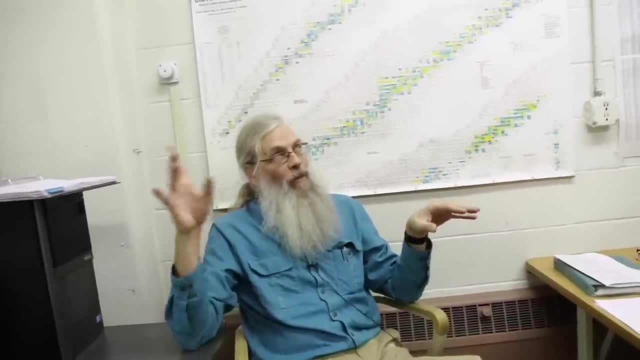 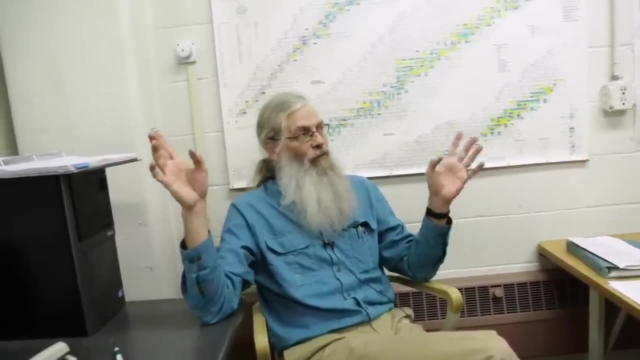 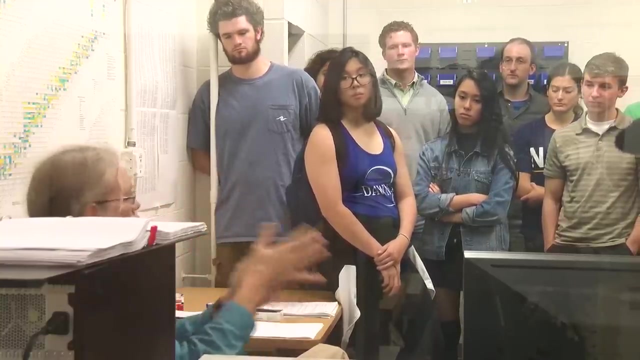 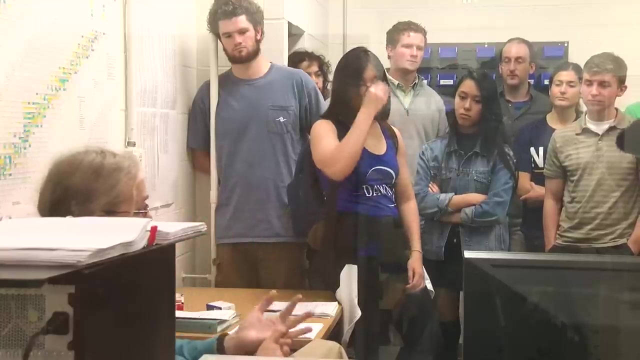 parameters disappear, notably the detector efficiency disappears out of the equation, because that's the parameter that you usually have the fuzziest idea about. and so you get, you reduce the uncertainty in your, in your concentration, by doing the sort of comparative method with a standard. uh, that all makes sense, okay, yeah, so when we run shorts, 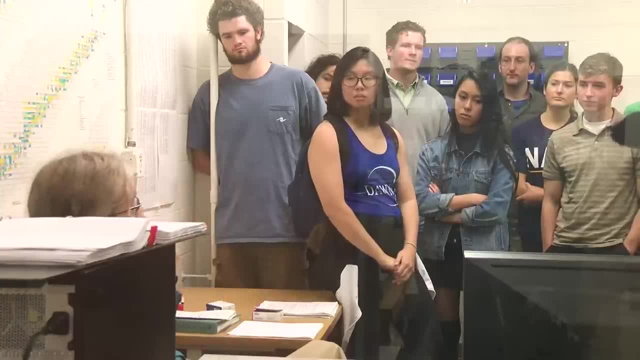 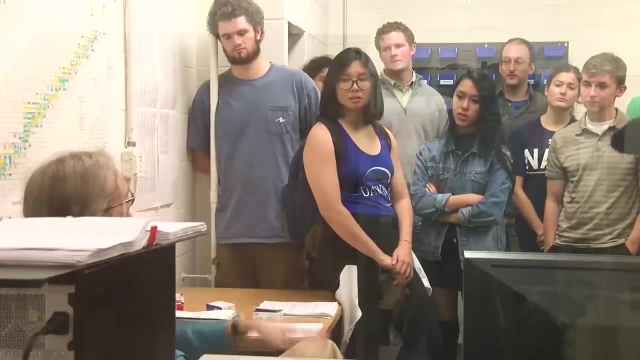 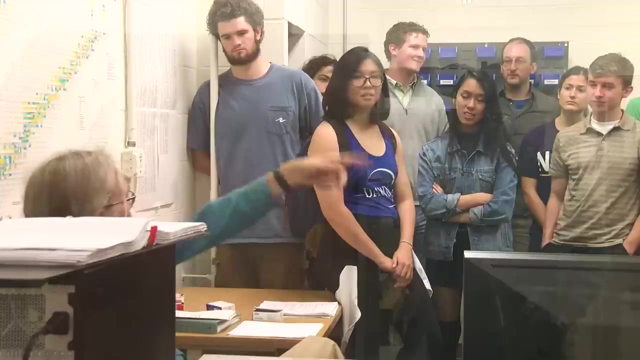 i guess in a month we'll take whatever your samples are. i've had feedback about: oh god, you don't want to run that many samples, um, but we'll figure out how many samples we'll run. oh, that's a lot of shorts in pairs, right? yeah, um, so i'll show you how the shorts get run, um. 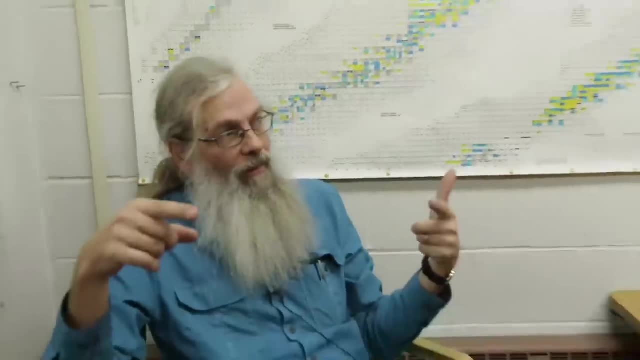 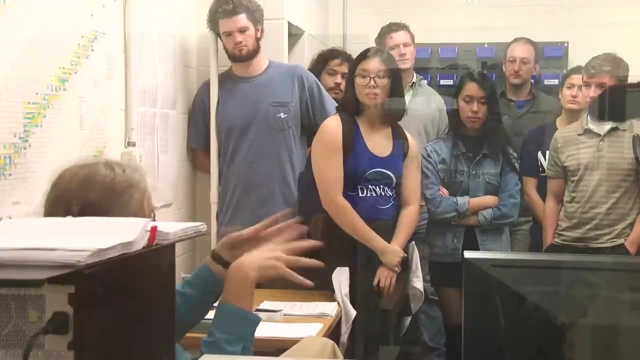 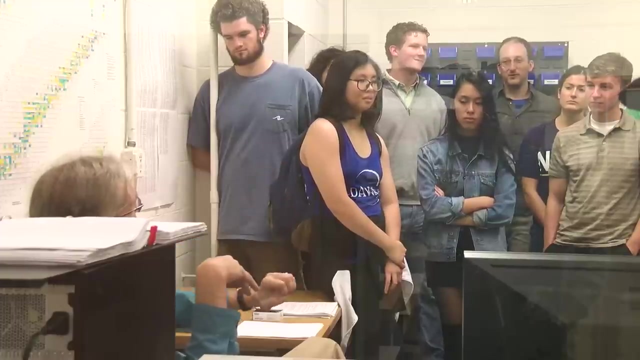 so when we run your shorts, we'll run your samples and we'll run standards, and then you can do the comparative method or, if you feel like it, you can do the other method, depending on what exercise you're going to do the other method. you don't want to do the standard method. oh, no, no, no, okay, not practical, oh, 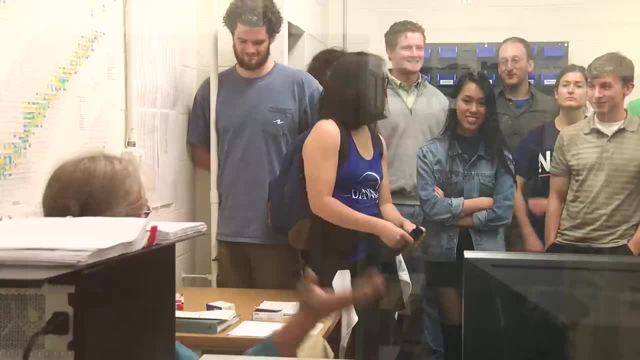 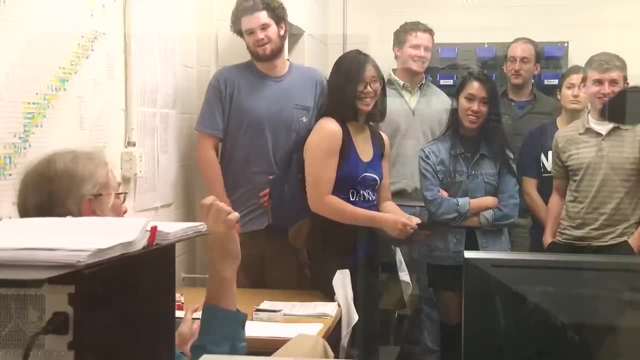 well, if the computer goes down, you can't get any data. anyway, i can do the comparative one on a envelope anyway. uh, Okay, well, we'll run standards or not, depending on how you guys are feeling. yeah, so that's that. oh right, so let's count your bananas. 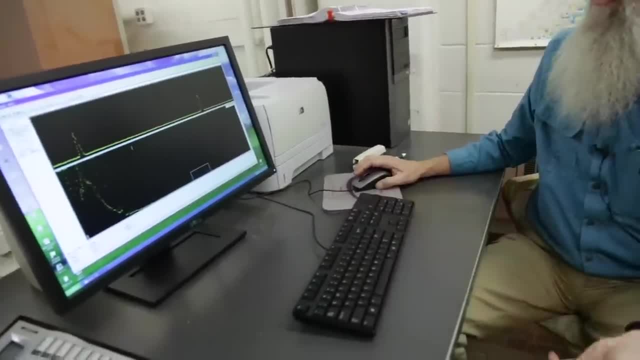 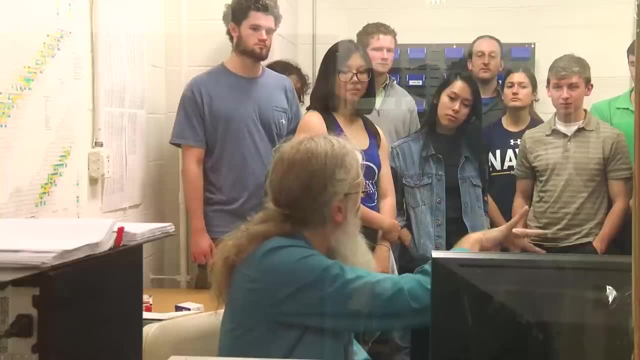 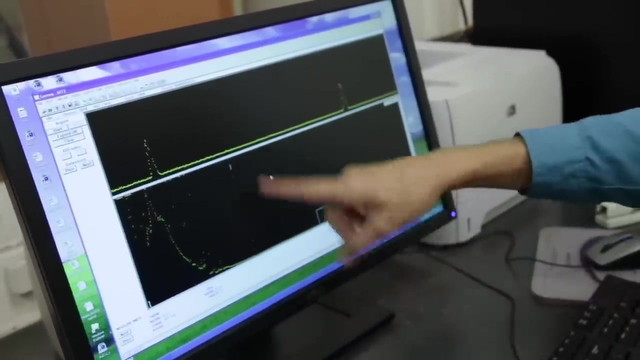 okay, so this is detector two. we did an energy calibration earlier today, um so yeah, actually these are. i've got a couple of little button sources. have you seen the button sources? yeah, so that's just a couple of cobalt av 60 lines and a cesium 137 line down Indian. 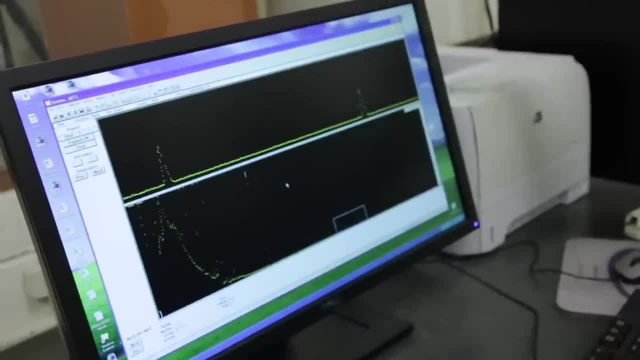 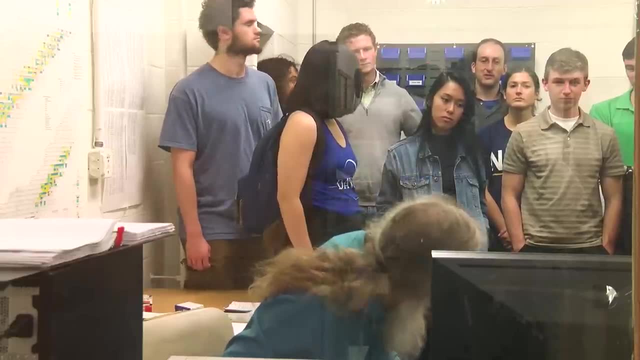 here and i know where those energies are. so that's just gets used to calibrate the detectors. we were playing around with one of those cobalt 60 buttons today in class. there you go. we mentioned the two gams per disintegration. there they are. there they are. they're kind of small there because 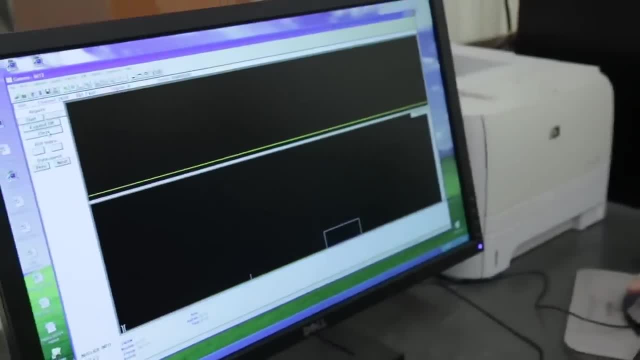 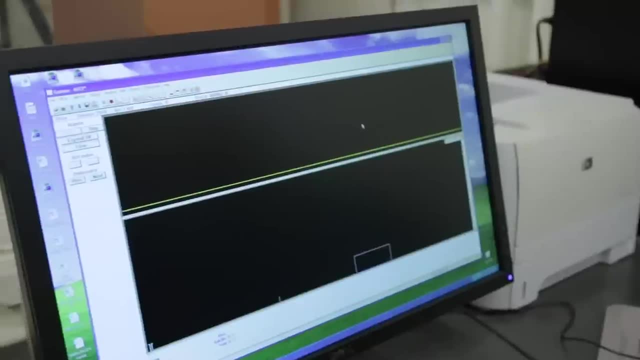 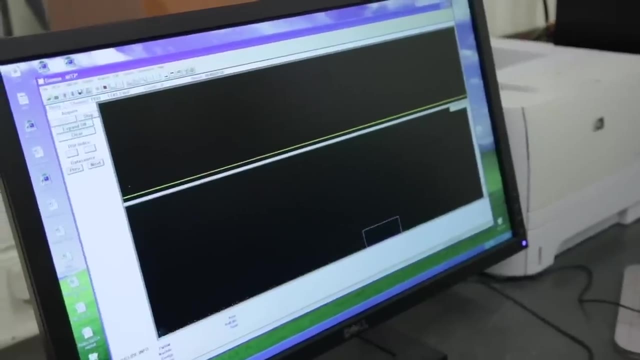 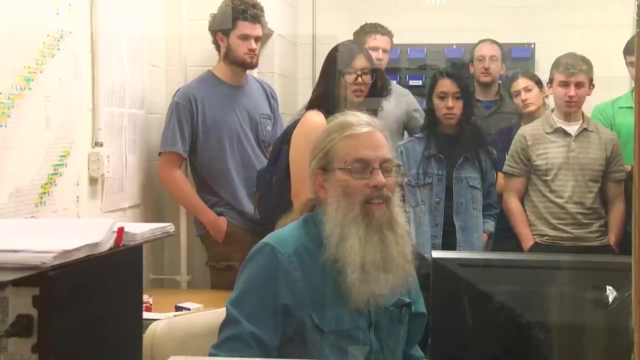 my buttons are probably 30 years old. oh, i got some fresh ones, yeah, so, anyway. so we cleared that out, um, and we just hit start and we're not going to see anything for a while. where are we out here? 14.. anyway, your banana peak will end up out in here. yeah, so that's. it'll take a while, we're. 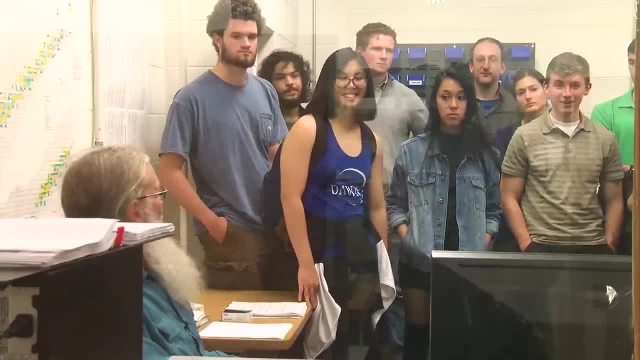 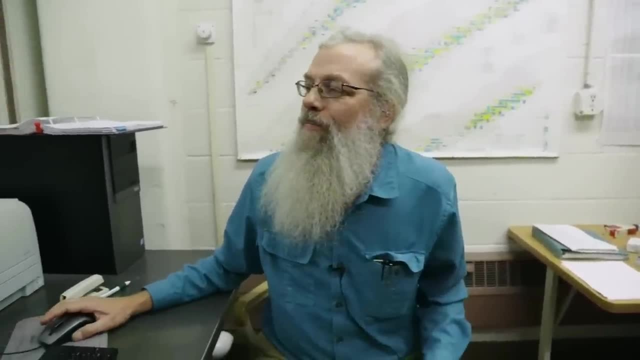 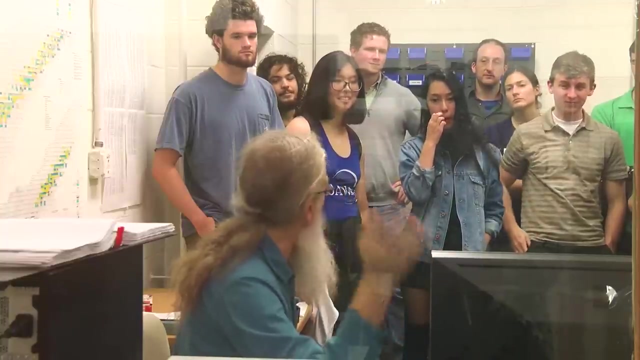 gonna let this count till tuesday because- why not? i don't feel like coming in over the weekend and turning it off, so, um, so yeah. so i mean this is just picking up all the gammas coming out of the bananas and everything else that happens to get through the land and 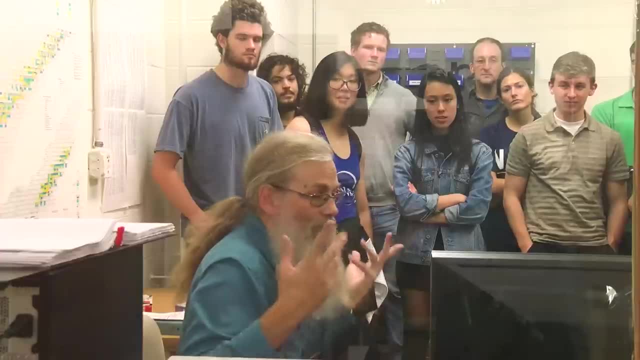 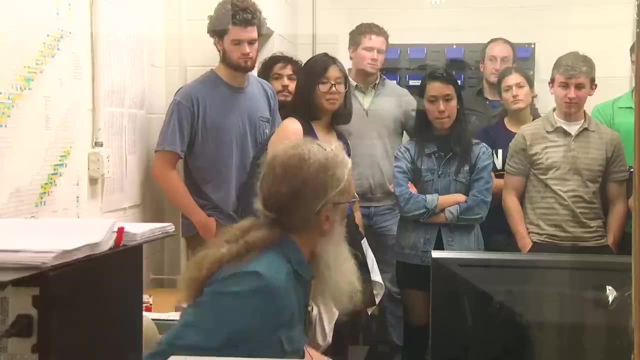 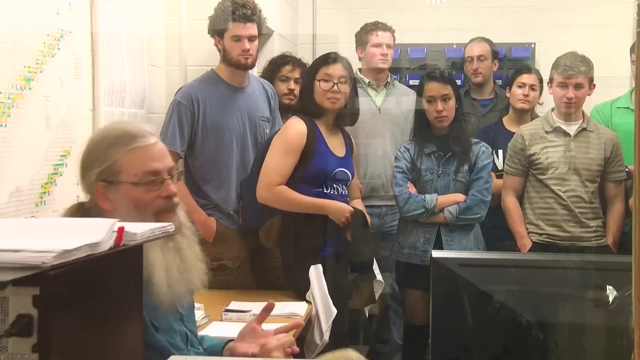 all the contamination on the inside of that um, and we just let it count and then you guys can calculate how much potassium 40 is in your ashes. uh, you'll need to do the background subtraction. um, i will give you. uh, yeah, i've got. we collect background spectra, you know, once a month or so. 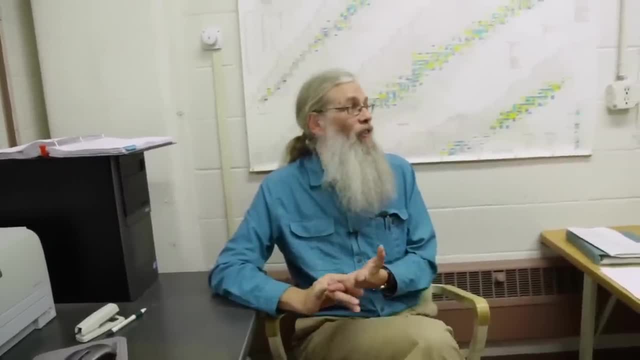 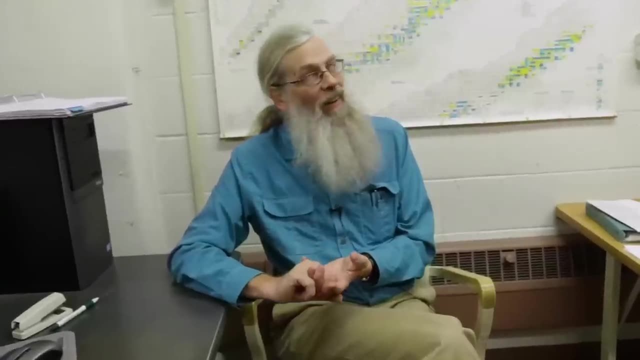 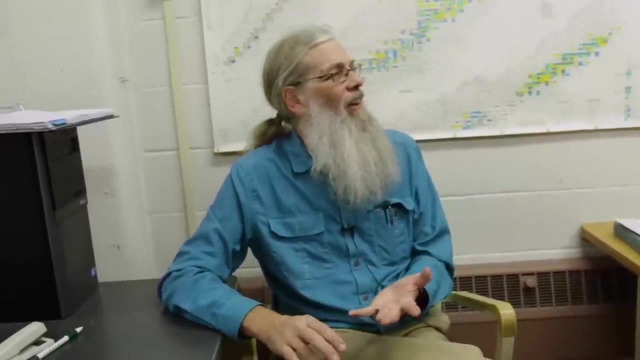 so i'll give you a background spectra. i will provide the efficiency for this geometry, which is pretty poorly defined, because i've got a program that'll do that and i can't give you the program and it's a pain in the neck to run. anyway, if we've got a really well-defined geometry, that's not a big bag. 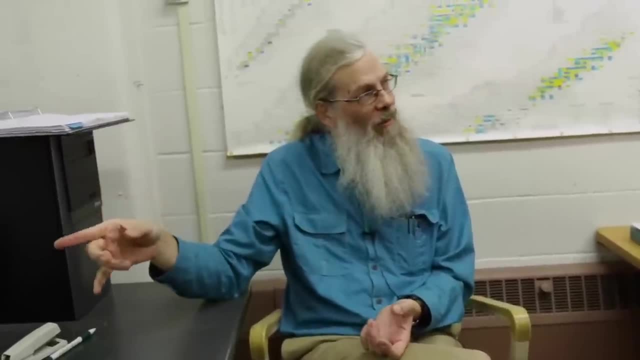 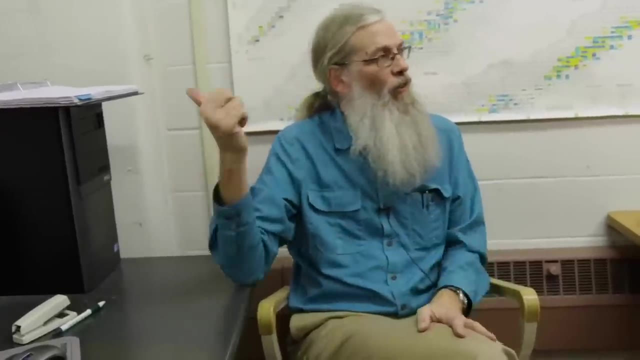 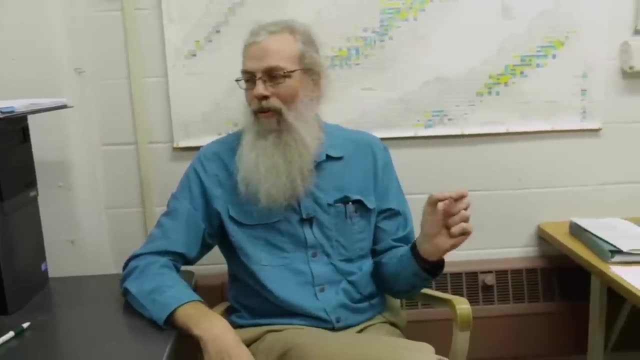 usually i try to count sort of point sources. so i've got an efficiency standard that i can use that. i know what the disintegrations in that are at a lot of energies and i use that to do an efficiency calibration usually. but i don't have an efficiency standard. that's that big um, it's just a point source um. 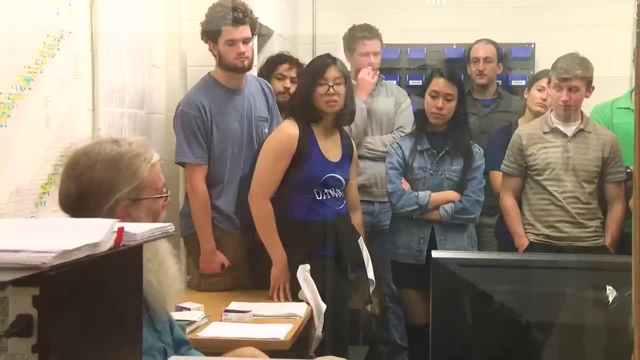 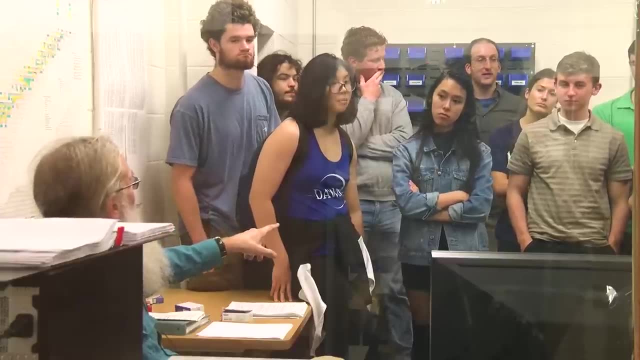 and i think that's the practical naa. from this end that all makes sense. i want you guys to not him to nod. yeah, i don't have any questions for mike on what you just heard. well time, because we were just talking about this stuff all week. good deal for neutron activation- um, that's kind of the. 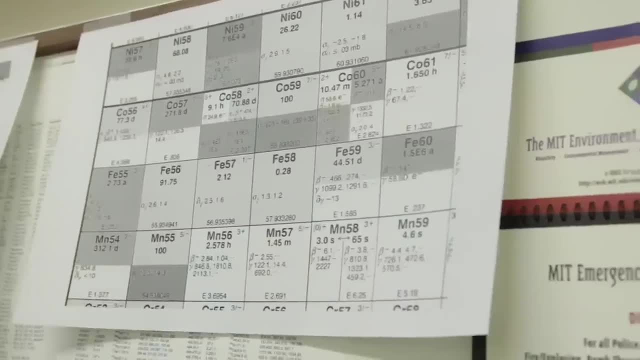 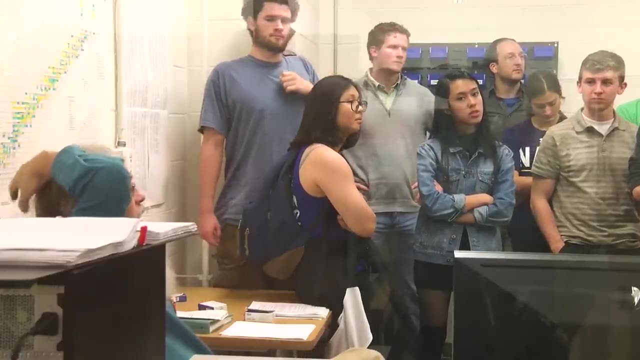 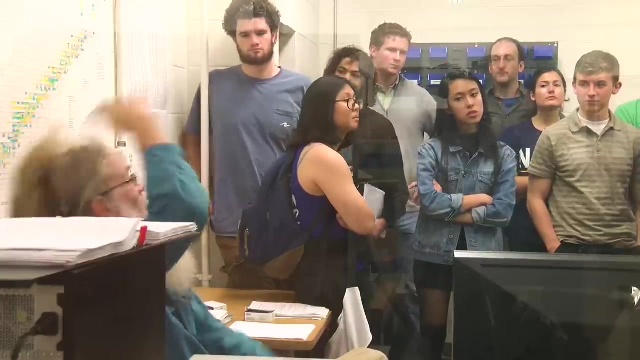 um, real common part of the chart. so there's the manganese, iron, cobalt, nickel- one of the things that you- what you like usually when you're doing naa- is you want a nice thermal neutron spectrum. you know what thermal neutron spectrum means, real slow neutrons, and they'll just give you. 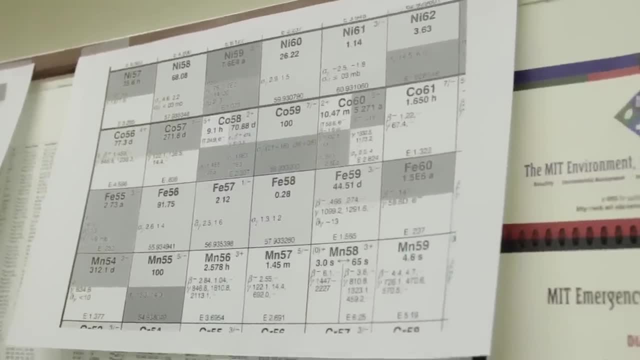 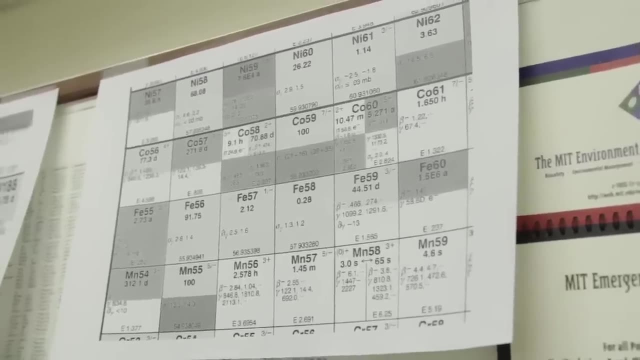 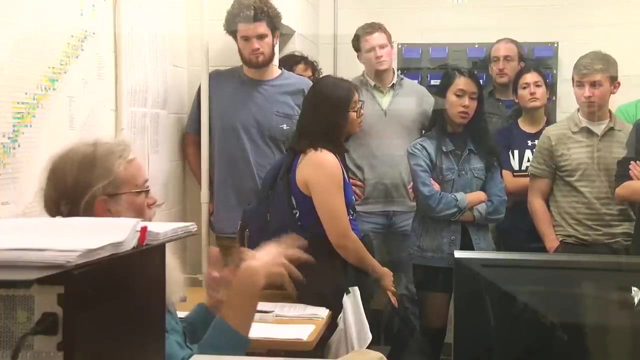 sort of an n gamma reaction. so on that chart, iron 58, iron 59, that's a nice you know n gamma reaction and that's the one i use to analyze for iron. if you're near the reactor you're also getting some fast neutrons which can give you an np. reaction. so if you're looking on the chart there, cobalt 59 if you get an np reaction will also make the iron 59 and that's a pain in the neck because then? because if you've got iron you've always got a little cobalt floating around. you maybe need to do a correction. 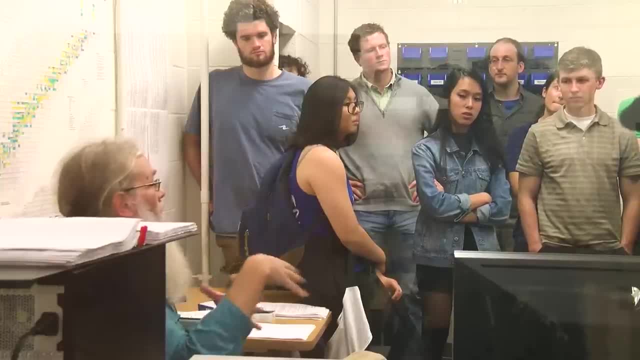 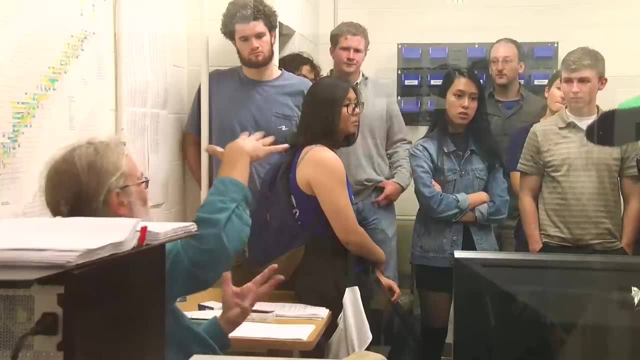 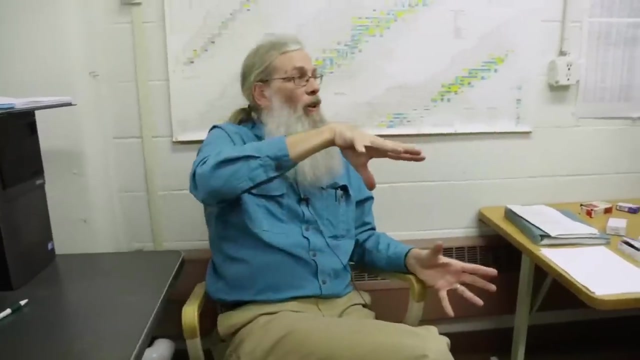 so, in practical terms, when you're running naa, you really want to have, you want to avoid having all these fast reactions? um, there's usually an energy threshold for the fast reactions, like one mbpv or so. it's not familiar from the q equation. yeah, okay, right, um, the place where we do the irradiations, 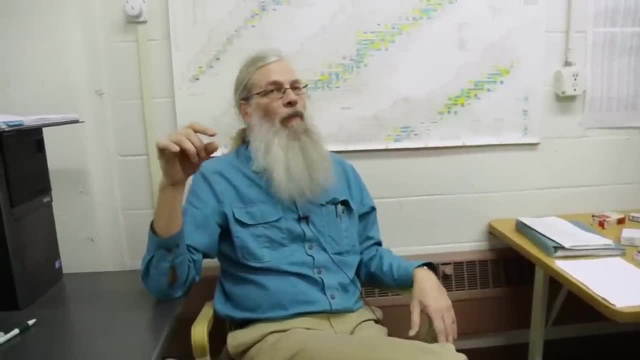 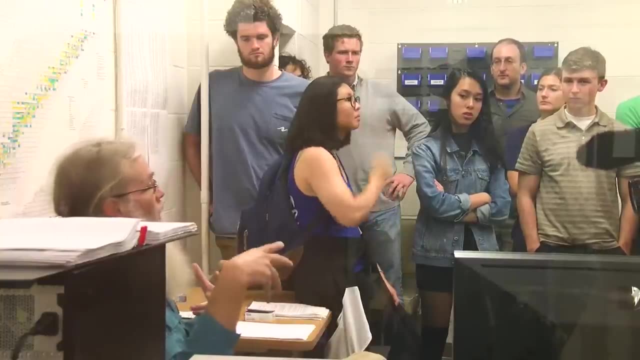 is very thermal, got a very low fast spectrum so i don't usually have to worry about that. there's a couple of times i actually use the fast np reaction if i want to measure nickel. you can see nickel 58, an np reaction, to get you cobalt 58. 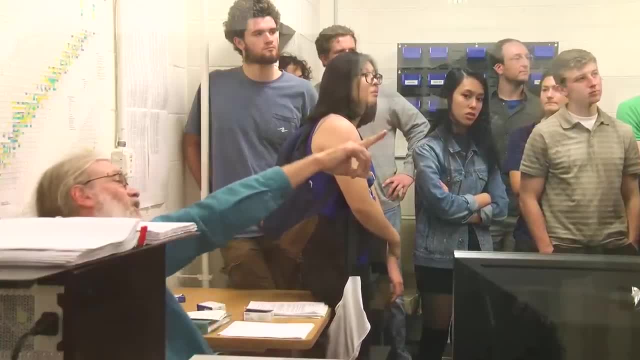 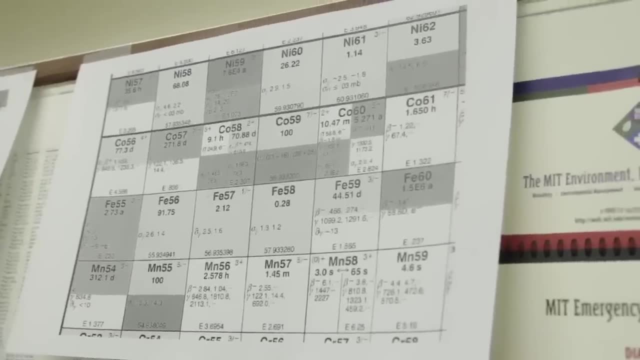 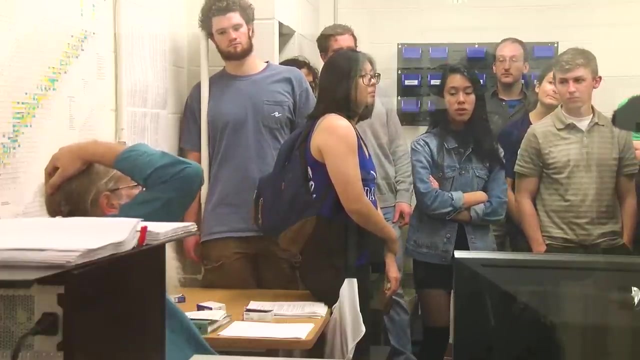 and since there's not a good reaction in gamma from cobalt 57, cobalt 57 isn't around usually. so that's how i measure nickel, using an np reaction um, and i need to put the rabbits in to where i've got a fast flux in the reactor, which i got a couple of spots for that i try not to have to. 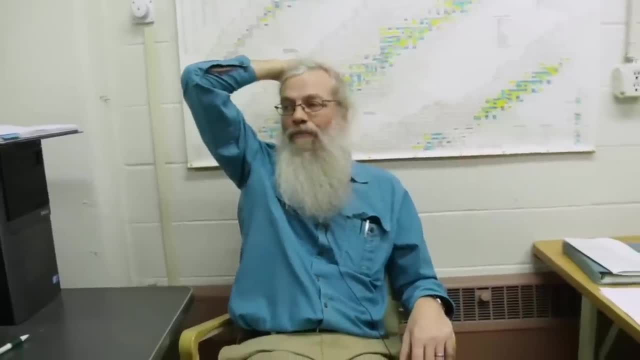 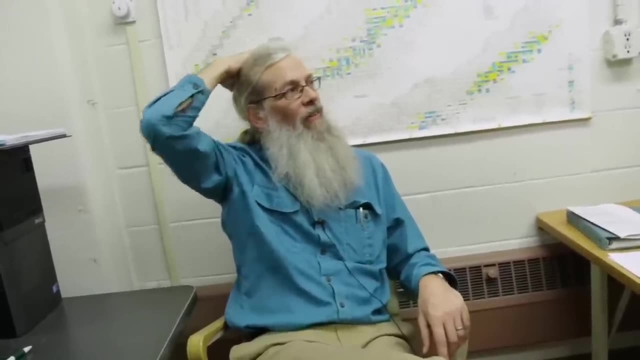 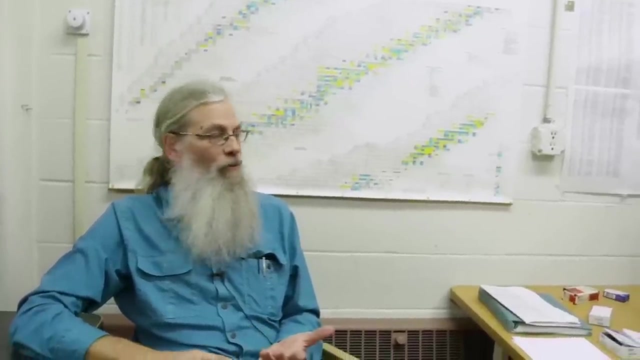 because it's pain in the neck, but sometimes people want it. on nickel, um, and we talked a little about you know what we've run in here for types of samples. i mean, why don't you tell us, okay, okay, so uh, back. you know, 15, 20, 25 years ago we did a ton of environmental samples in this lab. 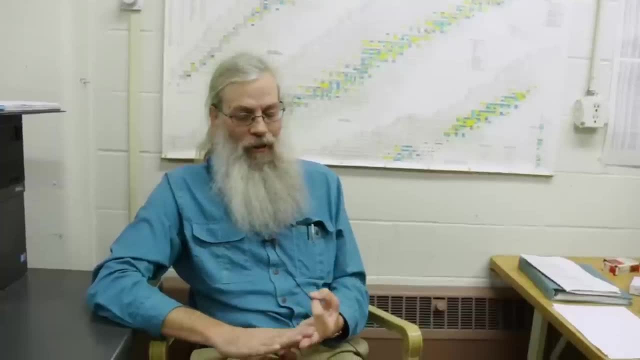 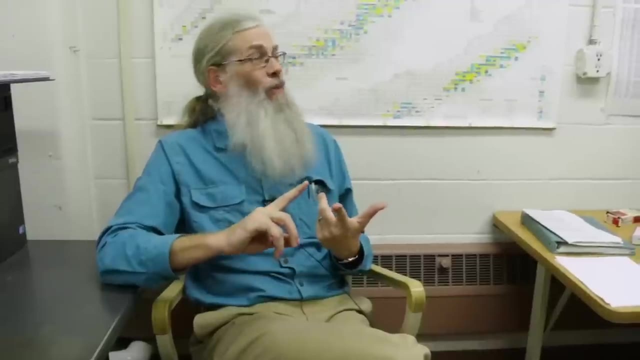 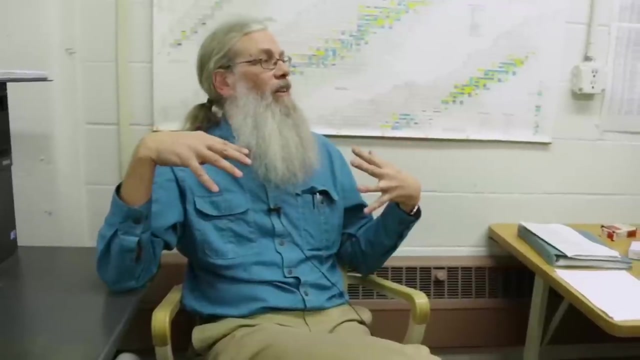 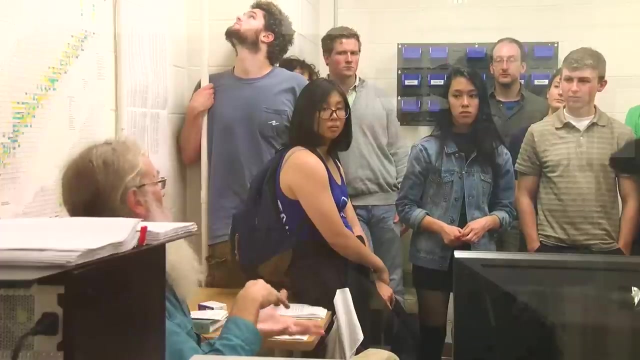 we had a whole like three grad students, myself included, who did atmospheric um particulate matter: rain, water, snow. we even did some fog collection, which is kind of fun, ice cores which are old particulate deposition, and it was all for trace elements in those kind of environmental samples, also lake sediments. other analytical methods have gotten a lot better. 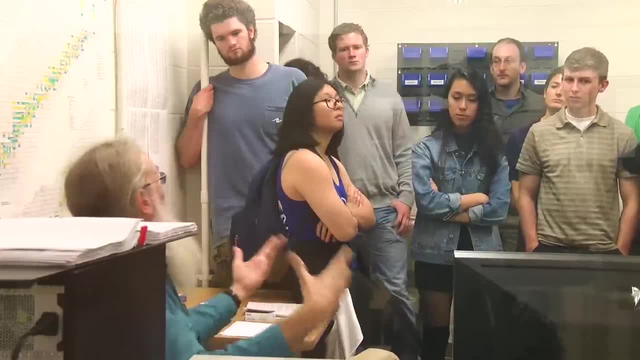 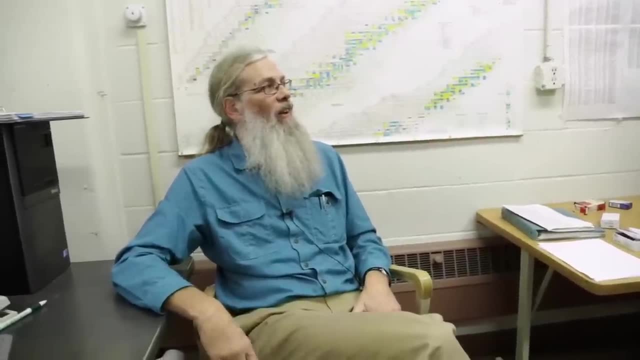 and so they've kind of caught up to naa and you don't need a reactor to run those. so the environmental side of this has kind of quieted down a lot, but it's still useful for a bunch of things, um, and so that's. you know, i do some work here now. i also work in the uh in-cord group. 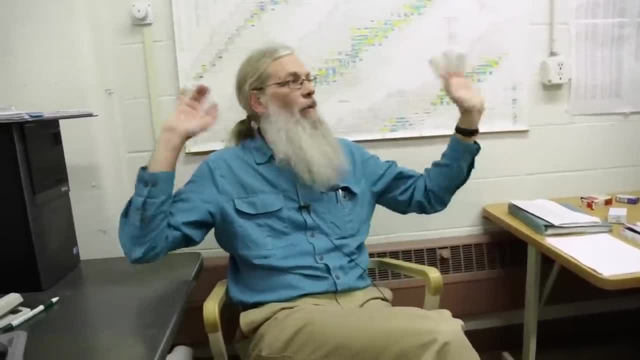 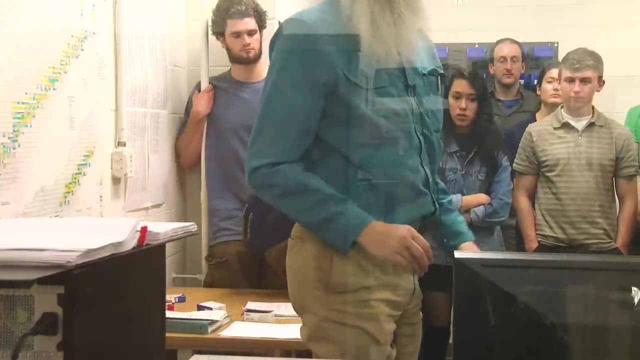 so that's a lot of my time. rather than just this, this lab, um practical things, let's go take a look at a couple other labs. you're not on wheels. you don't have a steadicam. no, okay, okay, you got a question. you've ever been asked to count. you're not on wheels. you don't have a steadicam. no, okay, you got a question. you've ever been asked to count. 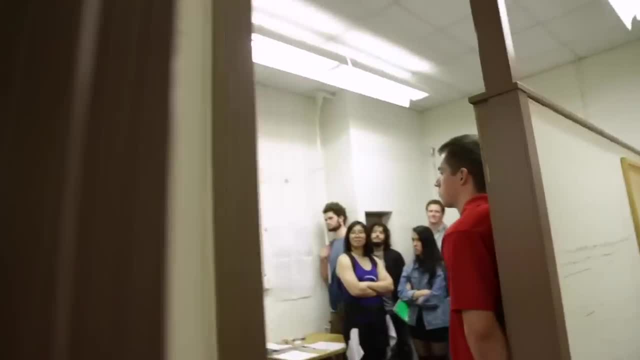 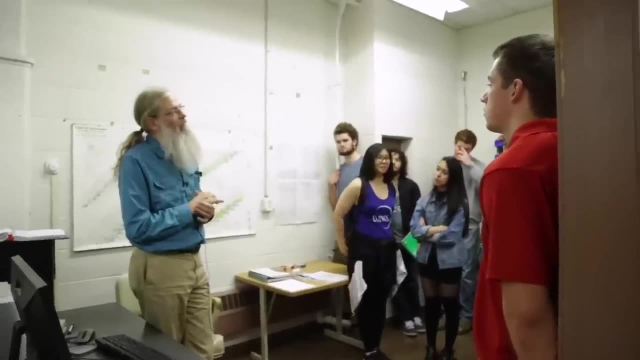 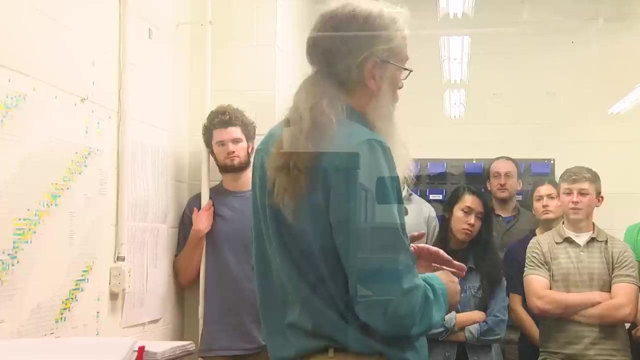 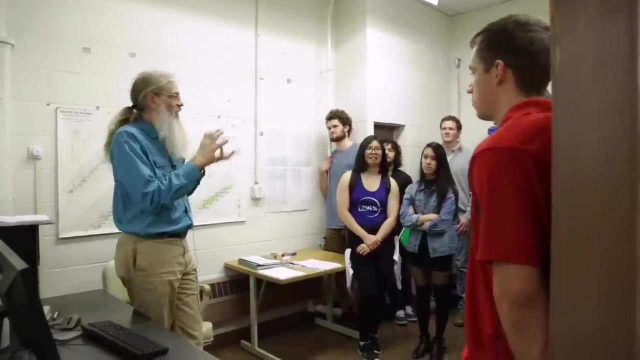 the weirdest thing i've been asked to count that's already activated or at all. okay, um, i don't know, brain tissue fish samples that we actually did the uh, fresh fish samples and you want to kind of homogenize those and we had this kind of titanium blender that you remember, the basamatic. 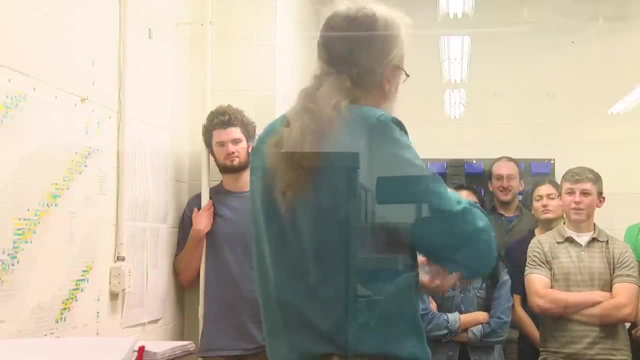 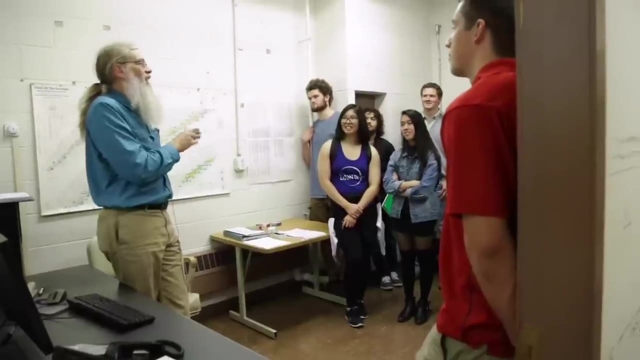 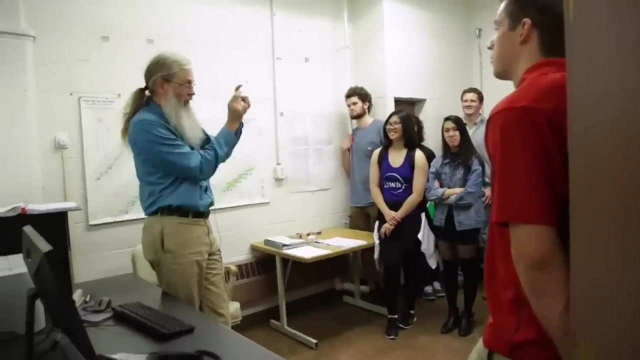 we had this titanium blender that we dropped the fish in and you completely homogenized the fish and then you took a little sample of it and freeze, dried it and then analyzed it for mercury. um, yeah, right, because i mean you guys saw, the rabbits are only this big and the samples i want are only that big. and so to get 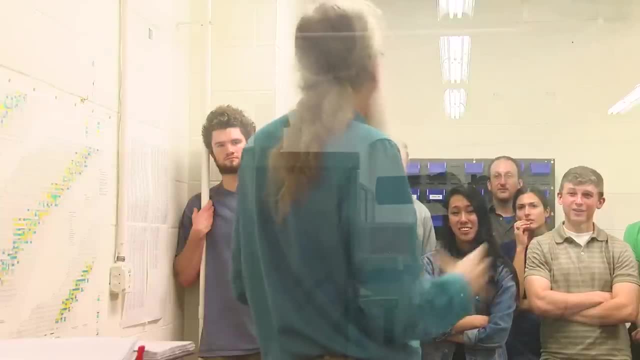 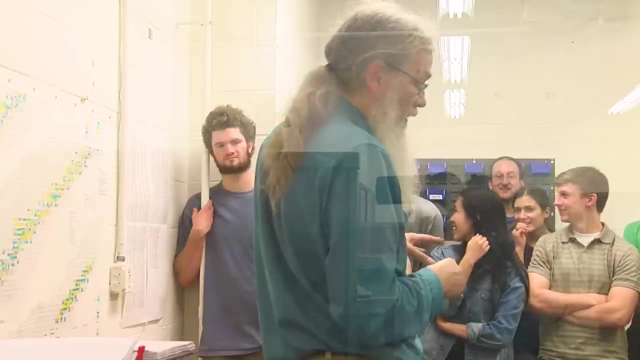 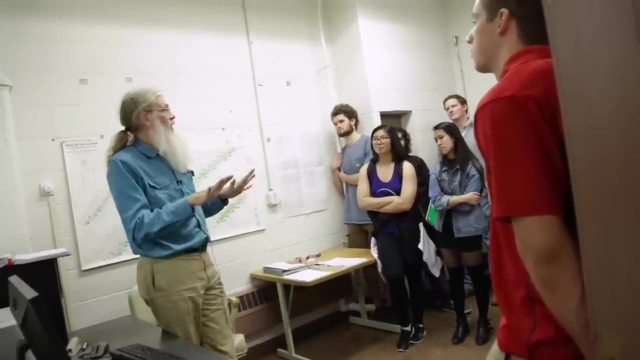 a representative fish. you want to kind of make a fish smoothie and then take a sample out of that. um, we did have a guy who came to me and was promising we were going to do this giant study using fingernails and toenails for nutritional analysis. i mean, he was working with a group. 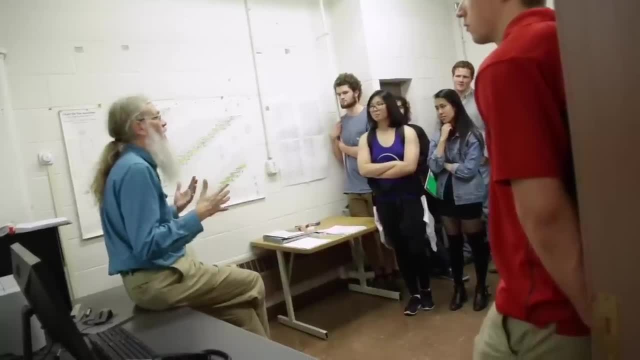 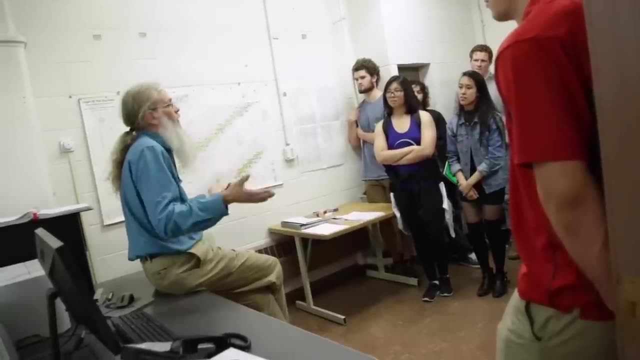 that looks at zinc deficiencies and fingernails and toenails will give you a good record of how much zinc you've had over the last you know week or month or whatever depends where you cut the nails, um, and so i was going to get you know a couple hundred. 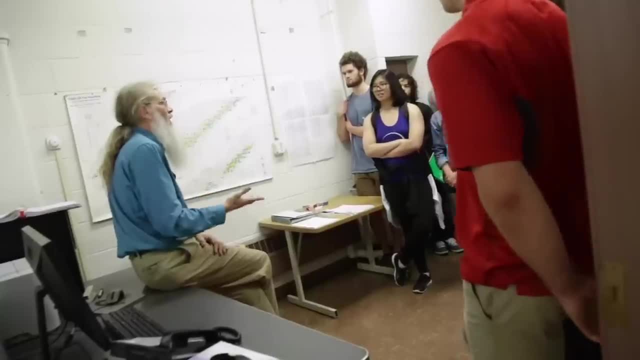 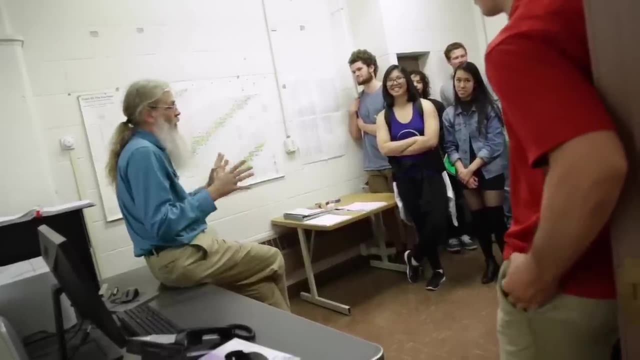 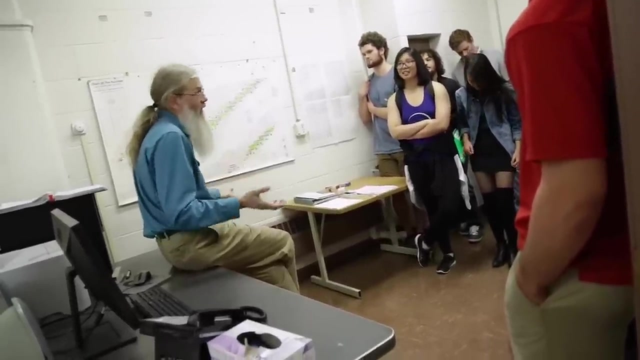 of African children's toenails? um, that didn't happen, but i did analyze my own toenails. well, if you, if you, went to somebody who was a little suspicious of you, asking for toenails is a lot easier than asking for a blood sample, because people will give up toenails. it's not a big deal. um, you all. have you ever seen the? 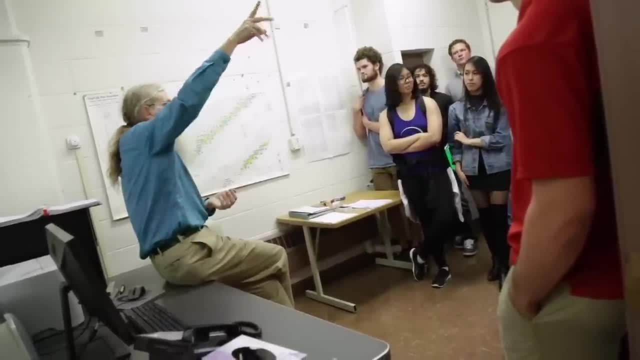 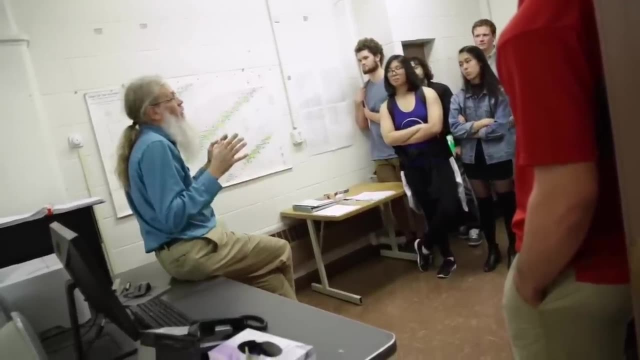 movie or read the book civil action about the supervun site in wu burn. it was a big old super on-site and wu burn had arsenic and chromium contamination. um, there used to be a lab- i forget which building it was in- that did a ton of research there. 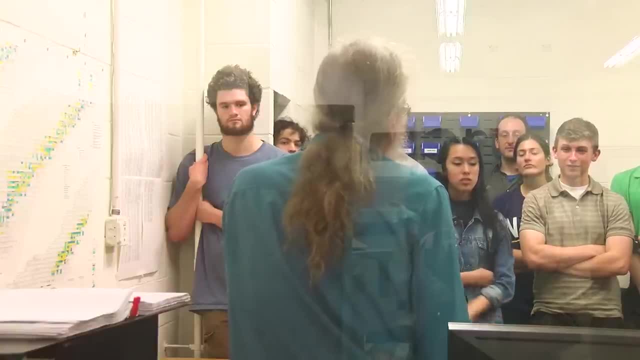 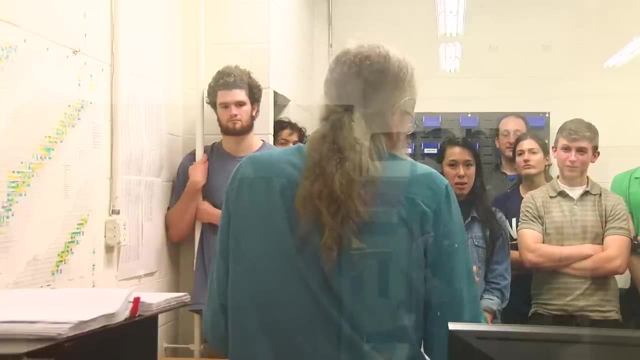 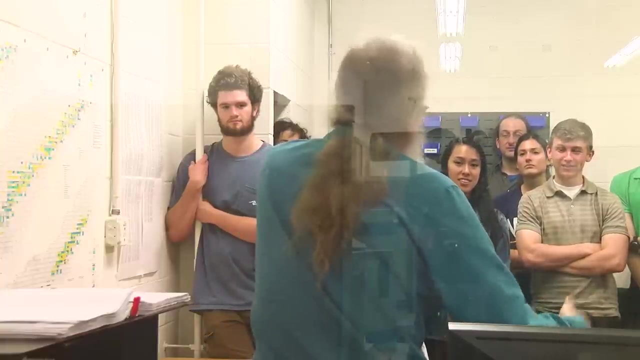 one of the things we did in this lab was we collected baby hair samples from people's scrap books. so we had baby hair going back 50, 60 years dated, because everybody knew how old their kid was and they knew. and we analyzed the hair samples for arsenic and chromium and then we plotted out. 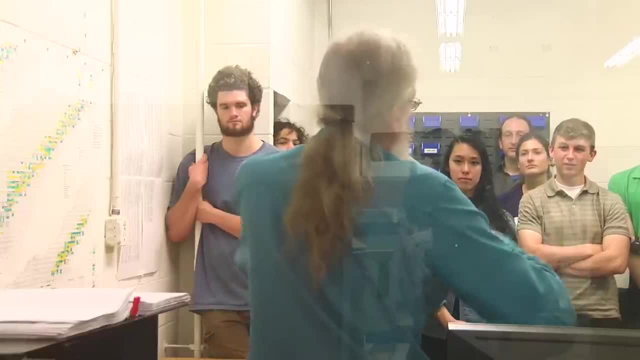 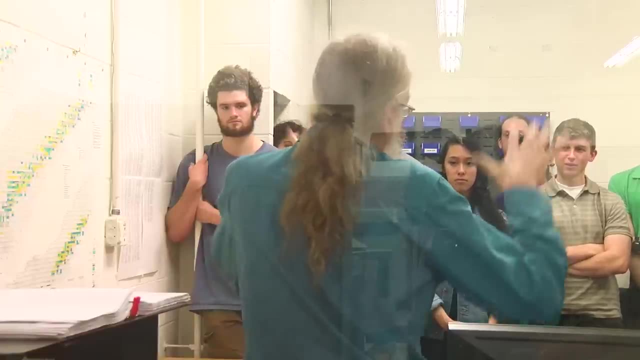 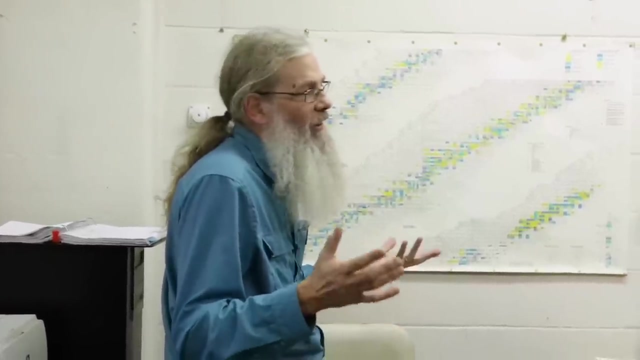 where they were when the sample was taken and how close they were to some contaminated wells. and because we did a fairly short irradiation, after a while the activities died down, we gave the samples back and so that was, and we found that it didn't correlate with the well water or 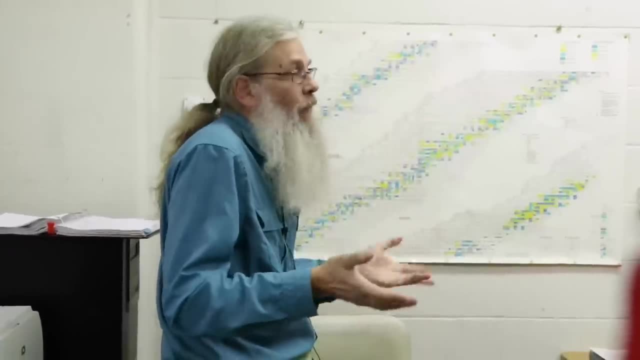 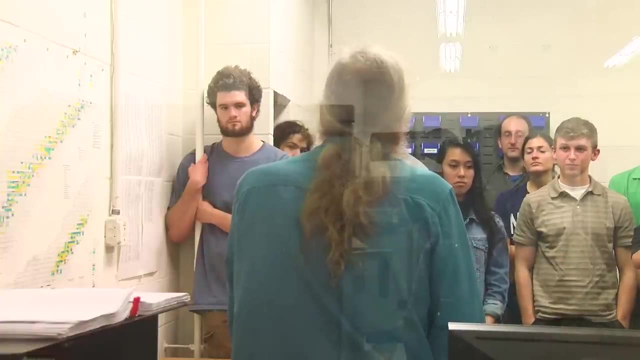 the time when the contamination was the worst, which made people happy, sort of in retrospect, you know that the contamination from that area didn't get into the well water. um, yeah, that was in the mid 90s or so. anyway, that was, you know, one of my samples and the 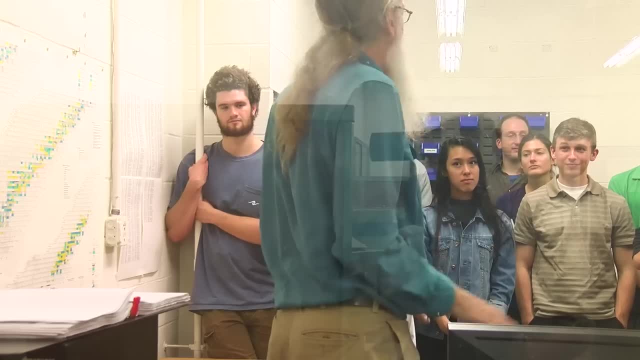 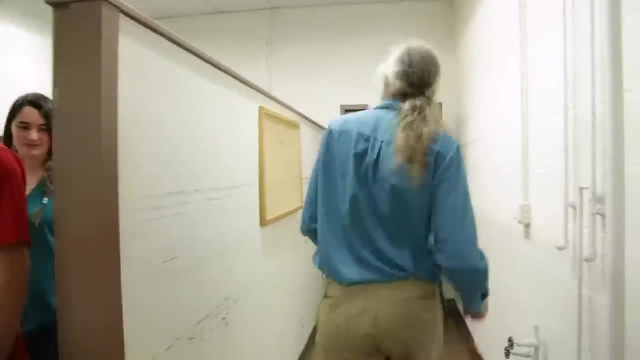 hair is a pain in the neck to work with, so i hope none of you gave me hair samples. i won't run them, okay, so let's go down the hall this way. you all got to follow, so this is, i mean, it's just a fine powder. 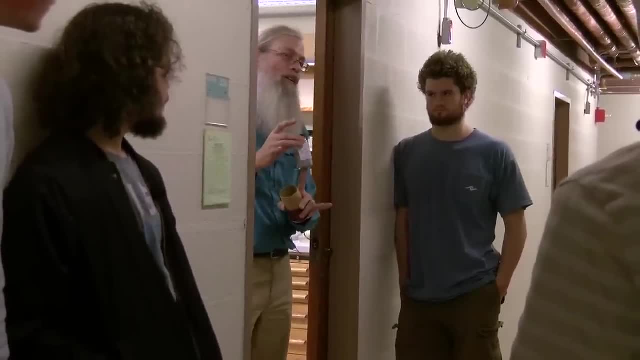 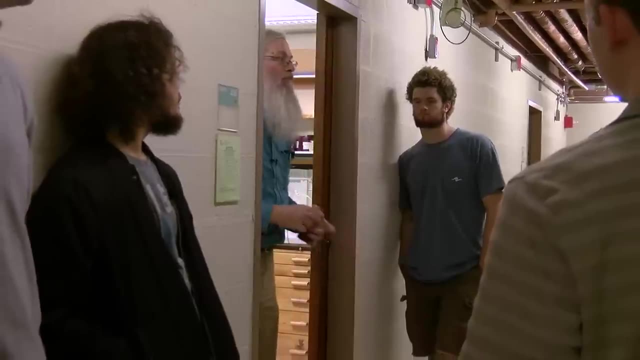 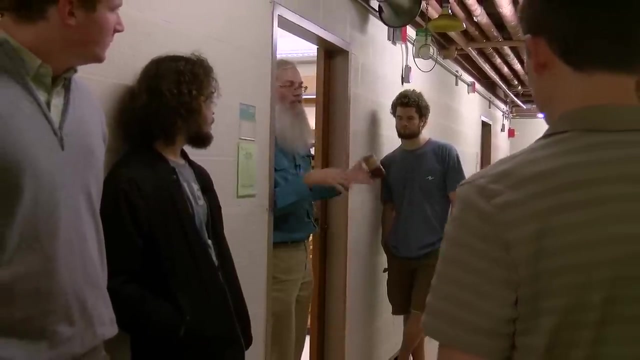 and it's a fly ash from a coal-fired power plant. fly ash means the ash that goes up the smokestack, as opposed to bottom ash, which is what falls down. and so, uh, they collect a whole, you know hundreds- of kilograms of fly ash, just homogenize it, sieve it, send it out to all a lot of labs to analyze. 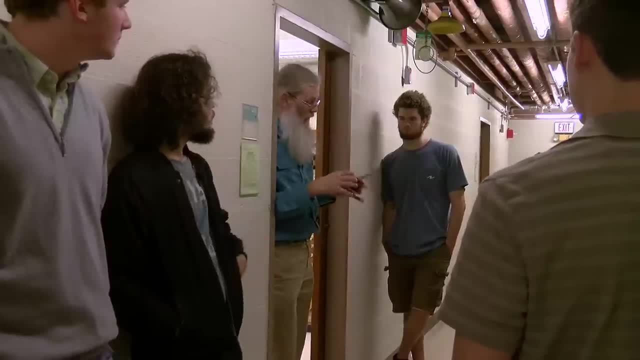 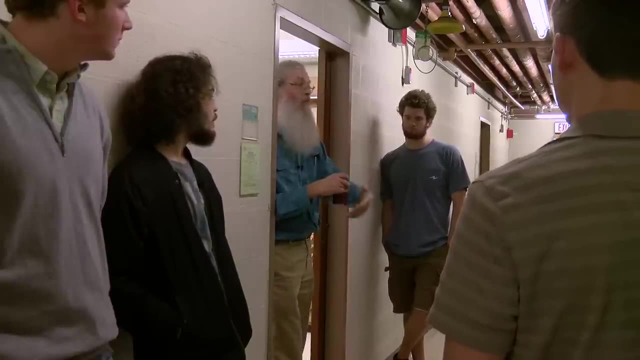 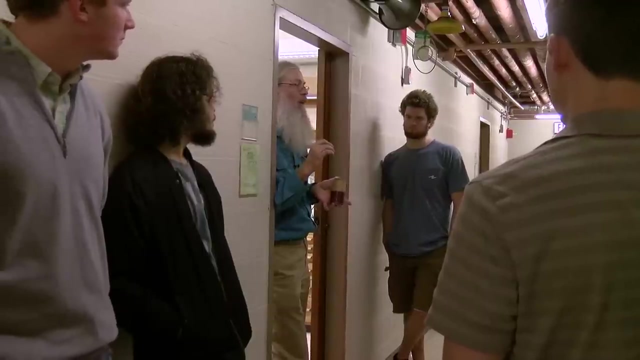 nibble. this is really good at this. take all the data, and so this is this ash is characterized for about 20 elements or so. so when i run my samples, if i were to run your samples with standards, i'd run a little bit of this- five, six, seven milligrams- and i know what the the concentrations are in. 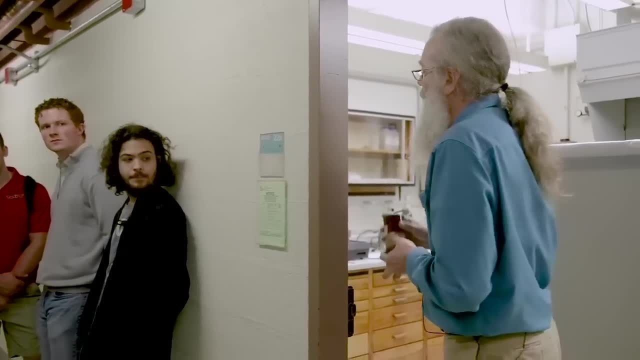 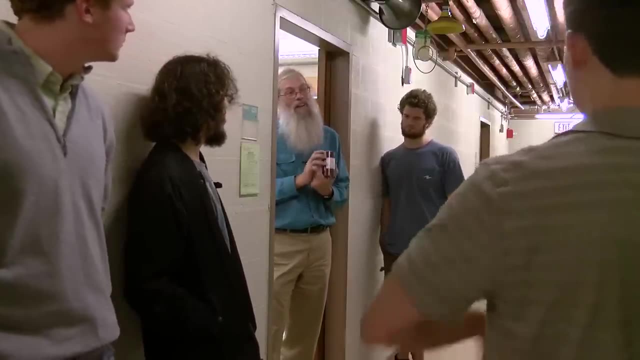 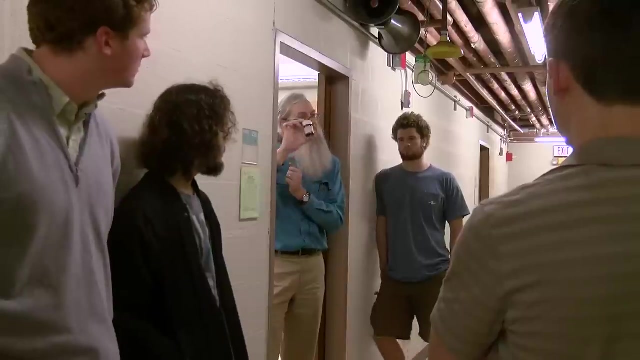 this, and so that's how i do the comparative method, and so i got you know this and they all look the same, and you know this is some soil from montana, next to a mine, so it's nicely contaminated with some metals. this is my iaea, mercury and hair. 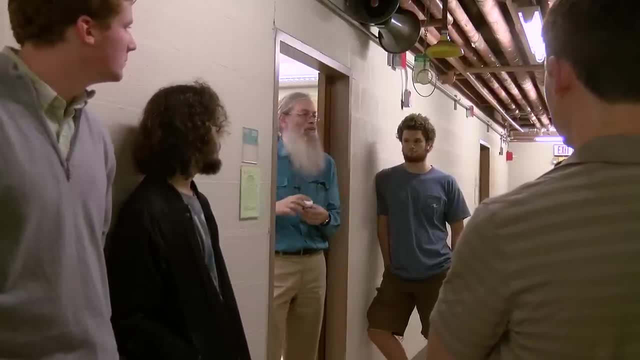 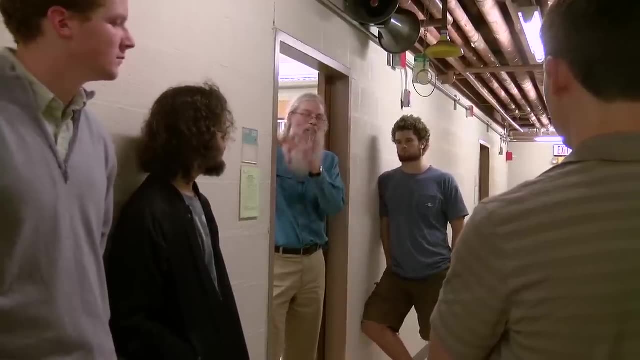 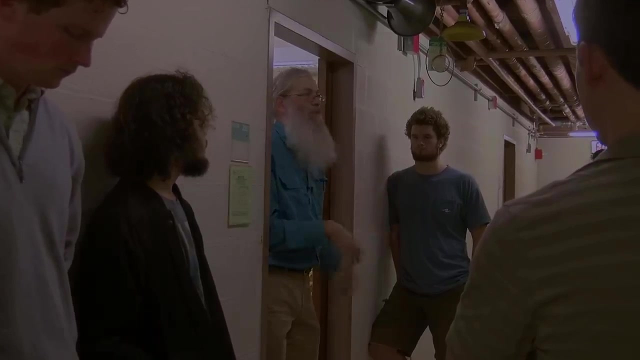 standard, but again, it's just a little powder and this is kind of what everybody uses for standards, and you just kind of have a whole collection of them and, depending on what elements you're looking for, you try to mix and match them so you get cover what you want without having to run five or six on them. this is my, my hot lab, or one of 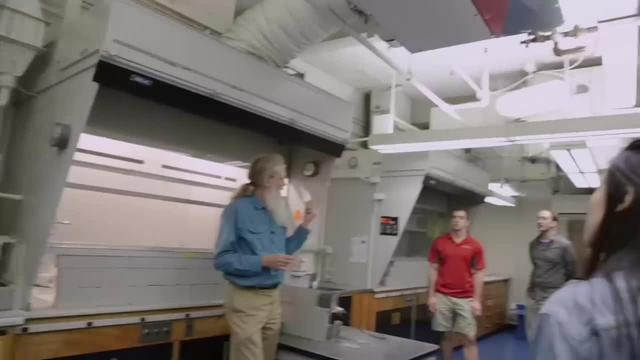 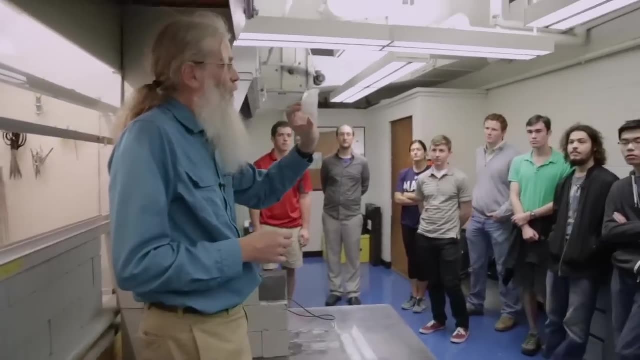 my hot labs. uh, you guys, last week, or whatever it was, i came by, so this is the rabbit- those of you who weren't there, these are. i call these. these are called rabbits because it's the little thing that runs through the pneumatic tube. uh, you guys are doing power nips later today. yeah, when you're. 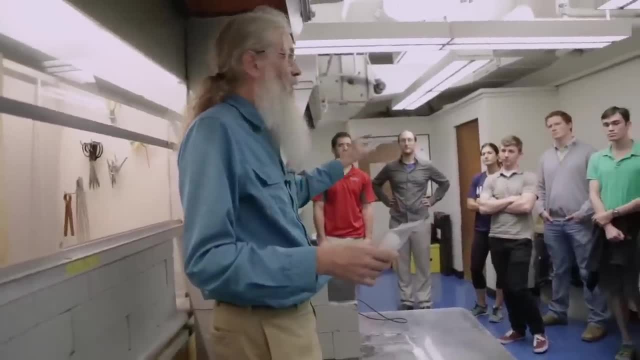 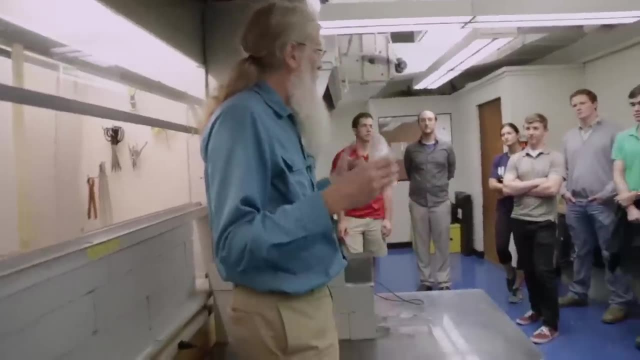 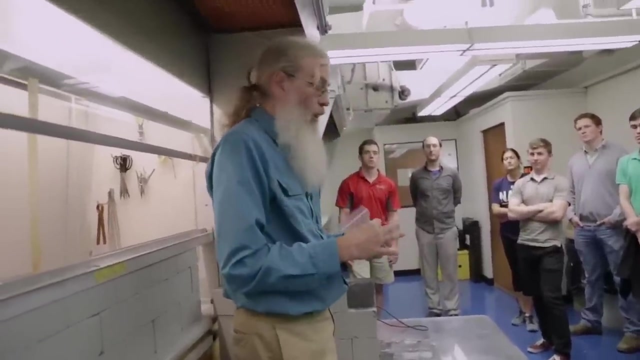 sitting at the control panel. there's a button, i think it's to the left and it says insert rabbit- and that's what this is referring to- for longer radiations. there's a spot in the basement in the reactor where they can get these and they send them into the, the radiation location for short. 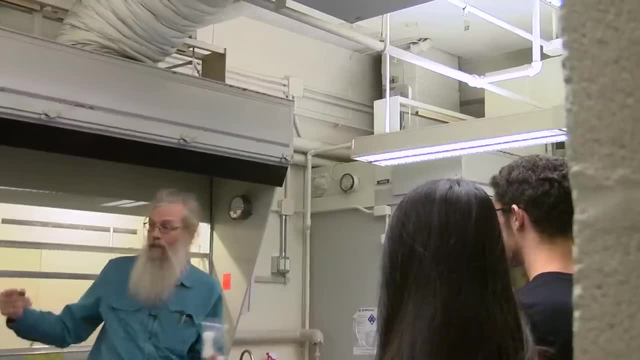 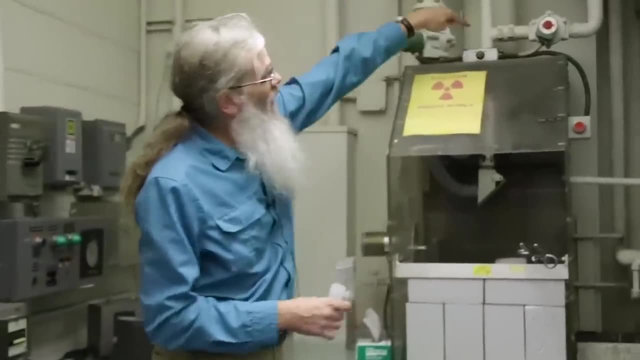 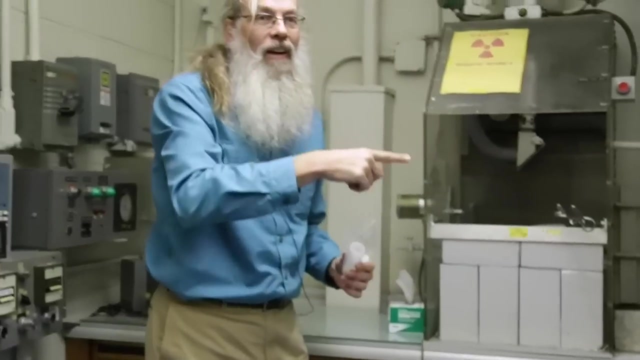 radiations like what you guys are going to be doing in a month. i send them in from here. that's okay. i just don't want to bump into that thing. um, yeah, so this is one end of the pneumatic system and so i can put a couple of samples in here. i stick it in that little tube there. 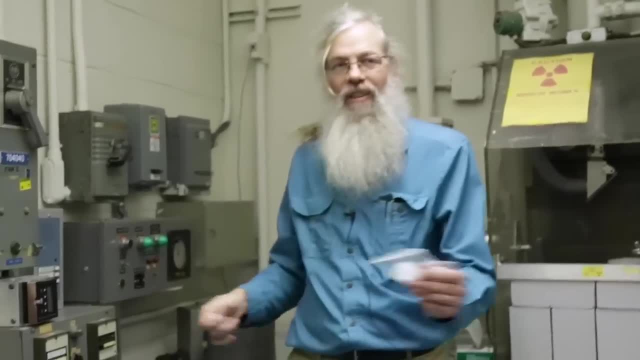 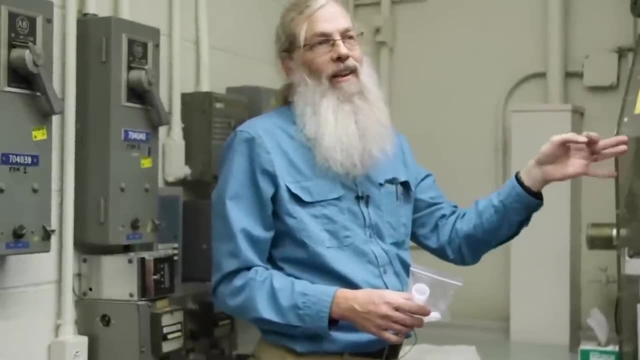 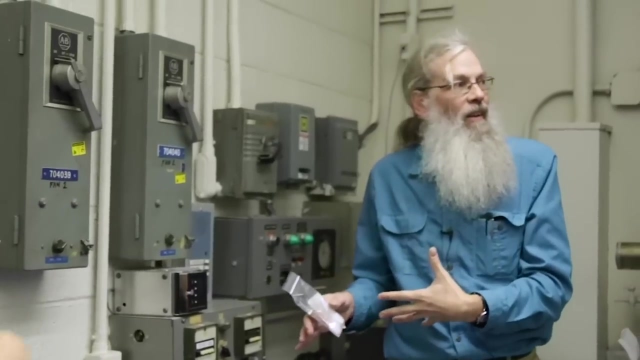 call the control room and say, okay, turn a bunch of knobs and switches and whatnot. it goes and in about 15 seconds it's next to the react, next to the core of the reactor and the graphite. i usually run shorts. i'll usually irradiate for about 10 minutes. we usually let 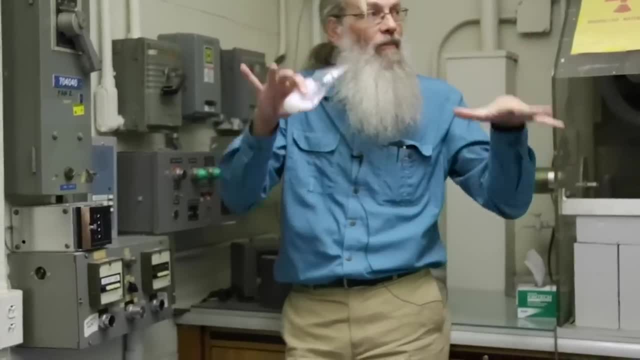 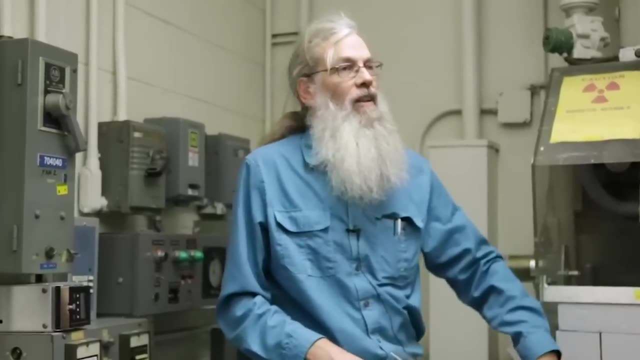 the sample sit in the reactor for a little while, so the very short half-life stuff decays away and then it comes back out here and the whole the thing just kind of shoots out there and bounces into here and then pop open the rabbit and in that hood 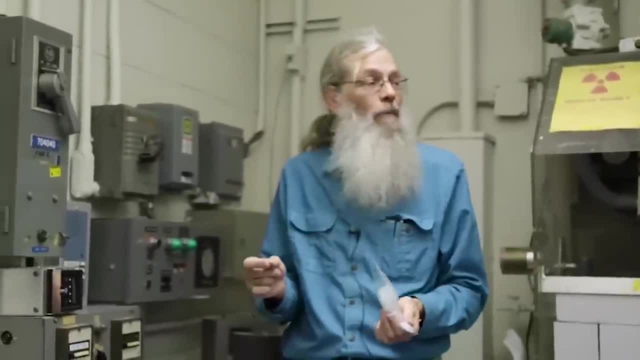 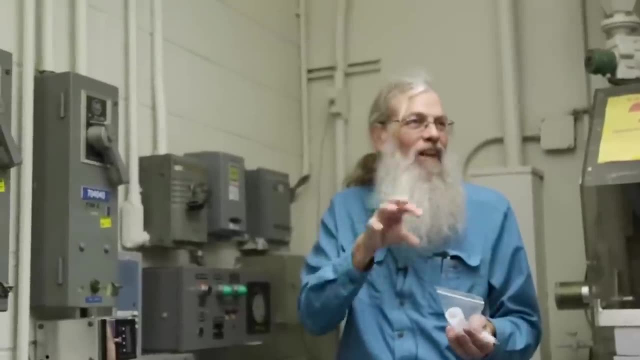 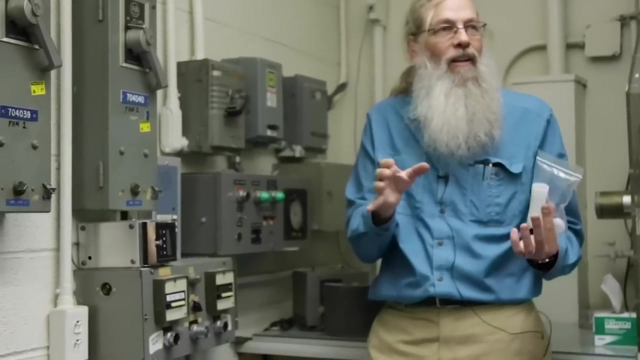 pulls the samples out. i usually try to repackage the samples um. so this is partly why i asked for stuff that's kind of one or two good solid pieces, because then i can take it out of whatever it was irradiated in, put it in a clean bag or vial and that way we don't have to do a a blank subtraction. 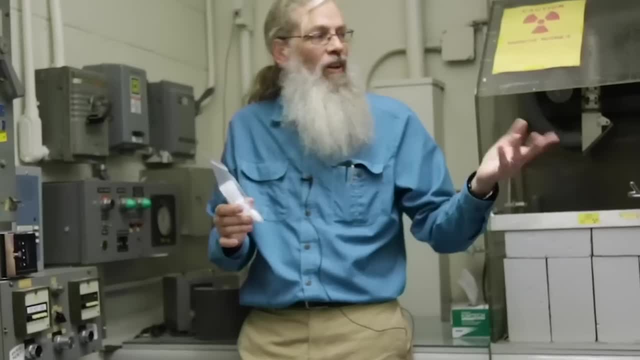 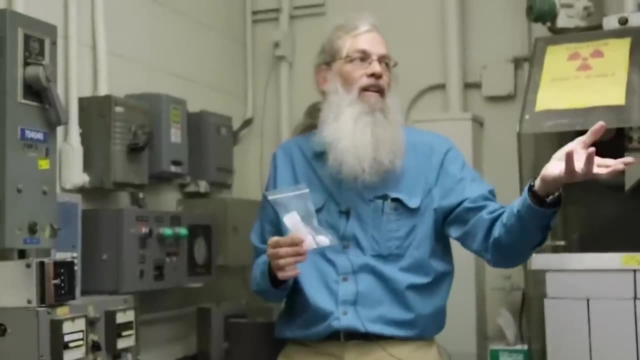 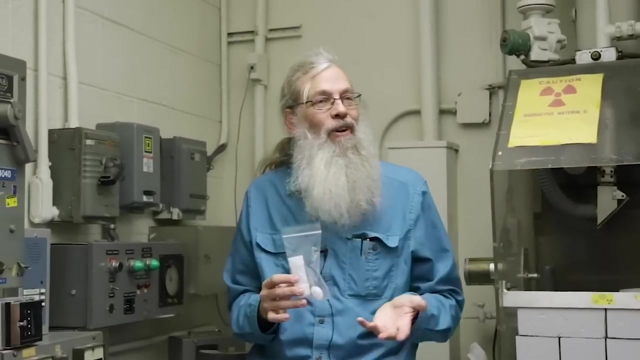 for the sample. that makes sense because otherwise, if i take like a little vial and irradiate it and then count it, i'll also have whatever elements are in the vial. um on the thing for when i'm running standards, and this is when, uh, you won't. if we're not running standards, you don't have to worry about this. 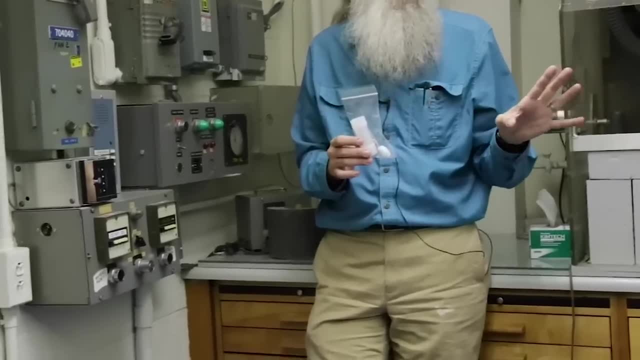 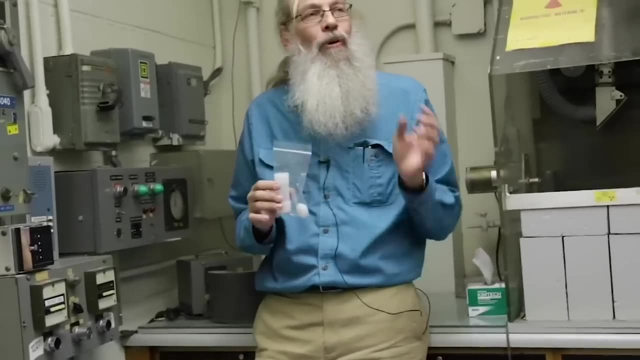 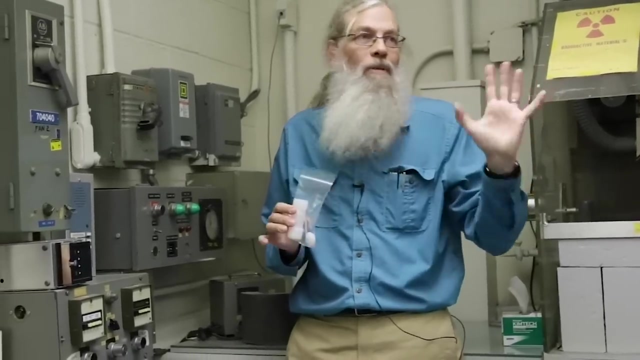 that powdered standard stuff. i'd never get that out of a bag because you'd never get all of it out and i'd have contamination everywhere if i started cutting open those bags. so i do have to do a bag correction for those. so when i do an irradiation i always irradiate a few, just empty. 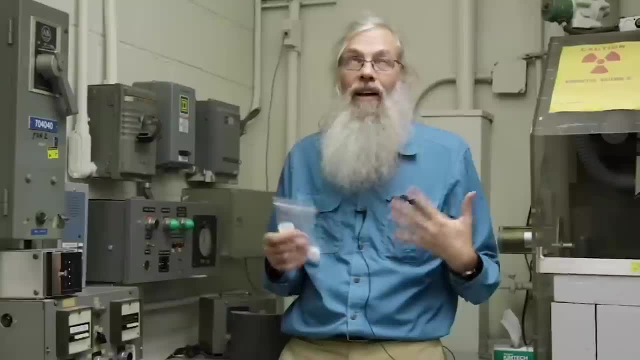 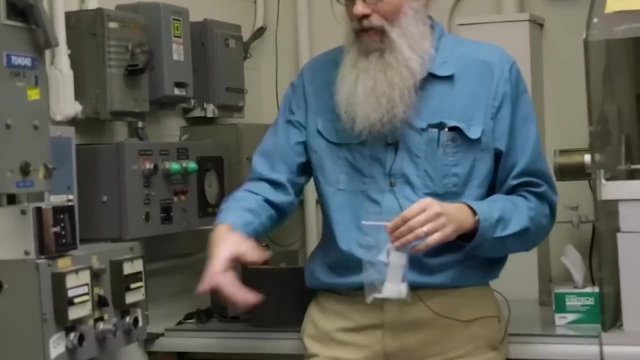 bags and then you're good to go and then you do a correction for those, because the bags have got aluminum and antimony and a bunch of things in them. um yeah, and so then, like, i take a couple of samples, i throw them in a lead pig. so i got a whole bunch of these floating around and i run. 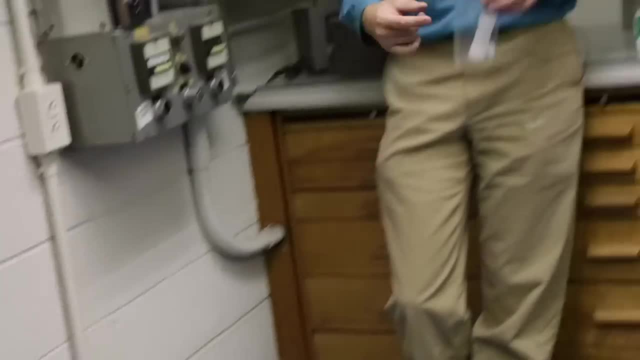 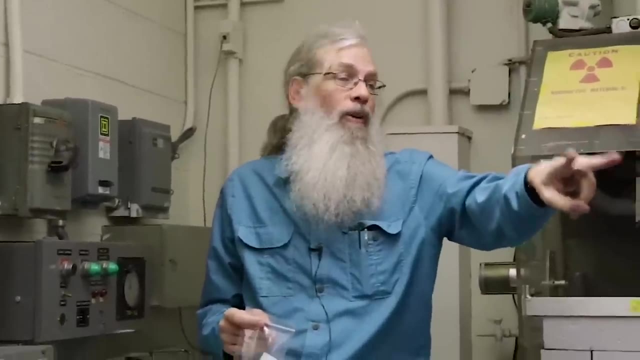 it down the hall and throw it on a detector and we count it. when are we doing shorts? um, i'll irradiate two samples at a time because i have two detectors. when i used to have four detectors, i ran four samples at a time, so you irradiate it. 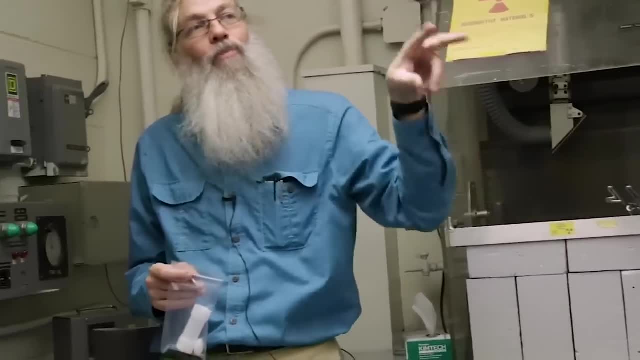 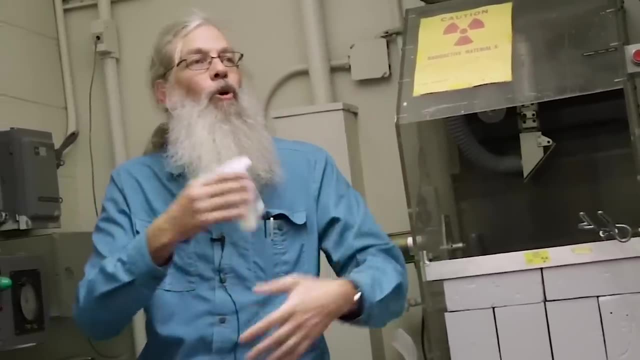 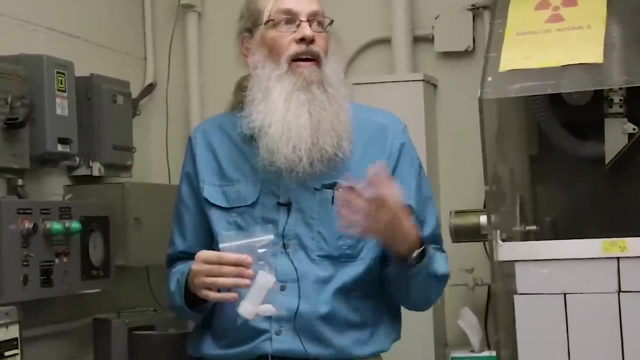 count it. while that sample, those pair of samples, are counting, you come down here, you irradiate the next two, so that you know you're just kind of always irradiating and counting. um, i usually do a 10 minute irradiation for shorts. i'll do a fairly quick count five minutes right after i. 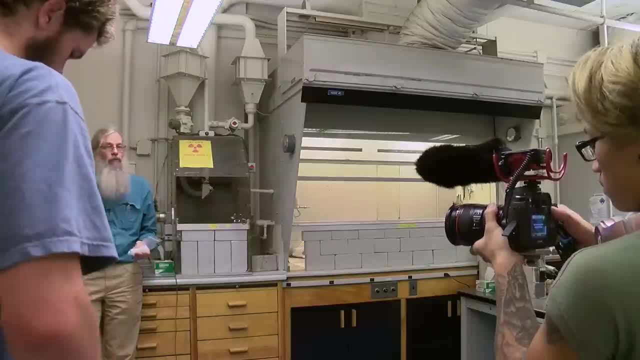 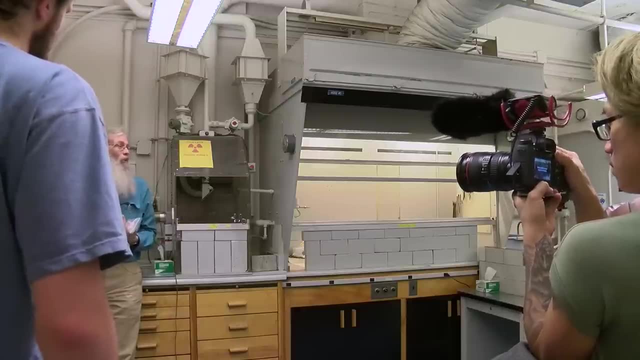 get the sample down there and that's looking for stuff with half lights, sort of under 10 minutes. the shortest half-life i've ever done is five minutes. look for is for aluminum. it's two and a quarter minutes, but things usually have a lot of aluminum. 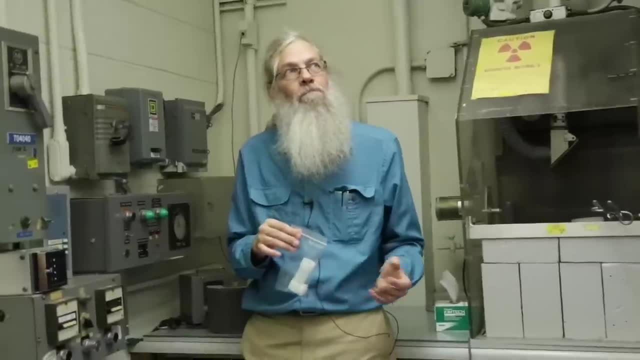 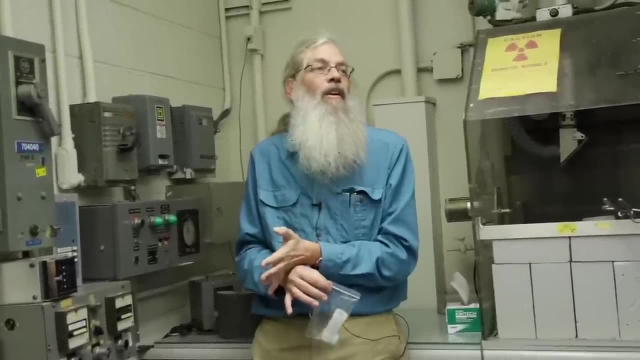 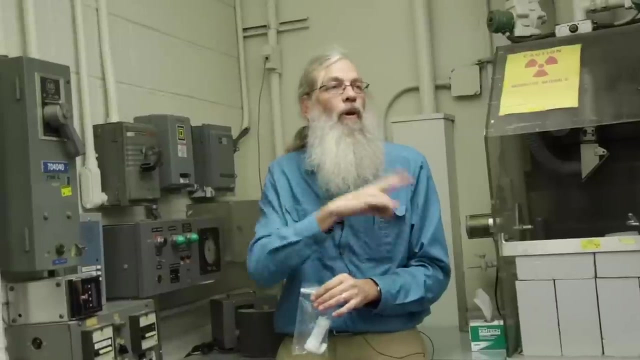 in them. so i see i see aluminum pretty well. um, for shorts, i'll count all the way up to about sodium, which is almost 15 hour half-life longer stuff. i'll do a long irradiation to count. there's a little overlap on my shorts and longs. that helps me do qa on things and if i run two standards i'll 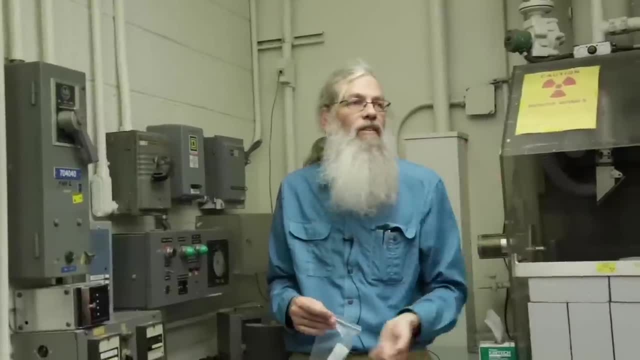 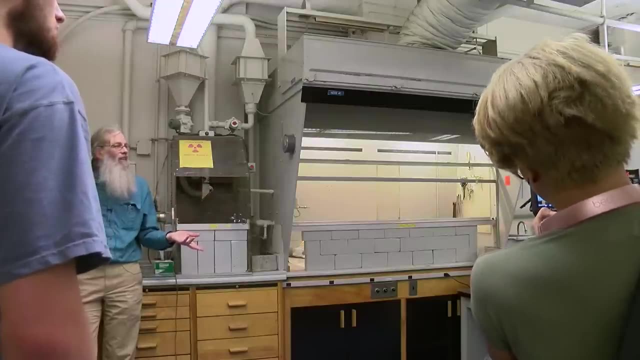 check, you know, the concentrations from one standards to the other. that's another little thing. i don't know what else we got. what questions do you guys have questions? it's pretty straightforward what sort of things you're going to be bringing in? yeah, what do we got? 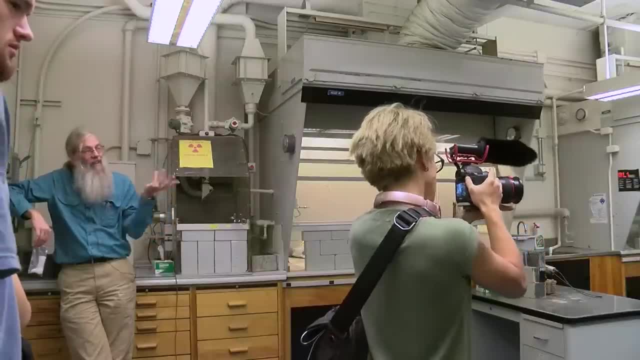 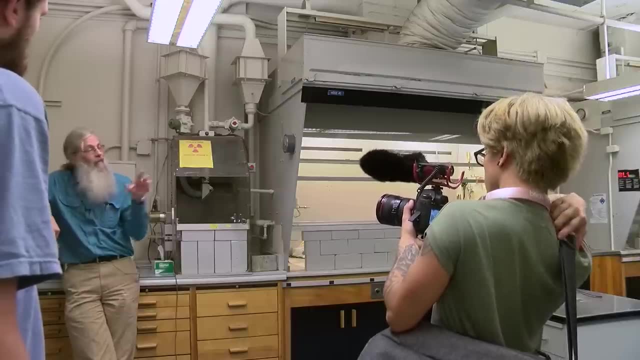 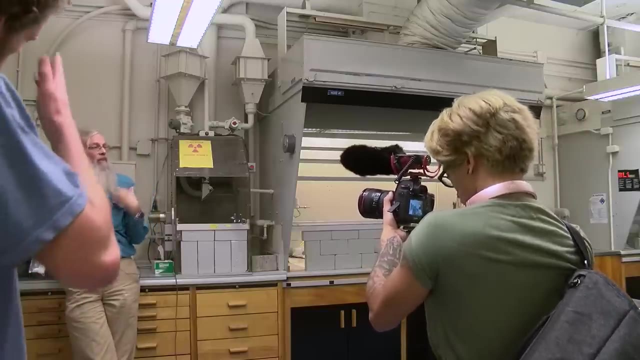 oh, yeah, yeah, okay. yeah, there was a lot of archaeology that did you know? um naa got used for that a lot. i don't think we ever did it here. fred fry, who's a professor retired now- uh, from eaps- earth, atmospheric and planetary- he did a lot of geological samples and 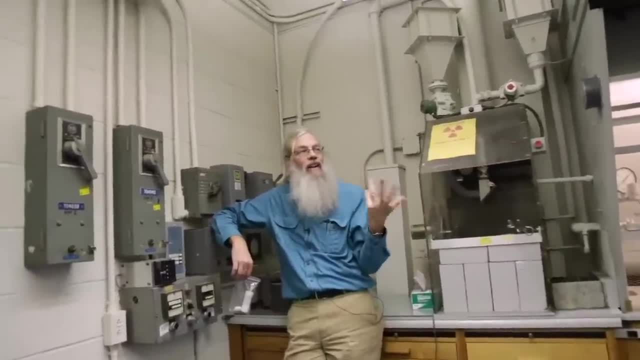 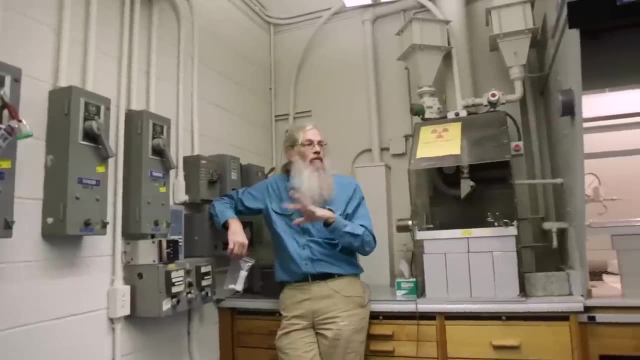 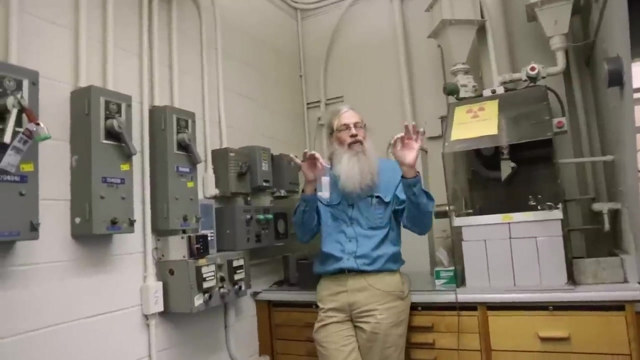 yeah, there's, i forget where it was that. they did all the archaeology. one of the things naa is really good for is, uh, rare earth elements which are hard to measure by other methods. i mean, i didn't get very low limits on that and by picking out various rare 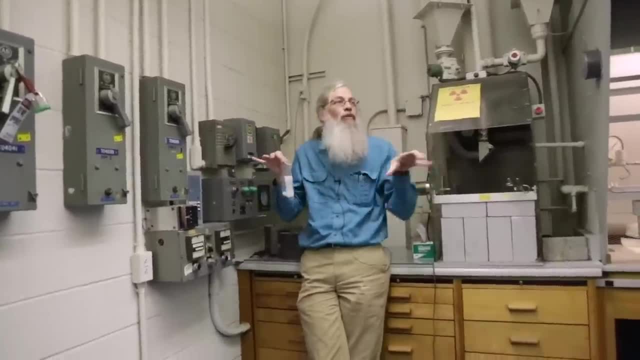 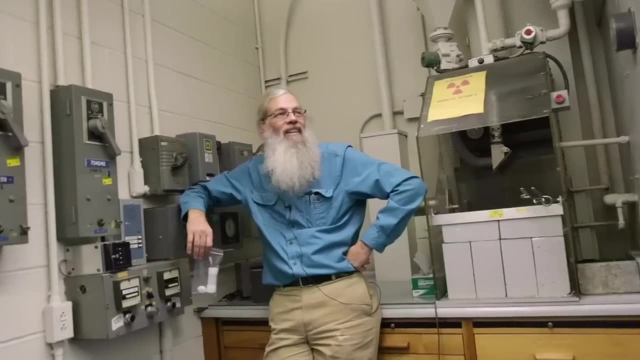 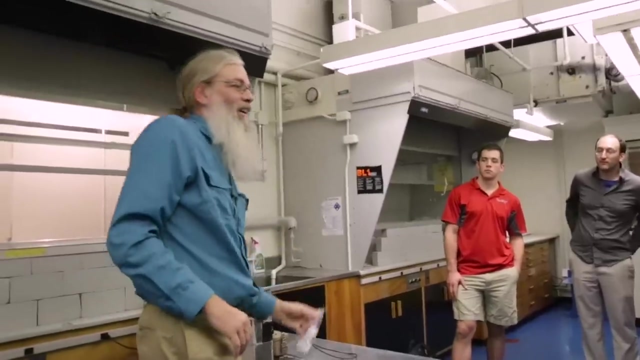 earths and the ratios. it can help identify where things are from in the world. yeah, can i use it sample if you give me a little tiny piece of it? okay, i mean, you know, i mean the like how small? well see, that's the rabbit. so it's definitely got to fit in there. 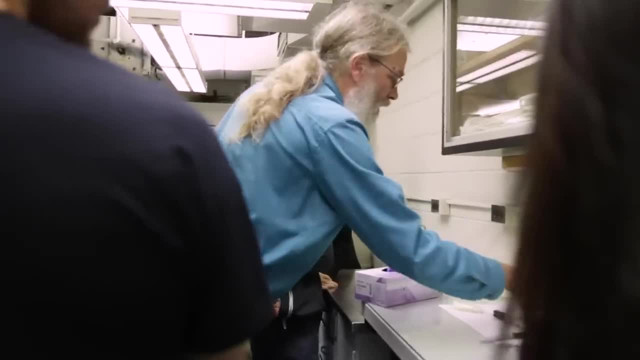 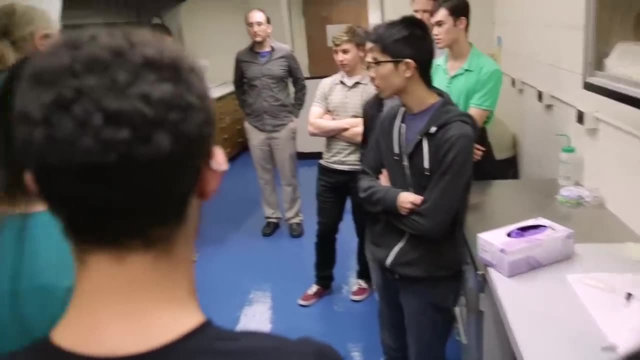 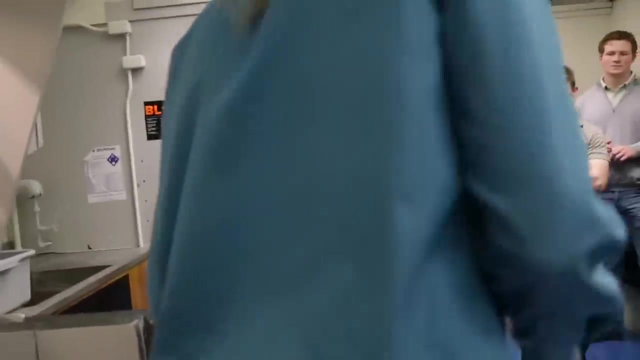 the thing i really like. yeah, excuse me, where's my vials? yeah, i used to have some smaller ones up here, but so you know that's should definitely fit in one of those. like see that guy, okay, um, my usual description of what size sample i like is if it's a piece that you would pick up with a pair of tweezers. 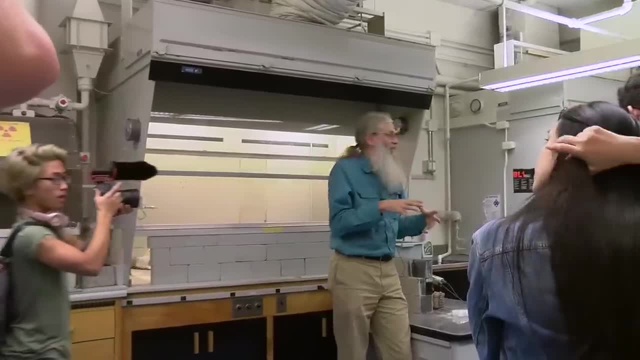 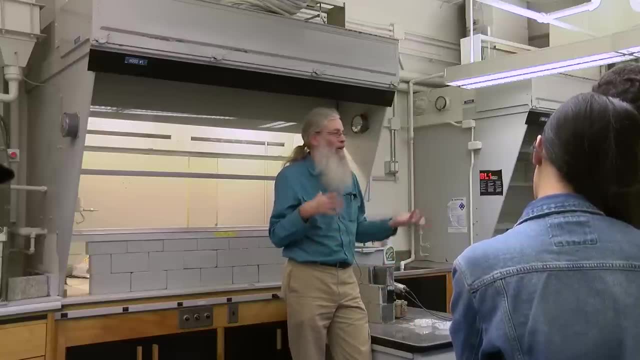 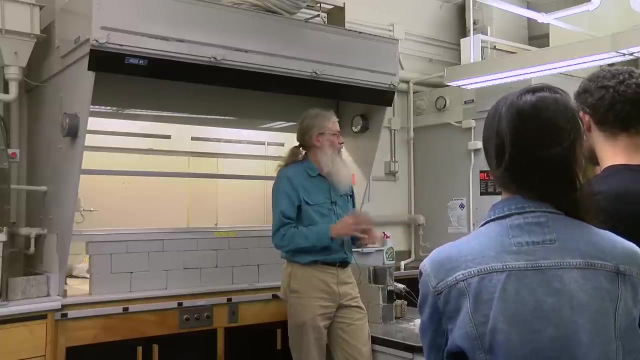 so not too small to pick up with. you know to be able to find so no powders, but you know, and you could maybe get it with your fingers, but 20 milligrams, 50 milligrams, 100 milligrams is just in the right ballpark. what else you guys think no, doesn't matter. we'll look at what comes in and 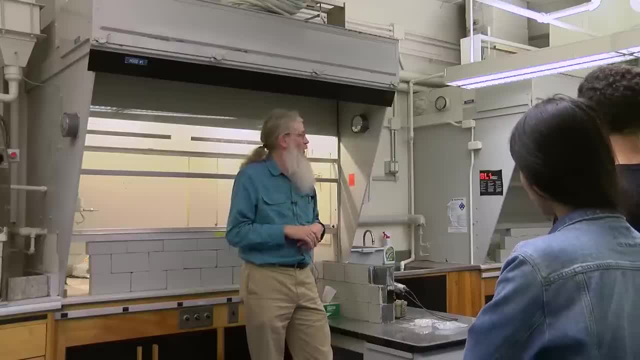 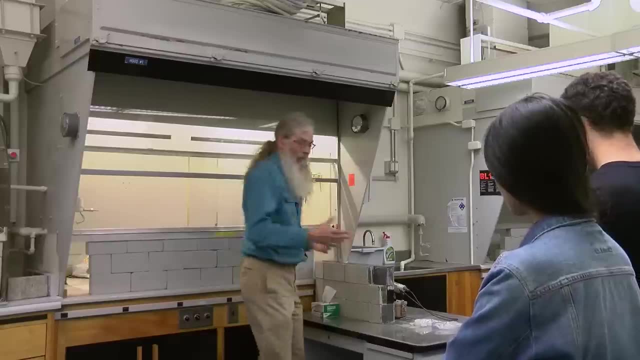 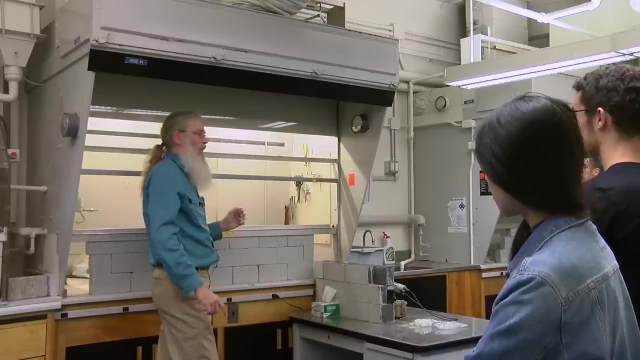 yeah, i might veto some things or not, but we'll see. we'll see what we got, okay. well, we got bricks everywhere, so when i, when i get the sample out of there, i do the repackaging in here, and so this is just shielding between the samples i'm working on and myself. i don't have. 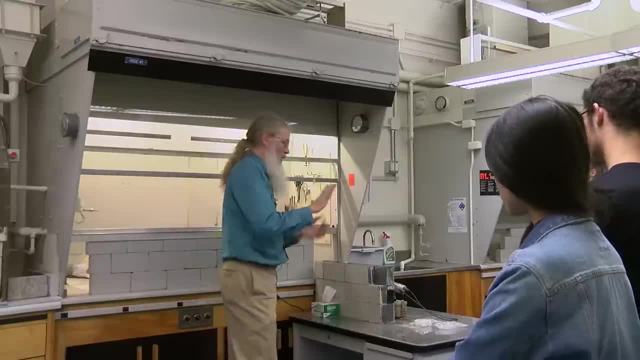 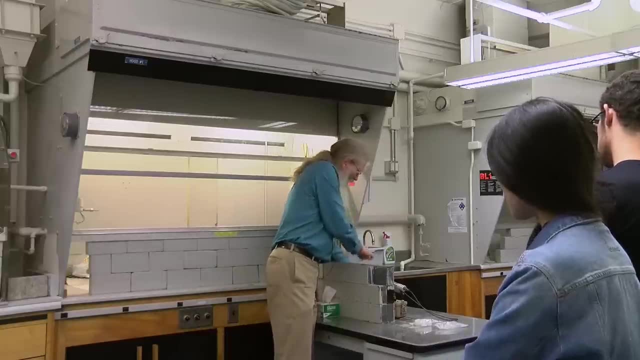 my docimity on now, but i usually i've got the symmetry and a ring badge, and then it kind of comes over here and i do the. this is where the heat comes in between those two pieces, and so you can the heat sealer is, So I'm going to heat seal it here. 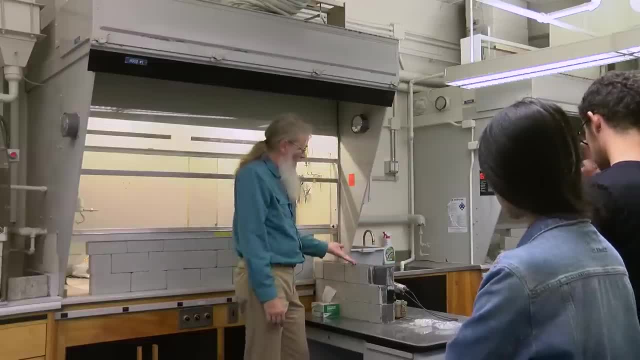 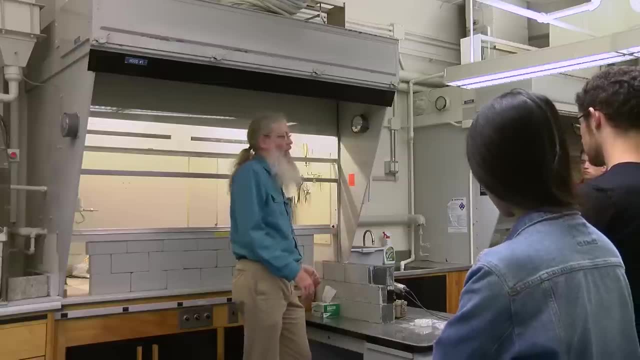 and then I'll have a pig over here. They're just painted lead bricks. Yeah, these are just painted lead bricks, And these have been here longer than I have. Sometimes things just are somewhere and you never move them. These, I think, are older than me too. 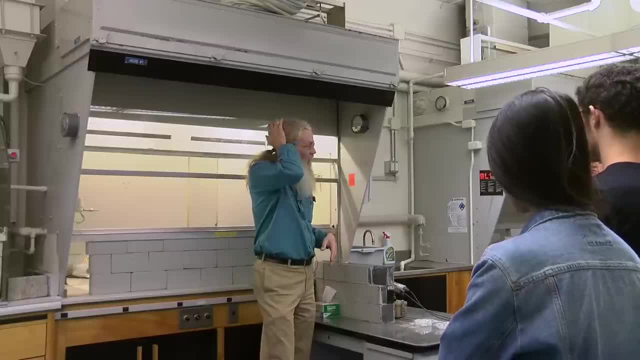 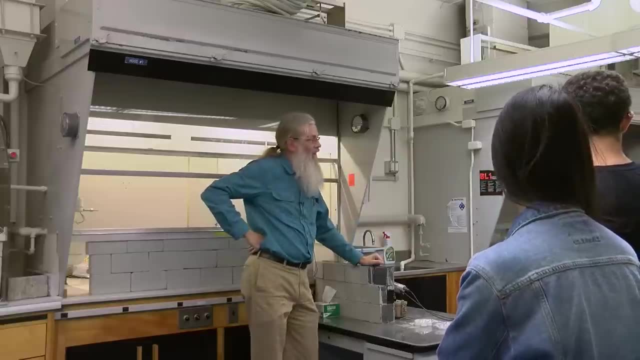 This lab has been doing NEA, I don't know- since the 70s, I think So anybody else. Is there a single brick that I could just hold to see how heavy it is, The full-size bricks like that size? 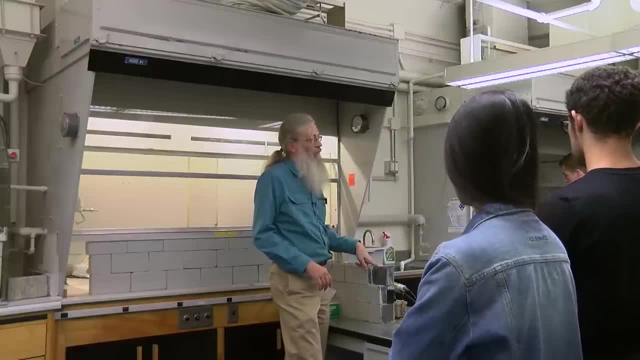 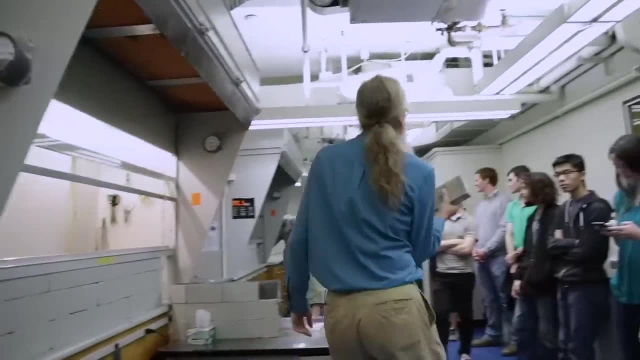 2 inches by 4 inches by 8 inches, weighs about 25 pounds. There's usually a bunch of them floating around. I don't know, Here you want this guy. That one's not quite full-size, So you know they're heavy. 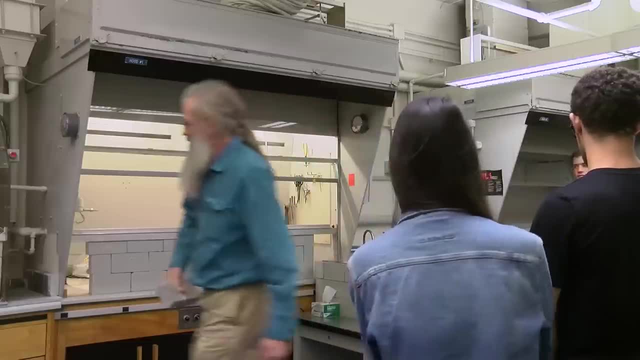 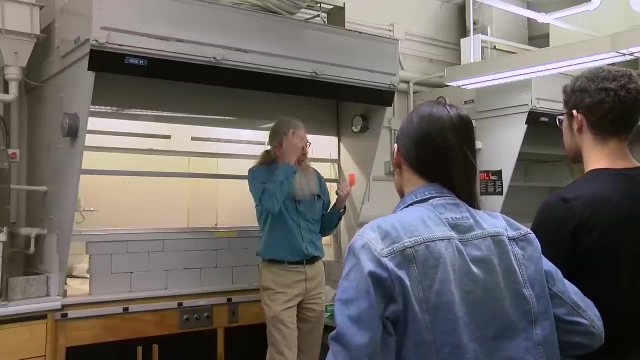 They're lead. Anybody else want to toss it? No, OK. When people ask me because I work in the reactor as well, they say: is there anything dangerous in the reactor? The dangerous thing is dropping lead bricks on your feet. 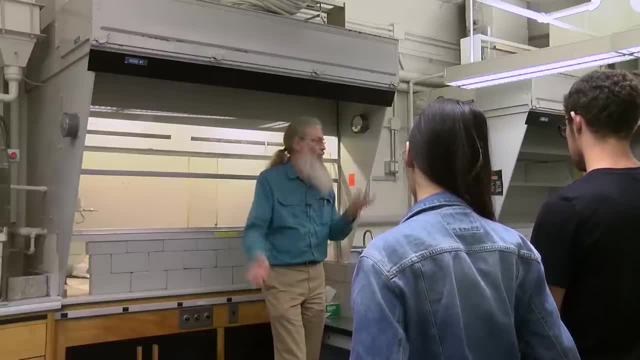 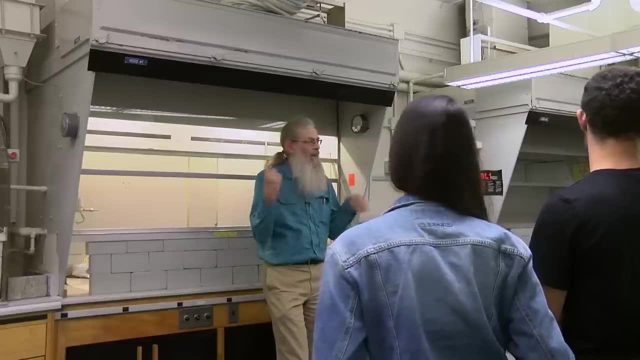 That's why I've got steel toes. If I missed the toe, yeah, I'd probably break my leg. I don't want to think about it. And they move much bigger things in the reactor. Have you toured the reactor yet? Yeah, 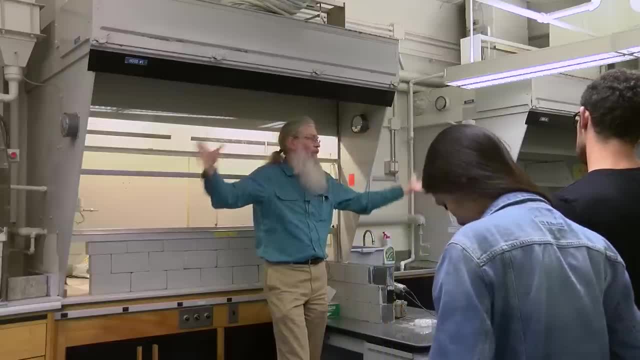 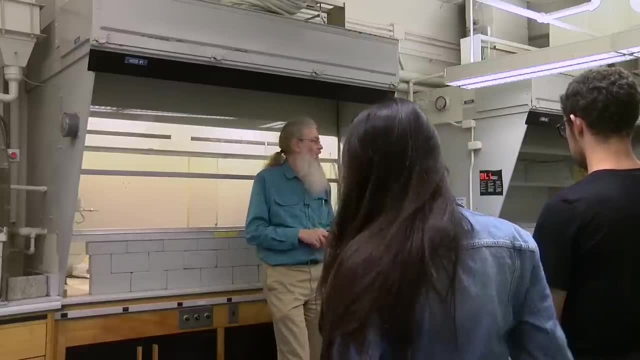 So I mean there's that giant crane there and they move five-ton pieces of shielding and that's the other dangerous thing in there, dropping really big things. We've never dropped anything. We've never dropped anything that big. I think somebody dropped a steel plate on their foot once. 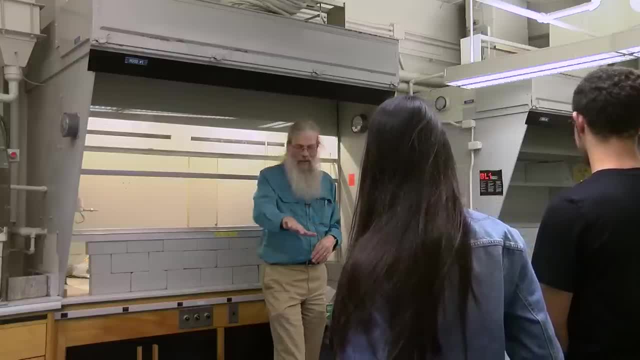 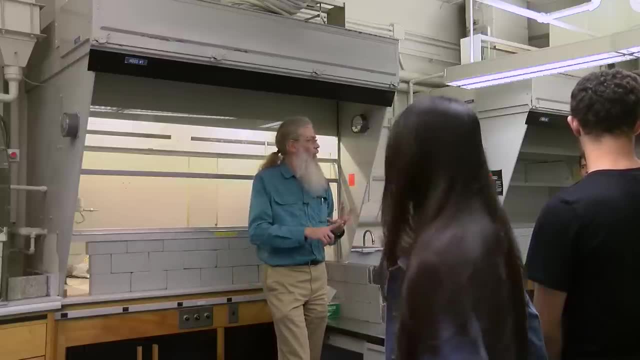 That was about the worst of it. You know, like four-foot, half-inch steel, Boom. That's what happened to my foot. Yeah, Oh, OK, Good. You know, when people trip and fall off ladders and it's the usual industrial accidents. 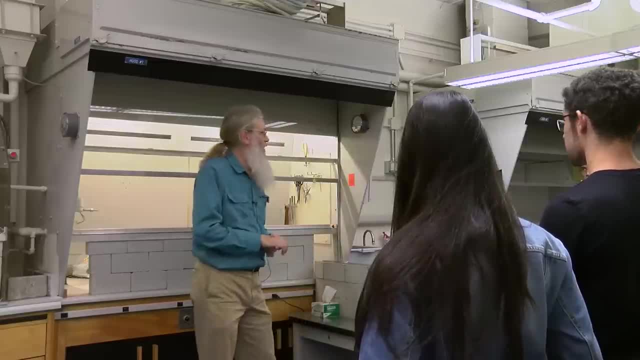 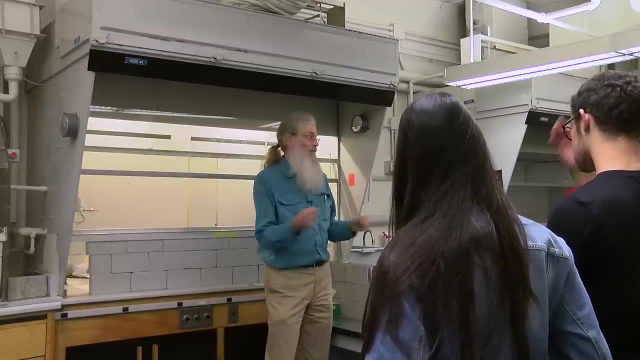 OK, Good, yeah, I mean I've broken a few, but not here Cool. Thanks a ton, Mike Sure, And I'll see you guys in a month or something and have fun running the reactor. Good day, folks. 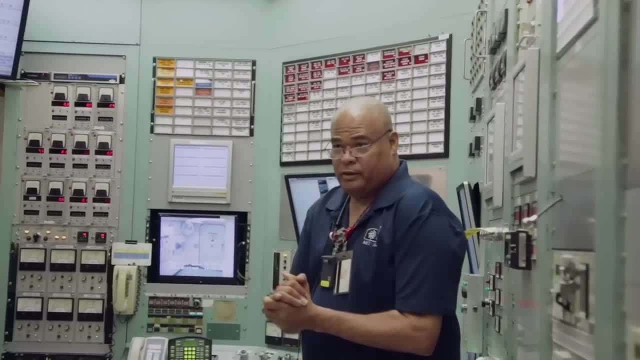 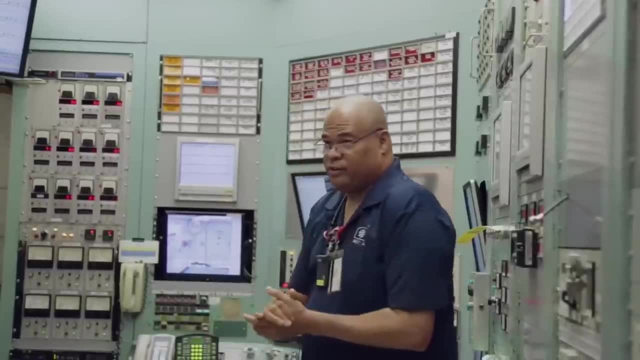 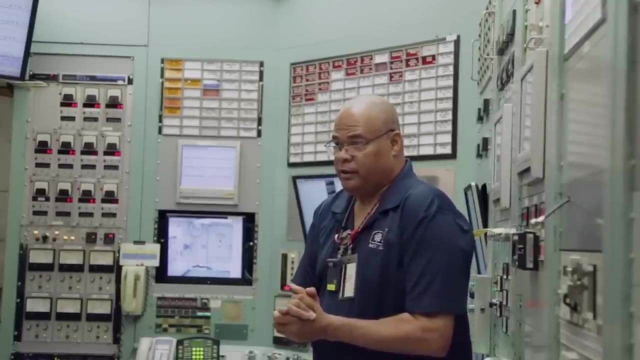 You guys are here to do an experiment on the reactor. It's in two parts. The first part is raising reactor power. The first is raising reactor power using a low-worth absorber called a regulating rod, And then the second part will be lowering reactor power using 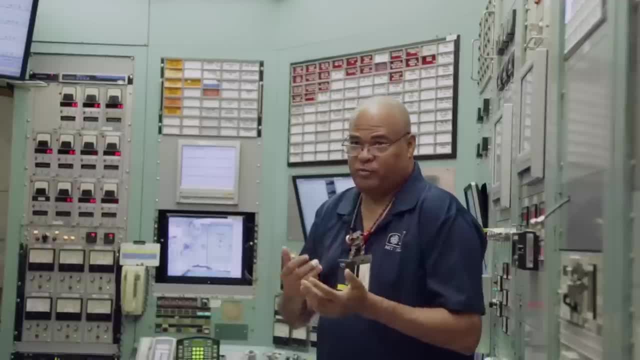 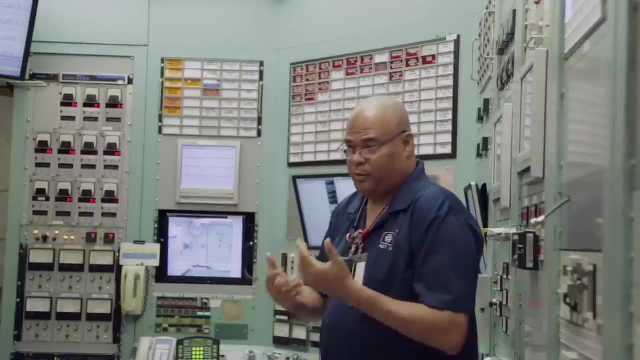 a high-worth absorber And the high-worth absorber, things will move much faster And we don't want to run into a chance of you accidentally going too high, So that's why we use a low-worth absorber on the way up. 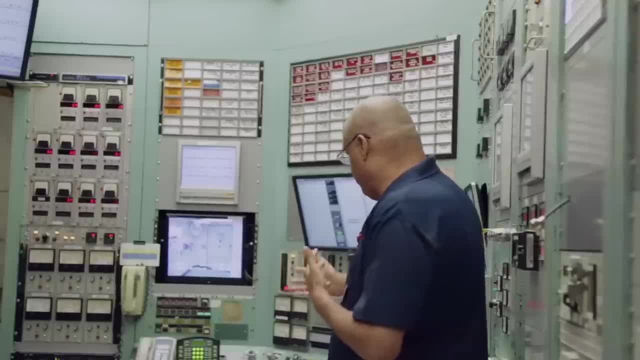 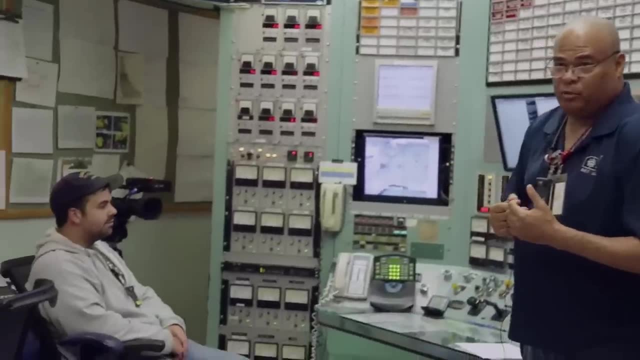 and a high-worth absorber on the way down, And I just want to show you the controls. With me today is Tim To actually do this experiment. we need two licensed people in here. One at least has a senior reactor operator. 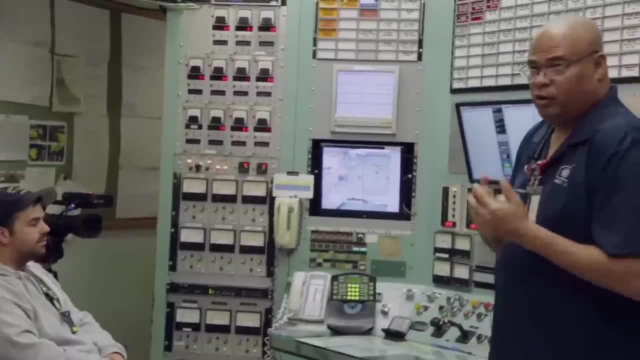 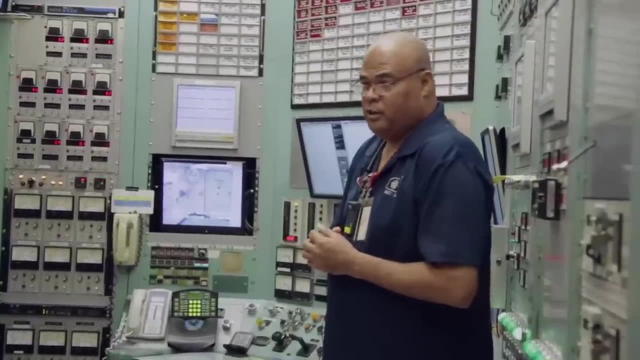 Both Tim and I are both senior licenses, So we have that covered. The only way you can actually do these manipulations are if you're in my training program, I'm the training supervisor for the facility, Or you're in a program that needs. 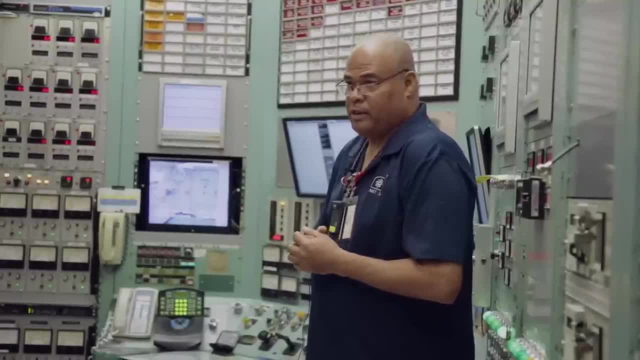 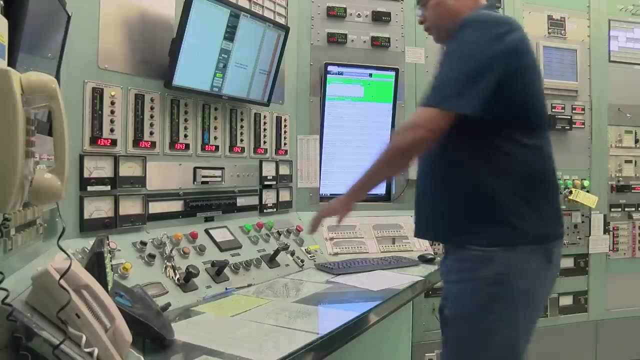 you to actually operate the reactor And the program you guys are in fits that definition. So I just want to show you some of the controls of the reactor. First we have our shim blade controller. This basically moves one of six shim blades. 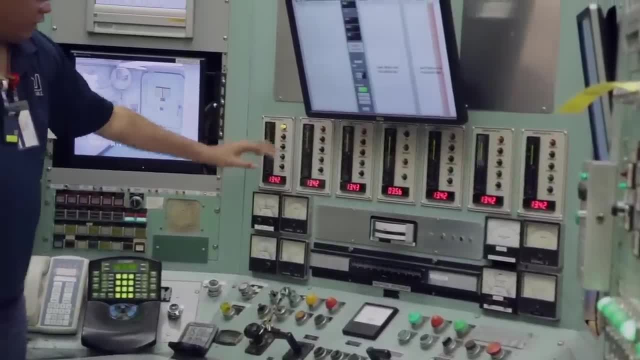 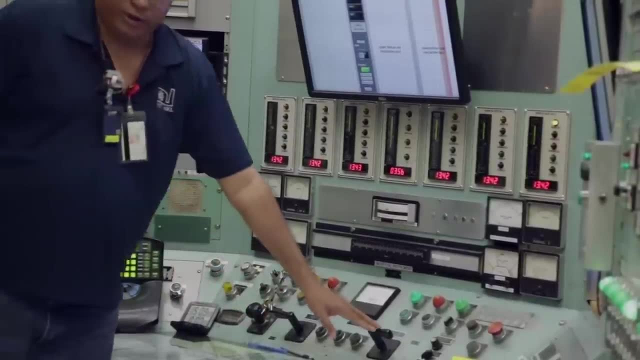 At a time. The one that's selected has this light on it And we can change which one is selected with the shim blade selector switch. This switch here is a regulating rod. This one will allow you to move the regulating rod up and down. 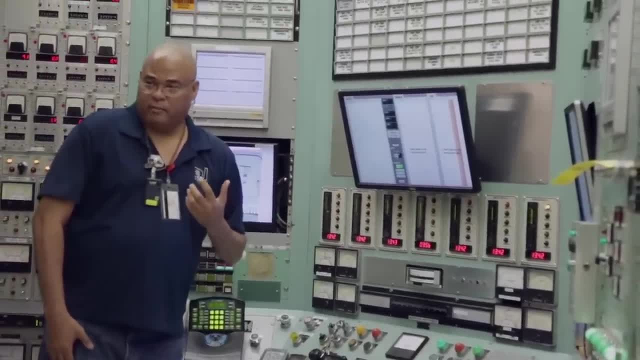 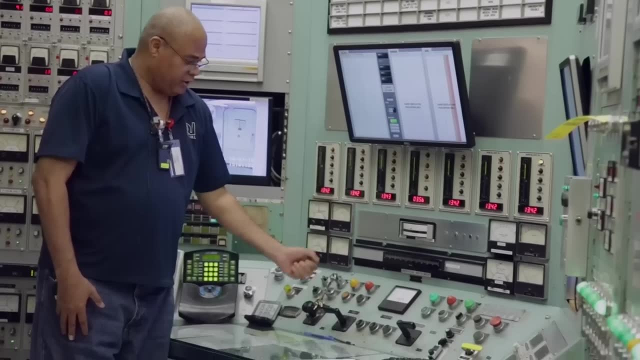 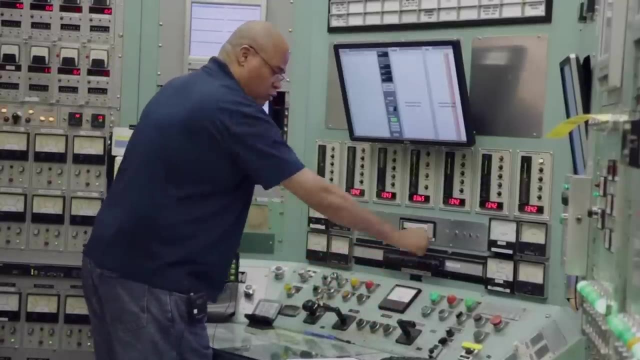 Our blades are fixed speed, meaning they can only move at the exact same rate at all times. Moving the shim blade in an upward direction or the regulating rod in an upward direction, take an underhand grip and pull up or twist upwards until it stops moving. it just a little. 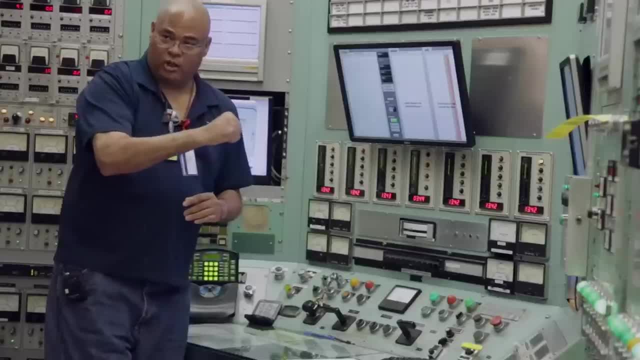 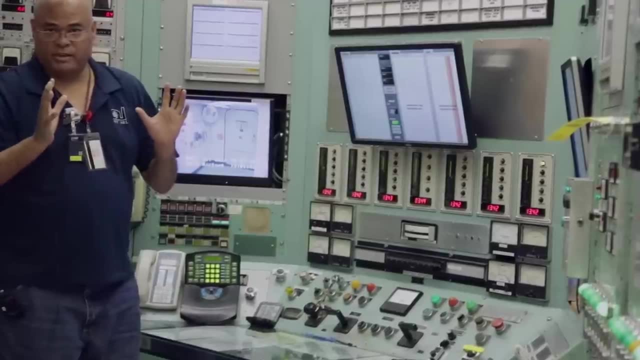 bit doesn't move anything. you have to move all the way until it stops and then the absorber will move in the outward direction. if you want the blade to stop, just release it. it's spring loaded and we'll go back to the neutral position and stop moving. if you want to drive something in the 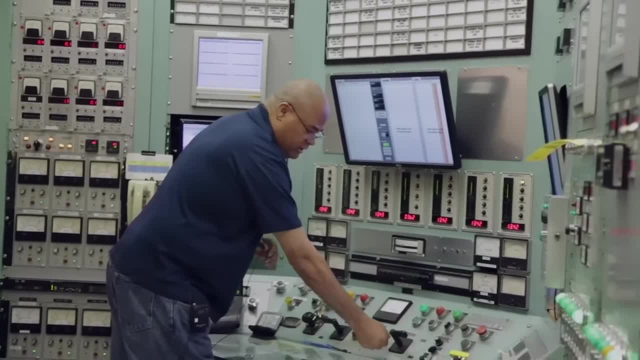 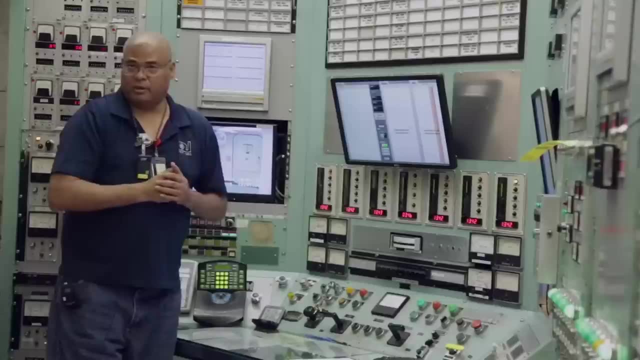 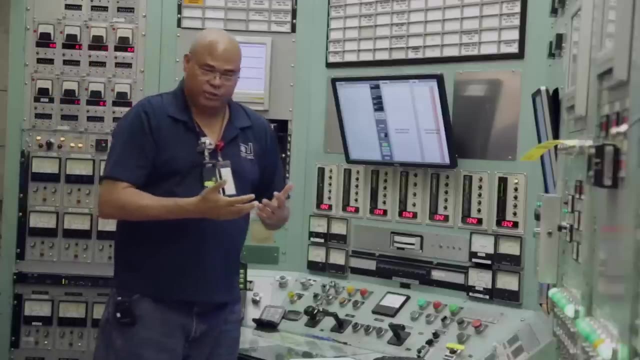 inward position. take an overhand grip and twist downwards and that will drive the absorber in once again. let go, it'll snap back up and stop the motion of the blade or the regulating rod. the experiment we're doing is basically changing reactor power by half a megawatt and we're 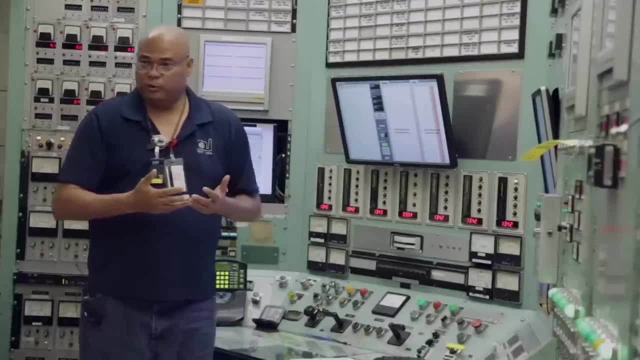 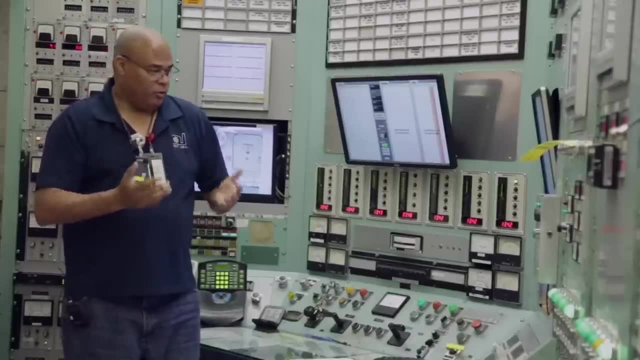 currently at 500 kilowatts. we're going to bring it, bring the reactor up to one megawatt and then bring it back down to 500 kilowatts. so before we can do this, you have to log into our logbook as a trainee on console. 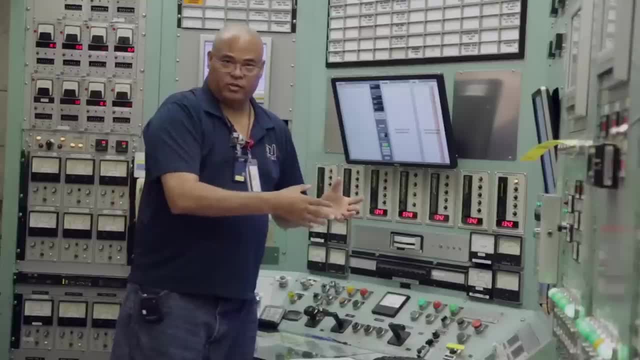 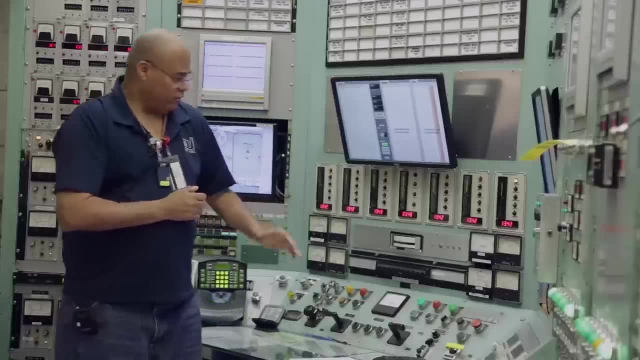 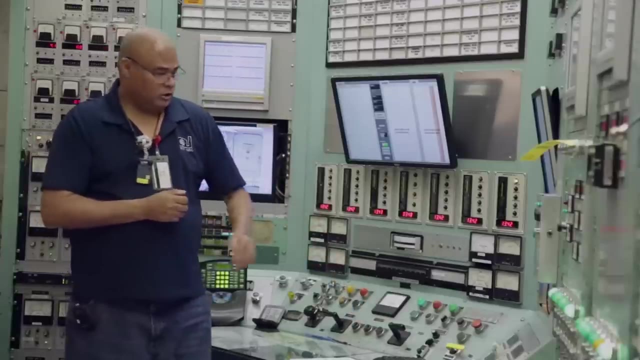 we'll show you the proper way to make the entries. as you make those entries, you'll go ahead and then do the actual movement itself. okay, so the first one is going to be using a regulating rod to move the reactor power up. what's the reactor power we have? 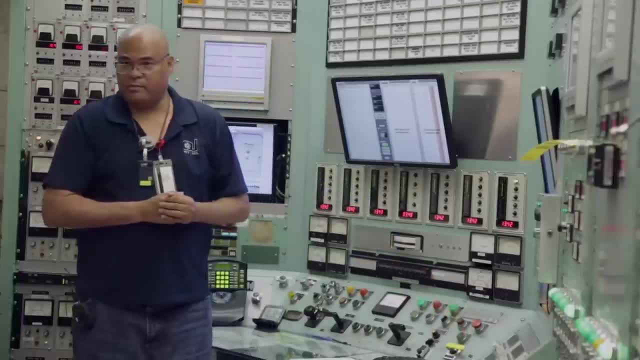 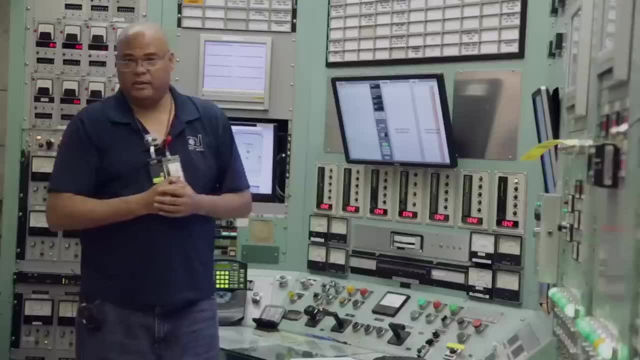 about nine different instruments that tell us what the reactor power is at all times, but the ones we're gonna be paying attention to are channel seven and channel nine. these two channels are what we use to basically tell us what the reactor power is. channel seven is what we control our automatic 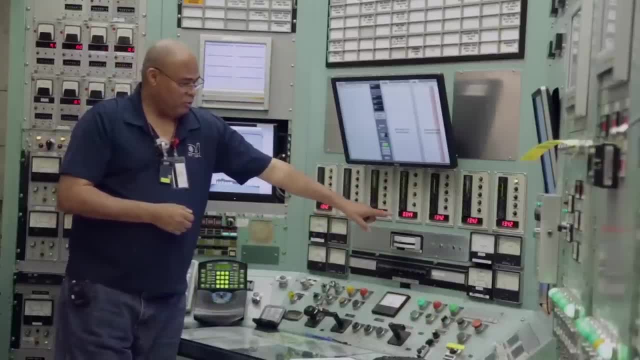 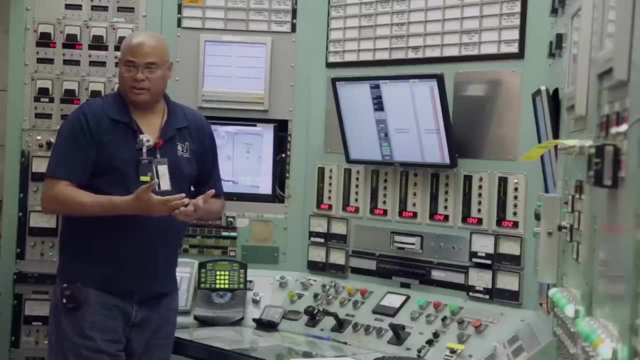 control at. if you watch the regulating rod, you'll see it move up and down on its own. that's because it's changing power based on what it sees channel seven is doing. so if channel seven sees that the power level is going too low, it'll cause the regular rod to drive. 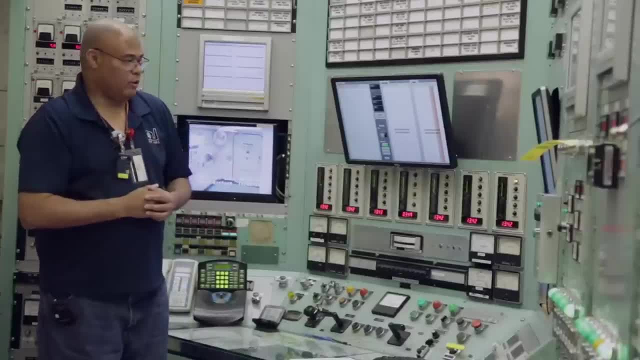 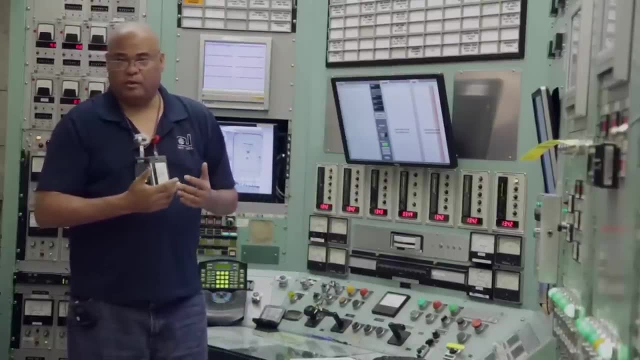 outwards to a increasing level of power for the regulator. there's also power in our locator ducts to increase the amount of neutrons, making the reactor power go up. Channel 9 is a linear power channel and it basically tells us what the power level is based. 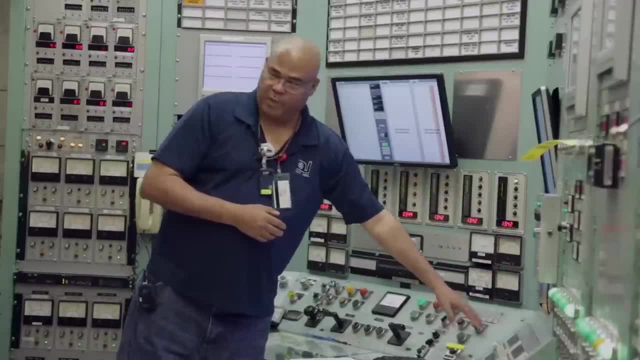 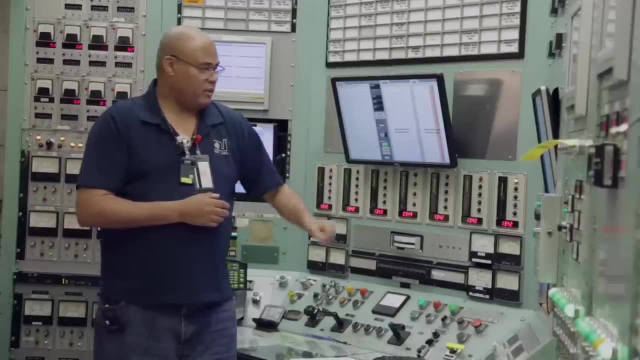 on a chart that we create. So it's not showing you megawatts or kilowatts or anything like that. it's showing you a current coming from a chamber and that current is then converted into megawatts and so forth. So right now we're at 500. 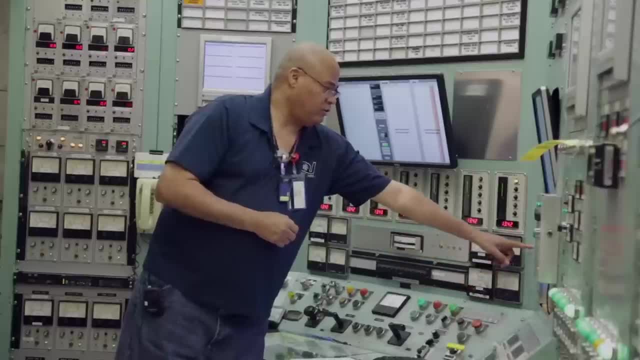 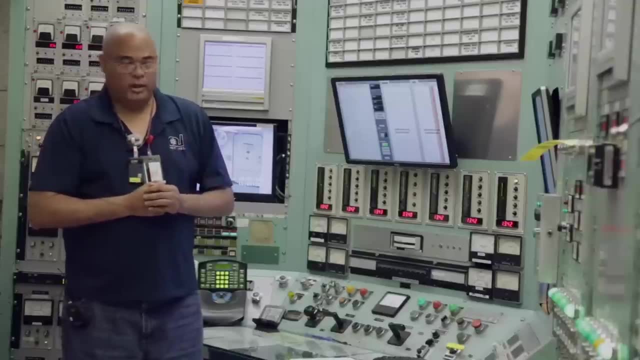 kilowatts, 8.5 microamps on this channel. and that's 8.5 microamps equals 500 kilowatts. You're going to be bringing the reactor up to 1 megawatt and since it's linear, it'll be double that, so 17.1.. Now you want to be careful when you 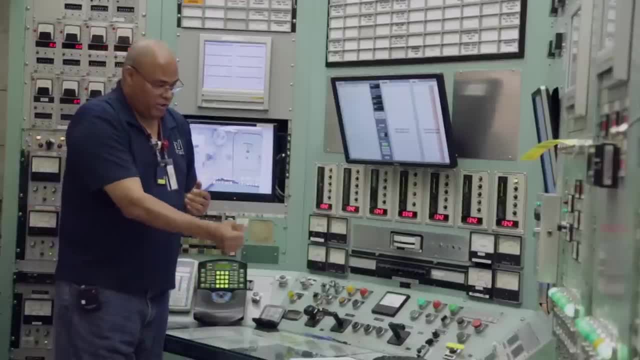 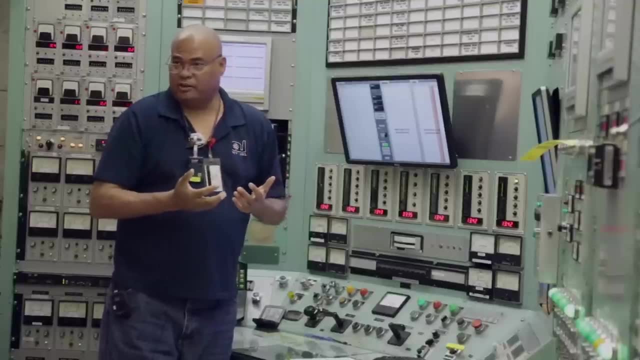 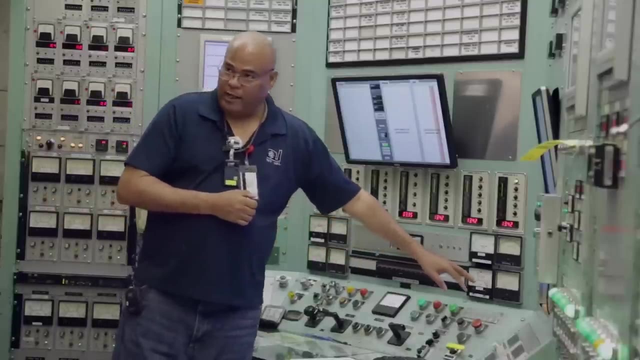 raise reactor power. so when you start to add power to the reactor by raising a regulating rod, you don't want to bring it. you don't want to keep raising it until you reach your value, because you have to actually stop the power increase as well. So we have two rules that we have to follow: One at the power level we're at. 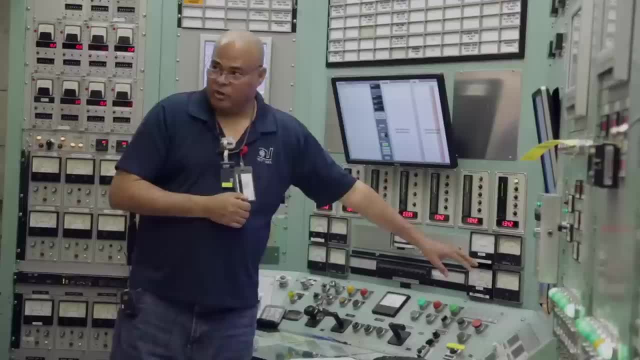 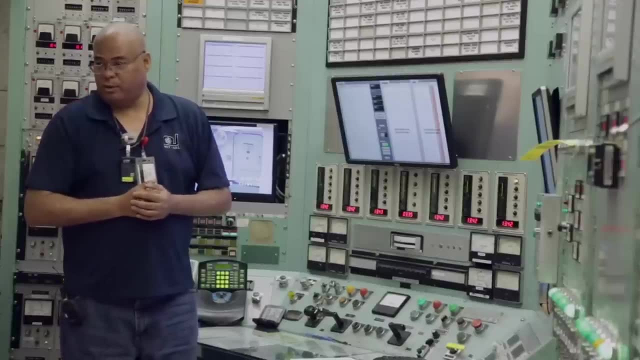 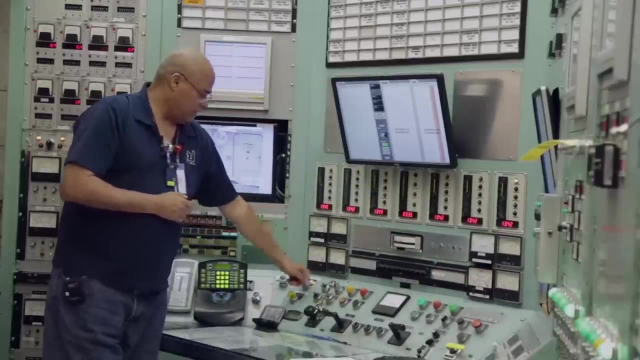 we have period, the reactor period. The reactor period is the amount of time it takes the reactor power to increase At the power level we're at. we're not allowed to go shorter than a hundred second period. Okay, so here is one of three period meters: one here, one here, which is selectable between two. 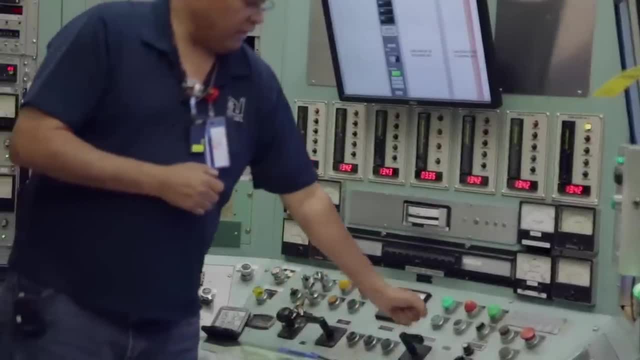 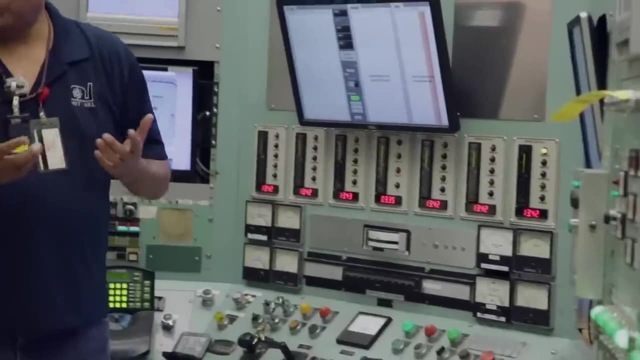 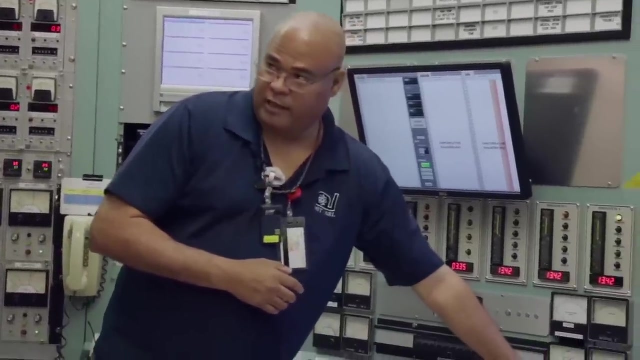 different meters. So as you're pulling up the regulating rod, one of the things you have to watch is to make sure that the reactor period doesn't go shorter than a hundred second period. If it does, you have to stop pulling blades. The other thing we have to watch for is to make sure that the power level- channel 9,. 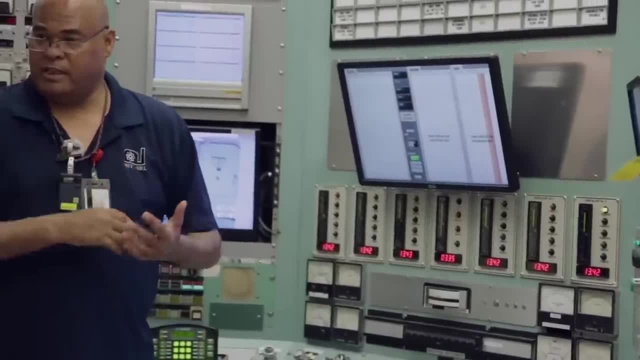 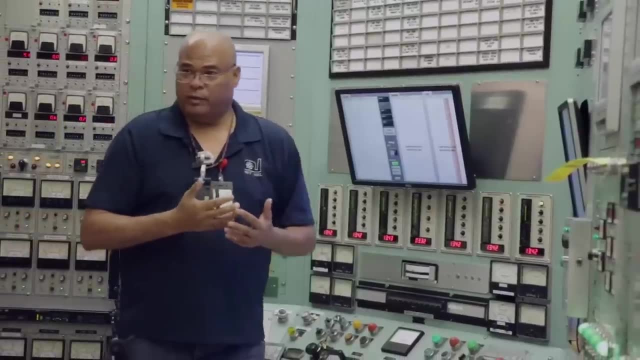 doesn't exceed where you're going to Not only not exceed, but we also want to make sure that you can actually control the reactor. It's called feasibility of control, and what that means is when you get to about 80% of the power level. 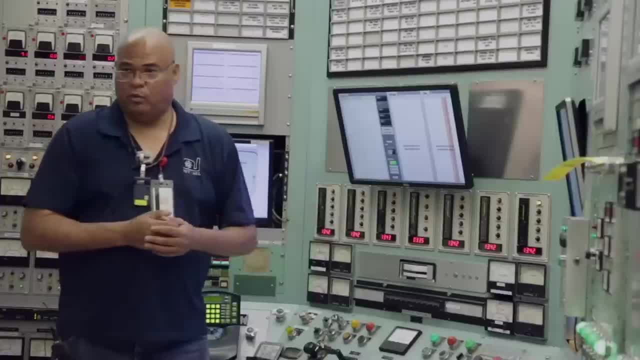 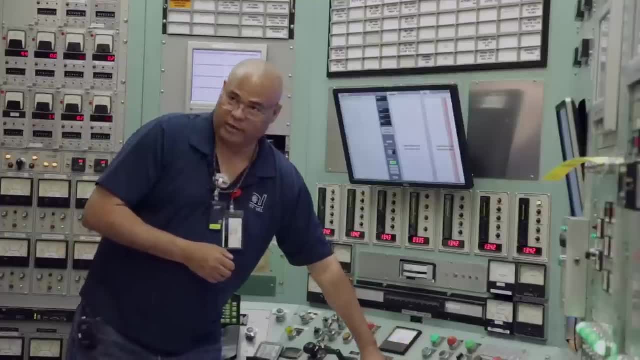 you're going to, since we're going up to 1 megawatt, that's about 800 kilowatts. you want to be able to drive the absorber in and hold the absorber in. You'll drive the regulating rod inwards and watch that channel 9 value It'll. 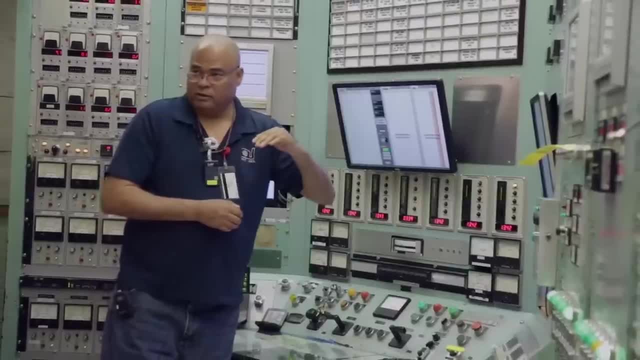 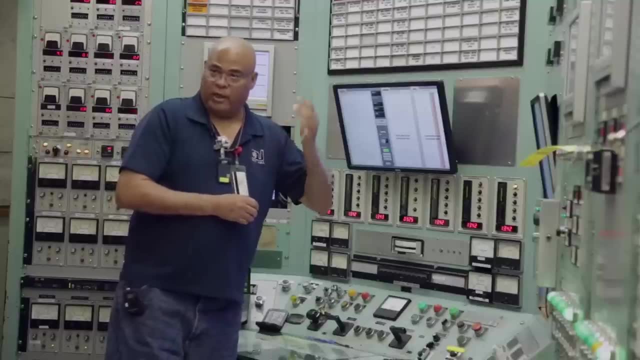 slow until it actually starts to go down again. Once it reaches that value and you see it going down, you now know that you could control the reactor and keep it from going away, React power increasing continuously. So what we're gonna do is, when you reach 80% of the power level you're going to, which happens to be 800 kilograms. 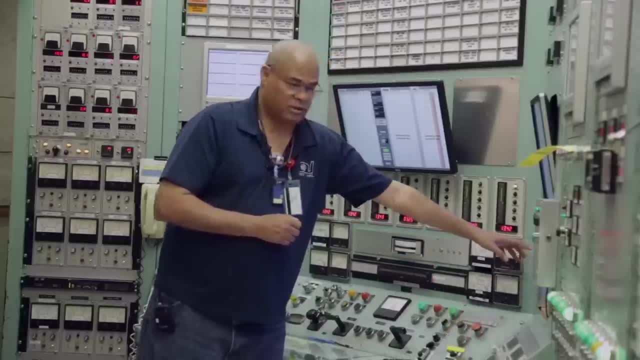 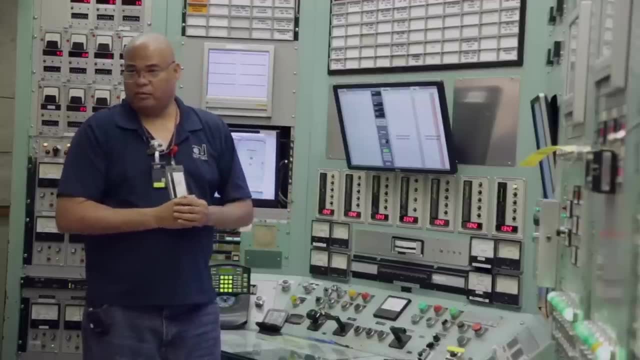 the power level you're going to, which happens to be 800 kilowatts, you're going to start increasing or lengthening the period by driving the absorber back in the regulating rod, And you'll keep holding it in until you see the number not only stop increasing. 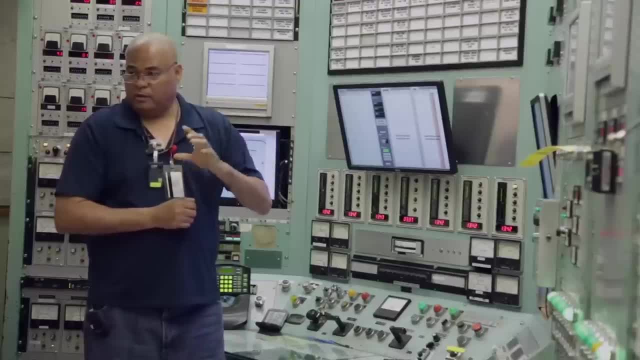 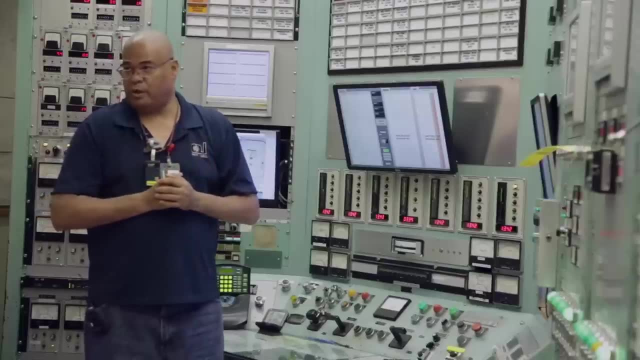 but actually go down a little bit As soon as you see it. go down a little bit. let go of the regulating rod. You haven't stopped the power at this time, You just decreased how fast it's going up, And then the power level will still go up. 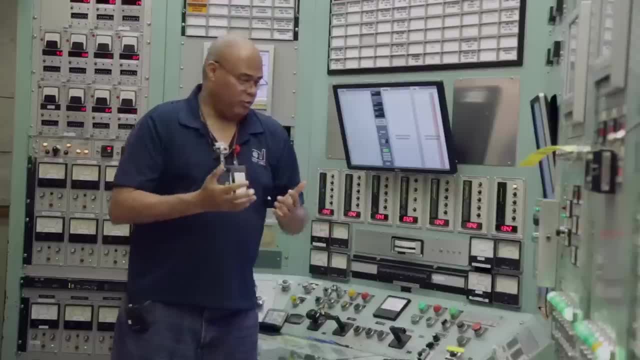 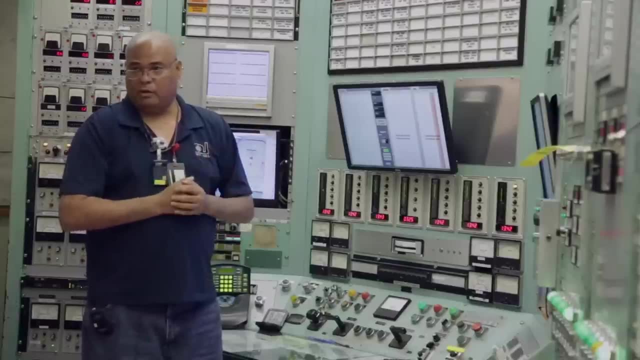 but a much slower rate than it was before. And once it reaches the power level you want to stop at the 1 megawatt, keep driving the regulating rod in to hold it at that power level. Once you're at that power level, you're. 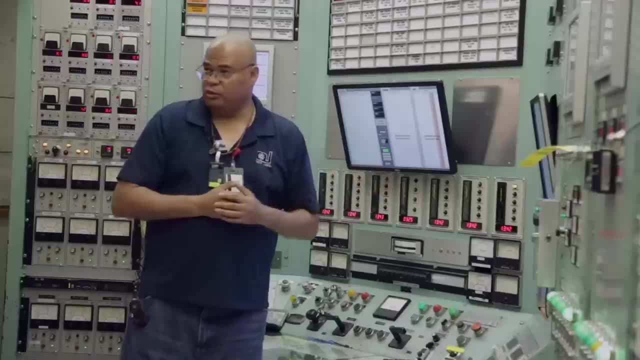 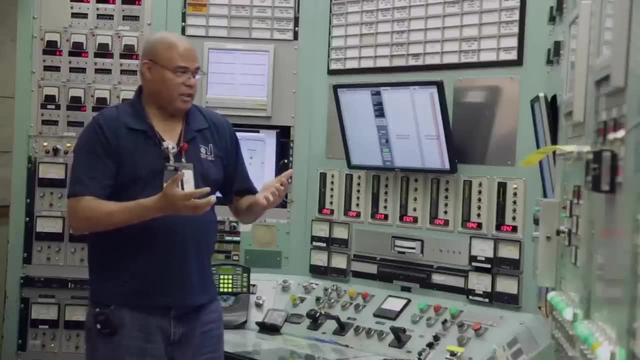 going to make an entry in the log book that basically says you made it to the power level you're going to, And then we'll go down in power. So once again you make an entry in the log book that says I'm going to lower react power to 500 kilowatts. 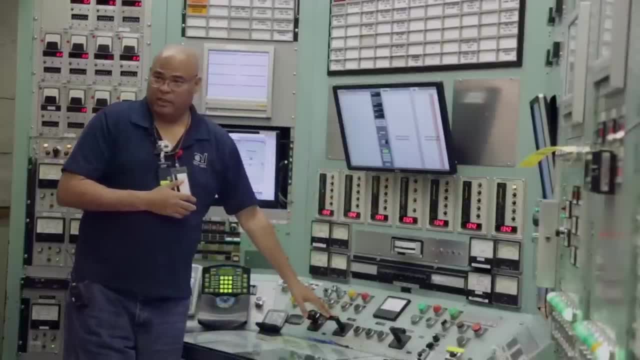 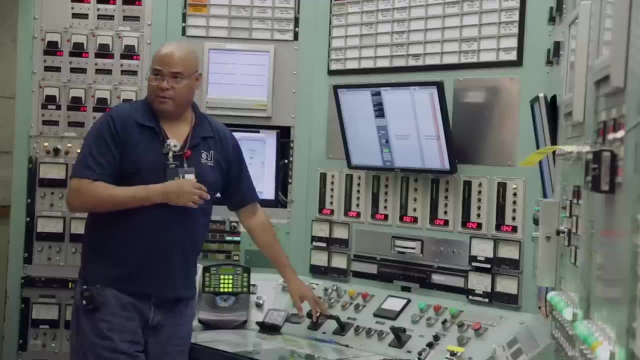 And then this time we'll use a shim blade. The shim blade is worth a lot more than a regulating rod- about 10 times the regulating rod. So things will happen much faster. So you'll be able to drive this in and react power will change much faster than before. 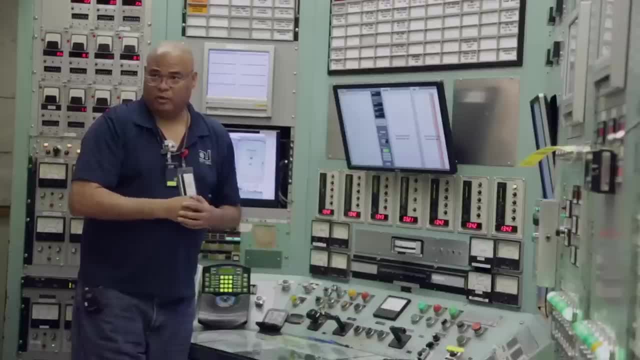 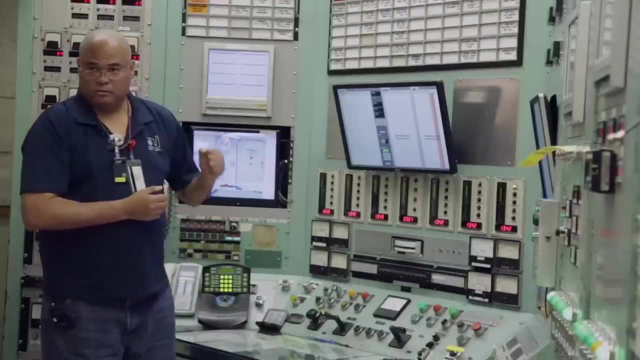 Same thing: as you get closer to the power level. you started at the 500 kilowatts. you don't want to undershoot and go too low. So at around 600 kilowatts or so, start driving the shim blade out to slow down. 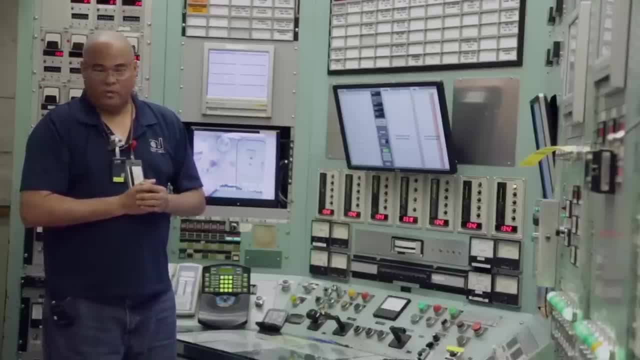 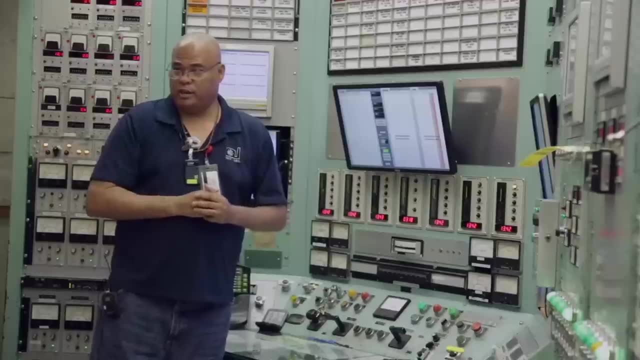 how quickly the power level is going down. And once you get back to the place where you started at, we'll use a regulating rod to fine tune it to keep the power where we want to be. There'll be another log book entry and your time on console will be completed. 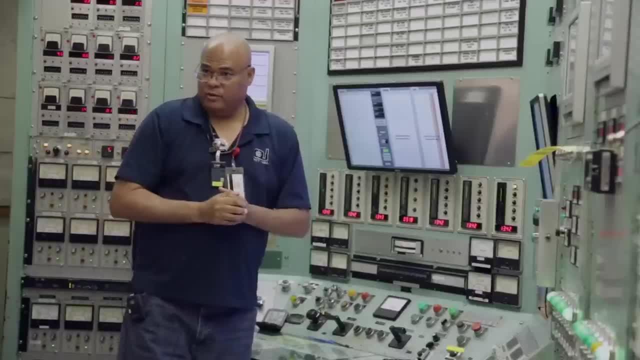 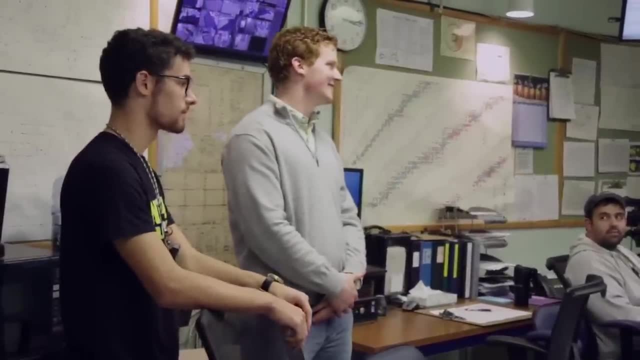 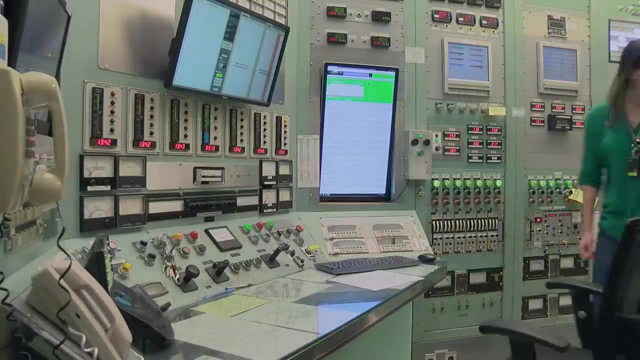 So with us today we actually have two MIT students who are actually in my training program And they've actually done a lot of work and a lot of these manipulations already. Sarah, let's go. It's been so long since I've done one. 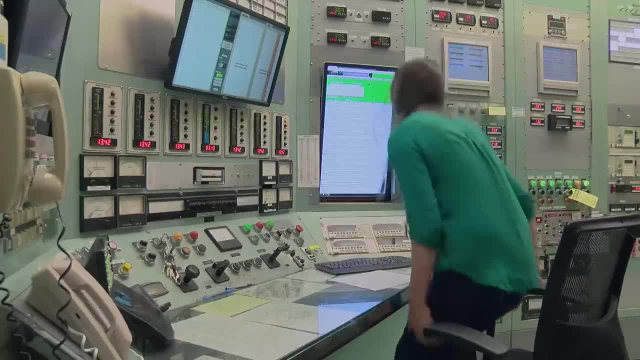 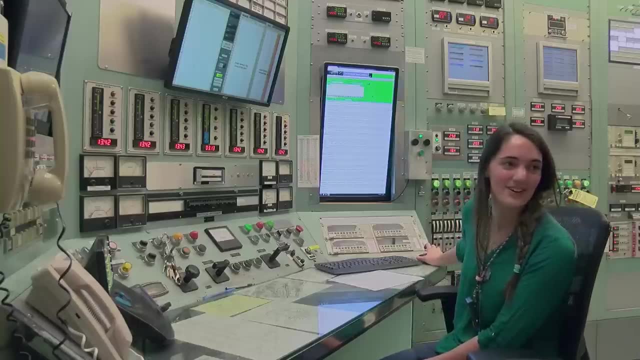 I'll take that one. So normally we sit and watch. If at any time you don't feel comfortable doing something, let us know. We'll ask you just to take your hands off the console and we'll take care of doing whatever is necessary to keep. 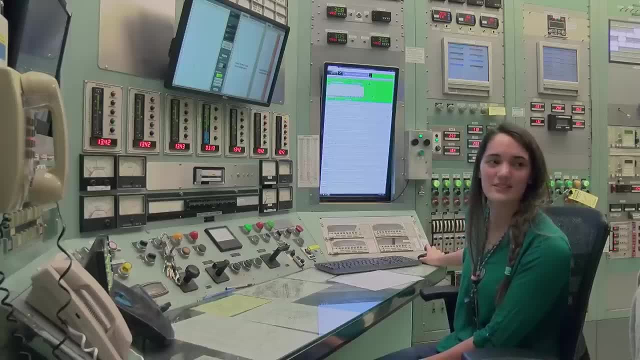 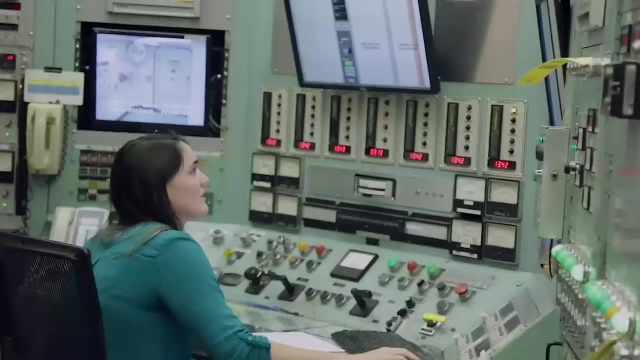 the reactor safe, But be aware we're a factor, we're 10 lower than where we would automatically scram at, so it'll be very difficult for you to get to some place. 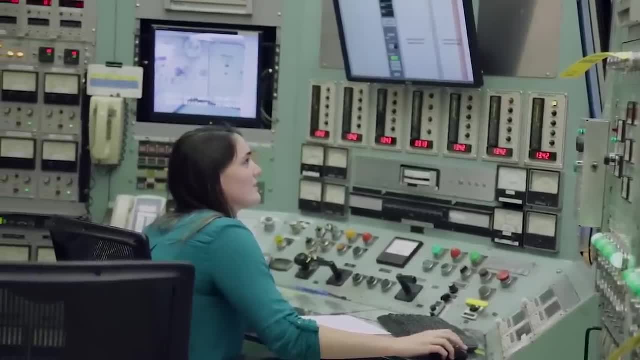 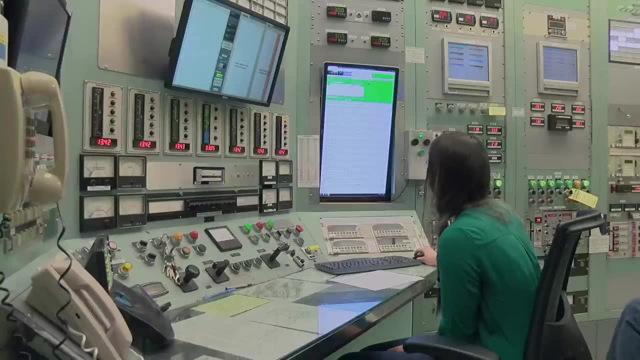 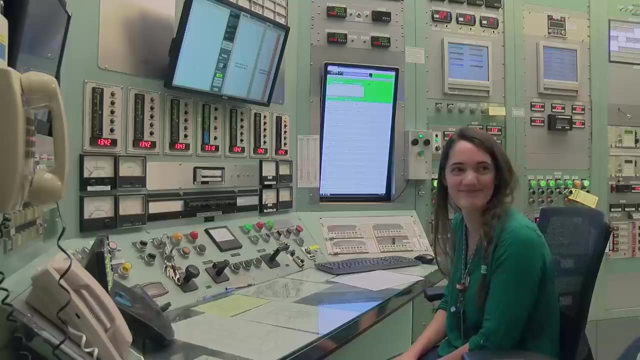 where we would cause a problem without us being able to stop it. Okay, so our normal. I don't know if you want to move or anything, but the supervisor normally sits kind of right in your way so that they can keep an eye on what's happening. 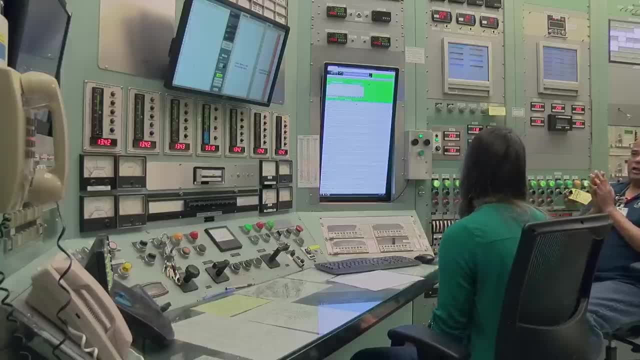 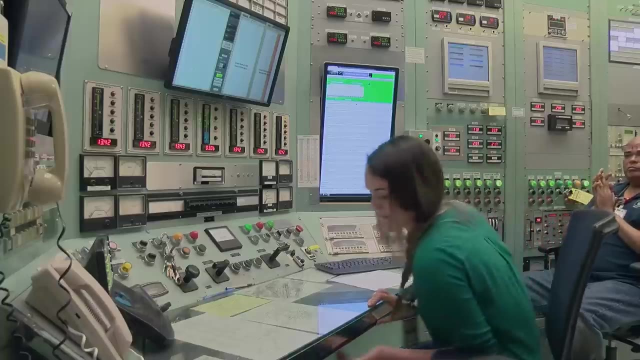 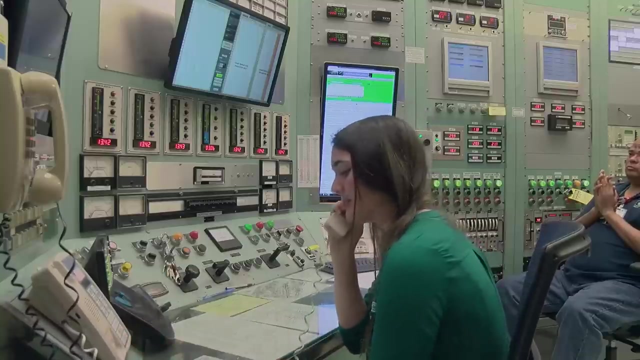 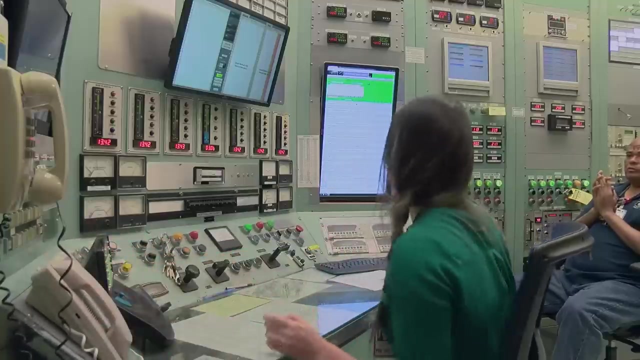 You can go ahead and make the announcement that you're that we're starting power manipulations, and then the last person make an announcement that we're done with power manipulations. Commencing power manipulations. Commencing power manipulations. Commencing power manipulations. 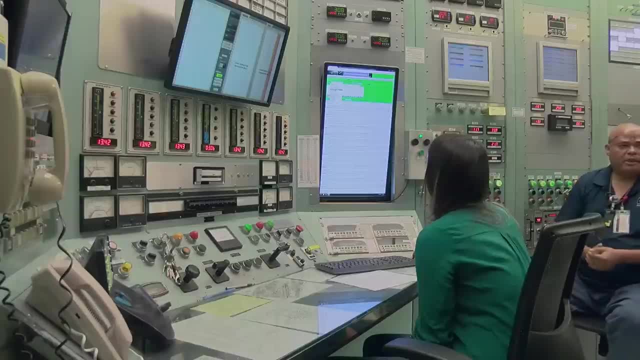 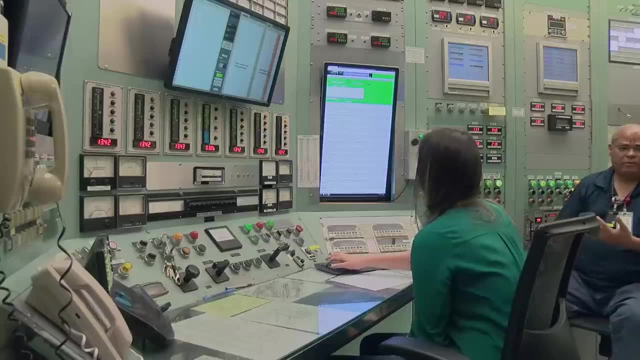 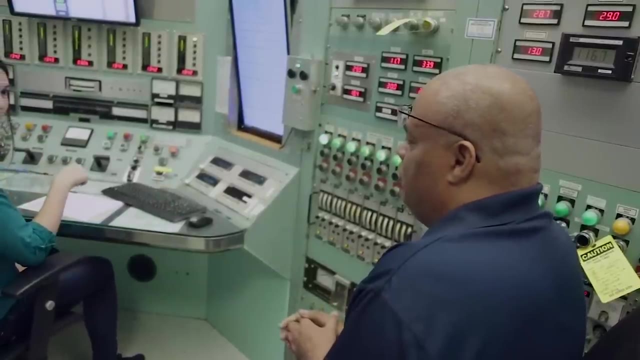 Right now the reactor is on auto control and when we do these manipulations, the reactor operator is going to take manual control. That will cause an alarm to come in, and this will only happen for the first time. So one of the things she's going to do after she makes her log book entry: no, we'll do. 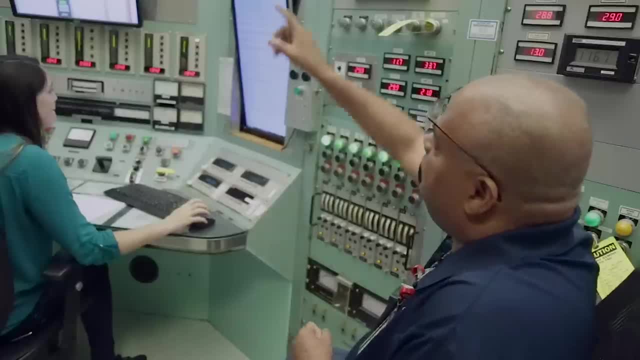 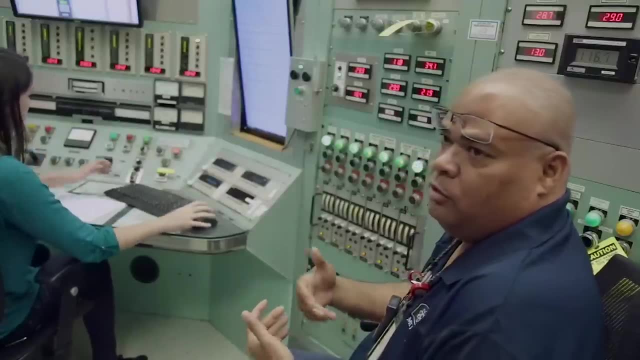 that at the end is she'll take manual control of the reactor. An alarm will come in on console and she'll answer it, and that should be the only time you hear this alarm, because we'll leave it on manual control until the final participant has done their manipulations. 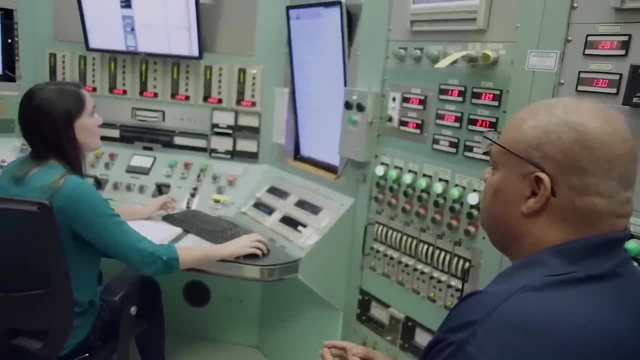 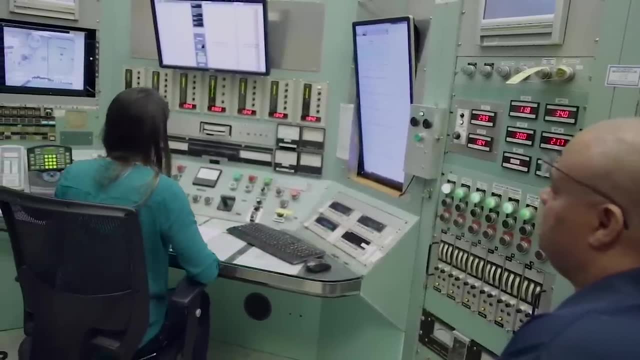 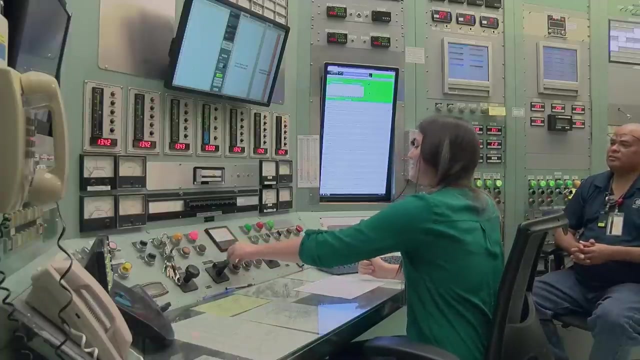 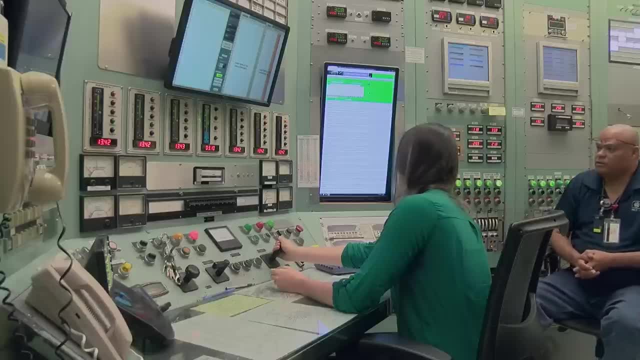 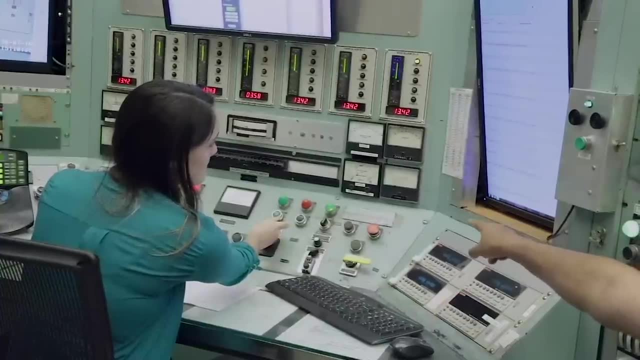 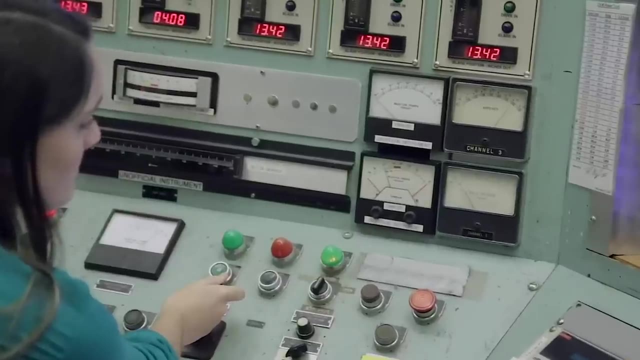 Okay, Okay, Okay. Now she's pulling up the reg rod all the way. you see the reg rod number going up, the period is getting shorter, it's no longer infinity, it's going closer to a hundred seconds, and channel seven and channel nine are increasing in value. 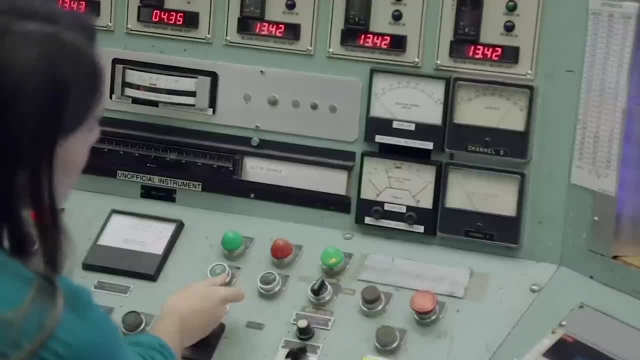 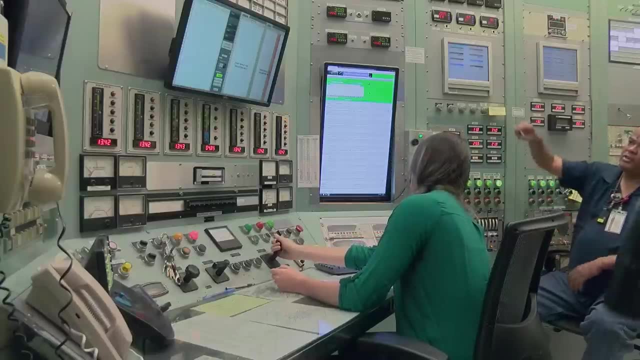 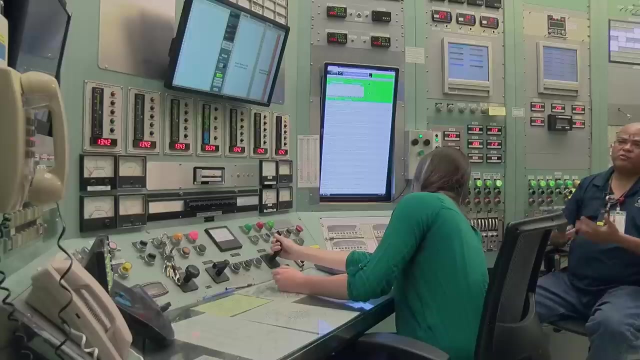 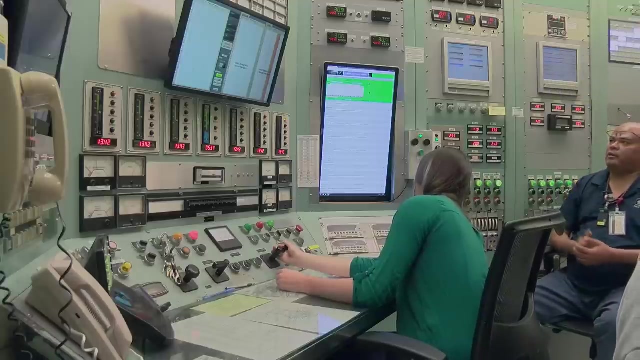 Okay, great, Okay, Okay, Okay, Okay, Okay Okay. Another way you can see it is: we have a display in front of the operator. Those three displays, two of them are just for evaluation only. We don't actually use those to control the reactor. 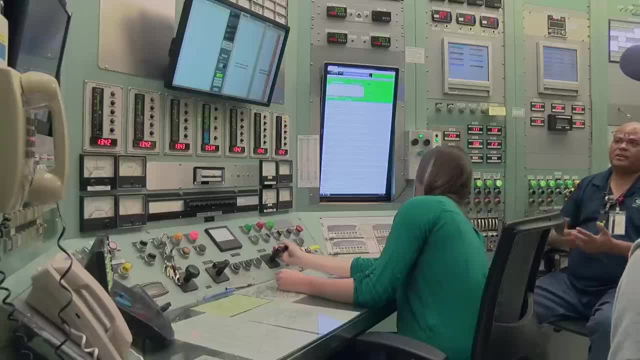 They're based on a system that hasn't been approved yet, but we're testing them to see how well they work. So you can see that the power level on the far left is going up. The middle one is showing what the actual power level. 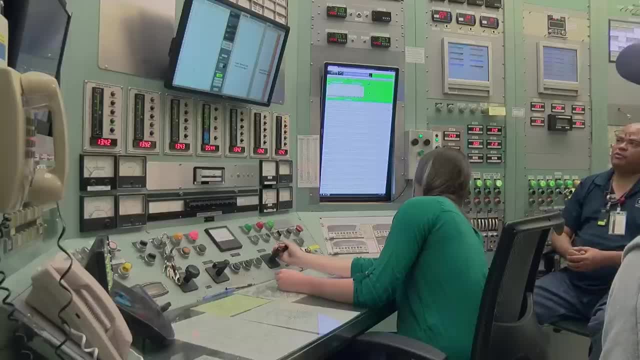 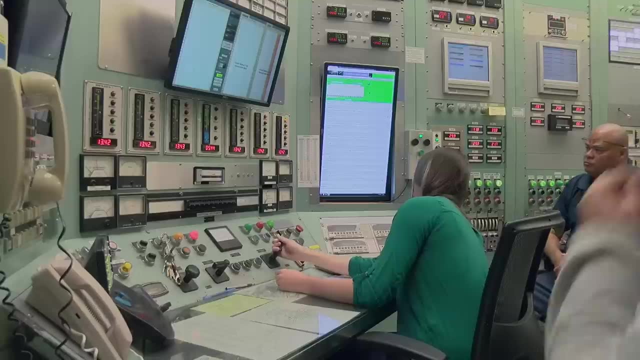 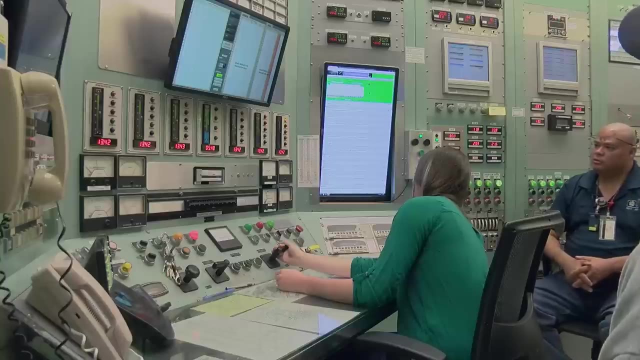 We saw 500 kilowatts. It's already up to 630 kilowatts and increasing, And the period that was at infinity is now around 160 seconds. So she's watching And so she sees the 800 kilowatt. 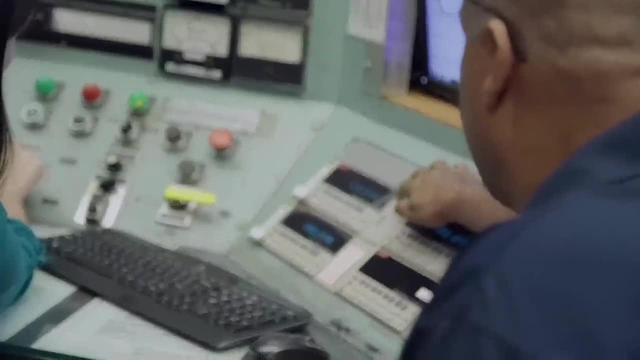 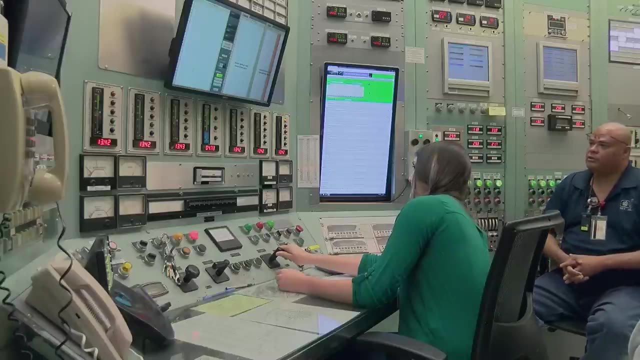 That value here on channel seven or channel nine And she started to drive in the regulating rod. So she's slowing down how quick the power increase is going And you see the period lengthening. It's no longer at 150, 160 seconds. 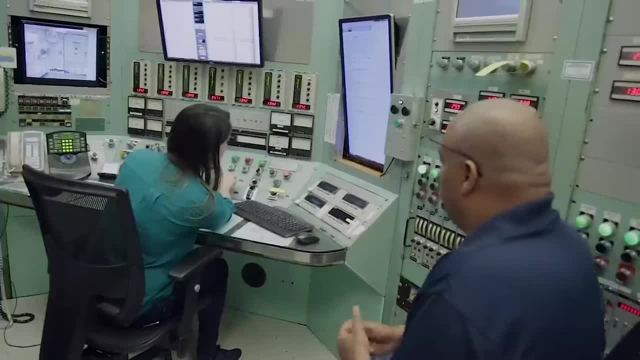 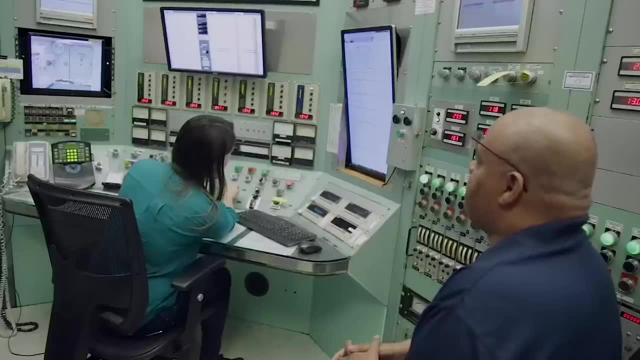 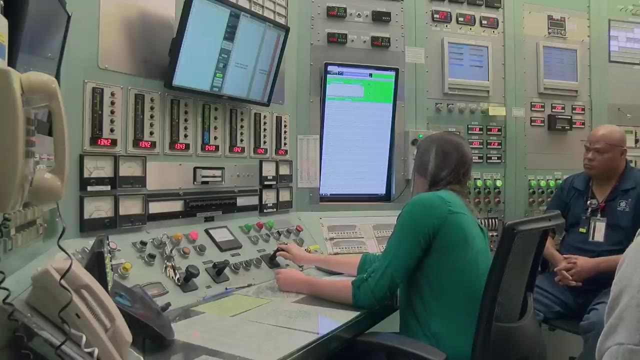 It's going closer to infinity again. So she's proving that she could stop the reactor power if she continued driving in this regulating rod. 07. 08. 09.. 010. 012. 013. 014. 015.. 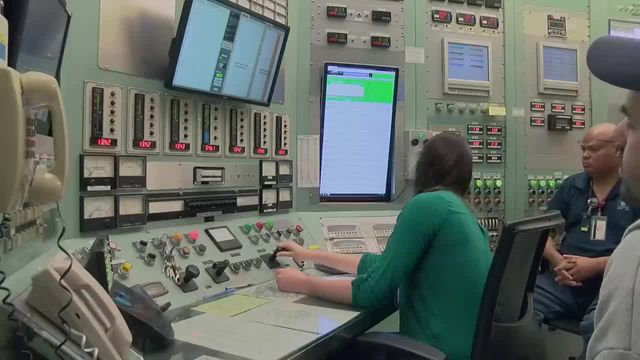 016. 017. 018. 019. 020. 021. 022. 023. 024. 025. 026. 027. 028. 029. 030. 031. 032.. 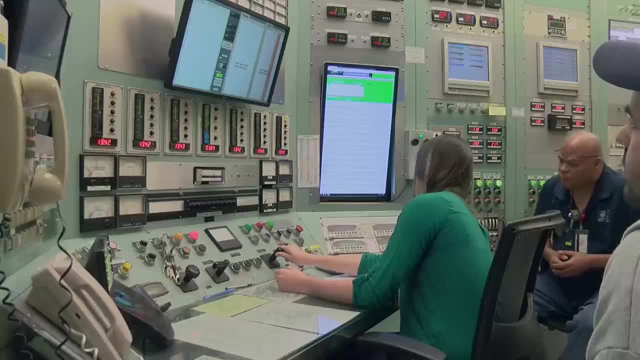 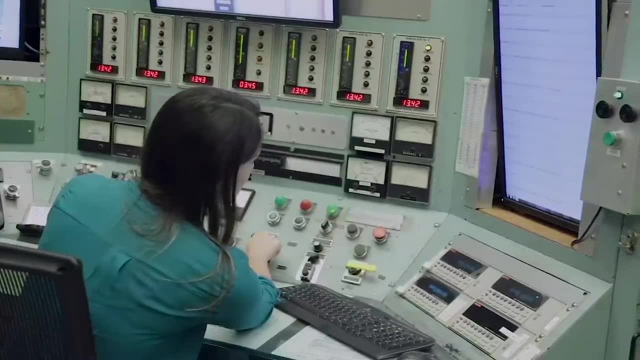 033. 034., 035. 036. 037. 038. 039. 040. 041. 042.. 043., 044., 045. 046. 047., 048. 049.. 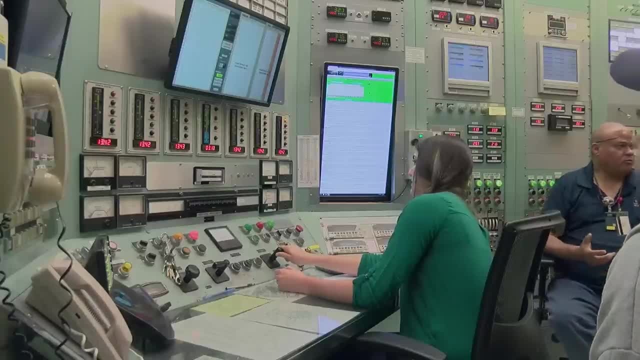 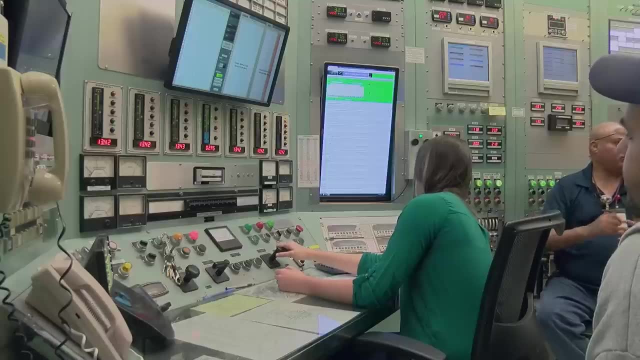 050., 051., 052., 053., 054., 055., 056., 057., 058., 059., 059., 060., 061., 062., 063., 064. 065.. 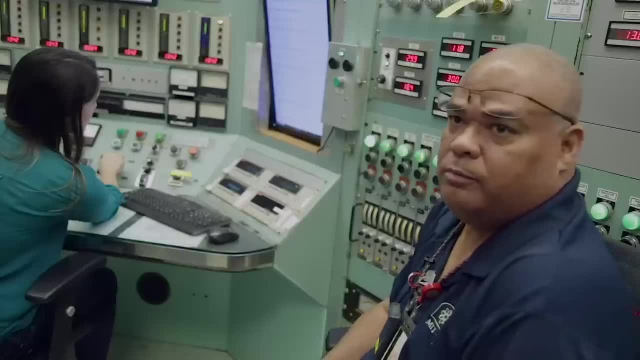 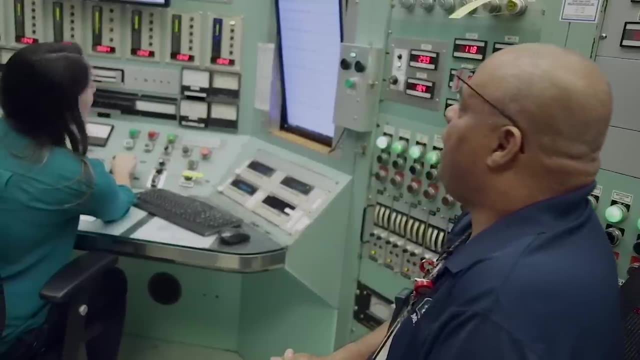 067. 068. 068. 069. 070. 071. 072. 072. 073. 073. 074. 074. 075. 076. 076. 078. 079.. 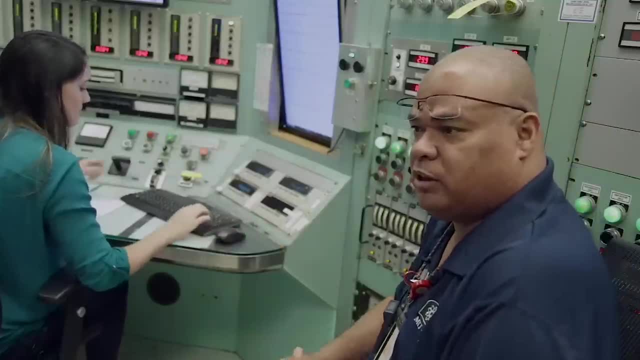 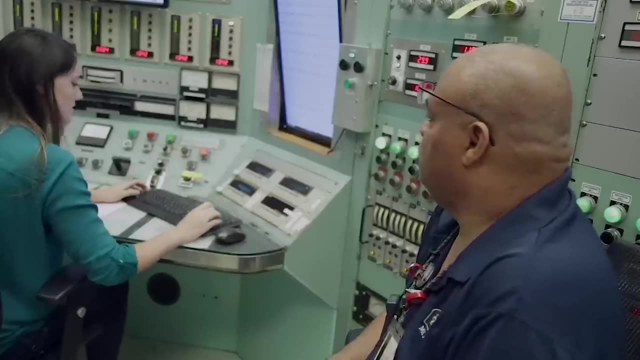 079. 080. 081. 082. 082. 083. 094. 095. 096. 097. 098. 099. 090. 021. 022. 023. 024.. 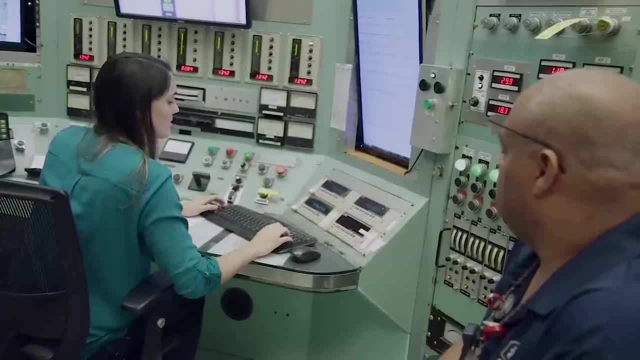 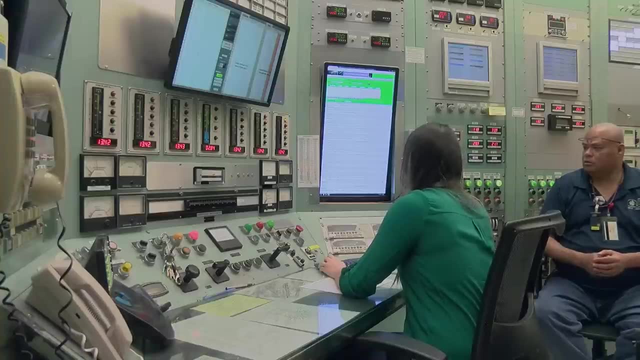 025. 026. 027. 028. 029. 030. 033. 034. 035. 036. 037. 038. 039. 040. 042.. 044. 045.. 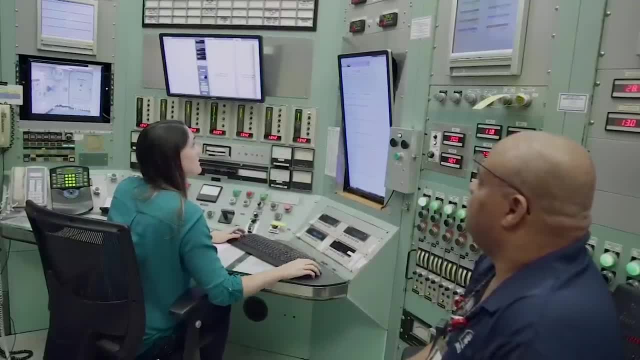 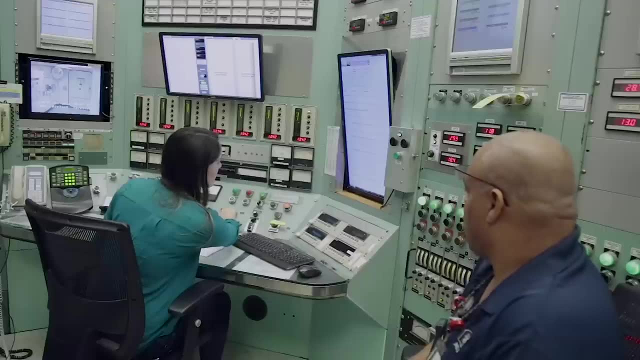 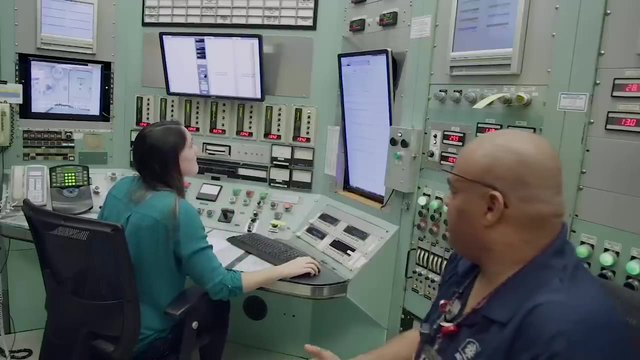 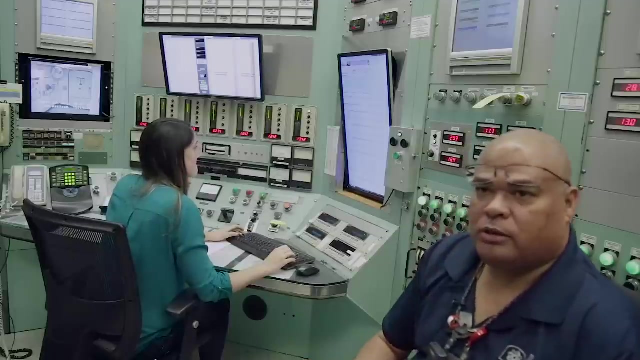 046. 048. 049. 059. 050. 050. 055. 052. 056.. So one of the things that could change the reactor is xenon. it's a poison that builds into the reactor while we operate. 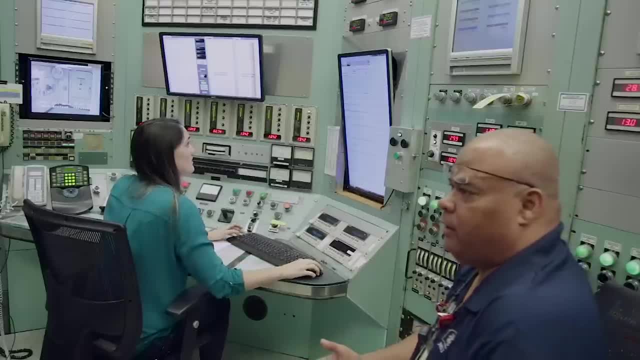 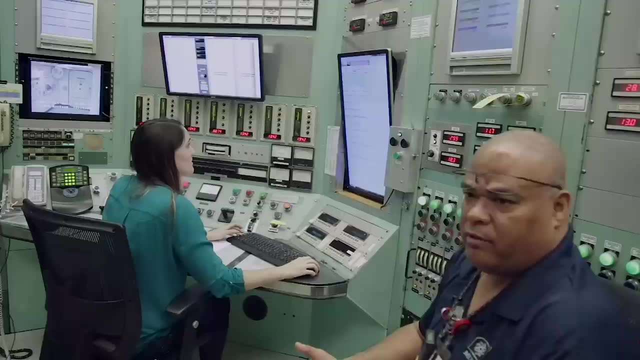 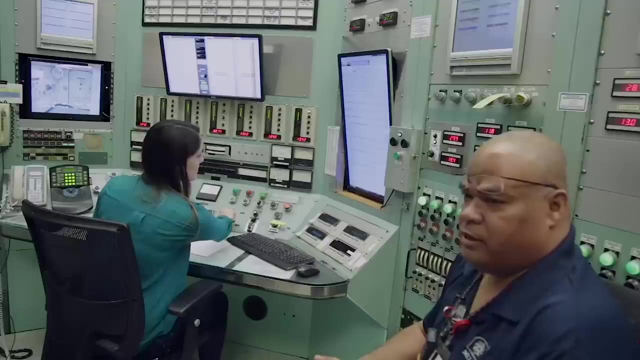 Poison in that it absorbs neutrons, not leading to fission, and it has two ways of being made and two ways of having removed. One is direct from fission and the other is decay. That's the way it's produced. the way it goes away is basically absorbing a neutron and 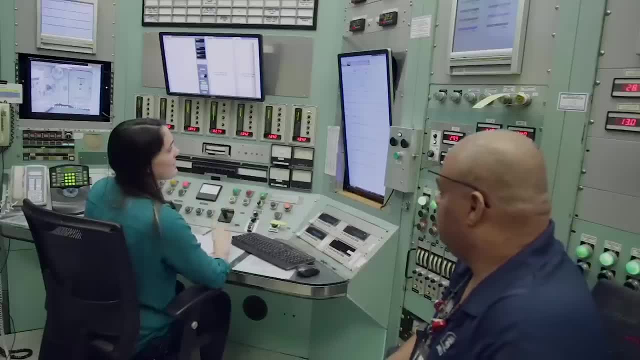 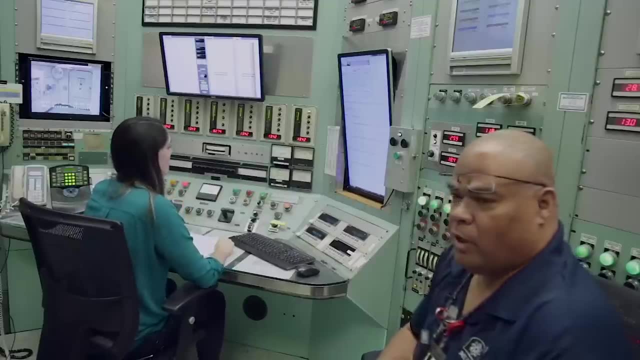 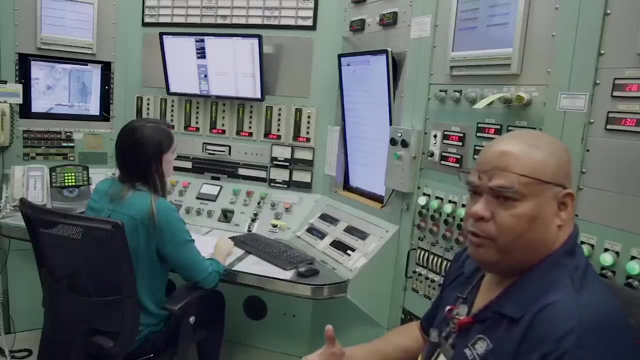 decaying to another isotope. I'm going to take it to half a megawatt at 8.56 microamps and use the same shim blade. Yep, use blade six. What happens is when we lower reactor power, the way we remove most of the neutrons is 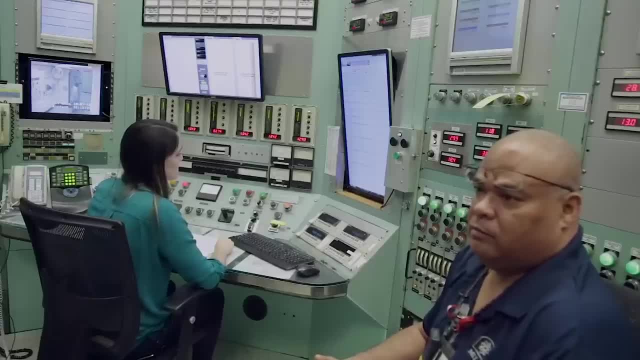 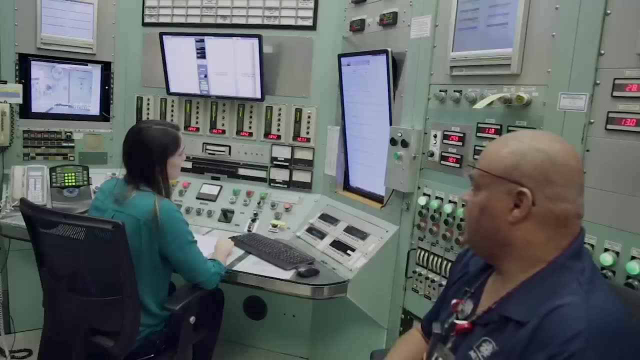 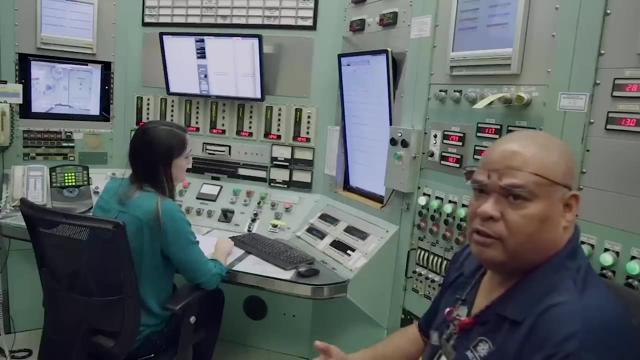 the same, Most of the xenon from burn up, basically the neutrons being absorbed by the fission process. the fact that we don't have the reactor at a very high power means that the amount of xenon in the core isn't being removed. 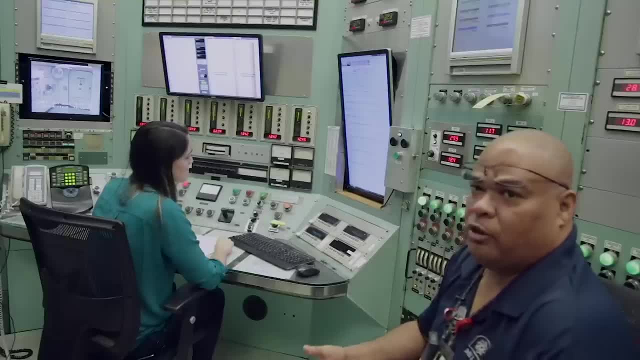 So we actually start. the power would actually want to go down on its own, So you would have to do a lot of regions and, for a while, A very large amount of reactivity that has to be compensated for. For this experiment, though, we actually shut down the reactor yesterday and we started. 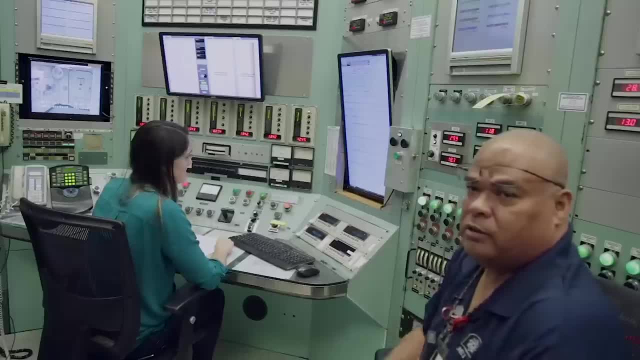 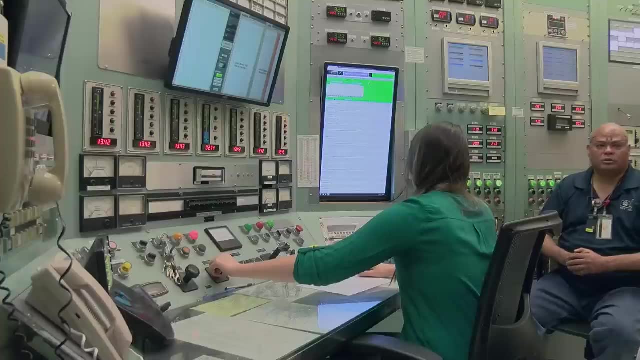 up early this morning, so it's not a big factor, as it normally would be after doing one of these lowering reactor power. Do you want to have her do a re-shim now, or do you want me to? No, I think we'll be able to get at least one more person. 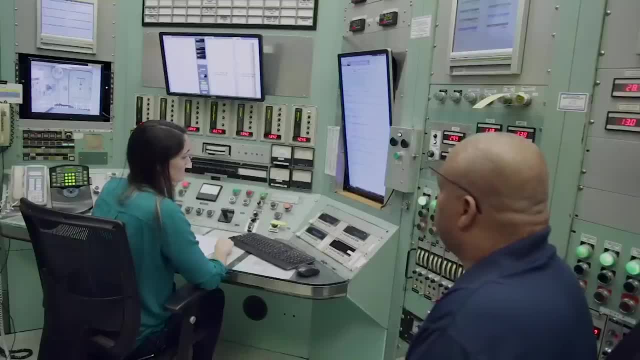 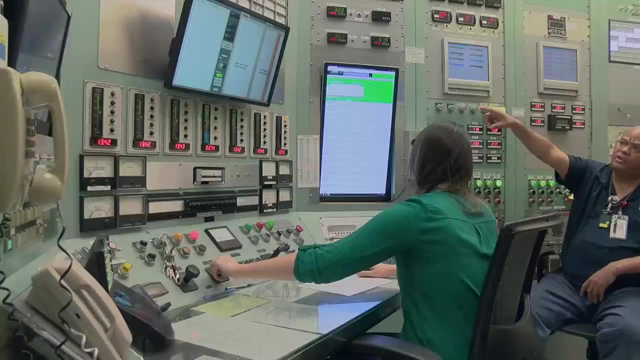 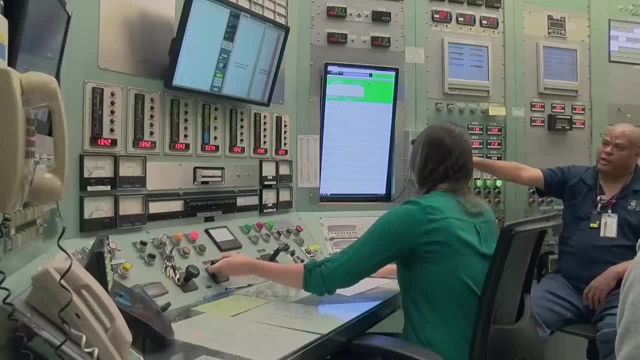 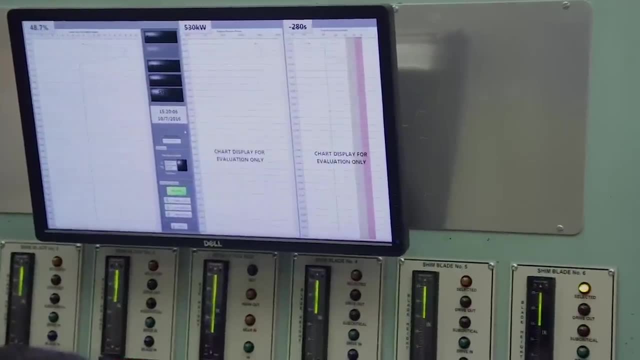 She's driving the absorber out again to slow down how quickly the power level's going down, And when she's done, the shim blade will end up about at the same point where it started, the 13.42 inches out of the bottom of the core.